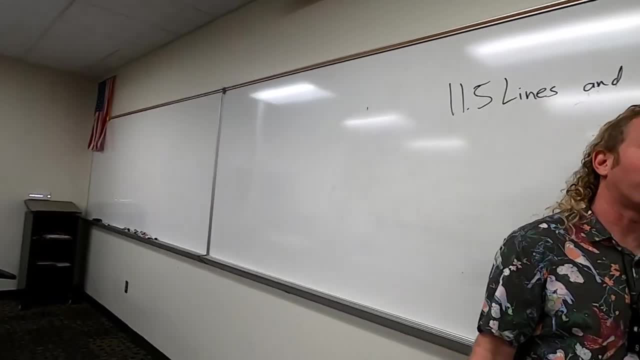 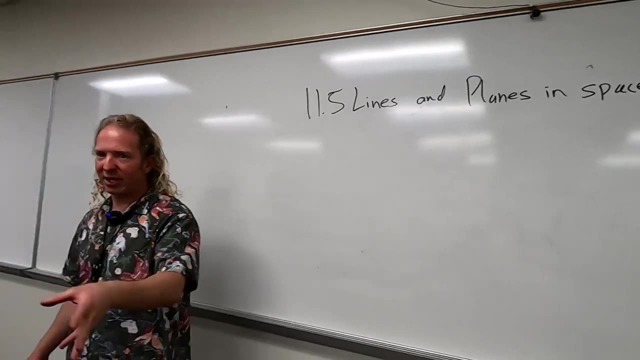 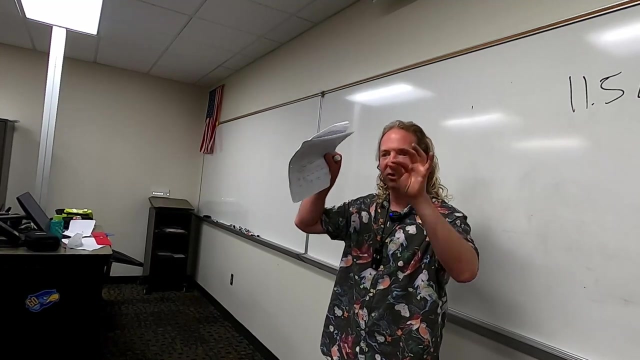 In two dimensions, if you have a point and a slope, you have a line right. In three dimensions, if you have a point and a parallel vector, you have a line. So in 3D, given a point on the line and a parallel vector, you can get the line. 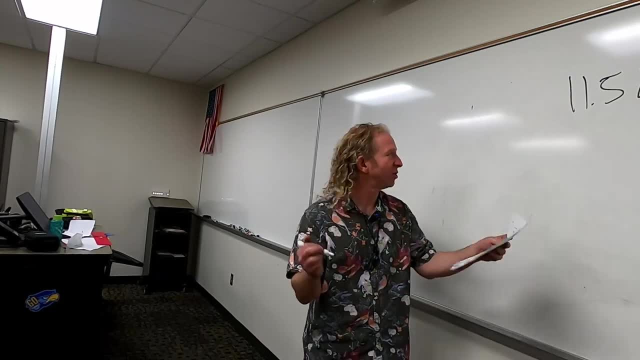 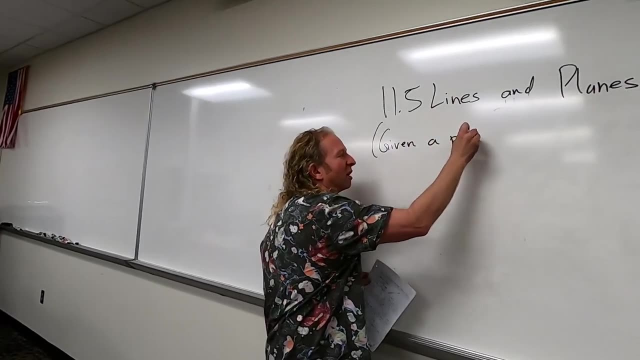 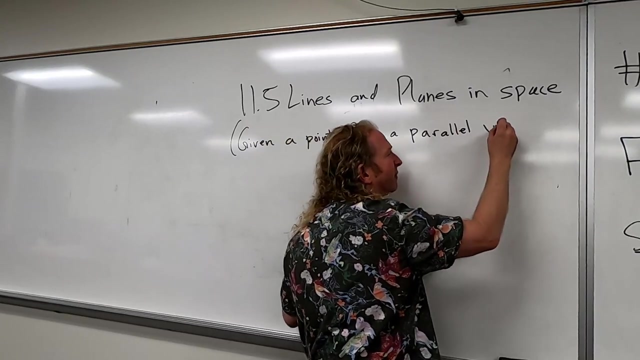 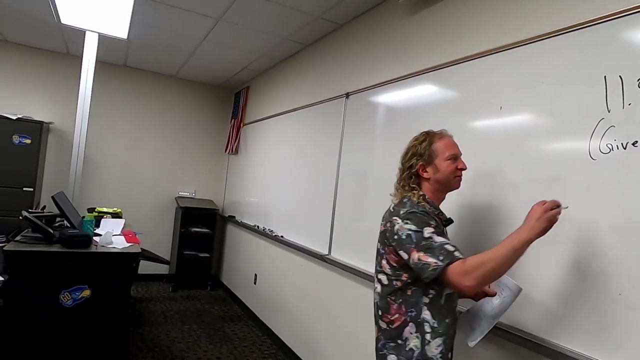 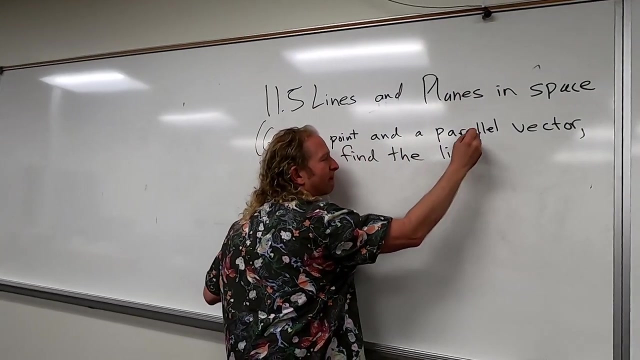 We're going to derive it from scratch, Like from scratch, So let's do it. So I'm going to write that down. So, given a point and a parallel vector, we can find the line. Okay, we can find the line. 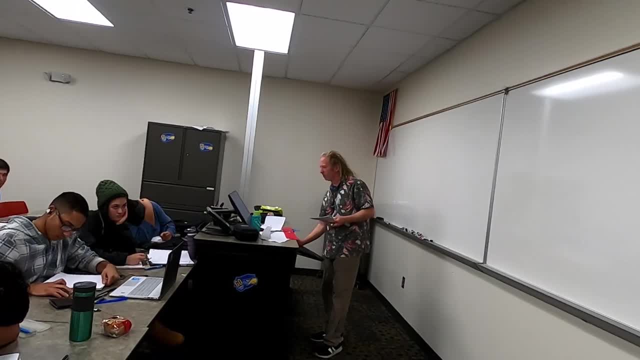 I'm going to make sure I can see the homework too, Because this is 11.4.. I'm probably going to need to at least look at some. I didn't write anything down for homework problems. I have notes, but not. 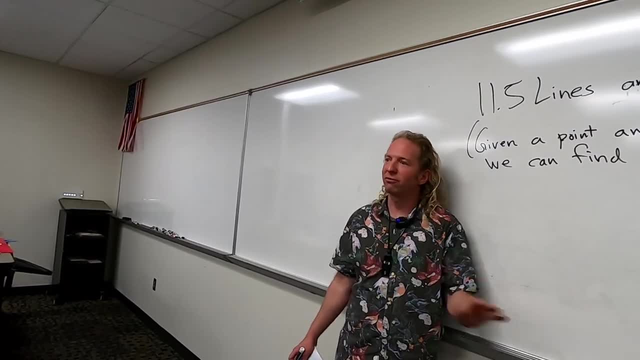 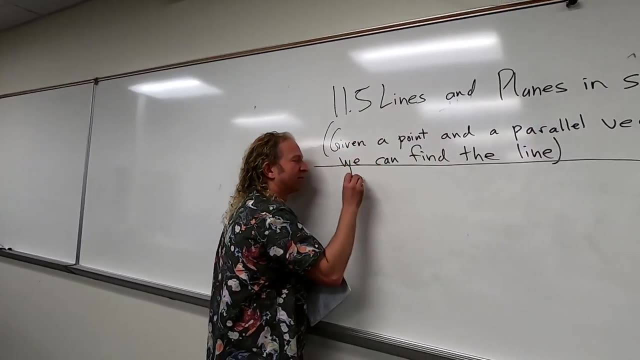 Alright, so let's derive it. Let's derive it from scratch, Like from nothingness. I wanted to use that word. So lines, We're deriving lines. So lines in space, Right, Like in three dimensions. 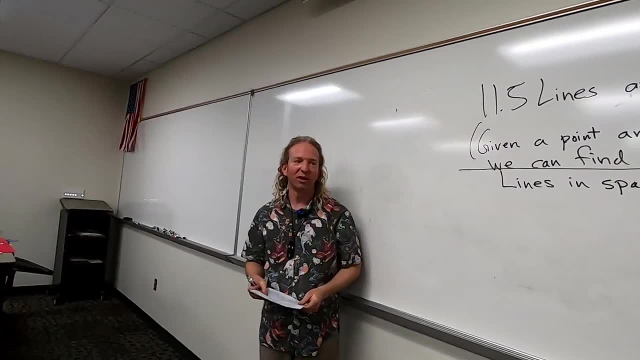 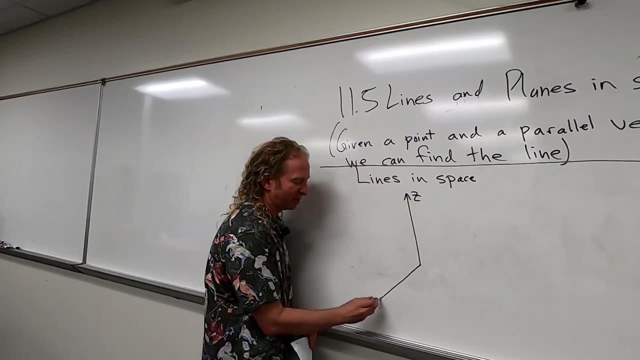 So an actual, like physical line. Alright, It's kind of cool, Okay, so this will be the z-axis. Okay, this is the z-axis And this will be the x-axis And this will be the y-axis. 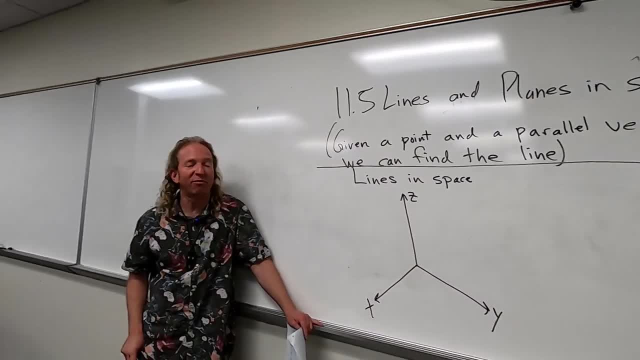 I'm going to go through it really slowly. So x, y and z. We'll also derive planes. We'll do some derivations in this class. It's kind of fun The ones that are like reasonable to do. 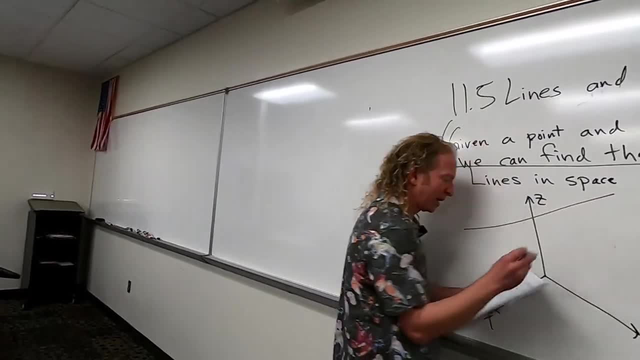 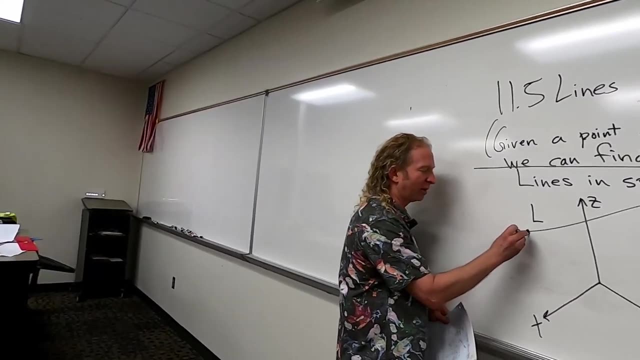 And then, so maybe here's our line, There's our line, So we'll call it L. There's our line, L, And I guess we need a point on the line, So I'm going to call it P. 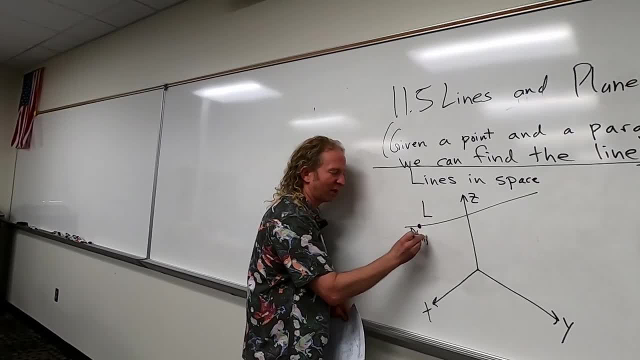 And I'll stick to the book's notation where they put a parentheses And an x1, and a y1, and a z1. They like to do that. They put a P and then the parentheses and they put the point. 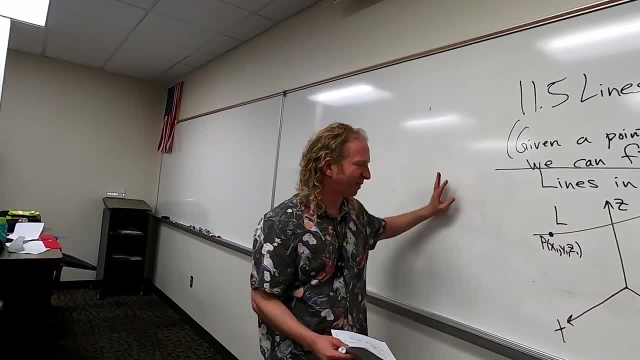 I don't know why they do that. They just put P equals, but it's whatever. Okay, And so that's going to be the point. Like we'll have those numbers Like 1, 2, 3, 4, 5, 6.. 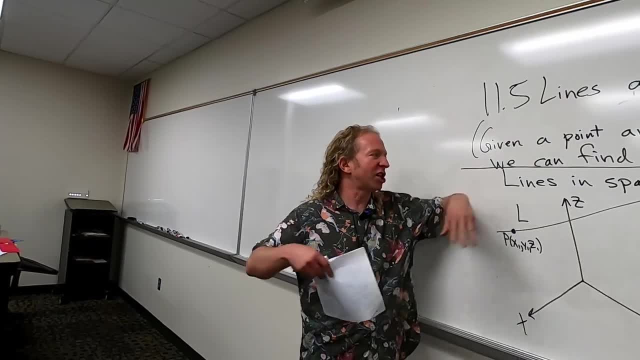 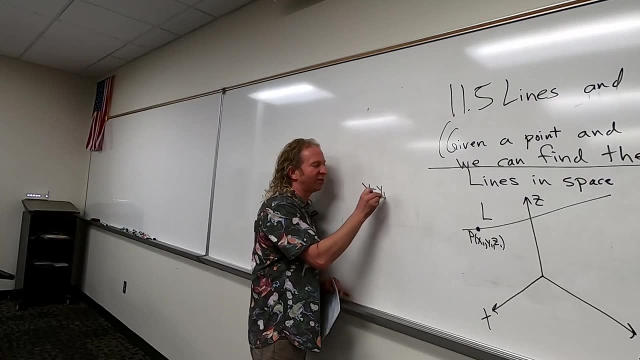 We're going to plug those in to the equation. Then you need, like, you need a generic point on the line Like you know, if you think about like, if you think about like the equation of a line in 2D. 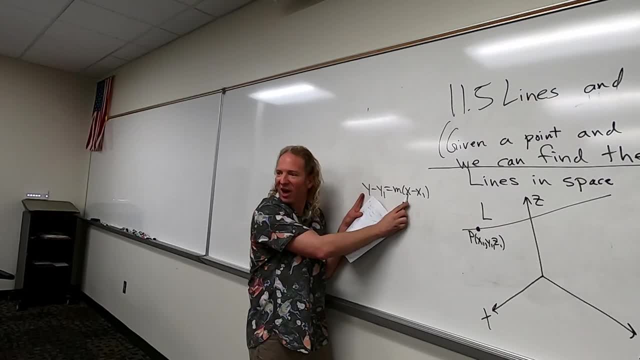 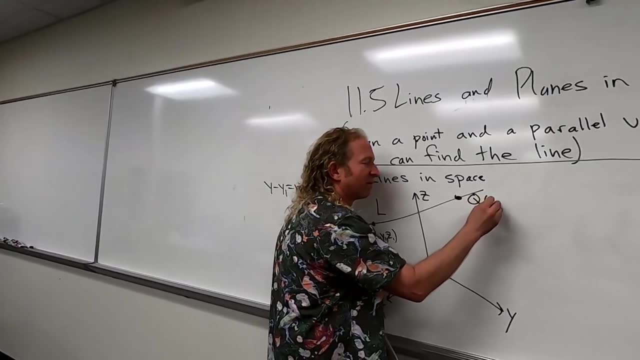 Like you got to have the x1 and the y1, but you also have to have the x and the y, Right, Right? So I need another point, Right? So I'm going to call that Q. So what we're going to do right now is true for all: x, y, z. 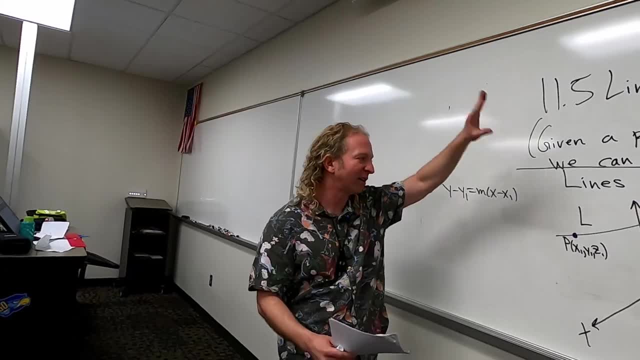 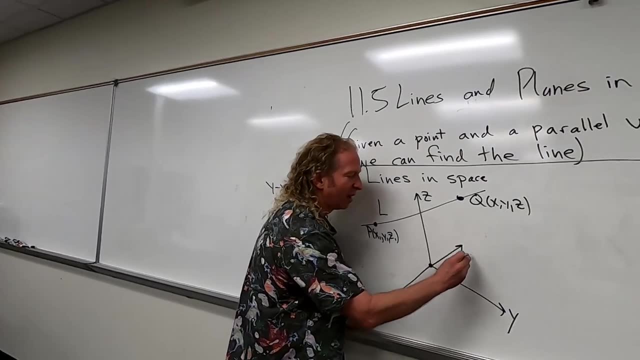 So what follows is true for all Q. So, for all points Q on the line, the following is true: Oh, we also need a parallel vector, Right? So I'm going to draw our vector here. There's our vector. 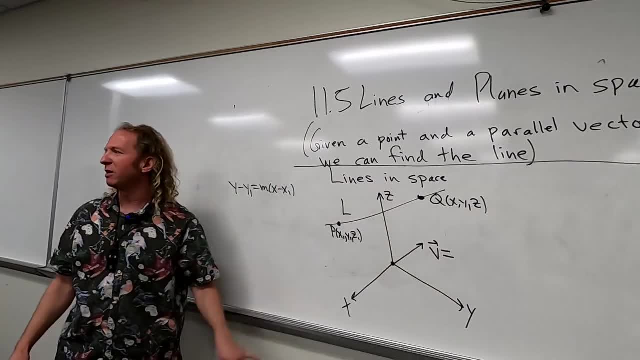 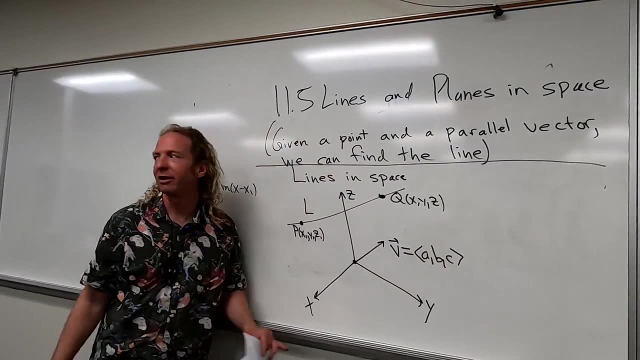 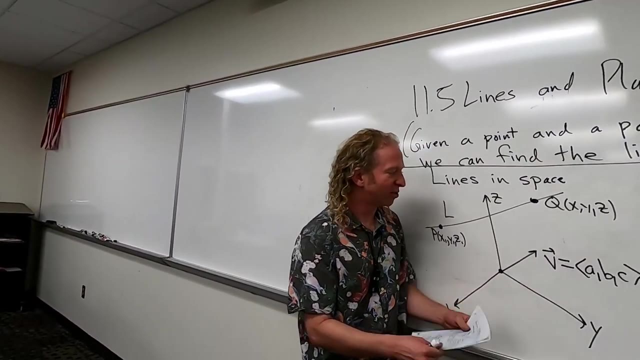 And let's call it V, And let's give it nice names. How about ABC, ABC, ABC is one, two, three, ABC, ABC, ABC. This, this has a name. This is called a direction, This is called our direction vector. 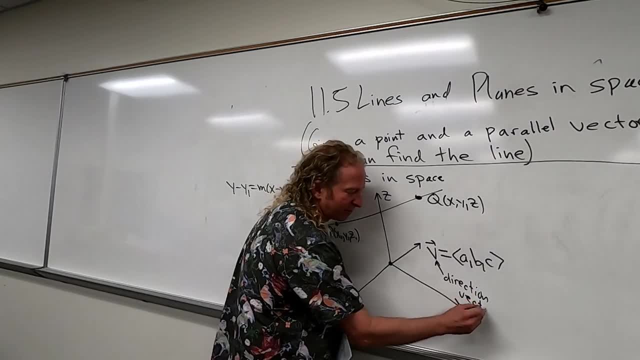 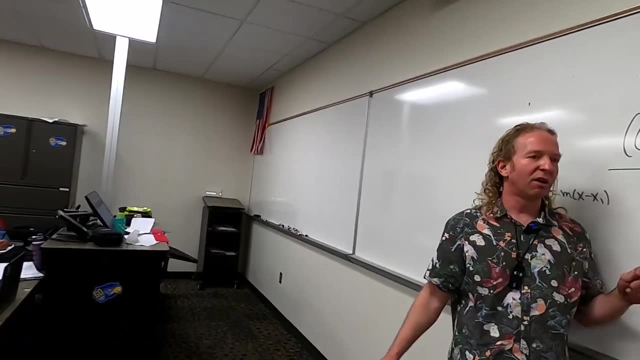 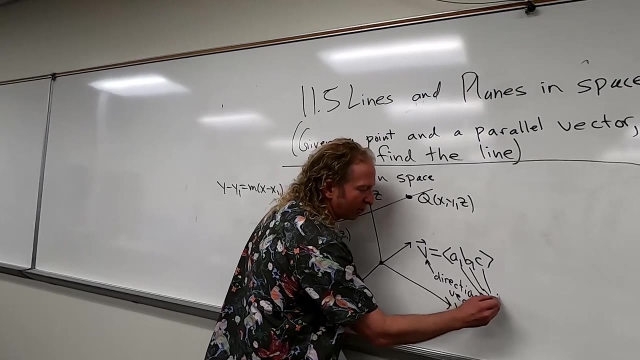 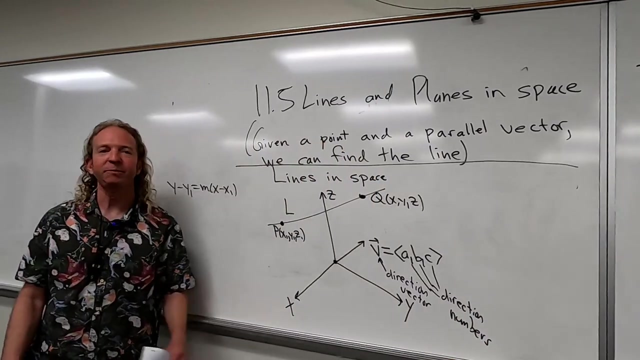 Direction vector- Direction vector- Extra knowledge Direction vector And the A and the B and the C are called the direction numbers- Extra extra knowledge. So these little guys here are called the direction numbers. Let me pause here. So so far we have this line L. 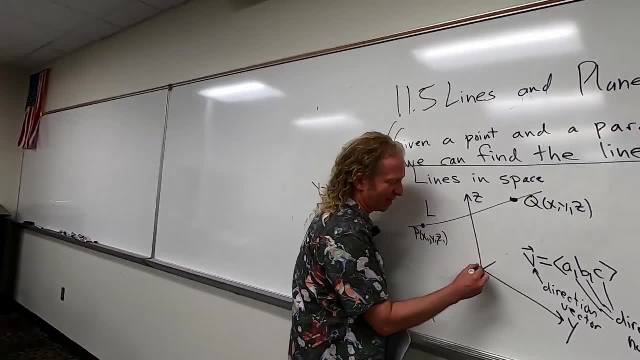 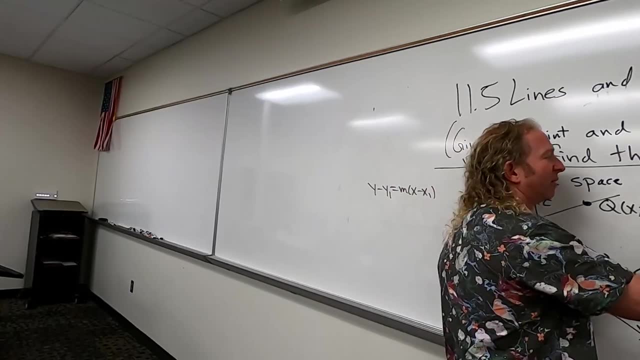 Right And this. that's a really bad picture. It's not bad, I guess it's okay. That's supposed to be parallel. So V is parallel to L Right V is parallel to L. So V is parallel. 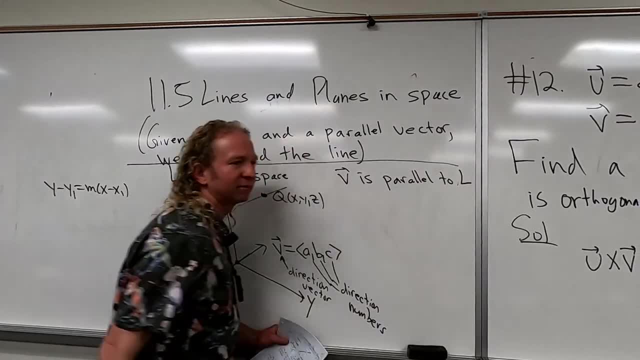 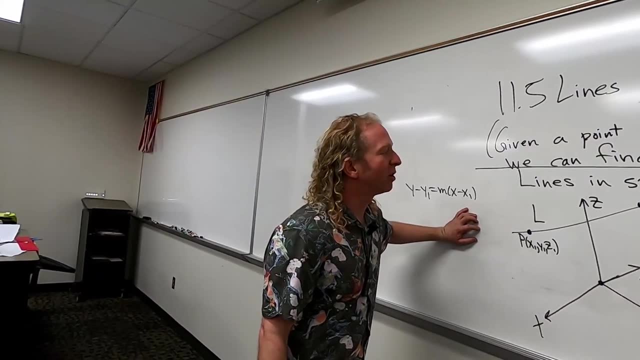 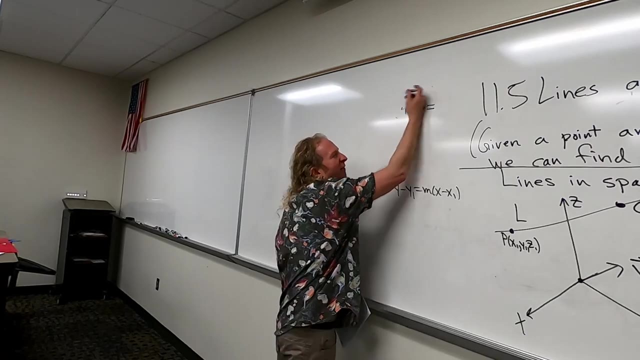 To L. V is parallel to L, V is parallel to L, So two vectors are parallel when they're multiples of each other. So like if I have like, if I have like one two, Oh sorry. 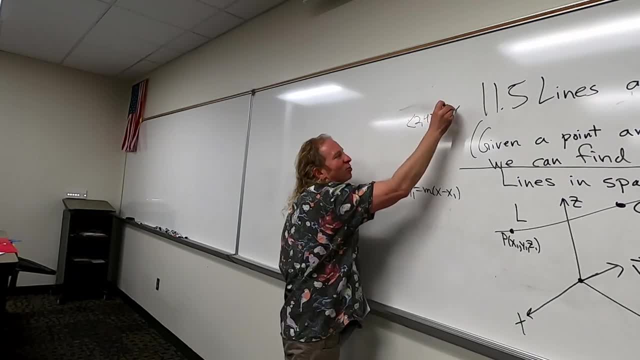 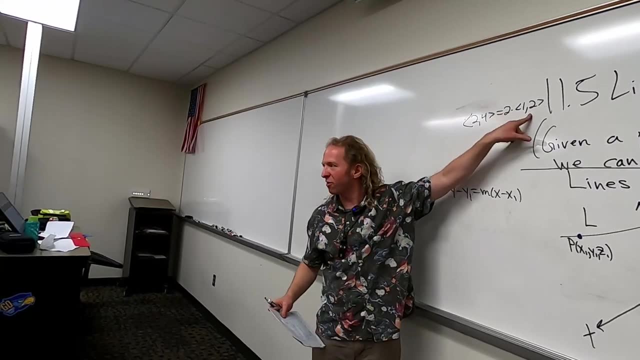 If I have like two, four, That's equal to two times one, two. These vectors are parallel. So whenever that happens, we have a vector equal to a number times another vector, The vectors are parallel. So if you have a vector equal to a number times another vector, they're parallel. 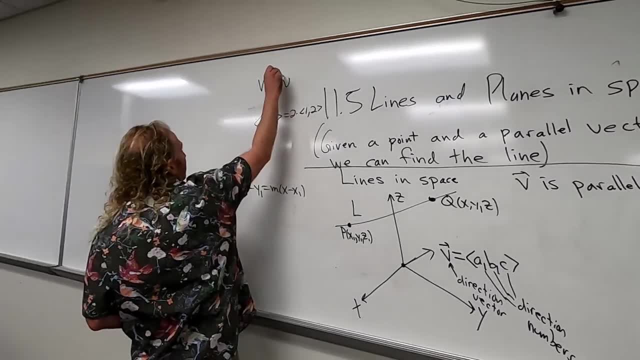 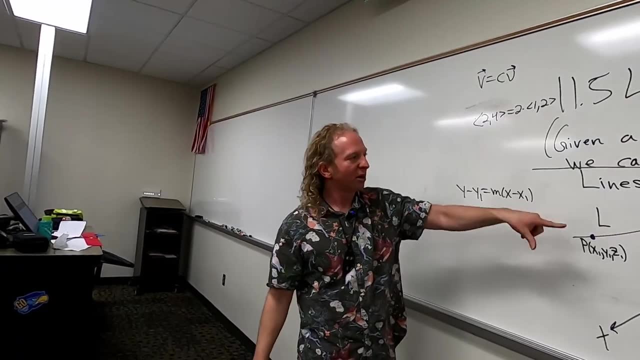 So, if I have like, So if I have V equal to C times U, V and U are parallel. That's the definition of parallel. So two vectors are parallel if they're multiples of each other. Okay, So we're going to use that here. 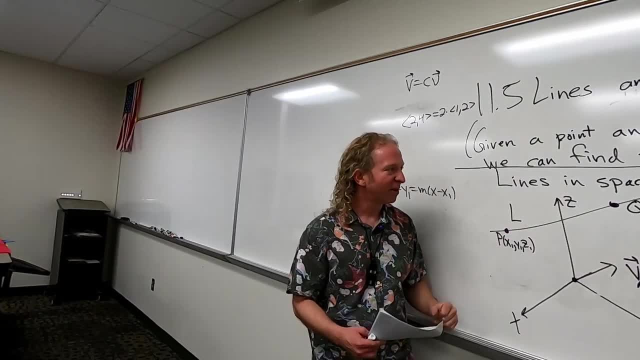 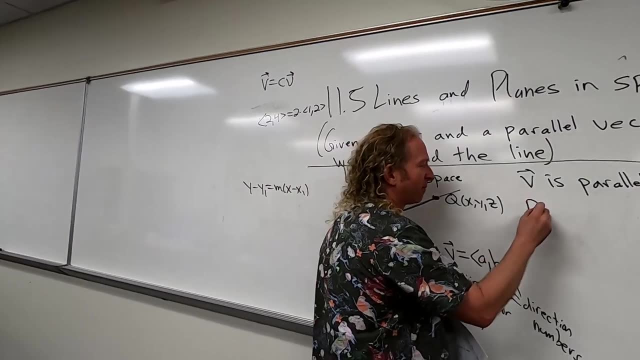 Okay, So we have a vector V. It's parallel to L, So that means that this vector here, PQ, we can form the vector PQ, PQ. PQ is equal to a number times V. I'm going to use T. 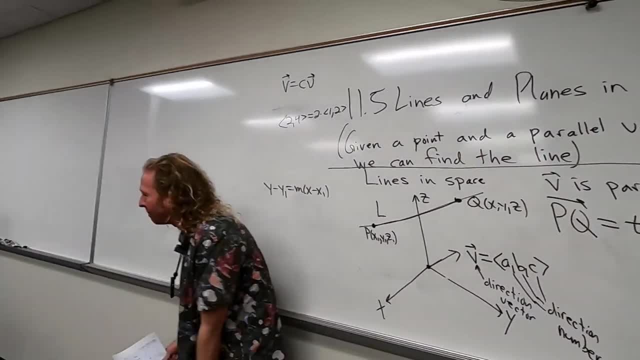 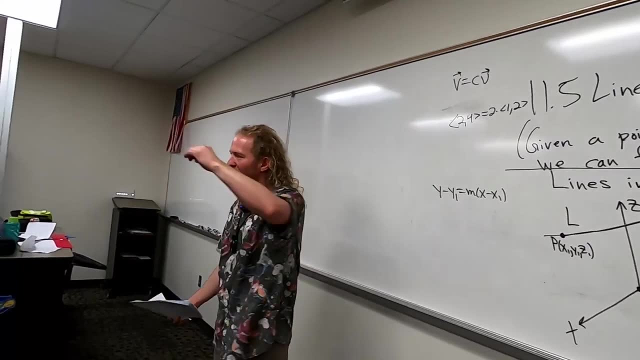 I'm using T because T usually represents time, right? A lot of this stuff is used in the real world, right, Like you have something traveling through space as time goes on, right? So T is a popular choice for our parameter. 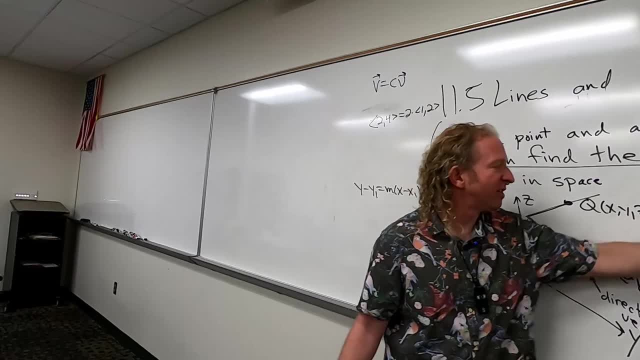 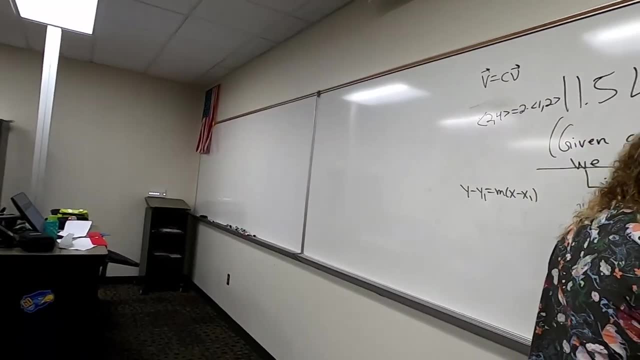 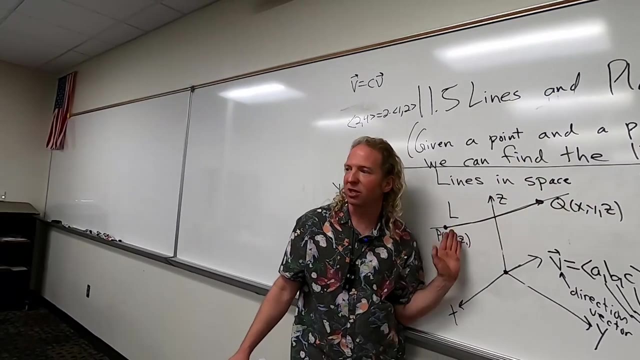 So, because PQ is parallel to V, these vectors are multiples of each other. Now we're going to use something we used the first day of class. I don't know if you remember this, but when you're trying to find the vector PQ, is it initial minus terminal, or is it terminal minus initial? 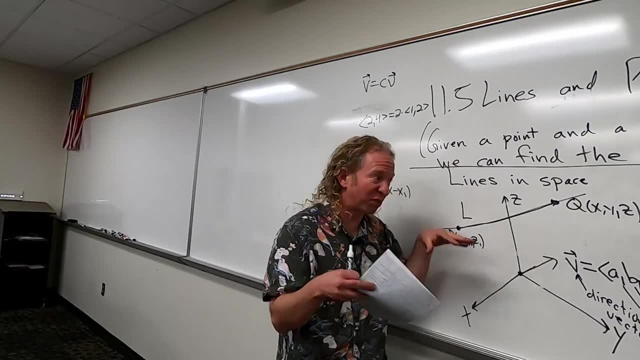 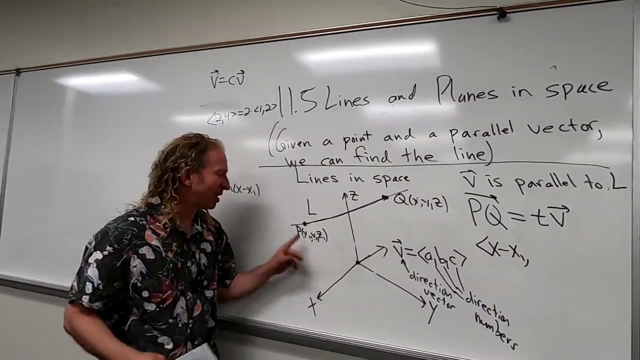 Terminal minus initial. Yeah, So we're using it in the actual derivation. It's beautiful, So it'll be X minus X1.. It's really amazing: Y minus Y1.. And it's really cool when it makes sense. 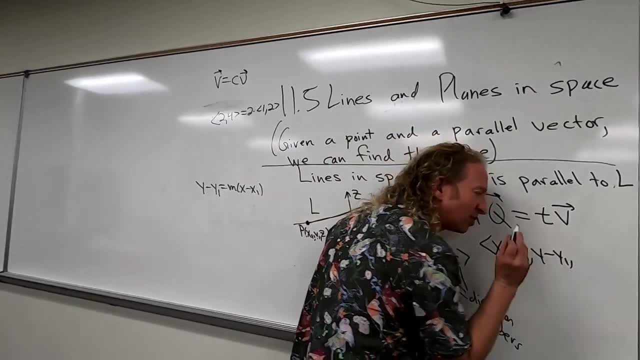 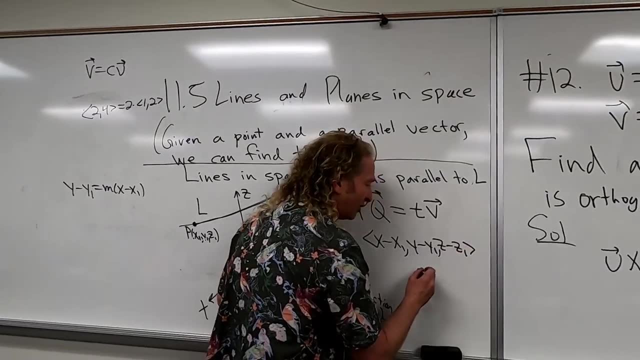 If it doesn't, it's okay, I'll go over it again, But like when it makes sense, it's so great. And then Z minus. I think most people don't understand derivations. That's fine. I mean, I never did when I took these classes, right. 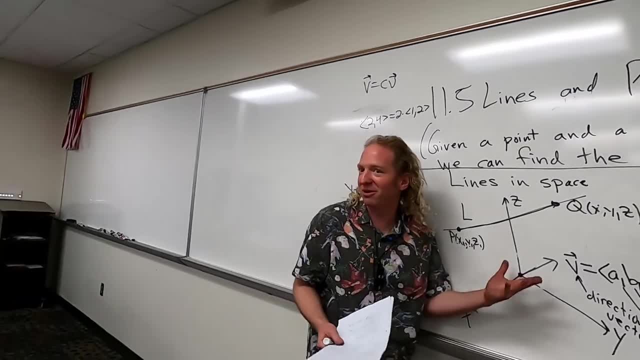 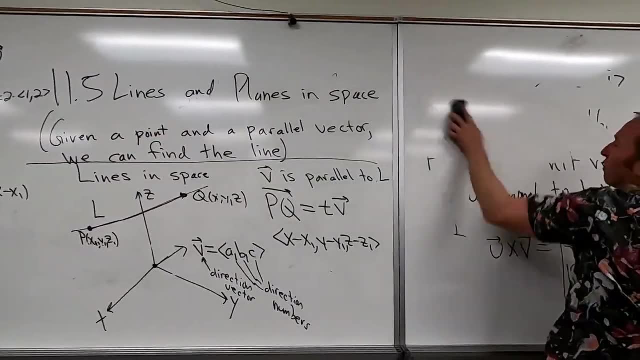 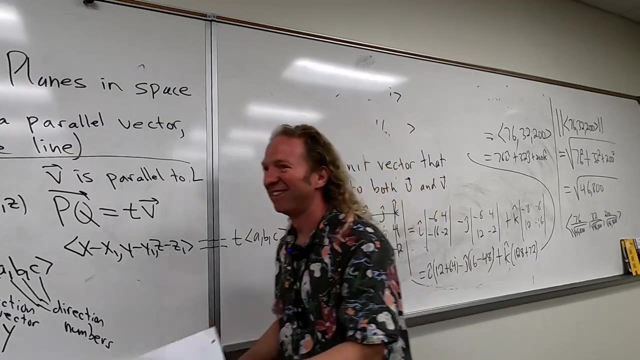 I just memorized everything and got an A. That's okay, right, But you know it's better to learn. And then T. I'm running out. I've got to come to the other board. Let's just break the rules and go over this. 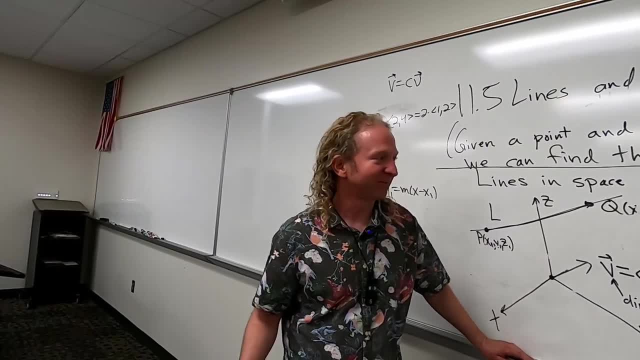 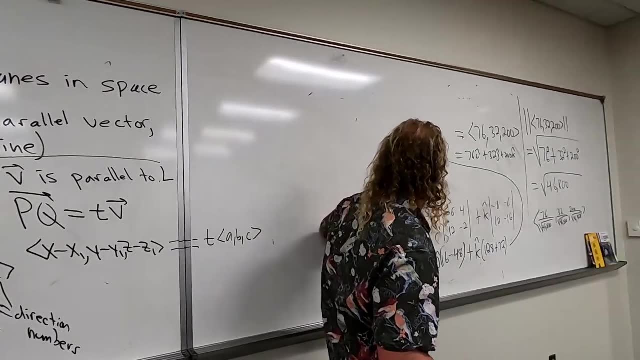 So we're there. So just replacing a V with V, Almost done, Almost done. We've almost completely derived the equation of the lines in space, And then we'll do some problems. So now you can just distribute the T. 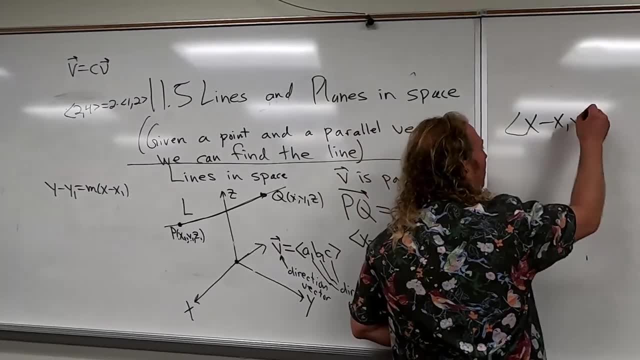 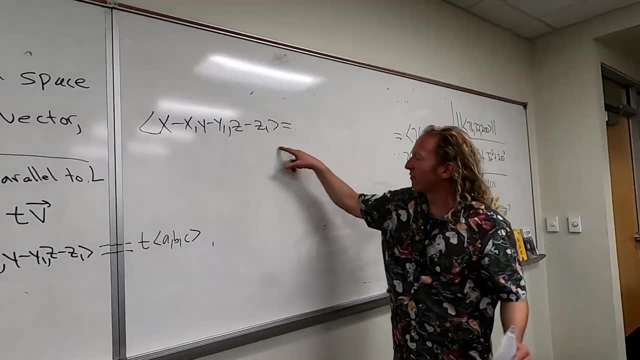 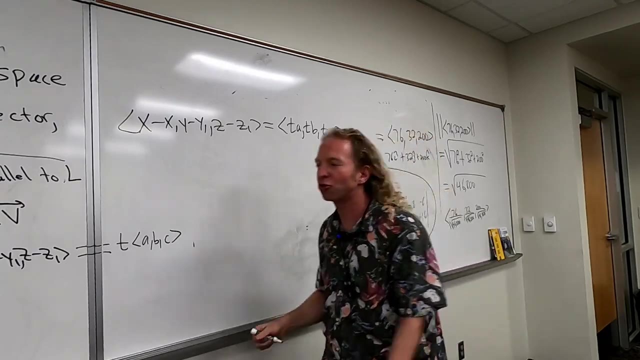 I'm going to come up here. So we have X minus X1.. Y minus Y1.. Z minus Z1 equals. And then we have TA TB TC. So we have TA TB TC. Right, Just distributing the T. 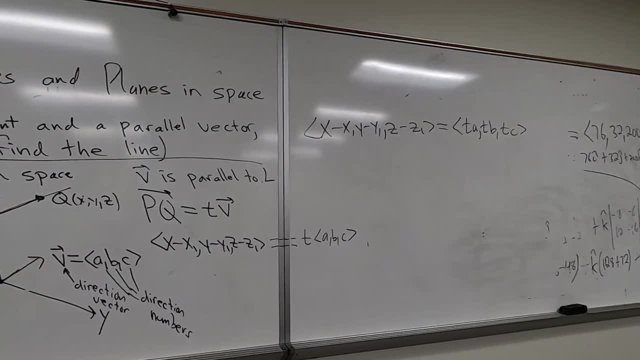 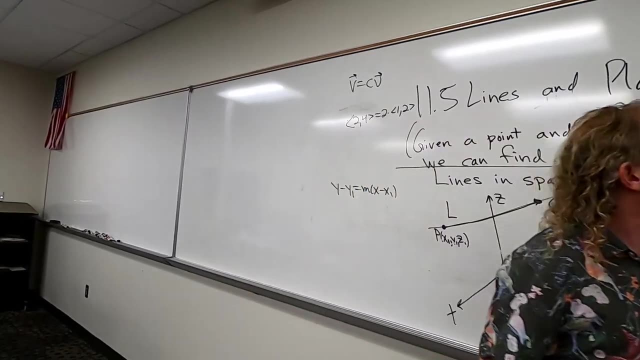 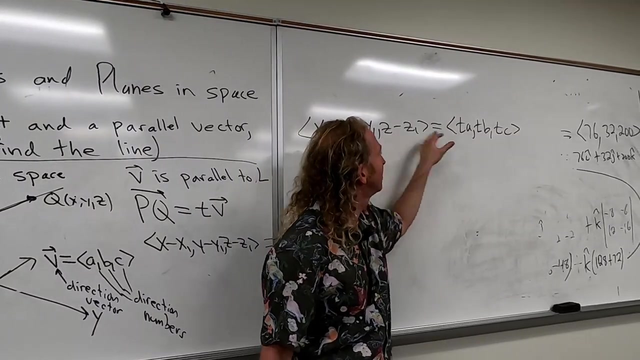 Yeah, beautiful. And then you have two vectors and they're equal. That means their components must be the same, right? So you basically set this equal to this, You set this equal to this And you set this equal to this. 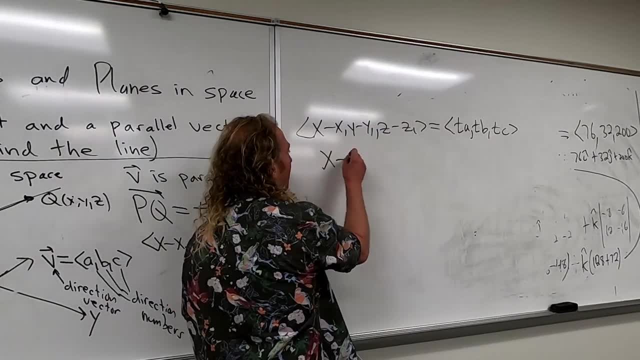 So you just set each of them equal to each other, So you get X minus X1.. It's really cool, Like if you could actually like explain this to someone you know. I mean that's pretty cool. 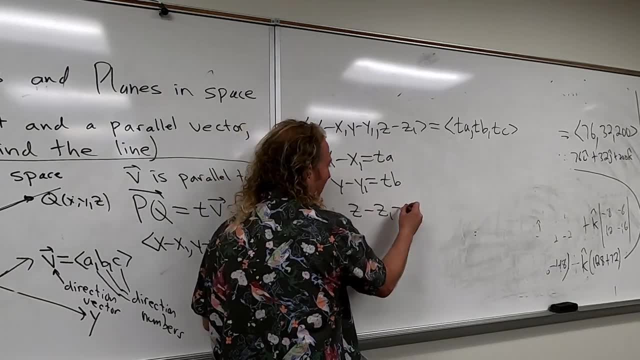 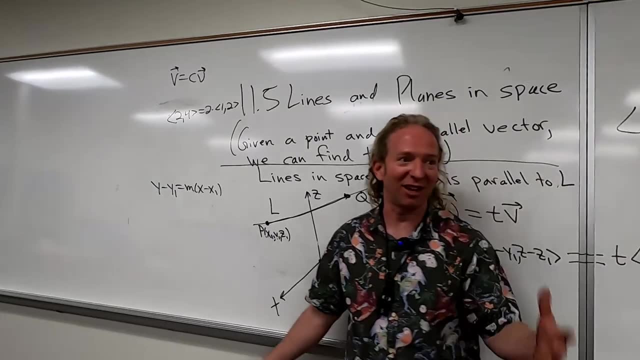 That means like this is the answer. Like I mean especially like as a student, like for like an actual student to like. just if you can explain this derivation to someone, that's like a big deal, I think, in my mind. 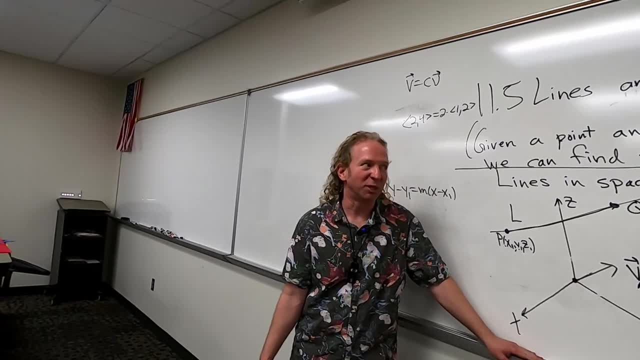 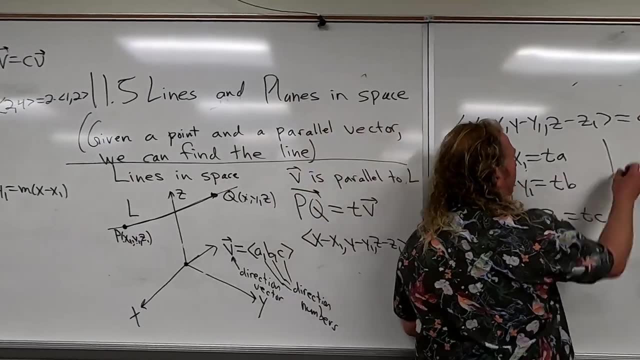 Most people can't right. I mean, it's pretty tough. You can solve for x, y and z. now right by adding this, adding this and adding this right, So you get x equals x1 plus ta. 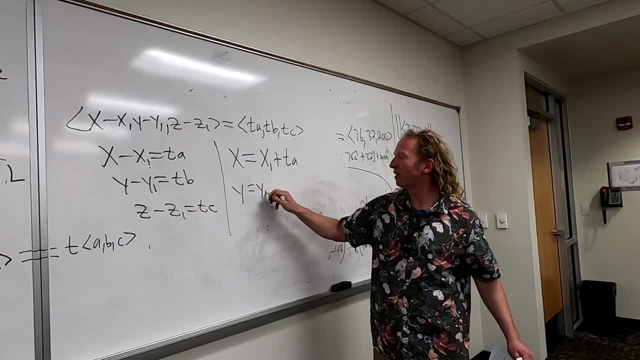 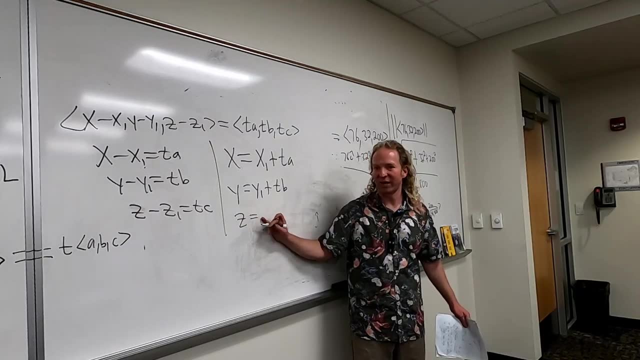 Okay, y equals y1 plus tb. That sounds bad, doesn't it? Isn't that a yeah Yeah, but people have shots for that right. So z1 plus tc. I think that used to kill people. It might still do it right. 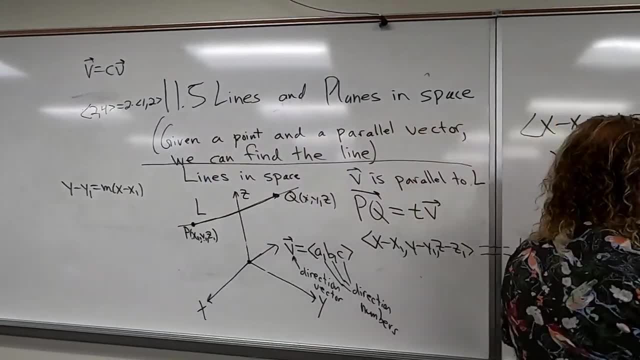 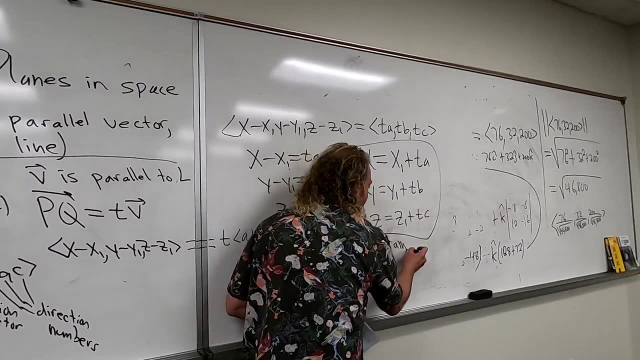 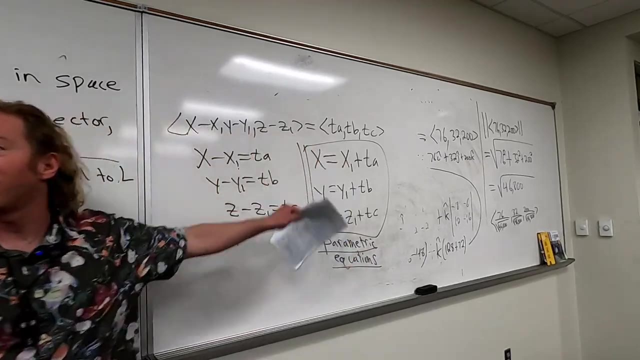 So I mean it's pretty bad. These, these have a name. These are called the parametric equations. right, These are parametric equations, So you want to memorize that for the test. right, That's the formula. 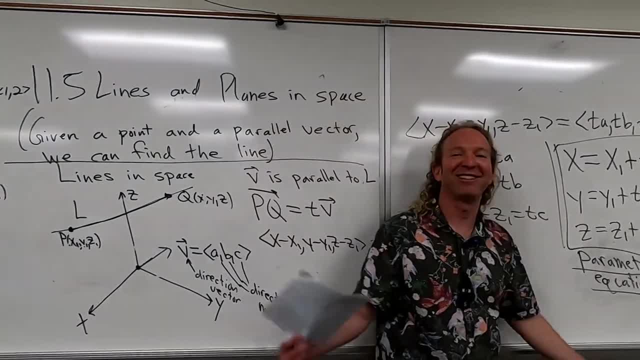 I could have just given you this Like: all right, let's do a homework problem. But like I don't know, We won't always do derivations, but sometimes Yes. come on, What's the t? T is just a. it's called the parameter. 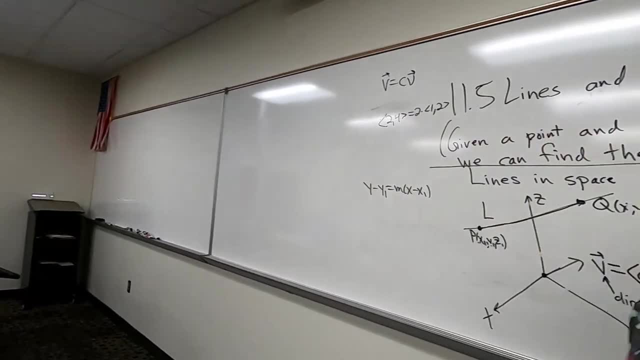 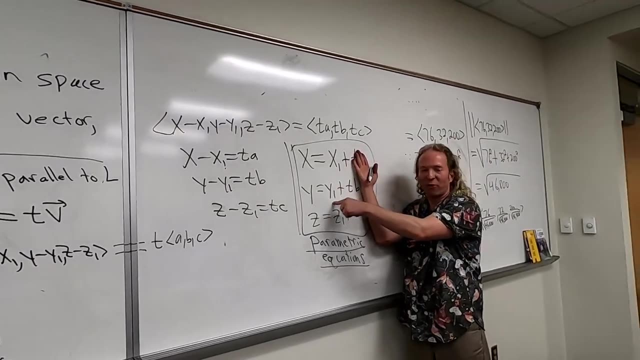 So t will vary. So, oh, check this out. So think about this. So if you plug in, t equals zero, you're just going to get x1, y1, z1, right, So you're here. Ah, you see. 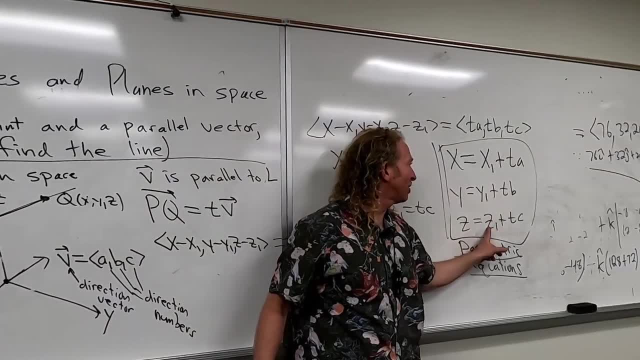 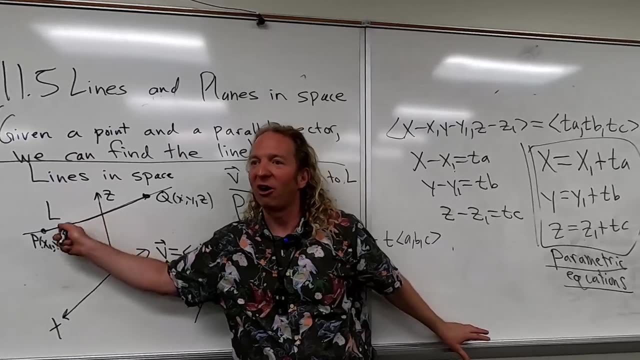 Plug in, t equals one, and then you have x1, y1, z1 plus abc. So like you're getting another point on the line, So as t varies you end up getting all the points on the line Right. so t could be time or something. 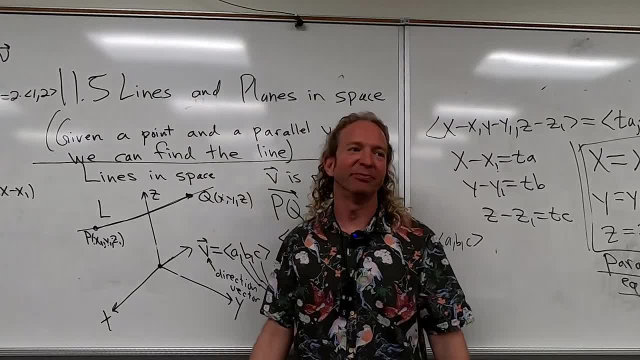 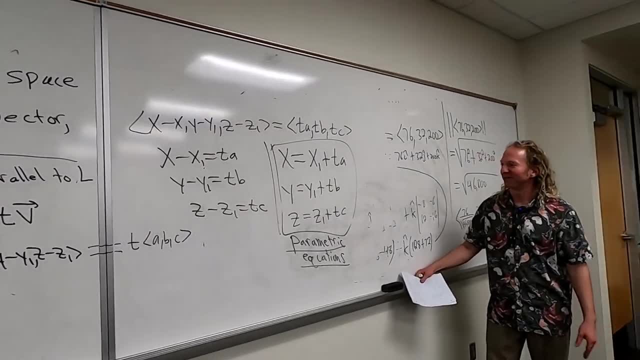 So, as time passes, you're moving along the line. It's pretty cool. Cool, Good, Kamal. Good question: Extra credit: No, I'm kidding, You don't need it. No, Ah right, So also check this out. 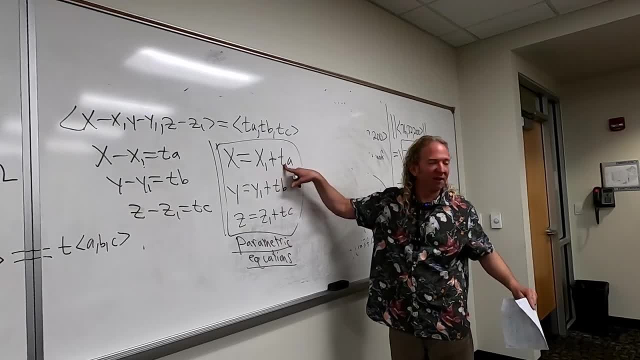 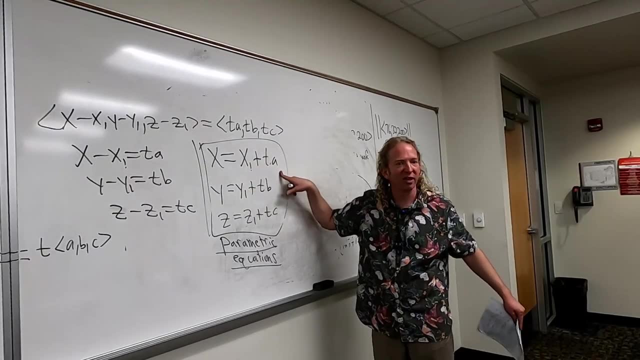 So if you solve each of these for t, if I solve this for t, you get x minus x1 divided by a right, Because I subtract x1, divide by everyone. see that. So if abc are all not zero, so if they're all not zero, 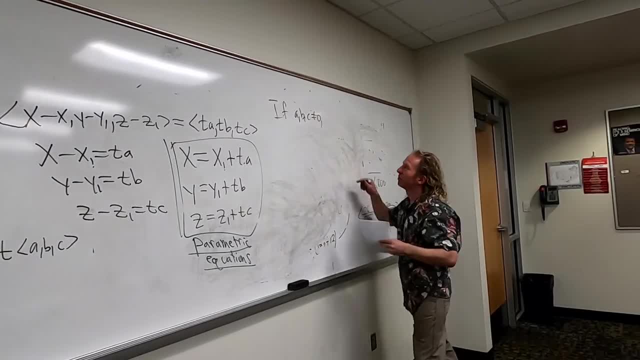 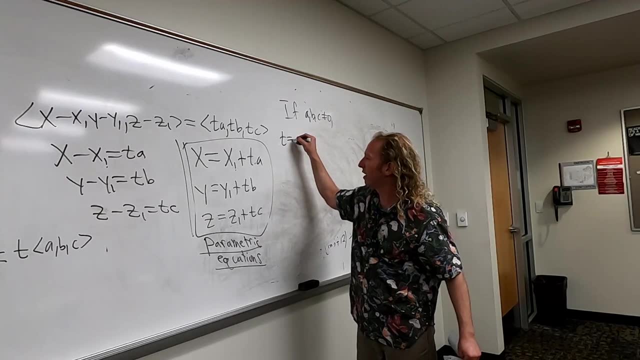 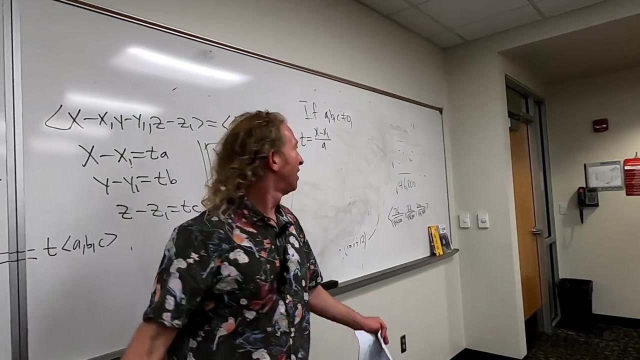 so if ab and c are all not zero, so none of them can be zero. you can solve for t And you get x minus x1 over a right. You can solve this for t and you get y minus y1 over b. 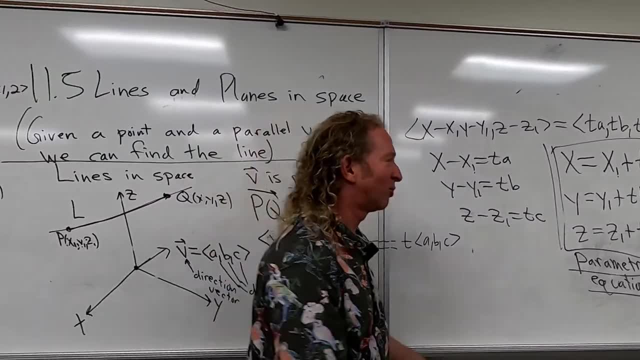 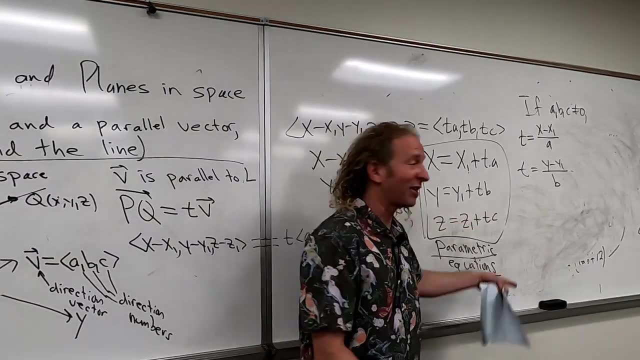 And it might seem redundant, but I'll just do it anyways. Why not? Extra steps are better. If you solve this for t, you get z minus z1 over c. That's why they can't be zero, you see. So all of these are the same. 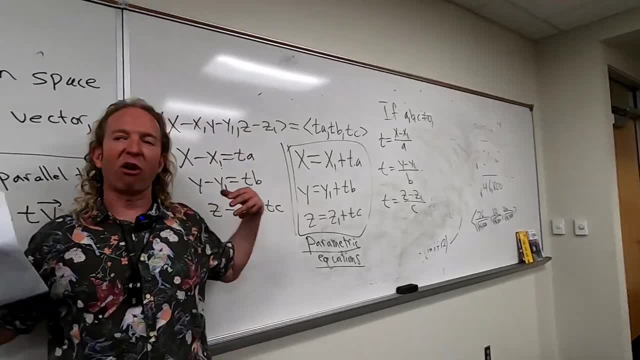 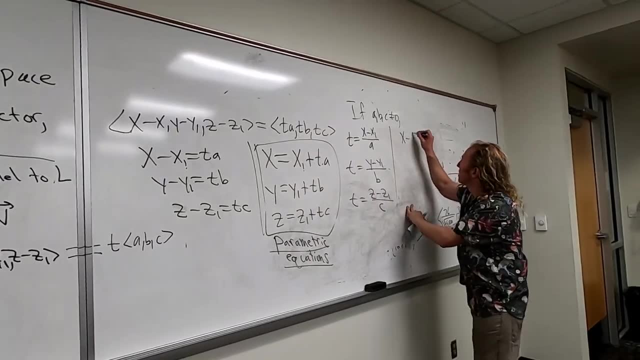 So you get x minus x1 over a. All of these are the same because they're all equal to t. These have a name. These are called the symmetric equations. So note that you have x minus x1 over a equals y minus y1. 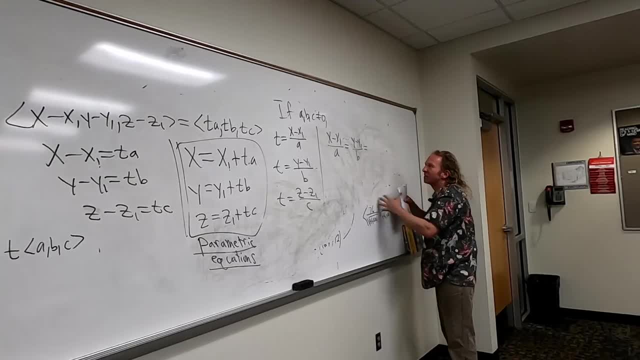 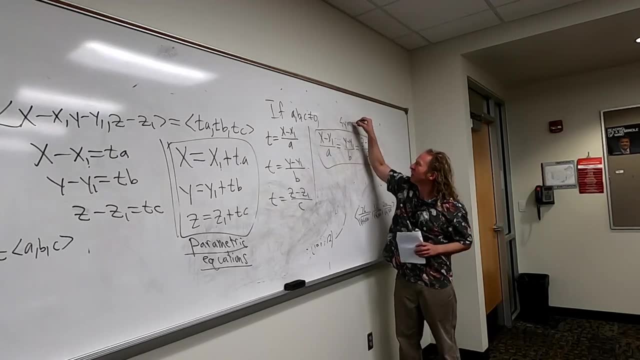 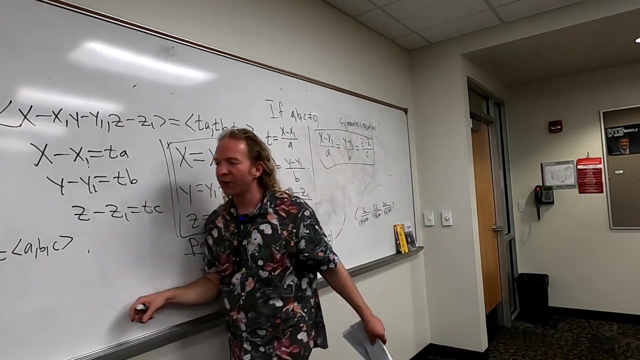 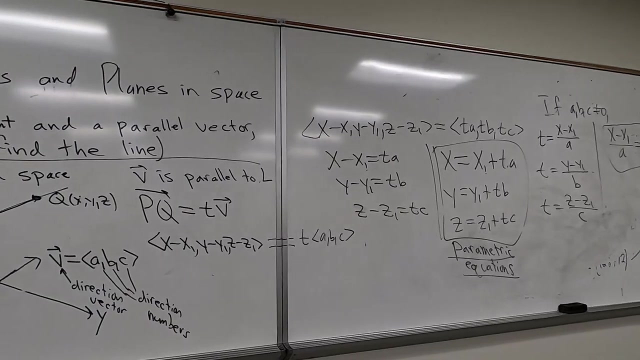 over b equals z minus z1 over c. These are called the symmetric equations, Symmetric equations. So the homework will have you find these, but they're multiple choice and the homework also. the homework will do weird things like multiply by numbers. So like sometimes you'll work it out. 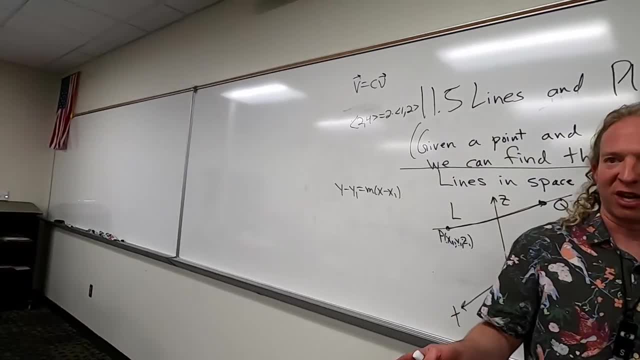 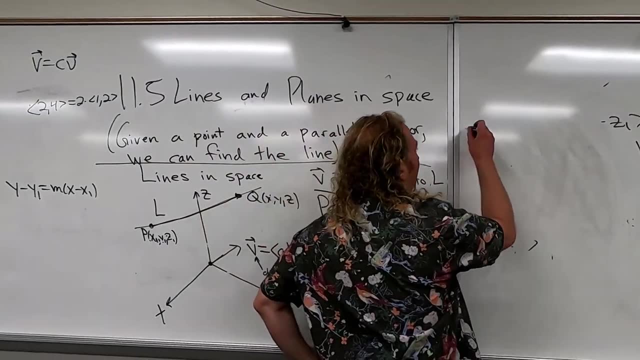 and your answer won't be there in the homework. That's because the homework does stuff. So like, for example: let's just say that let's say that you're doing the homework and you get x minus 4 over 1 half equals y minus 2. 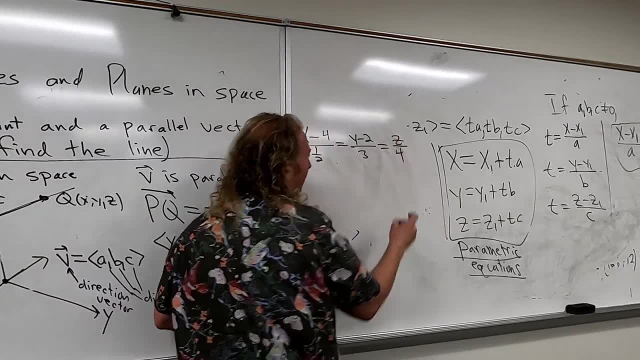 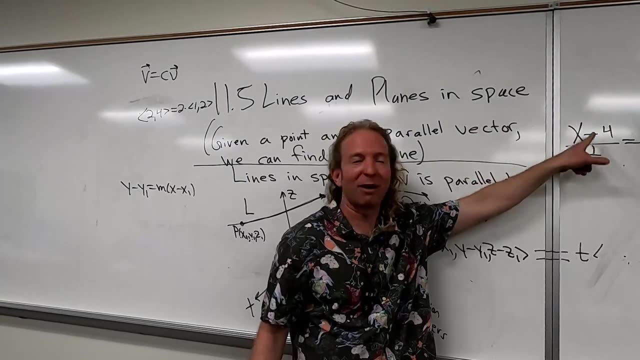 over 3 equals z over 4, right. So you get that The homework might multiply everything, might rewrite this too. it might distribute it. It might write it as 2x minus 8, right. Or it might multiply everything by 1 half right. 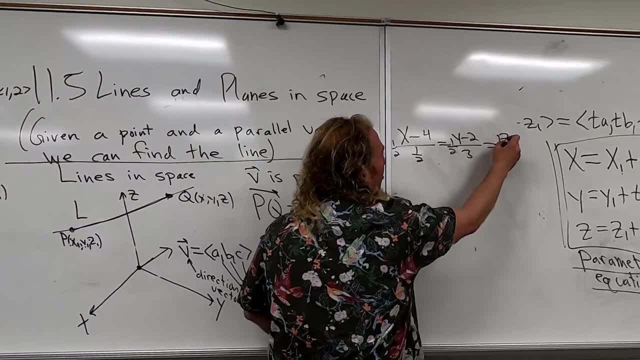 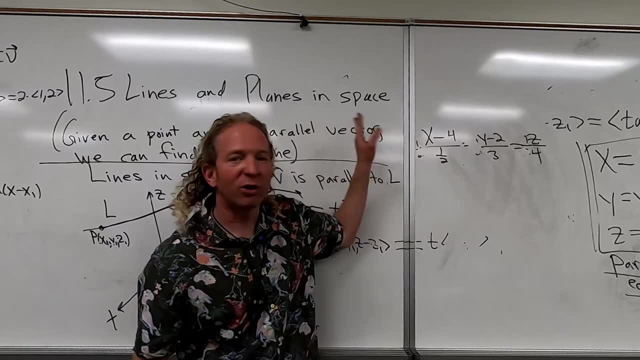 It might multiply by 1 half, multiply by 1 half, multiply by 1 half so that you would- well, that's so that you would, the 2's would cancel, or something right? So it does stuff, it rewrites things, okay. 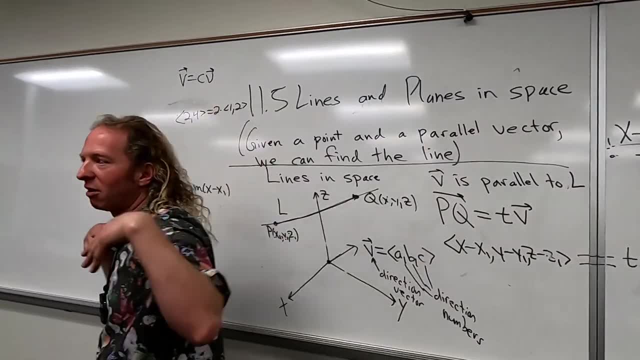 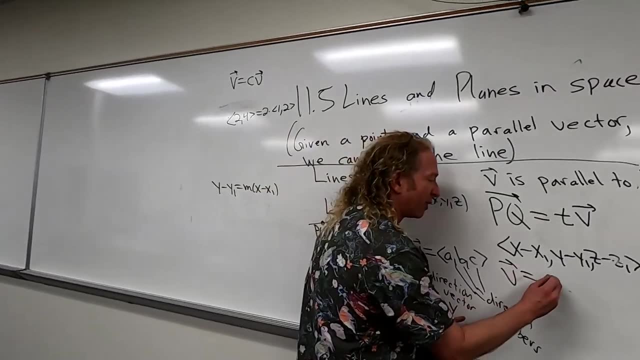 It rewrites things, So the homework makes manipulations that aren't normal. Okay, So the reason is okay. the reason is when you get your direction vector, like let's say you get this, and let's say you get 1, third, 6,, 2.. 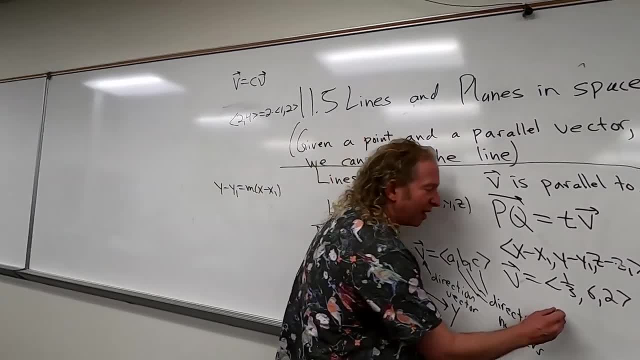 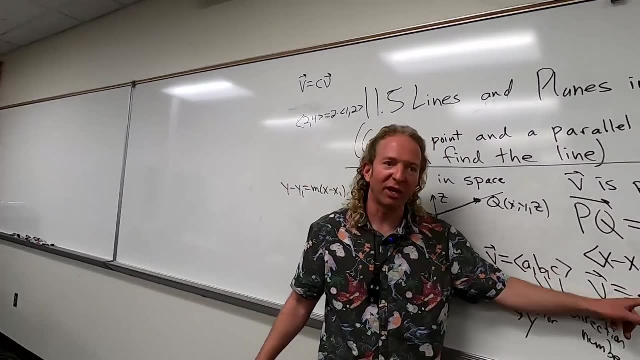 You say: I don't like that fraction, You can multiply it by 3 and get 1,, 18,, 6.. Same answer: right, Because this is still parallel, right? So the homework will do stuff like that in its work. 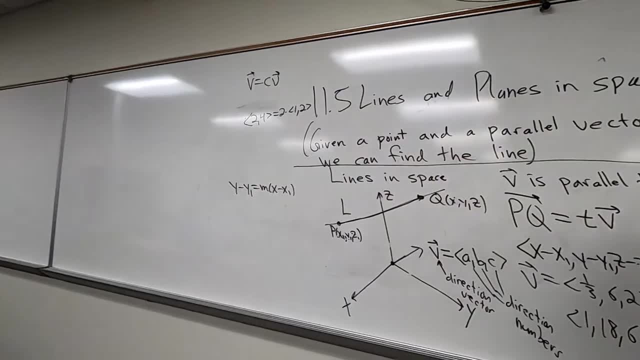 and so the answer is reflected that way. On a test I don't care right, As long as it's correct. on marker, right? People do this on tests too. Last semester a couple people got really clever- One guy- 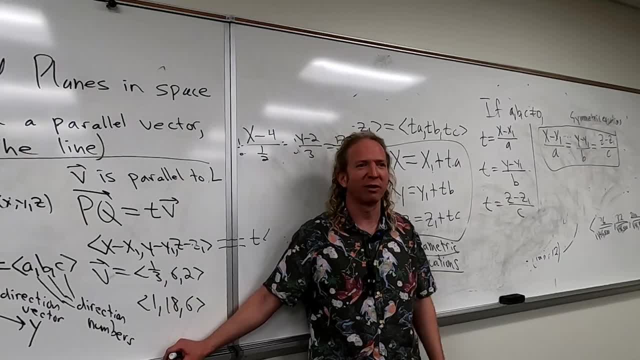 I don't know who he was, but like he did it on every problem, Like he was always multiplying his vectors by numbers, I'm like why? But he got an A. so Yeah, Yeah, But you could do that right. 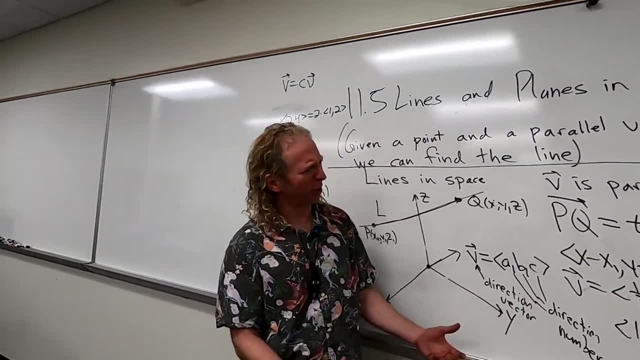 You can multiply by. yeah, he was multiplying by negative numbers. I'm like, oh, is he just doing that on purpose? Like what the heck? And I was like this guy. I was like, I looked at his test for a long time. 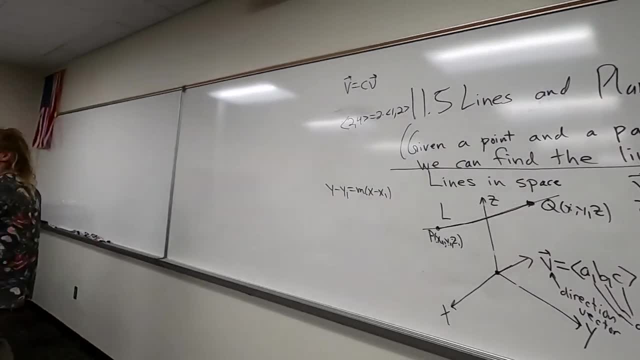 Like he really knew what he was doing. Like I was like, oh it's really weird, I don't know why, but yeah, weird. All right, So we'll do some problems. Any questions on the derivation? Any questions on the derivation? 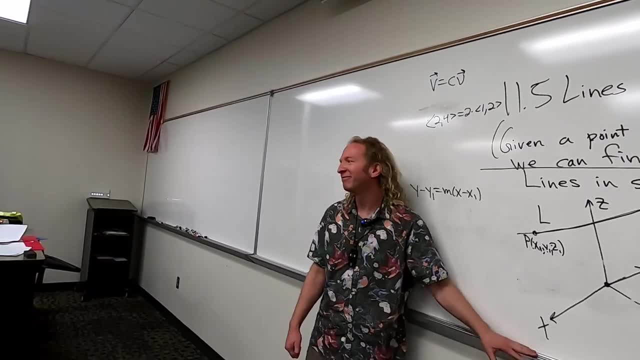 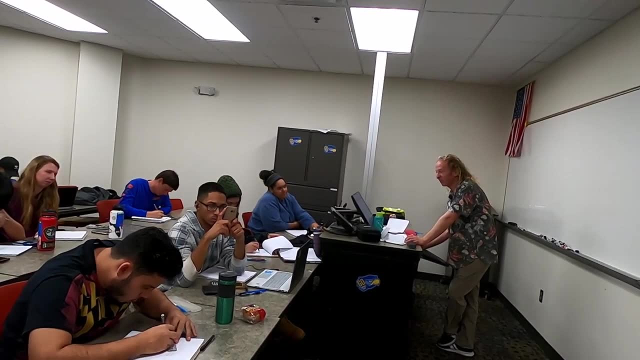 Does it make sense a little bit, The Really, Let's do it. Let's do some problems. How about number wrong section? This is 11.5.. Sorry, Oh, there is no 11.6.. I took it out. 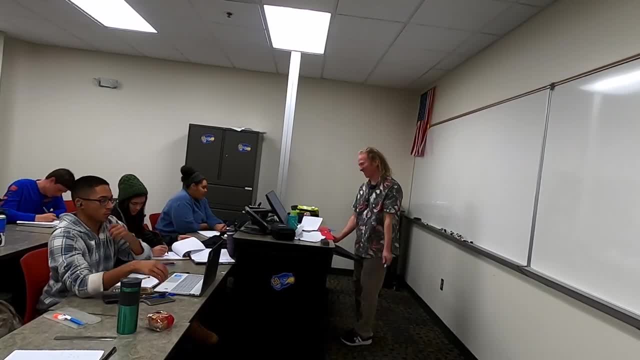 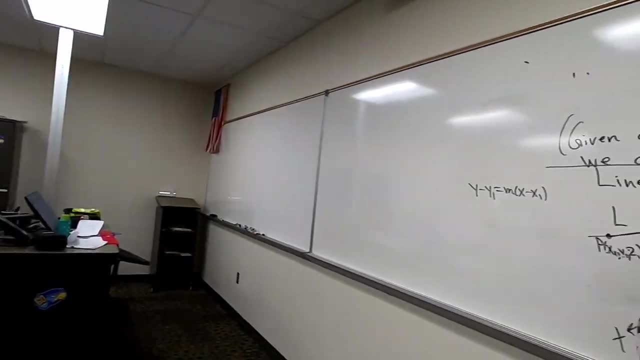 Ah Yeah, me too, I didn't even notice. Yeah, All right, Let's do number one, Why not? It's a nice fun problem. Right, let's do it. Let's do it Number one. it's easy. but there's. 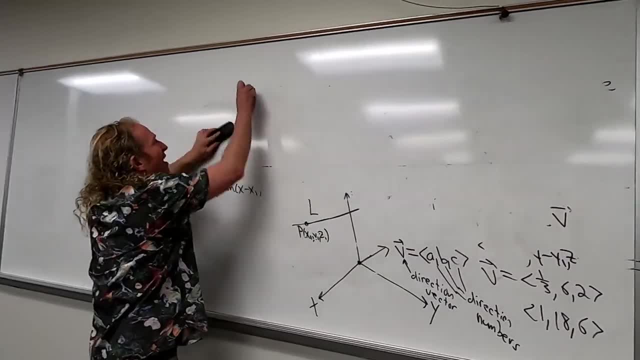 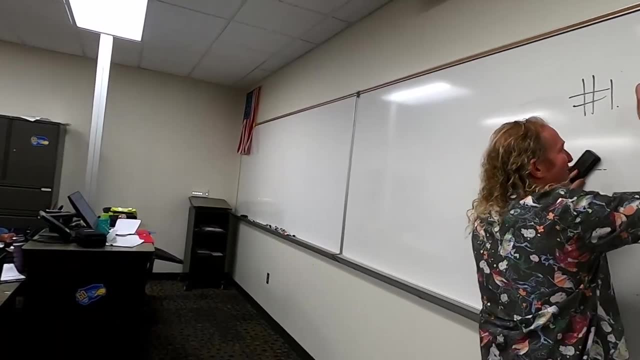 nothing wrong with easy right. Easy is really good in math, because math is already really good. It's really hard. so whenever we have an opportunity to do easy problems, we should embrace it right. So 0.000, there's plenty of hard stuff. 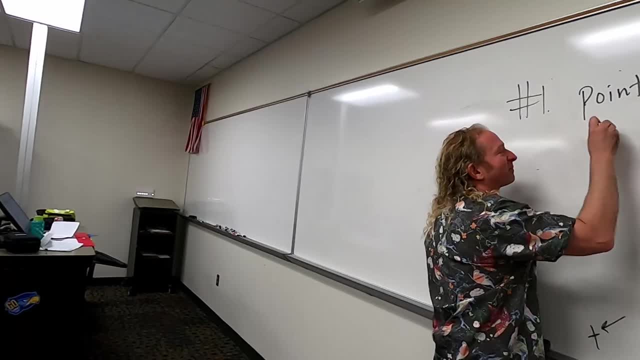 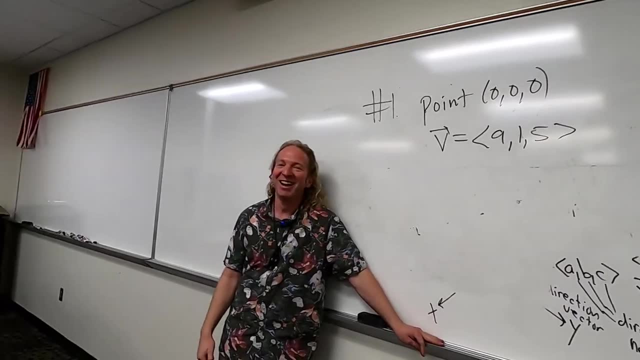 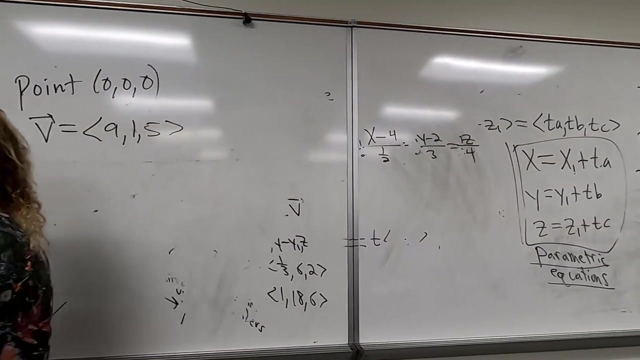 915.. 915, thanks, That's like a phone number, Like 915, that's the area code. And what do we have to do to find the Set of parametric equations and symmetric equations? OK, Symmetric equations. 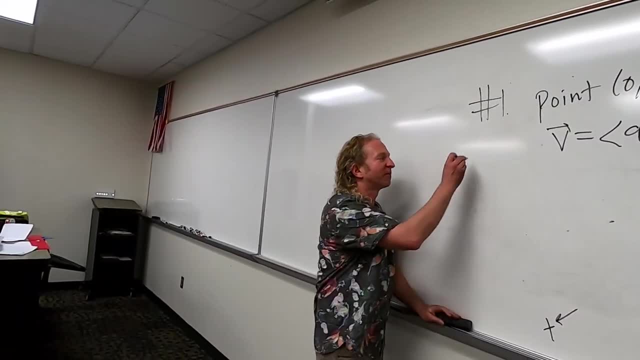 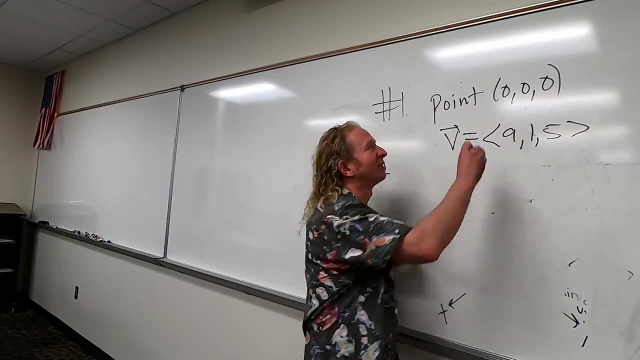 All right, Cool stuff. So parametric and symmetric- Good stuff, Let's do it. It's a solution. So let's identify our variables, I guess. So these are x1, y1, z1.. These here Haven't done this in a while, so I'm going to show all the steps. 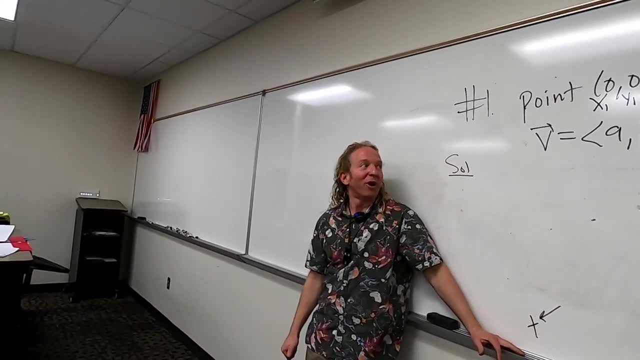 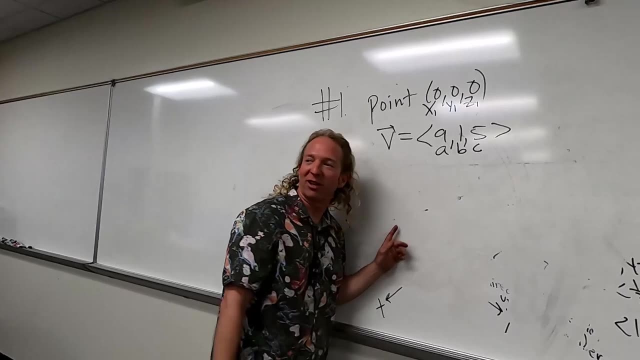 Was there any more points today? No, What letters did we use for these? Do you remember A B C, A B C? Yeah, Do you remember what they were called? They had names, Direction, Direction, numbers. 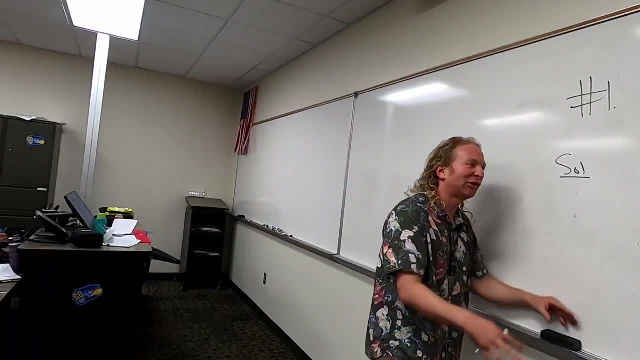 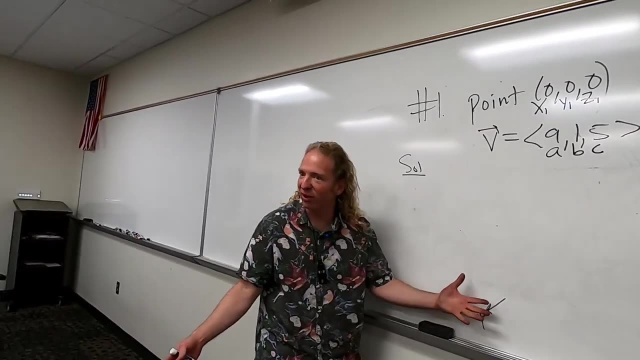 Direction numbers. Yeah, good, Good to know everything Like really like, really like learn it all right, Like the derivation, the names, like really like boom. That's it right Now. we just let's do this first. 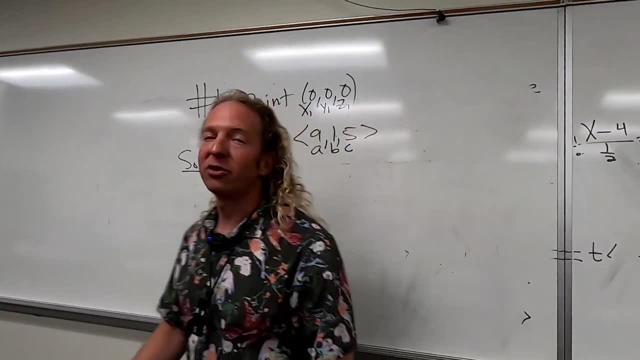 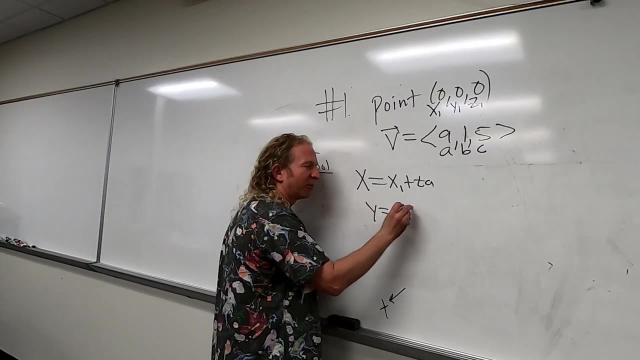 So you just plug in the numbers into these formulas, right? So I'll write the formulas down. So x equals x1 plus ta. I know it's kind of weird to write it down, but like I don't know, When you're first learning a formula it's useful to write it down. 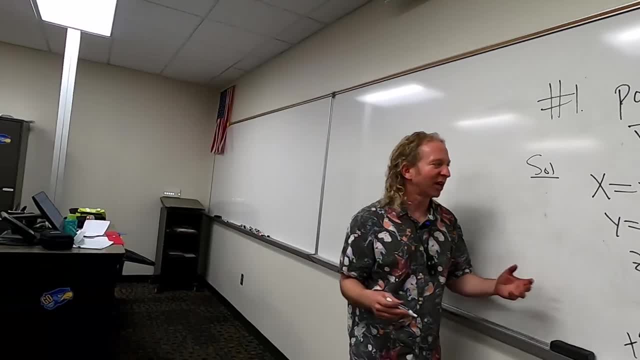 I remember when I first learned like y equals mx plus b. I remember learning that And, like my teacher said to write it down every time, I did a problem And I did and I learned it. So I mean, that's how you learn right. 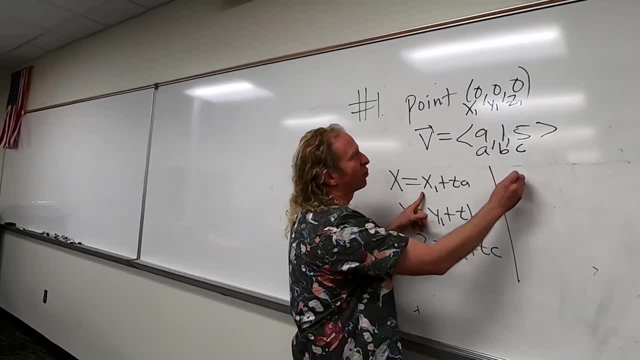 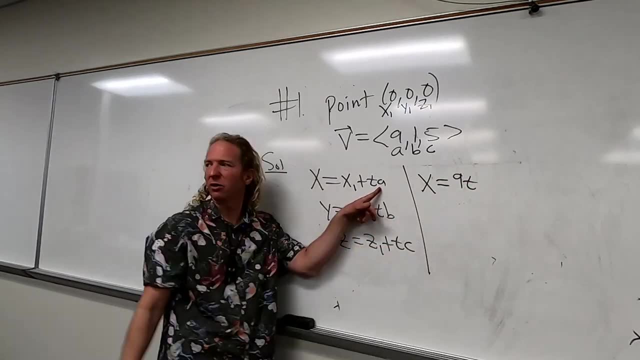 Just writing it down And then just plug everything in. So the first one it'll just be 0 plus ta, So it'll just be 9t, Is that right? Yeah, OK, It's just kind of weird, because the 0 goes there and it's t9, right. 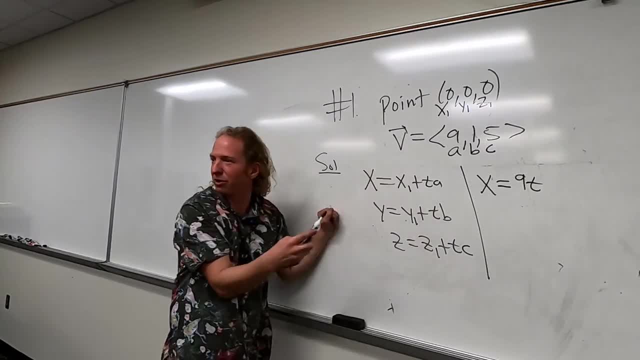 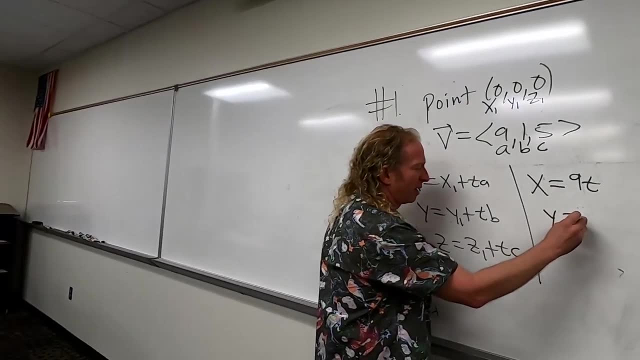 It's t9, because a is 9.. So it's 9t. It looks a little weird. You all OK with that? OK, And that's 0.. So it'll be, I guess, just t right. 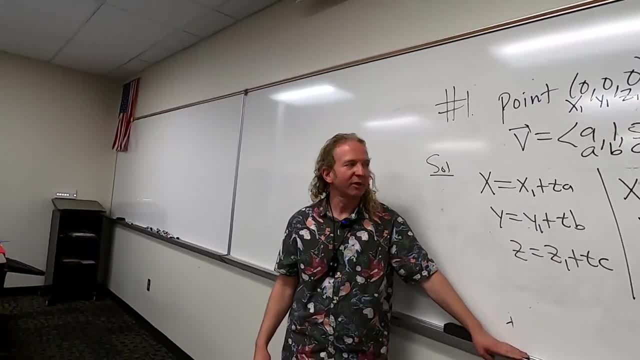 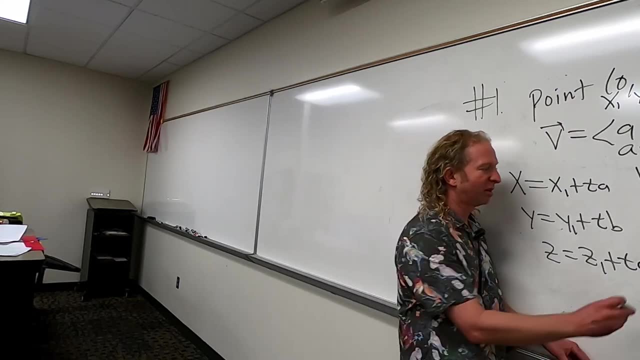 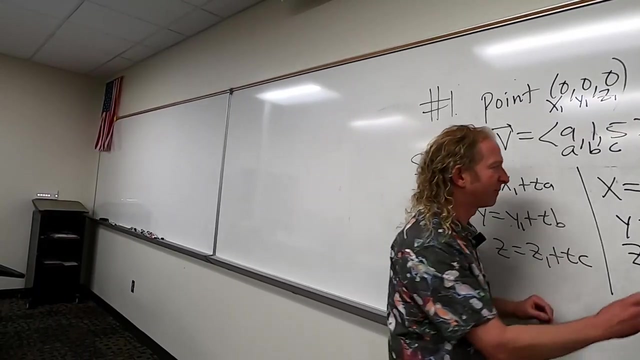 Because it's t times 1.. It's t times 1.. It's t times 1.. And the last one would just be: z equals t5, so just 5t, Yeah, 5t. I wonder if in my notes I wrote down the formula different. 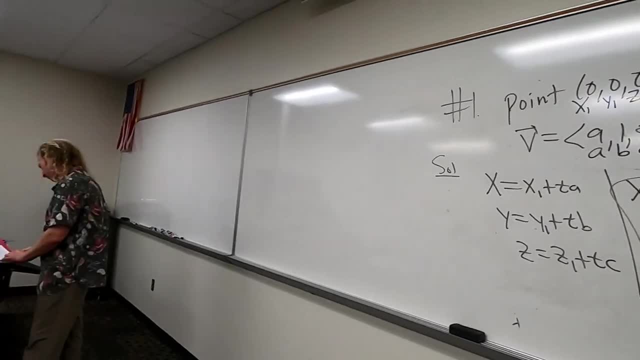 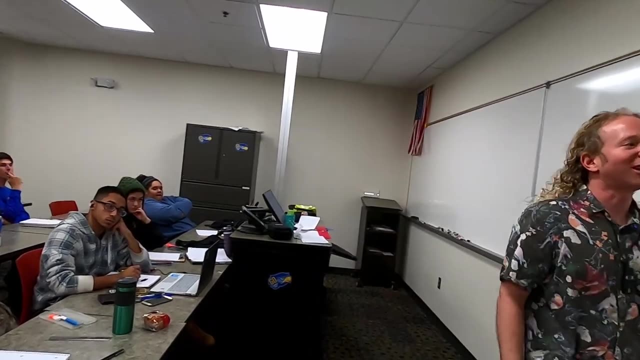 Like I don't even know. Like did I write? No, I did, It's at bt ct is what I wrote, right? Oh, in my notes I wrote it down like this: I wrote it down as at bt ct. 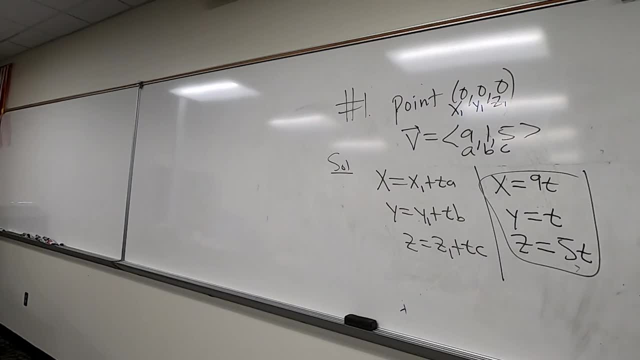 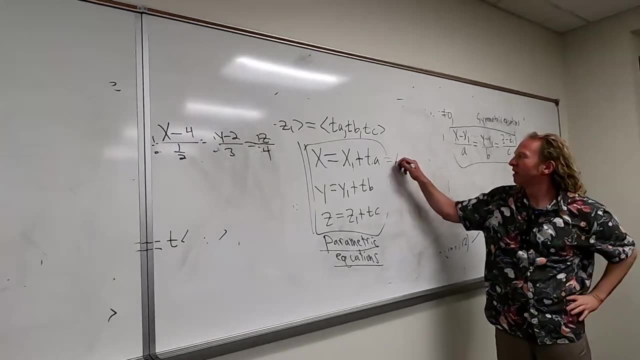 For some reason I wrote it down backwards here because I wasn't looking at my notes, But it's the same thing, right? ta is at right. So if you want to make it easier, maybe you can think of it as x1 plus at y1 plus bt. 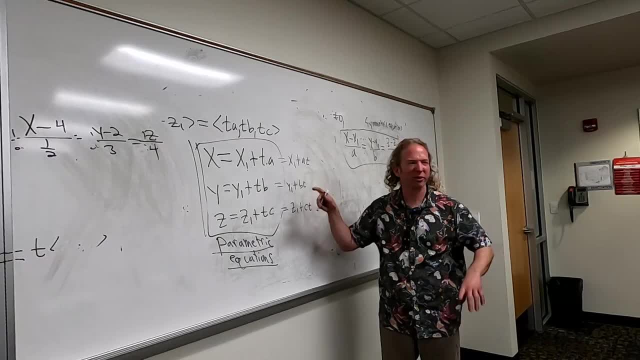 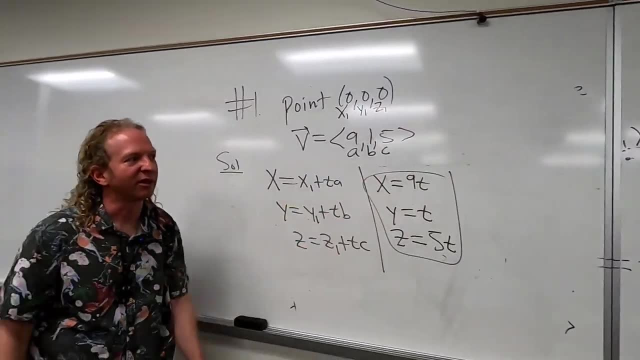 That might be easier. OK, All right, z1 plus ct. I don't know, I thought it was a little bit confusing. Maybe it's just me because it's late. But yeah, same thing, right, Same thing. 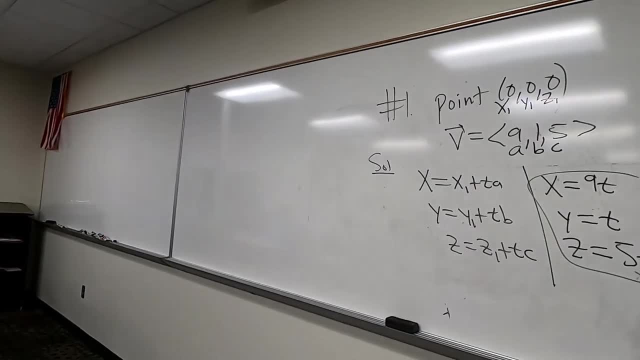 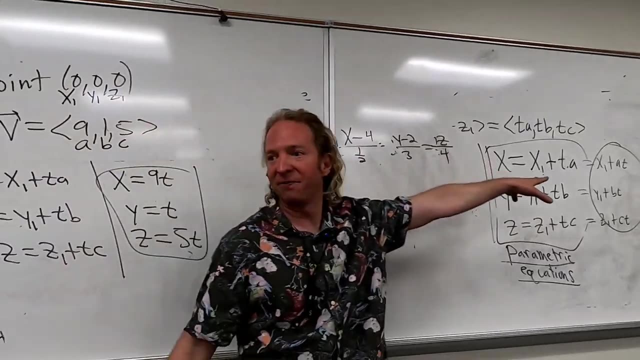 So you can do it that way. maybe That way you have the number in front right. It's just a little bit easier. So I like this better. For the symmetric, we just solve for t. You don't have to memorize the formula. 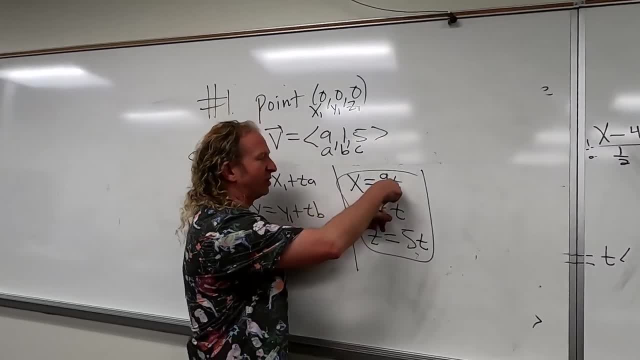 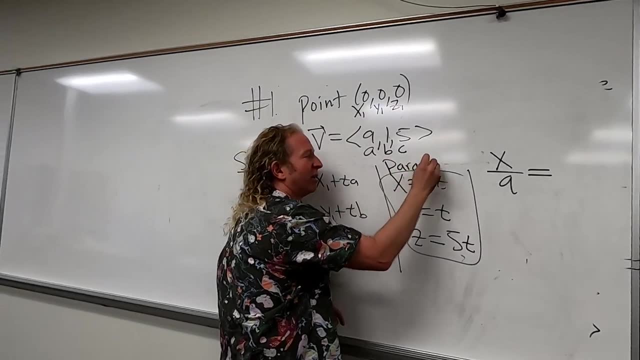 You can just solve for t every time. It just makes it easier, right? So solving for t, you get x over 9.. Boom, Oh, so these are parametric. Sorry, parametric, Forgot to write that, Sorry. 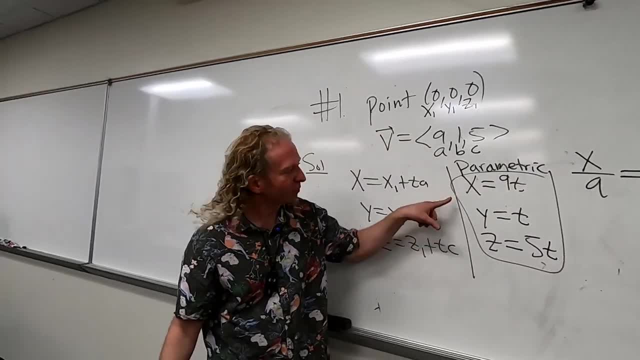 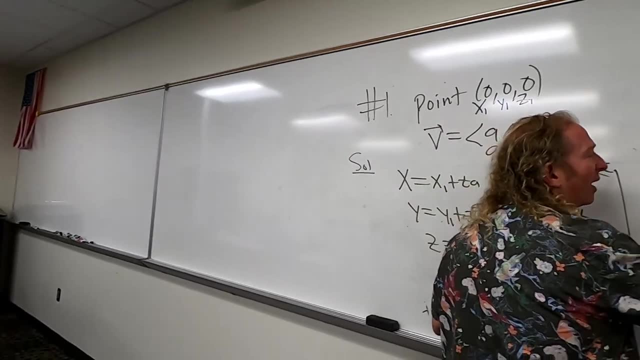 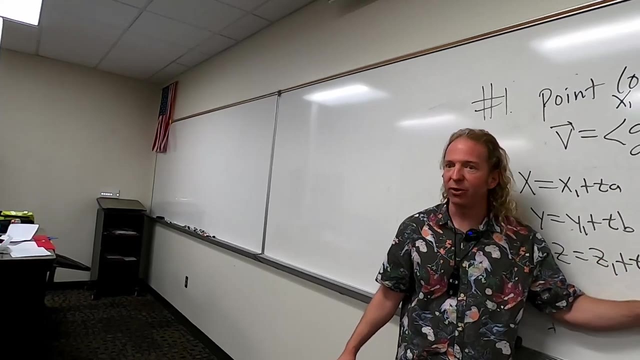 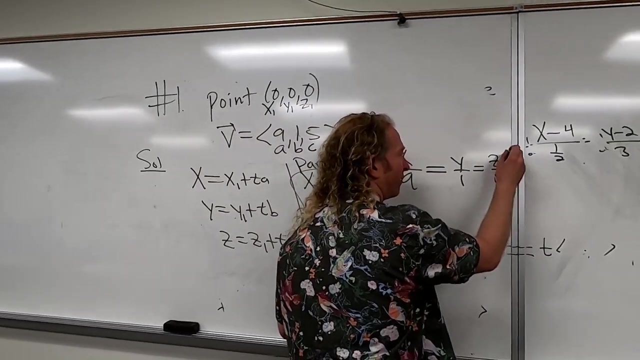 Parametric: So x over 9.. So y over 1.. Right y over 1.. So y over 1.. You can just put y, And the last one would be z over 5.. Right z over 5,, z over 5, z over 5.. 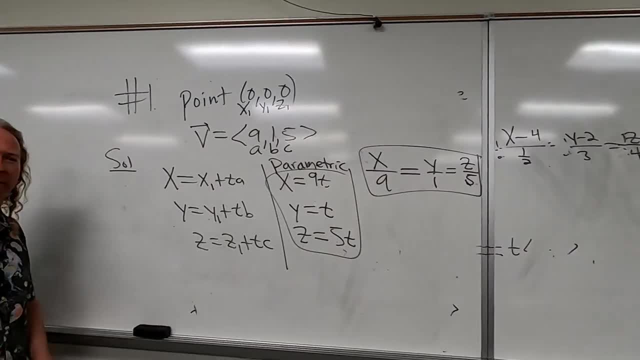 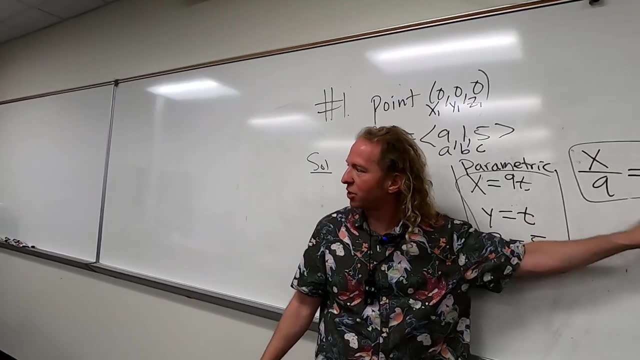 And is that one of the choices? Nikki, for this one? Yes, It is OK, cool, Good, And these are called. what are these called? Do you remember? Symmetric, Symmetric, Good, Symmetric. I'm going to write that down. 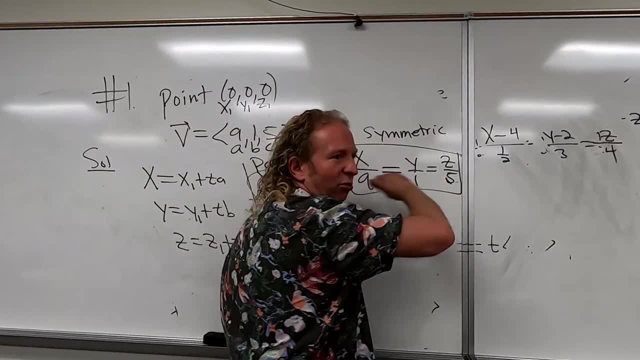 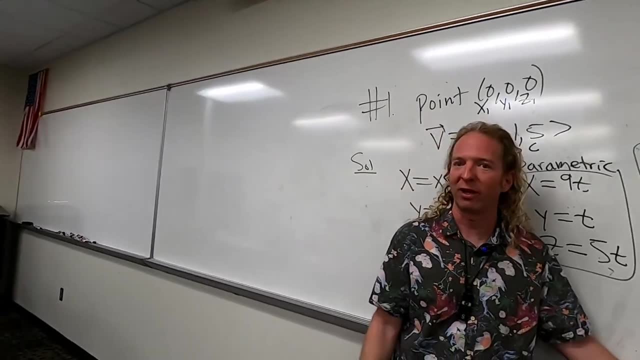 Symmetric, Symmetric. We're going to do many more examples. We'll do all the hard ones, All of them. This was the easy one, So we'll do all the hardest ones. I signed all the ones that were available. that. 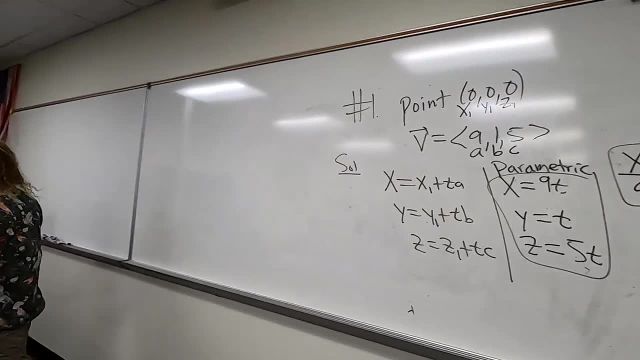 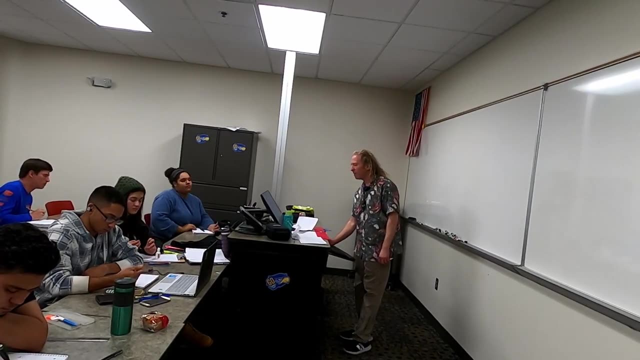 were related to this. So yeah, let's keep going. So number two is really easy. I mean, we could do it, Maybe we should do it. Maybe we should do it. Let's just do it, Why not? It's college. 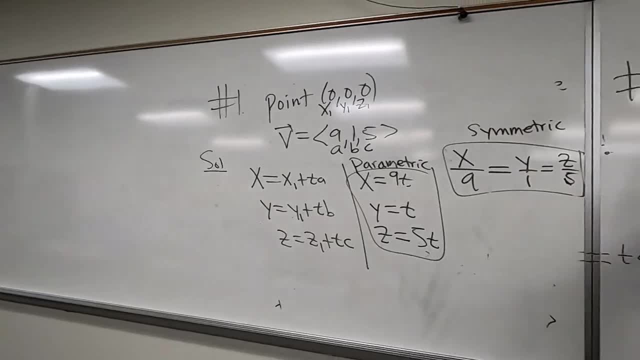 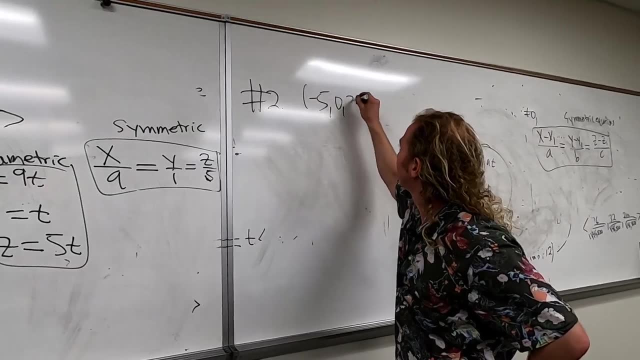 Let's do it So. number two: We've got time, Nikki, can you read me the stuff? Number two: Mm-hmm, The point is negative: 5, 0, 7.. And b is 5 i half plus 4, j half minus 8 k half. 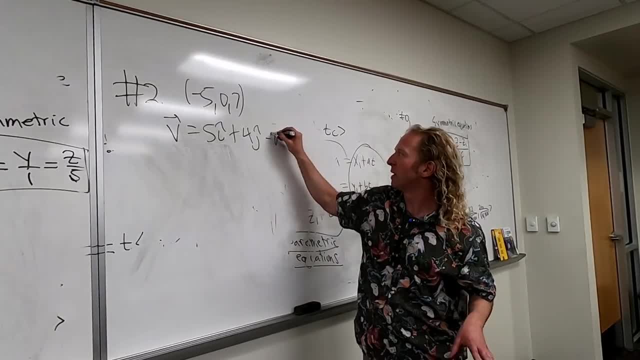 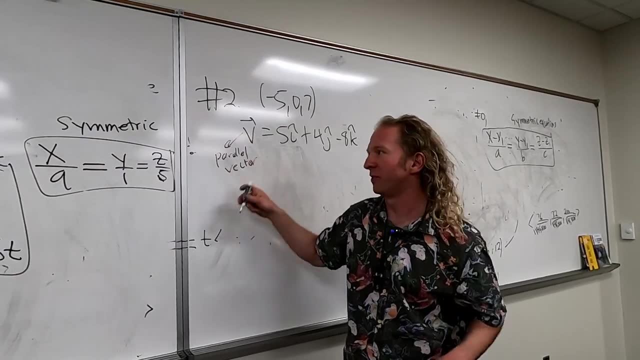 What is it? Plus 4 j, minus 8 k, And this is parallel. So this is our parallel vector. OK, All right, I probably should have emphasized that over here. This is our parallel vector V. this is our point. 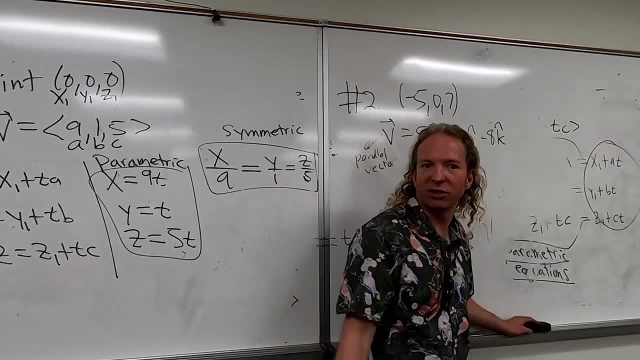 Do you all want to try this one on your own? maybe, Maybe, take, yeah, try to do it. So just try to plug it into the formula, See if you can get it. And then I'm just going to look at the homework. 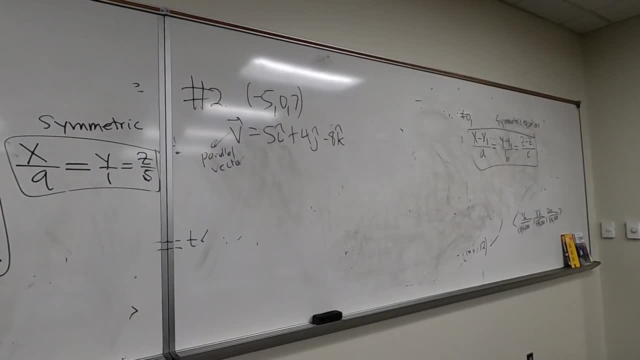 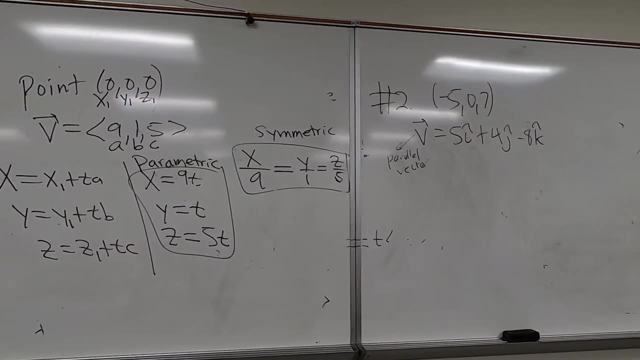 while you try it. I'm just going to see what's up, See if it gets harder, Because I'm assuming it does, But I haven't looked at it since last semester. Let's see. Oh wow, Oh wow. 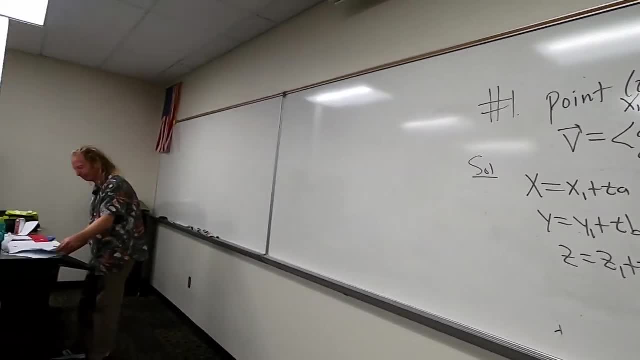 Parallel. So you have to. So 3., 1., Ah, 3., 4., 5., 6., 7., 8., 9., 10., 11., 12., 15. 16.. 17., 17., 18., 19., 20., 21., 22., 22., 24., 24., 25., 26., 27., 27., 28., 29., 29.. 30., 32., 33., 33., 34., 33., 34., 35., 36., 35., 36., 34., 42., 54., 35., 58., 51.. 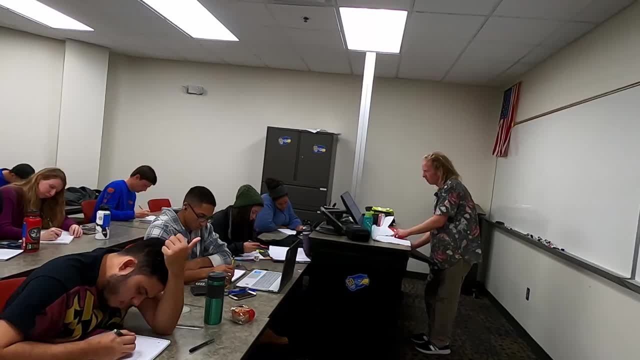 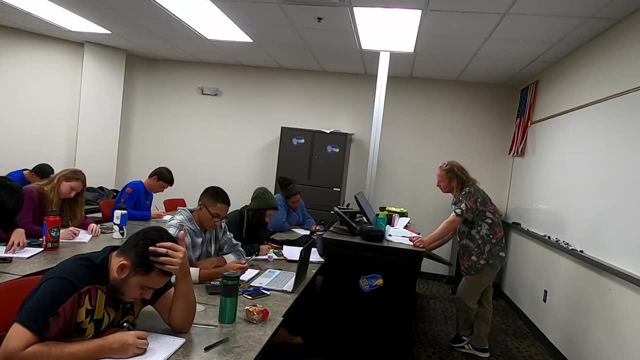 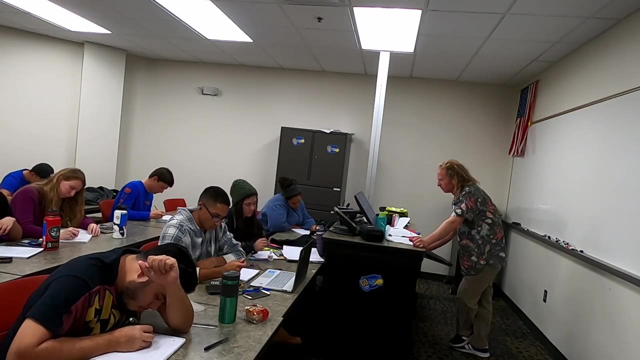 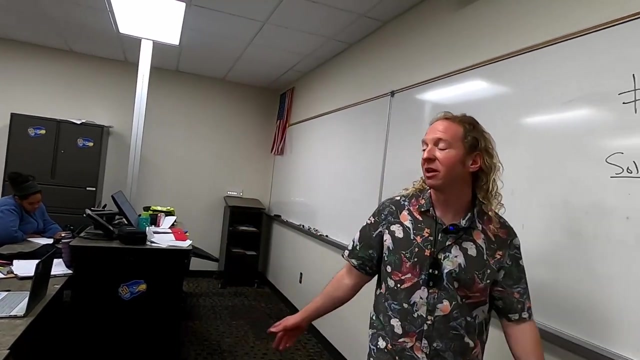 62., 52., 53., 53. 53. interesting, yeah, apparently i have all of the homework problems worked out for this section too. so after class, if you want, you can take pictures of my notes, although the numbers are a bit different, but they're all there, i thought. apparently. i thought this section was hard. 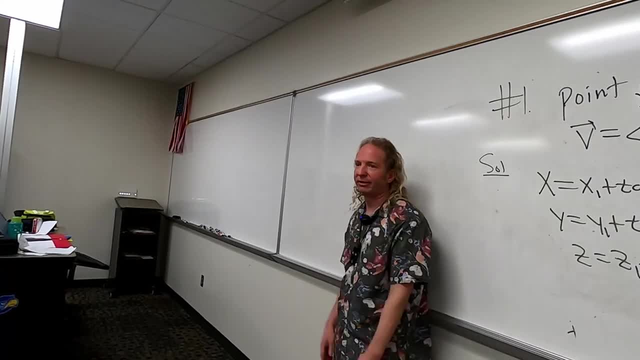 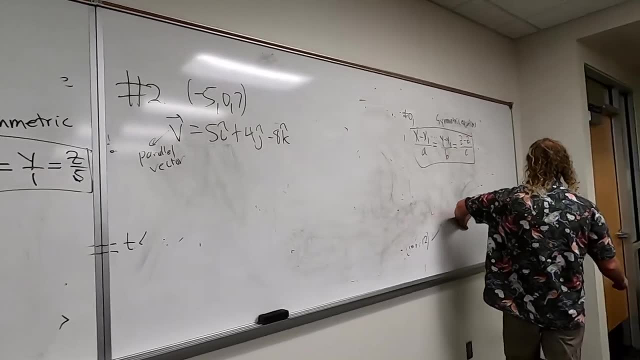 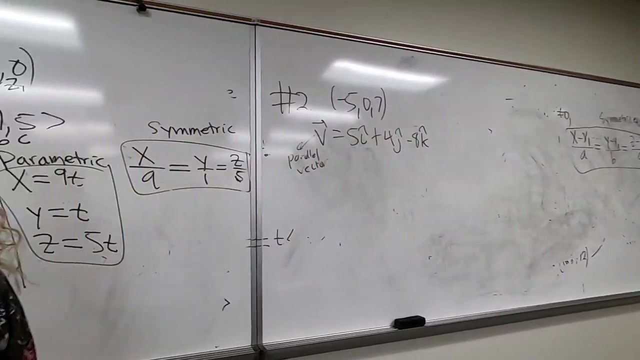 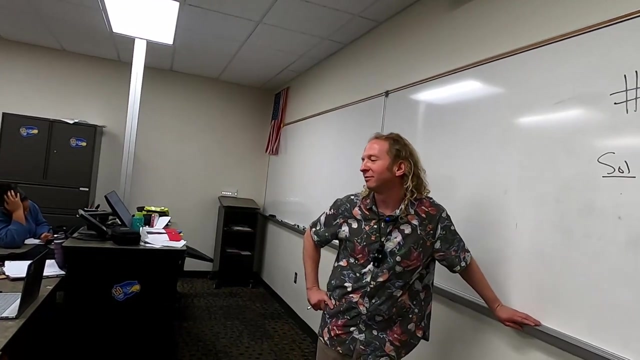 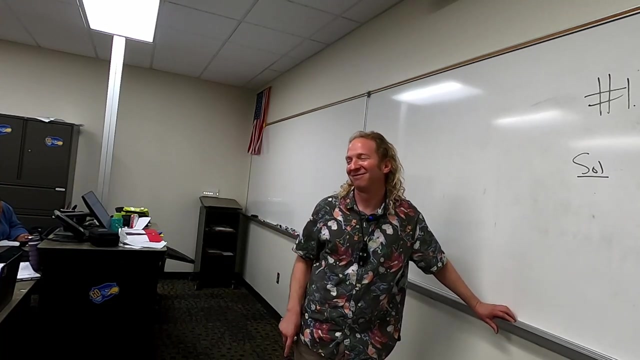 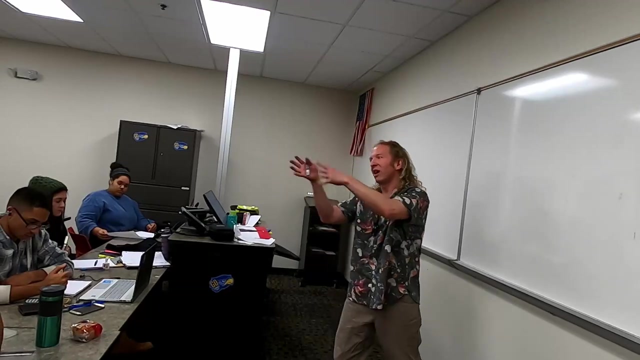 so i kept the homework. usually i just throw it away, but i kept it. it's like meaningful. do you have to stay here anyways, isaac, like till this late, or no? oh, no matter what. oh, okay, okay, so it doesn't matter. okay, good, so i don't feel bad for you. 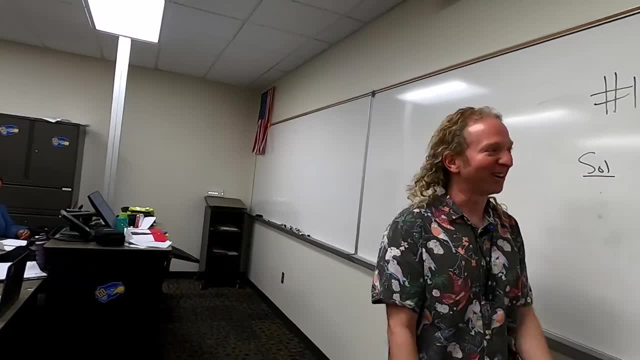 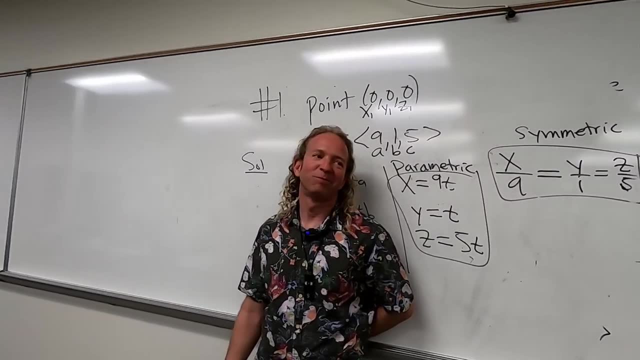 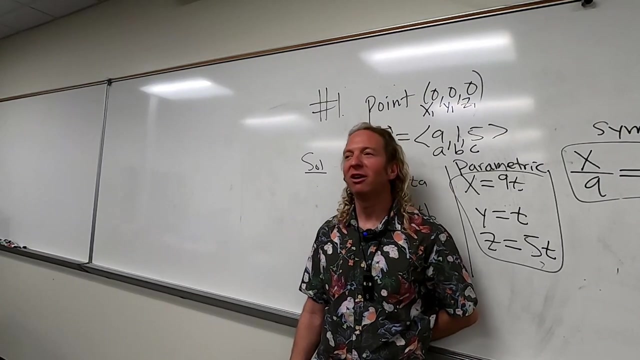 i mean, no, i shouldn't say that. no, okay, it's great, almost volunteer hours. how many do you need total? how many hours before some stuff? i've never volunteered. well, i volunteered here at work, but that's work, it's like a job, so like like i volunteered for, like i volunteered to help. 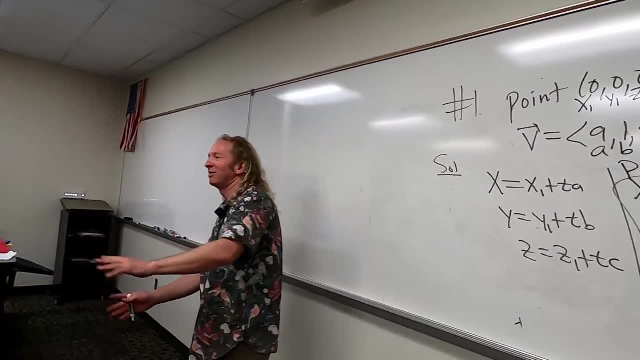 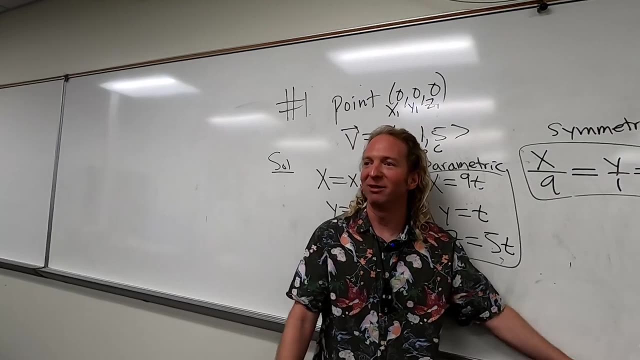 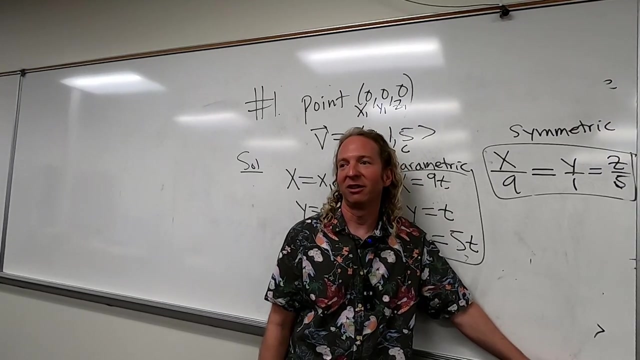 people at work with work things, but not like outside of this. i've never, like you know, i've helped people with two things like i give people rides, and they're not like my official volunteer hours. i know like a lot of med students volunteer, that's cool students. 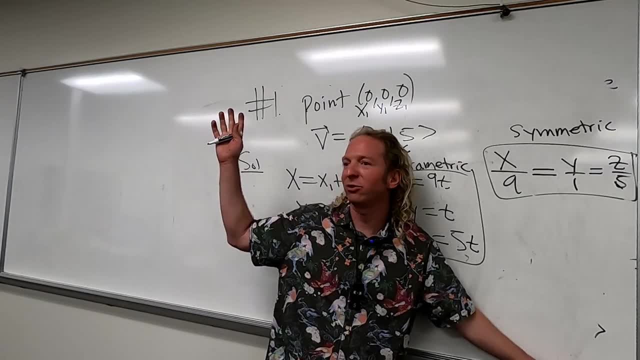 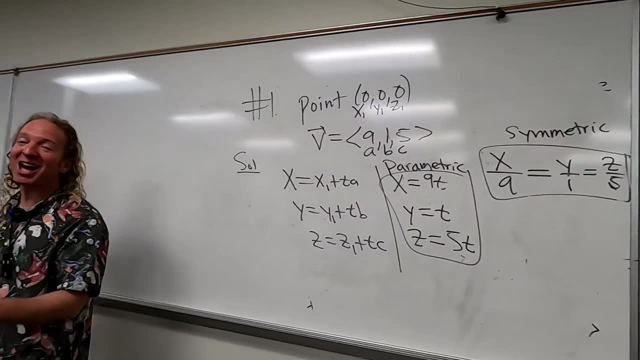 they have to have like volunteer hours and stuff. anyone going to med school here? any med school students? yeah, i know it's very unlikely. i was like i'm like no one's gonna raise their hand. yeah, yeah, i had a med school student in calc two once. yeah, his name was anup. he would drive two and a half hours to come to class here. i remember 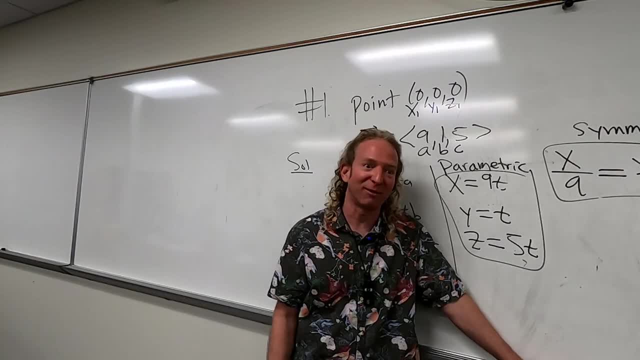 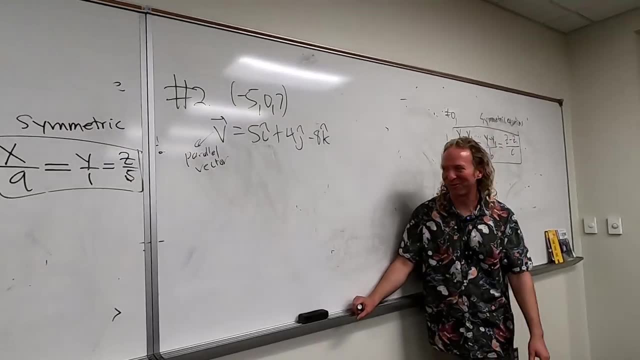 i wrote him a recommendation for med school. i know i tried to make it as good as i could. i'm like i'm a terrible writer. i hope he gets in. i don't know what happened to him. it's been like four years. he wanted to take it to uh further his application. he said that some med schools 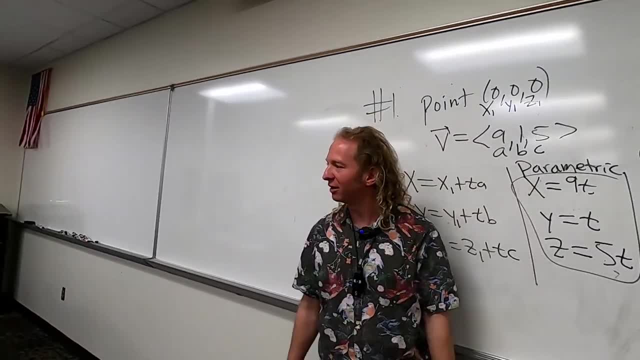 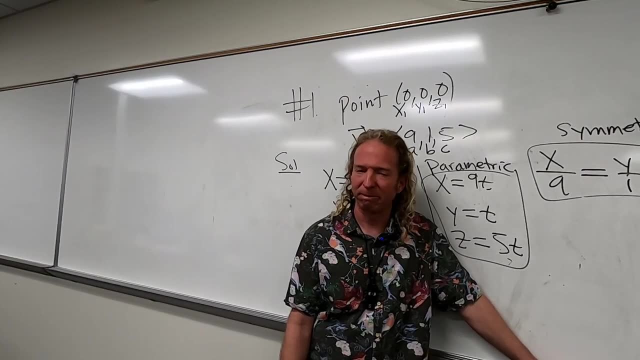 look favorably upon that. He was really trying hard to get in. He's really Maybe. yeah, He lived in Jacksonville, I think. Yeah, he was taking a night class. Yeah, he was really. I mean, he did all the homework. 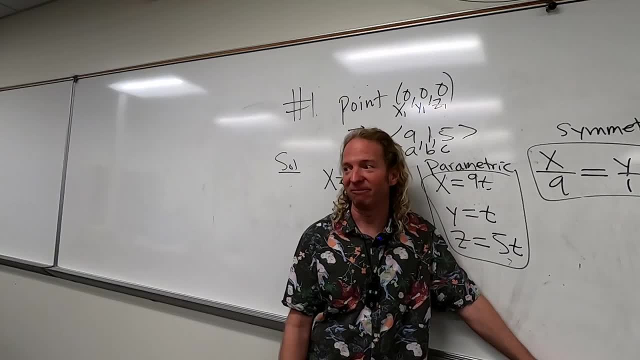 I mean, the guy was like a rock star, Like he worked really hard, Hundreds. All right, let's do it. It's a solution. I know, Yeah, it's interesting People, you know, come and go. 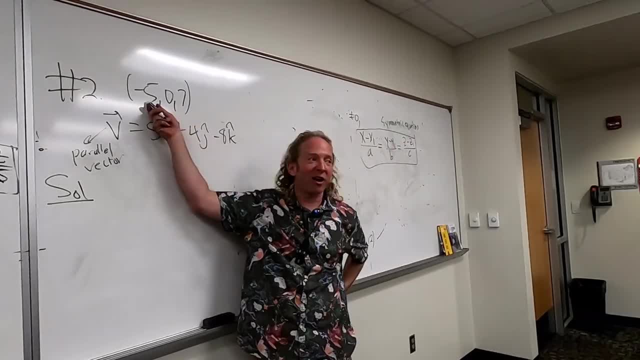 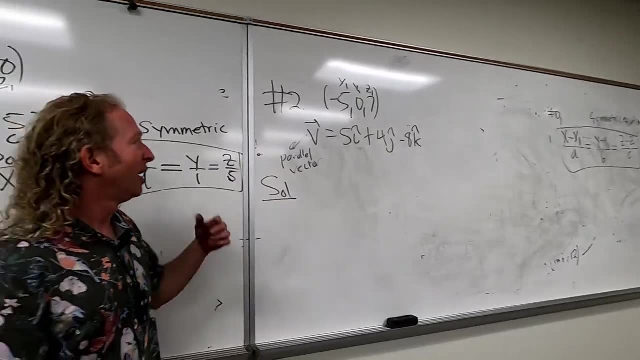 They do, they do. It's weird. All right, so these are X1, Y1, Z1, right, So X1, Y1, Z1.. X1, Y1, Z1.. And Oh, I'm going to write this in component form. 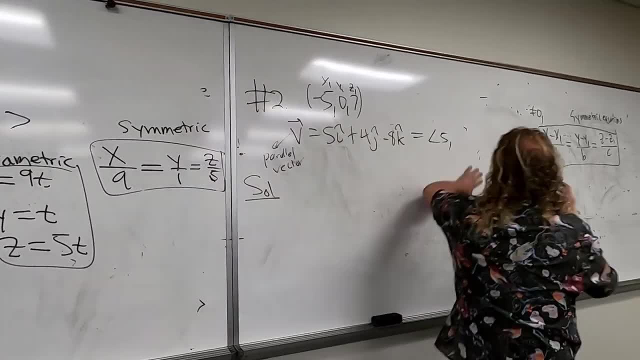 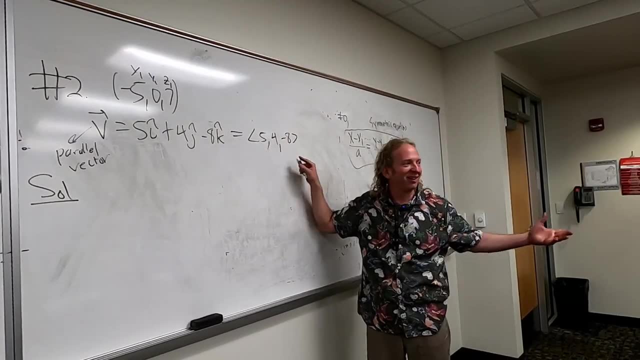 because it just looks better. So that would be 5,, 4, negative 8.. So what are these letters? Do you remember A, B, C, The direction numbers? Yeah, good stuff. So now we just use the form. 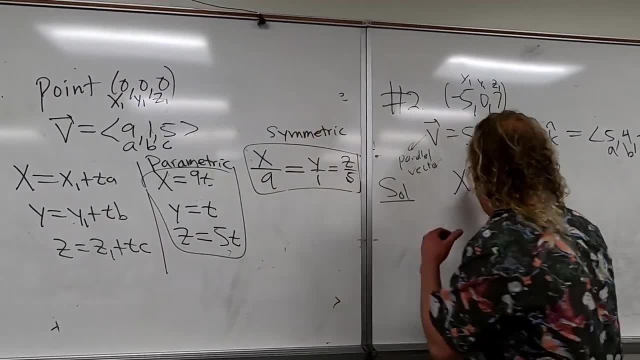 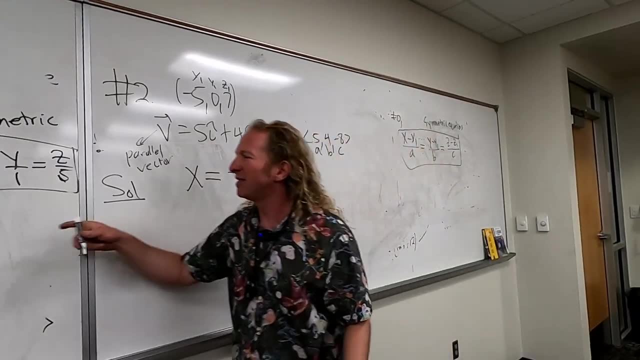 We just use the formula which is here, So I'll just jump to it. So it'll be: X equals, So X1 is negative 5 this time, So negative 5.. Oh you know, it's AT right. 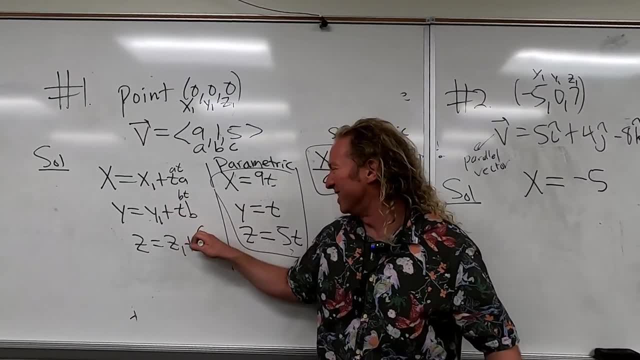 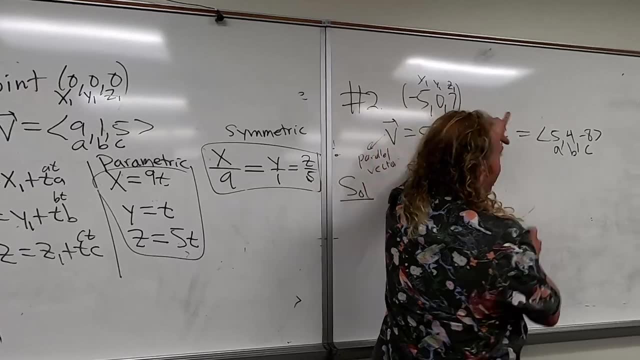 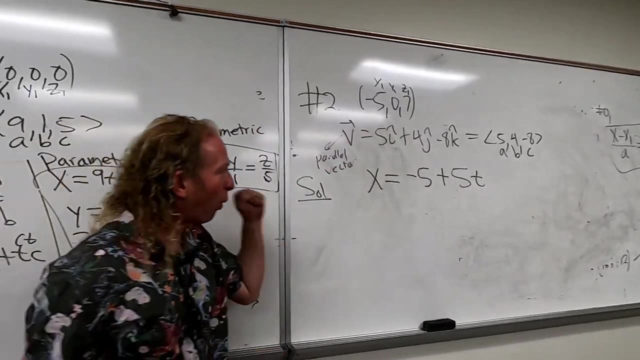 We talked about that. It's really bothering me, BT. I know It's only bothering me, So lost Negative 5 plus 5T Plus 5T, 5T Y Is equal to 4T right. 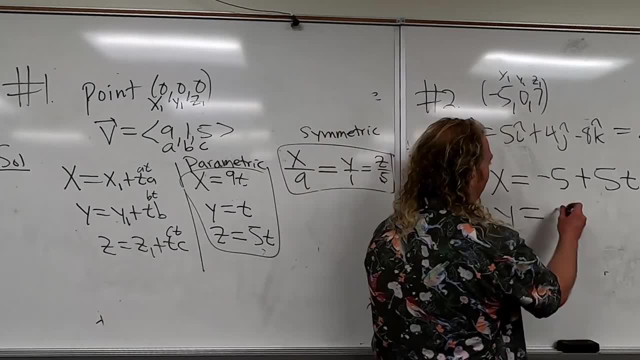 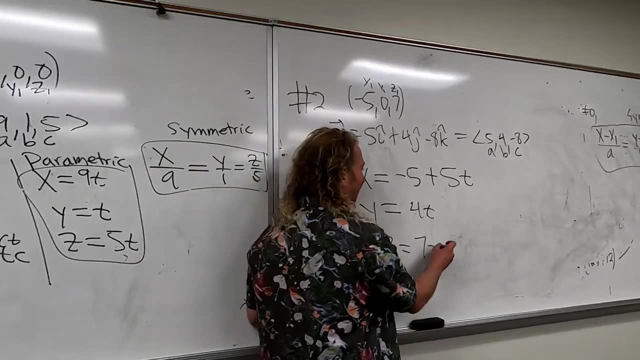 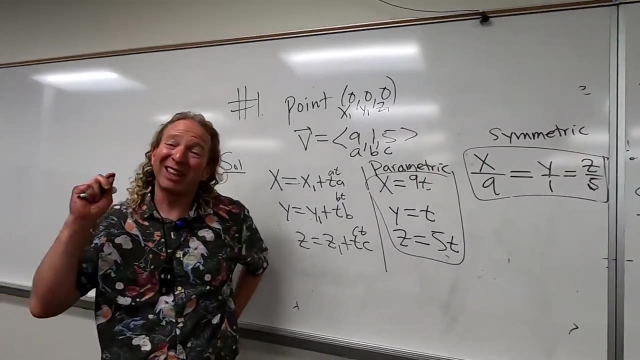 Because the Y1 is 0, right, Very good- 4T. And then Z is 7 minus 8T, Minus 8T. What are these called? Do you remember the Parametric? yeah, These are the parametric equations for a line. 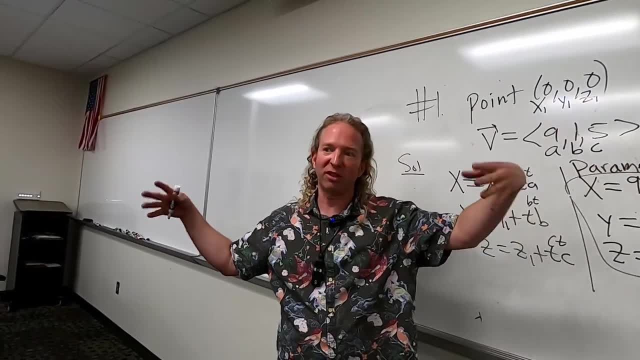 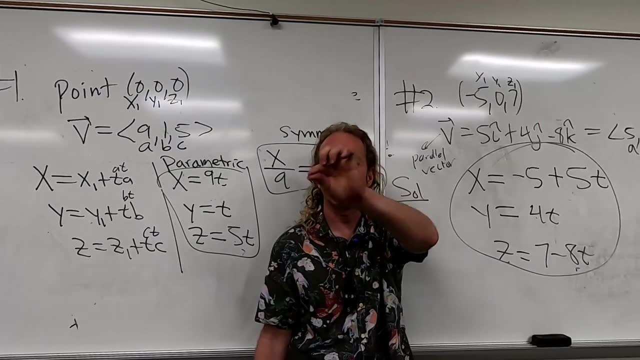 You can find parametric equations for any object in the world in theory. right, It's a big deal. right, It's a big deal. It's a big deal because, As time passes, you can model where something is right. 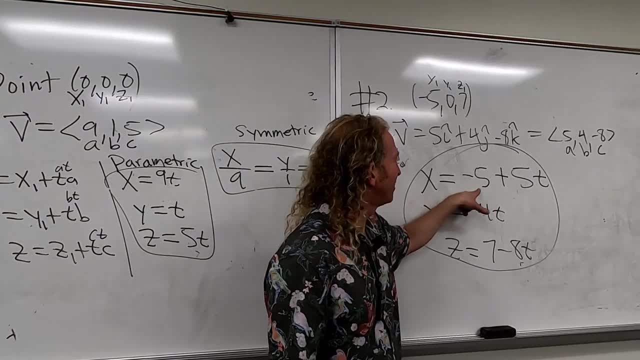 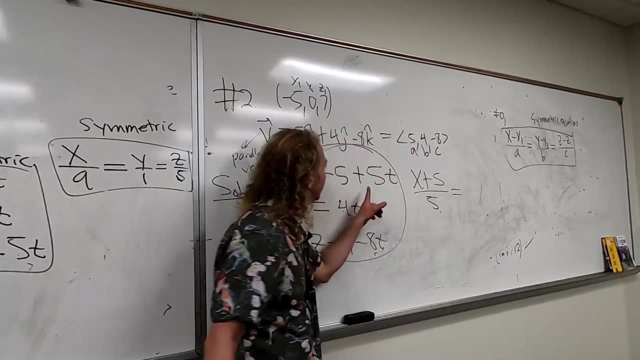 To find the symmetric you just solve for T, right? So in this case we'll add 5, divide by 5. So it'll be X plus 5 over 5.. It's a big leap there. So adding 5 and dividing by 5.. 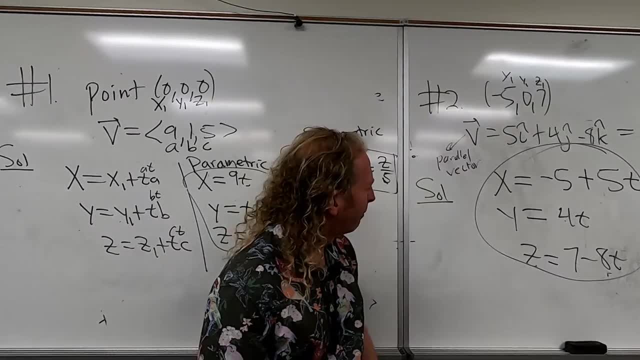 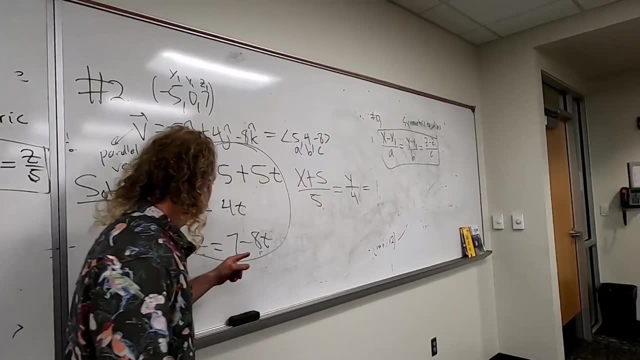 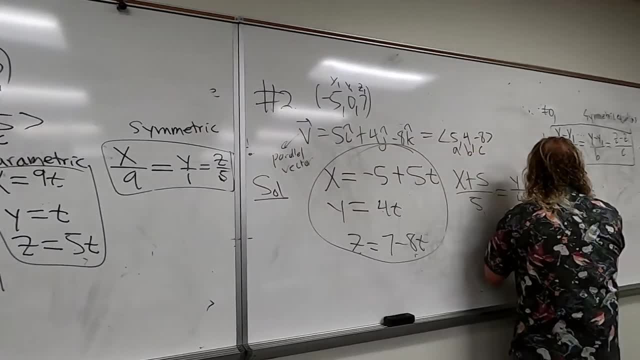 Don't worry about it, Please don't. Someone will, so I'll have to do it anyways, But lots of people will. People will get really creative, Like that guy last semester. he was like: you know, oh, you know, multiply by 20.. 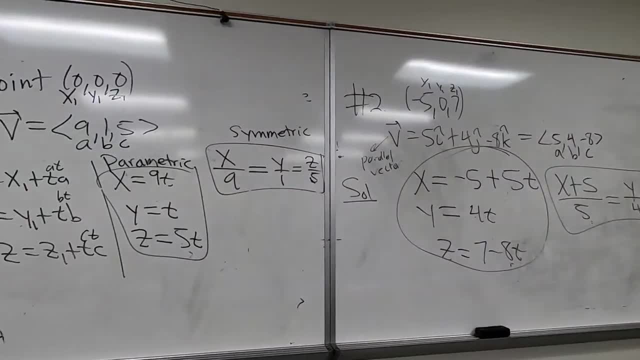 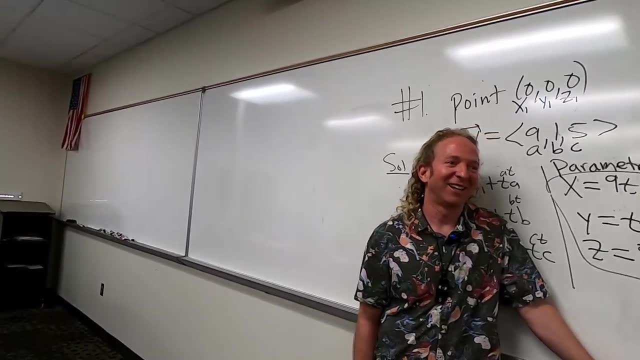 Like you know, It's just ridiculous. I don't even know what his name was, I just remember the test. I'm gritting it. I'm like, oh, what the heck? Yeah, I have a different answer. They do. 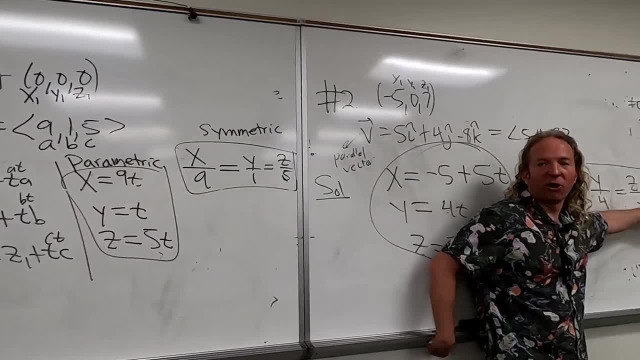 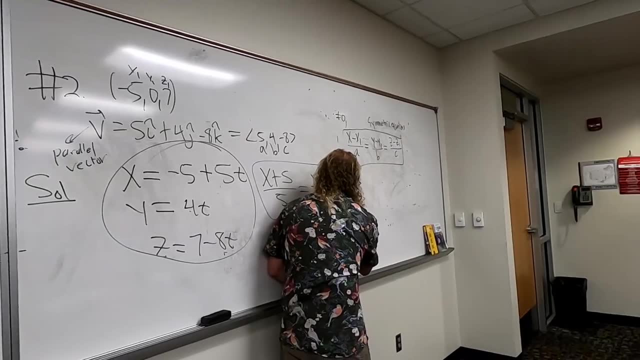 7 minus Z over 8.. Okay, So the homework? Yeah, they did it in negatives, In negatives. Okay, Yeah, so the homework does this, Thank you. So the homework does this? Yeah, They do that. They distribute the negatives. 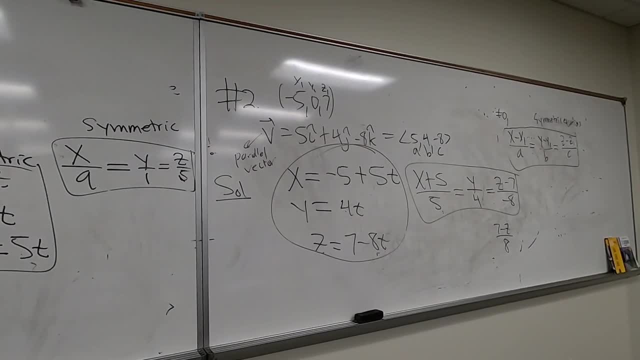 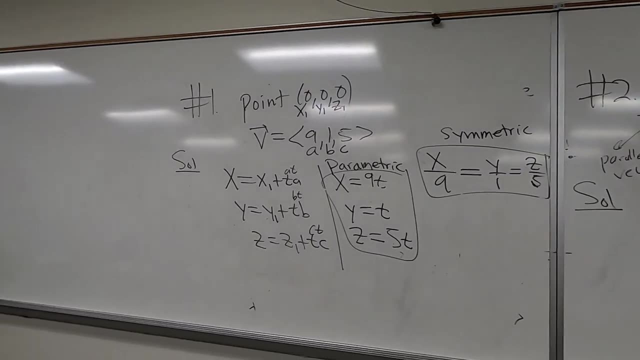 So it's multiple choice in the homework. So, All right, Let's keep going, Let's do. I guess we should try number three. Let's try to do that one. So number three. I think it's a little bit different, a little bit harder. 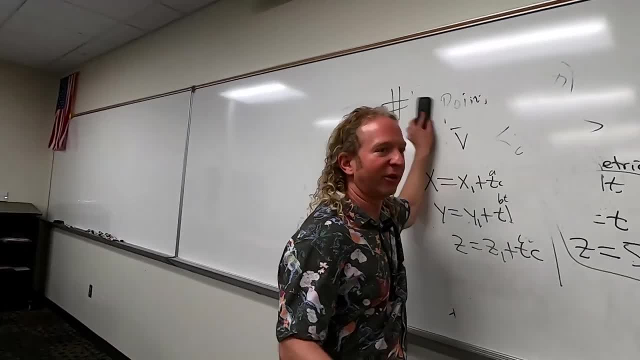 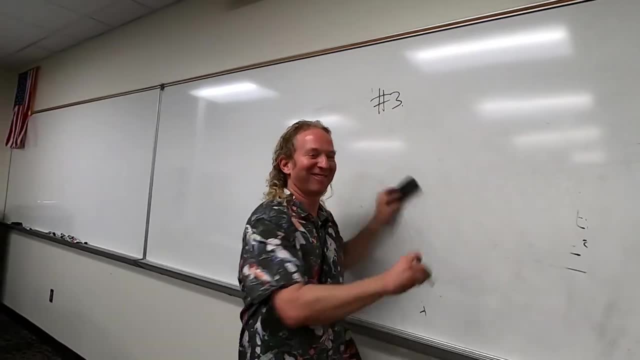 I'm actually not sure how to do it yet, so I have to read it and think about it. I have an idea, I think. So they give us a point. So they give us a point: 7 minus 3, 3 over 5.. 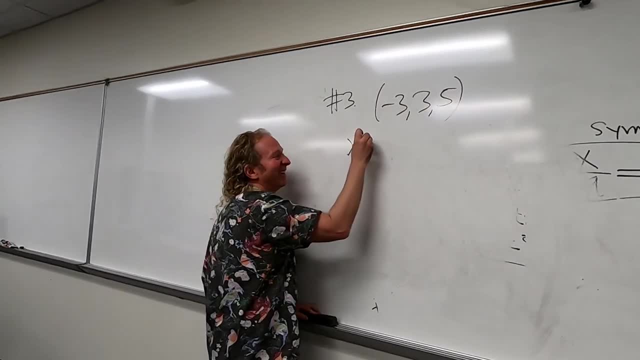 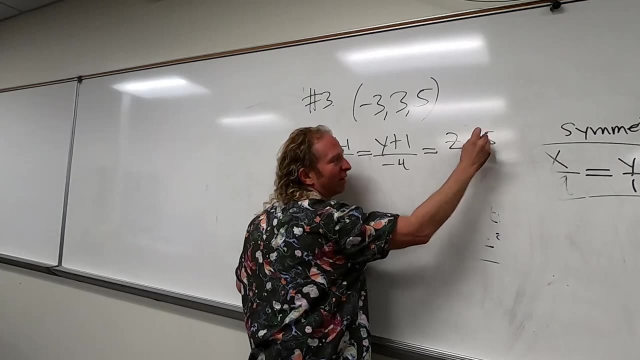 Thank you. Parallel to X minus 1 over 3 is equal to Y plus 1 over negative 4 is equal to Z minus 5.. Like that, Yeah, Oh, thank you. Okay, Perfect, So it's parallel to this. 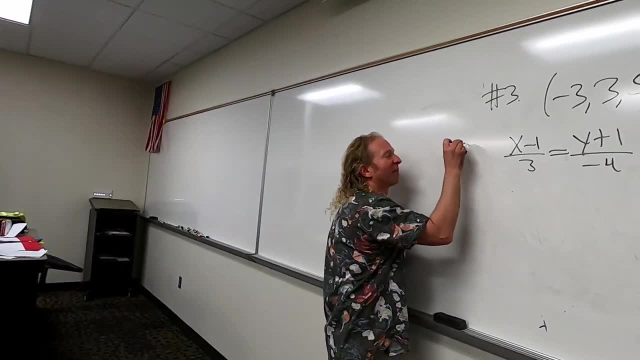 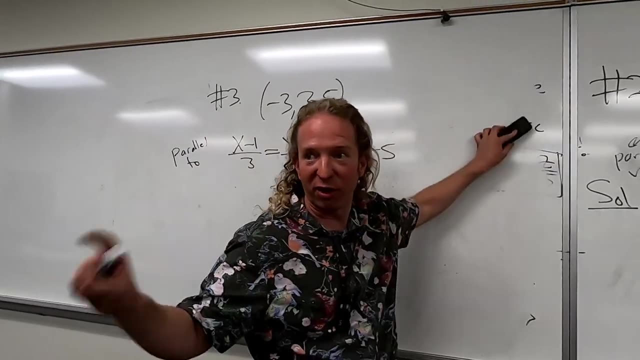 Parallel to this. Okay, Nice question. The ones on the worksheet are a little bit, I think. on the worksheet I put the best ones, Like there's some that are in the book that aren't in the homework and they're on the worksheet. 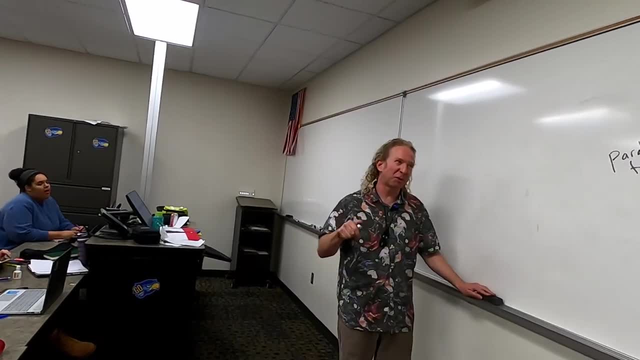 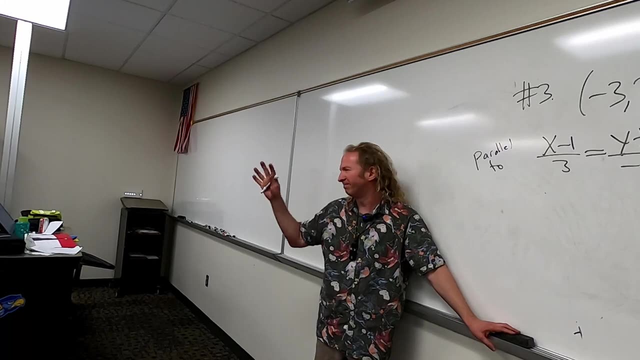 So when you stay for the worksheet, please stay right, It'll help you, okay, Especially today's worksheet, Last time's worksheet, don't even worry about it, You don't even have to do it probably, I mean, unless I reference it when I make the test. but 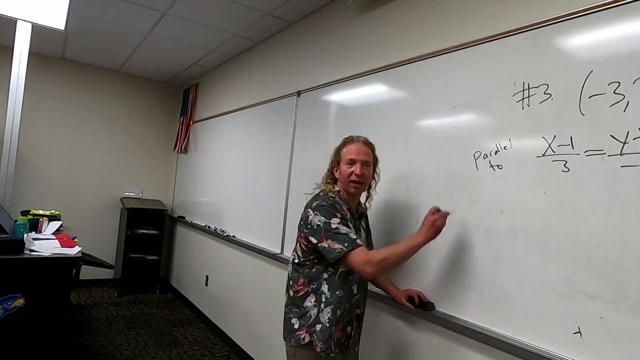 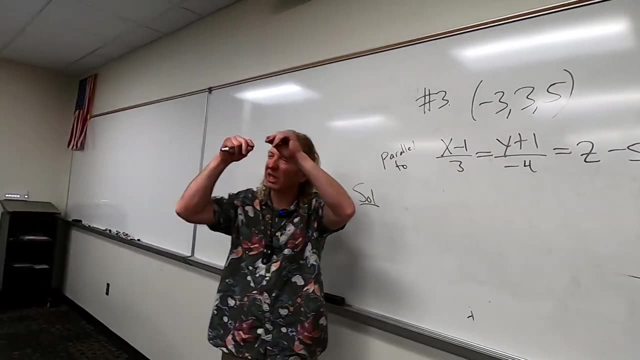 Yeah, You don't even have the answers for it. so Okay, Solution: huh, No, but still online. Yeah. Yeah, if you click on resources and website, all the worksheets are there. You have to click it though. 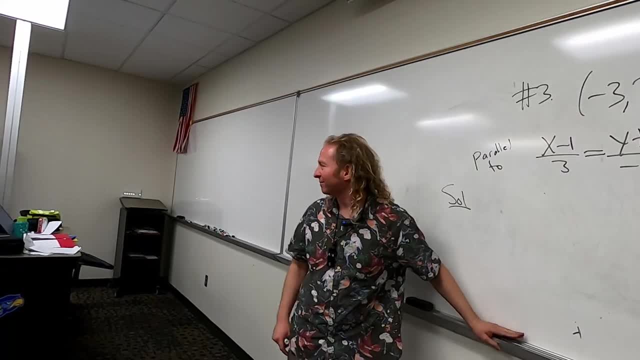 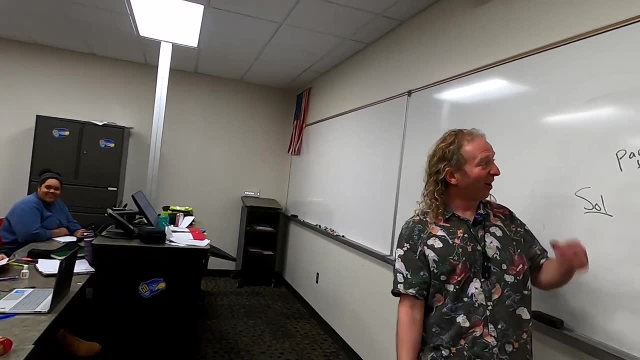 You have to click resources. I'll show you later. I know they made it, so you have to click it. I know you have to click it. I know because people don't know, right? All right, so we have our point, right. 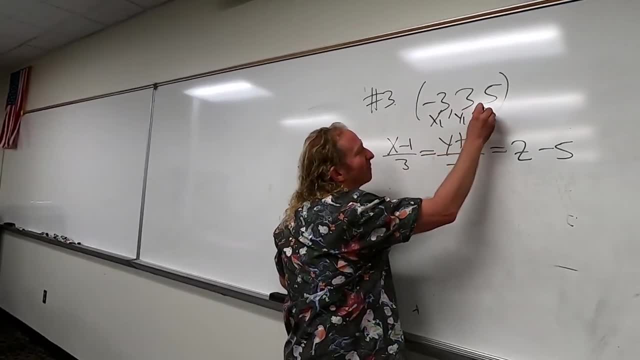 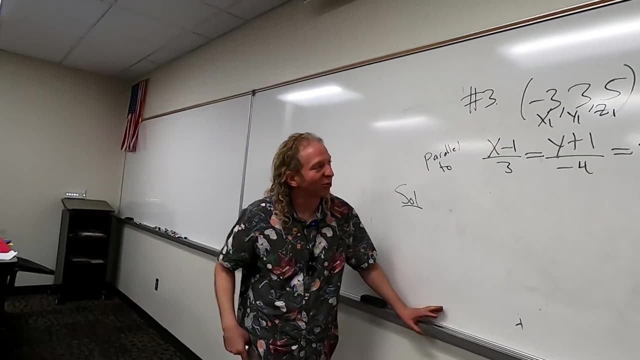 That's our X1, Y1, Z1.. And this is really over what number here? One Good Josh, It's over one. Very good Josh, Excellent, It's over one. So now we can find our ABC. 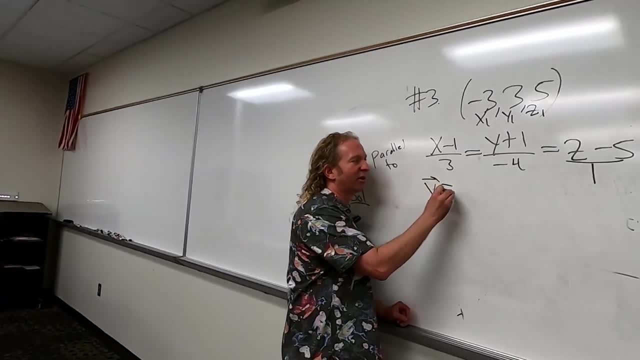 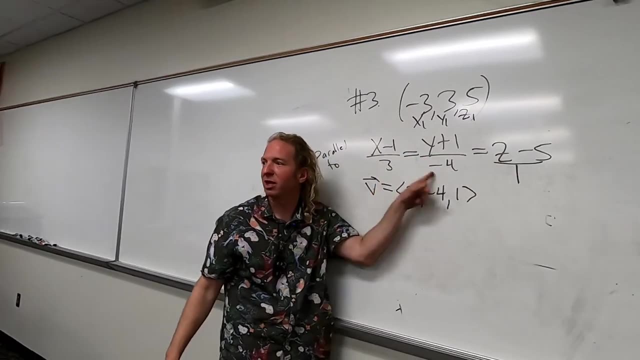 So I'm going to go ahead and write down our direction vector, just to be pro. So it'll be three Negative, four, one right. Those are our direction numbers, right. A, B, C, right? You see that? 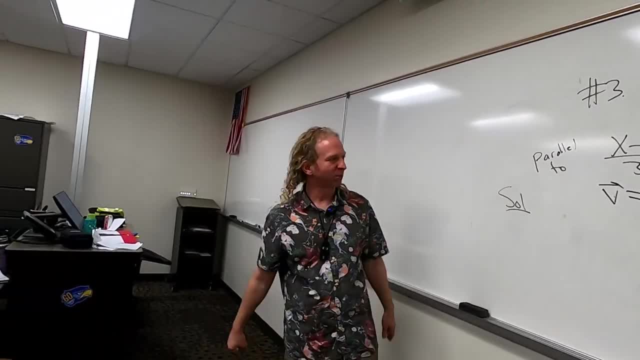 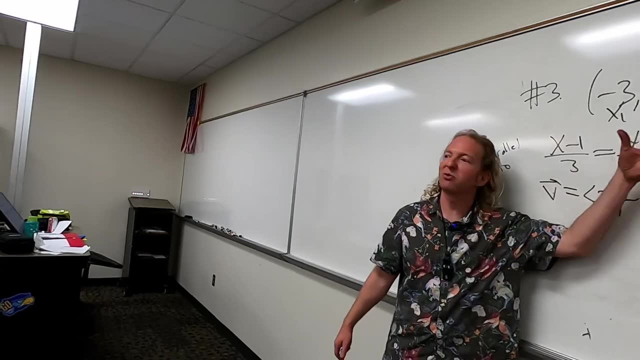 Those are the ABC direction numbers. Okay, And that's it right. That's it Now. I thought it was going to be harder. I think the harder one is the plain one. There's one like this with planes and it's really tricky. 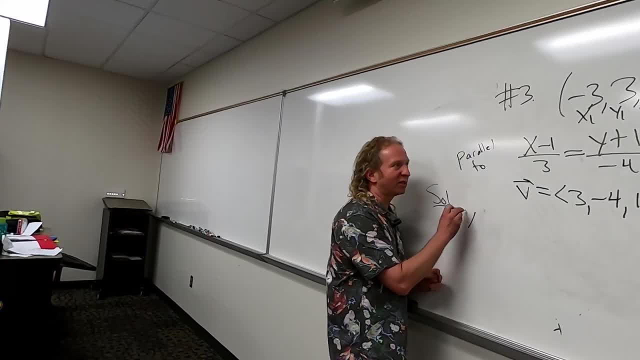 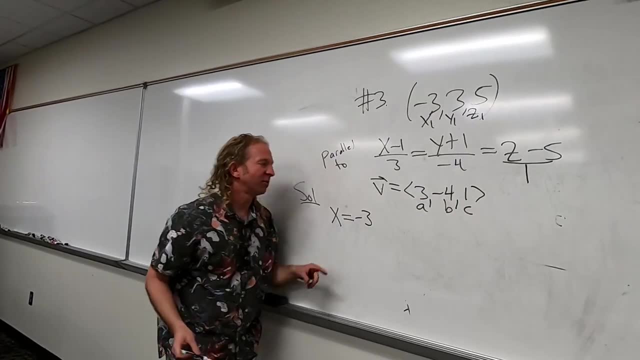 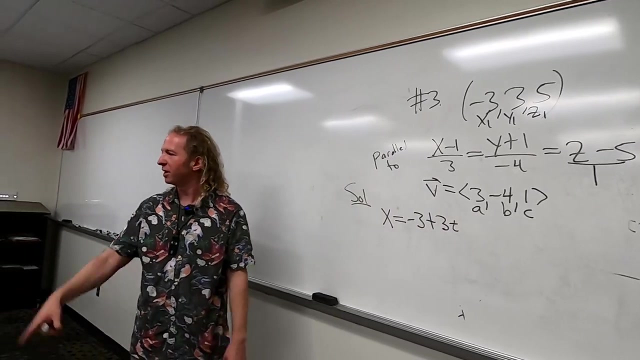 So now we just use our formulas right. So let's do it. So it'd be: X equals, So negative three. This is our ABC. So it'd be negative three plus three T. right Plus three T. Yes, Kamal. 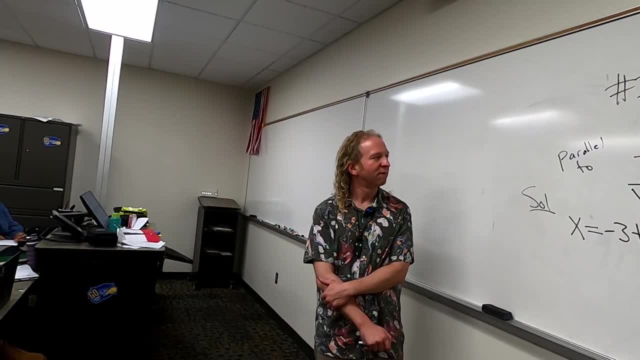 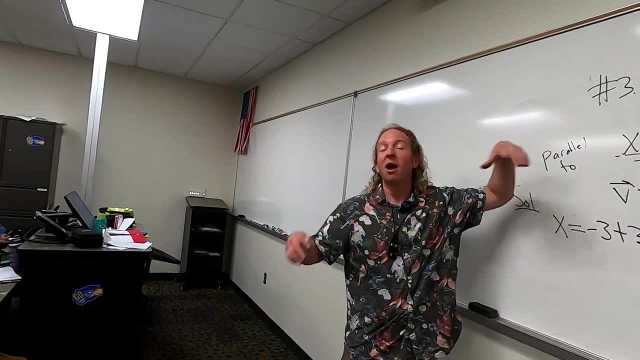 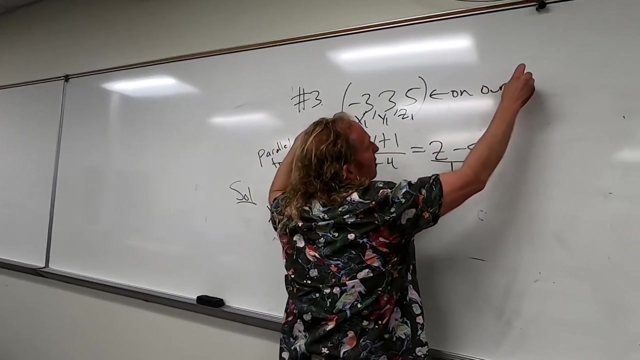 It's like X minus one over three. Shouldn't the X one be negative one? No, Well, it will for this line, But our line is parallel to this line And this is a point on our line. Hmm, It doesn't matter. 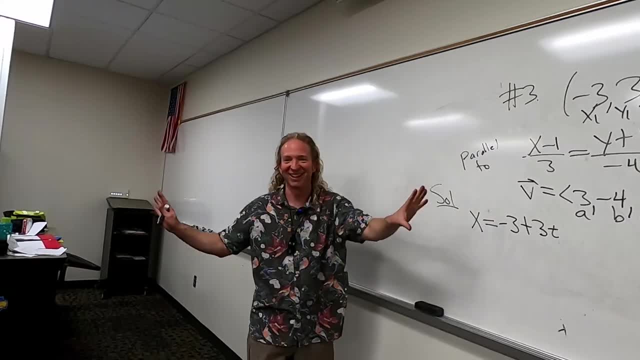 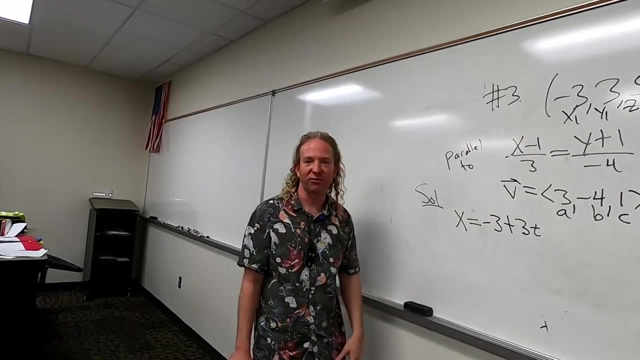 Yeah, this is a different line. Yeah, Yeah, No good. Yeah, it's different. Yeah, so our line is parallel to this one, right? So it's different. And then Y would be three, right, That's our Y1, right? 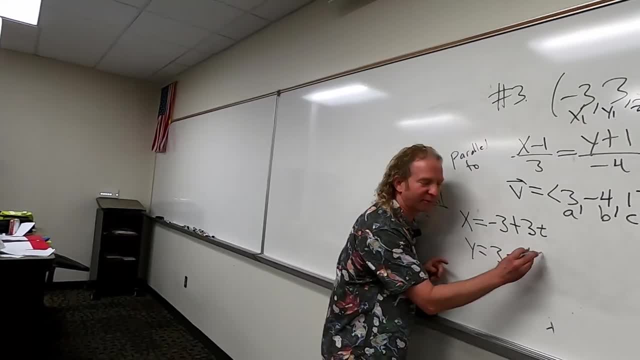 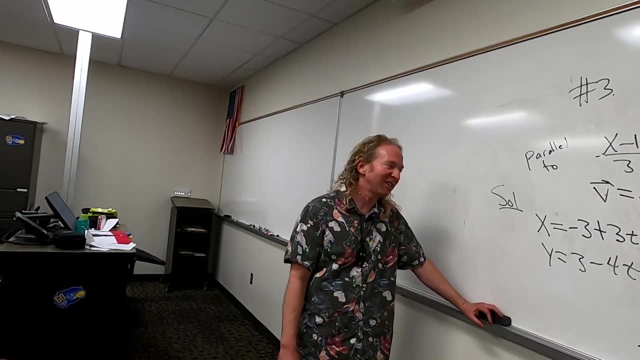 And then minus four T. Every time you write four T it makes you think of the number 40, right. Four T, Four T. I always have that Four T right. It's four T, Four T, not 40, right. 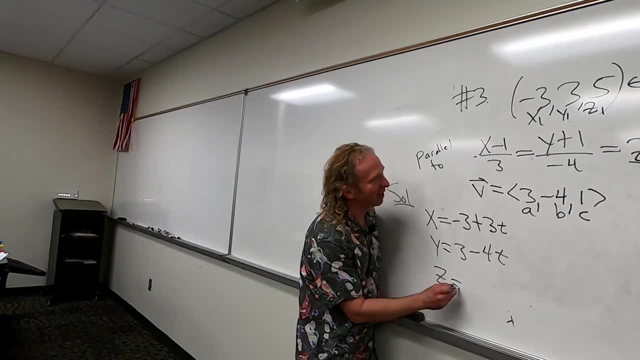 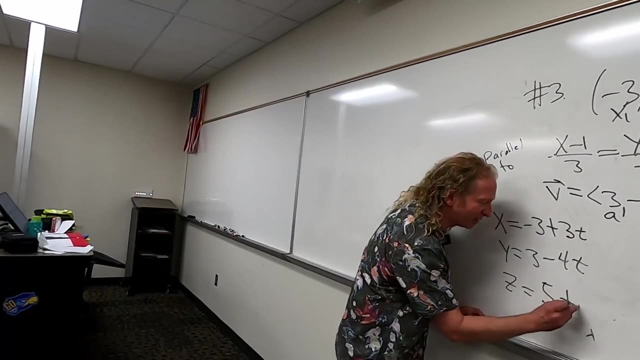 It's just a weird, weird thought process. And then Z is five. five plus T, That's a plus little T. My T's have tails on them, by the way. if you're wondering why I do that, It's so they don't look like plus signs, right? 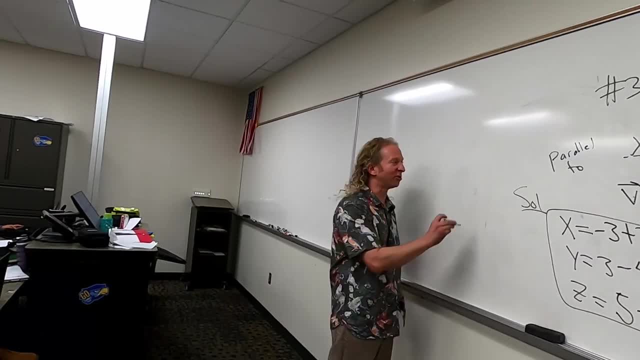 You do a lot of math. You just have to make up new letters Like the same thing. I used to do, this two, But then I started to do like calc, three, Two, Z, Ah, what's going on there? 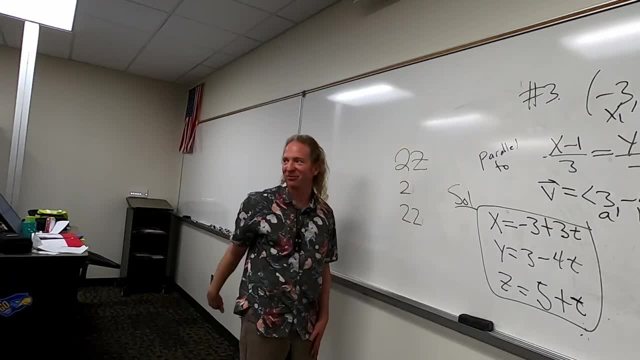 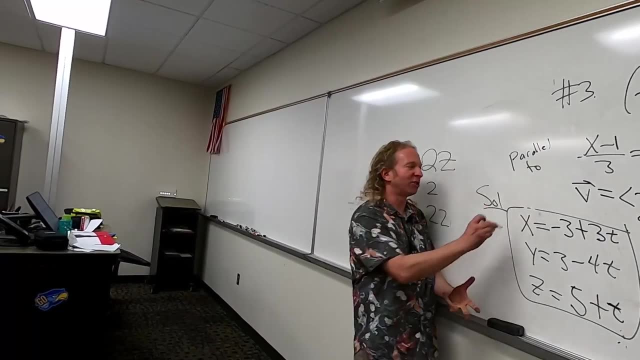 So now I do two Z, Like they're all. They're, like you know, very different. So, whatever works, And these are the parametric. Yes, I'll write it parametric, Because on your test it will say: like part A will want parametric. 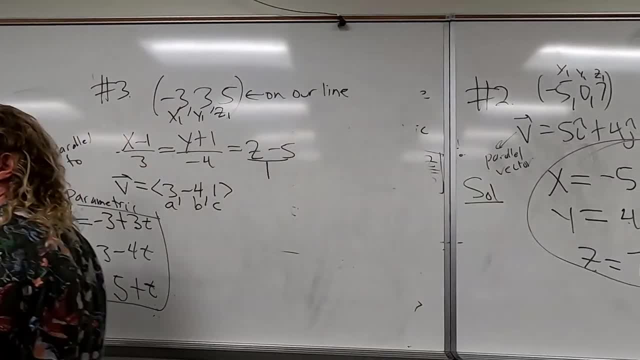 Part B will want symmetric, So you have to like, put them in the right place. So you're just looking for the equations. Mm-hmm, Same, Yeah, all these are the same. Just want the equations, Yep. 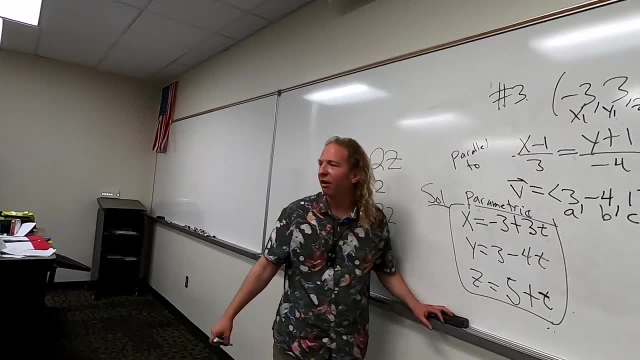 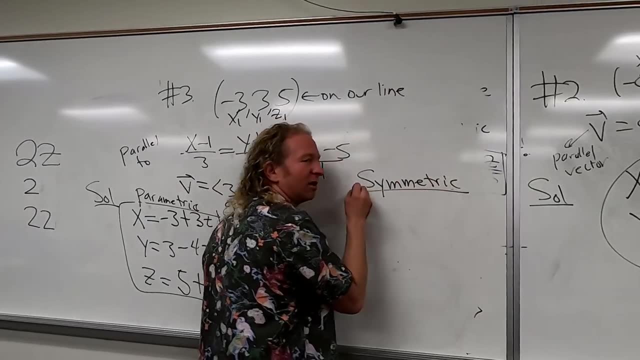 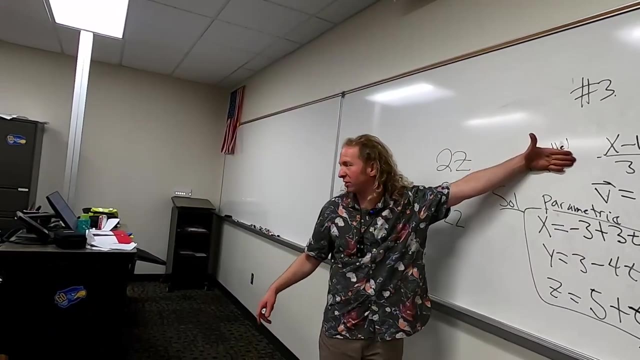 Any questions on that part? All right, Let's do the symmetric, Symmetric, Symmetric equations. So for the symmetric, we take this one and we solve for T. So we're going to get different symmetric equations than this, right? 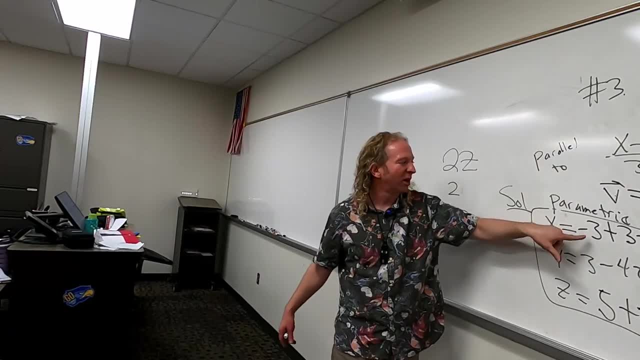 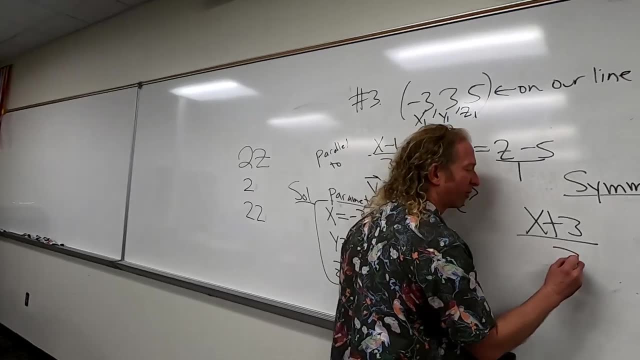 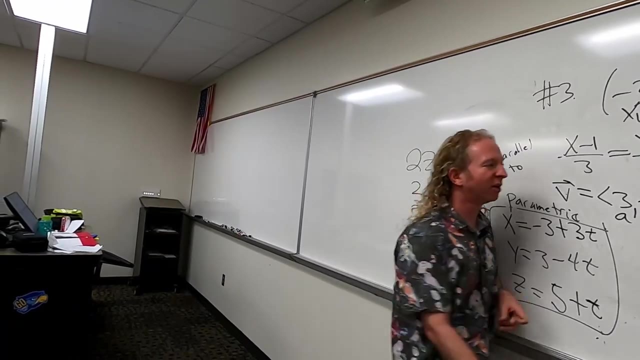 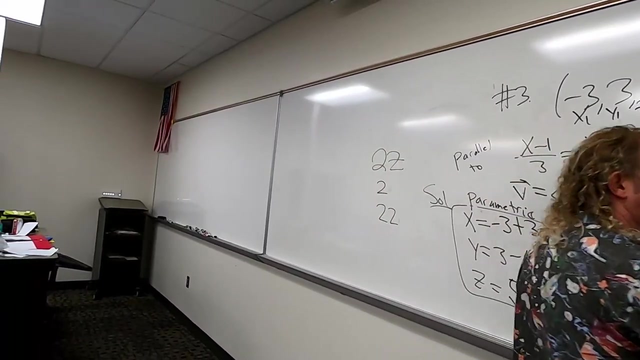 So this is some. Our line is parallel to this one, So it'll be X plus three over three, So X plus three over three. We're adding three and dividing by three. Y minus three. Y minus three over negative four. yep, negative four, very good. 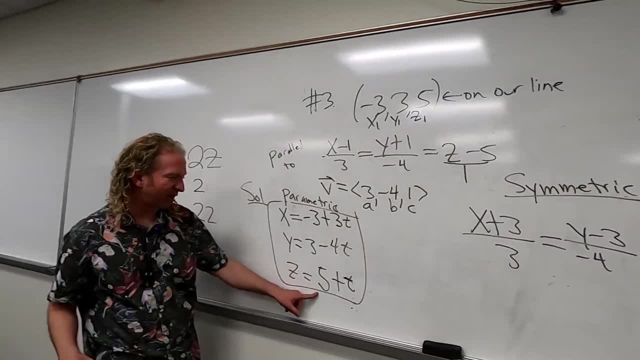 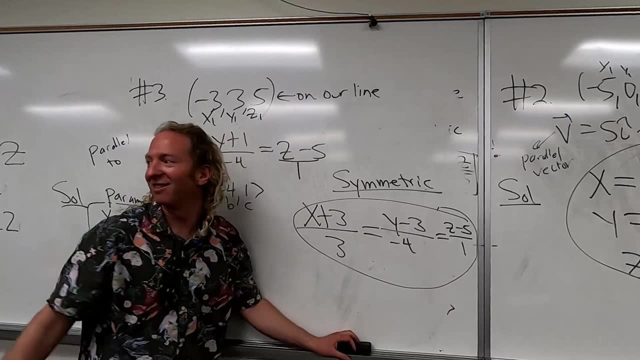 And that's equal to Z minus five over one. I'm going to write it over one just because it looks good. You don't have to. Sorry, man, You're not partnering with us on this episode of SciShow. Thank you. 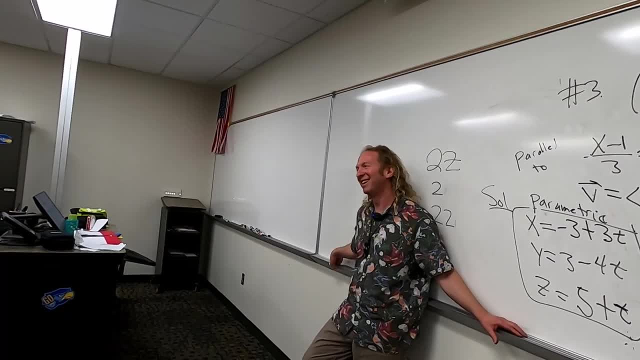 No, it's okay. That was really funny. That's good, That's all right. It would have been funny if it was like a song or something, But it's okay, It's good, It's still good, Good work. 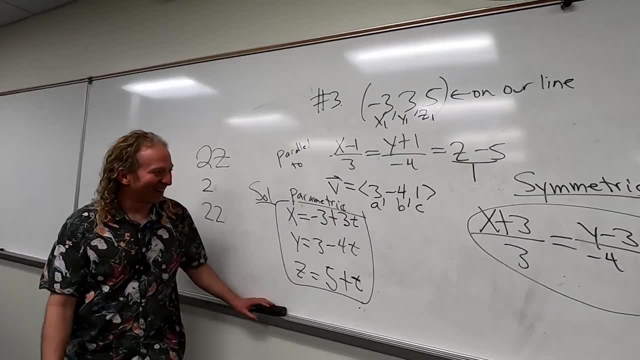 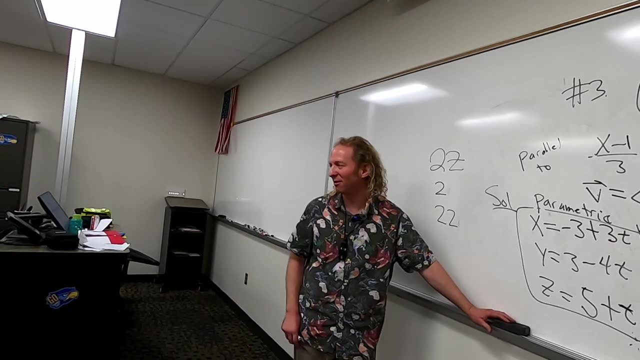 It's all right. It's all right, It's all right. So yeah, I forgot what I was going to say. Any questions? That's happened to me before My phone went off years ago. Never again. It was like some 80s rap song. 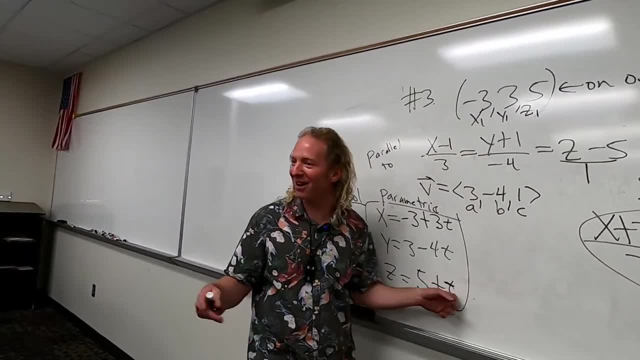 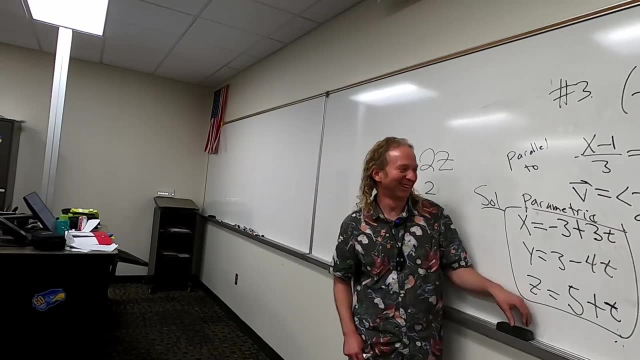 Any questions? Yeah, It was that song. It takes two to think they can go right. Remember that song? Yeah, I was teaching trig. Yeah, And the class just like looked at me, like what? Any questions on this one? 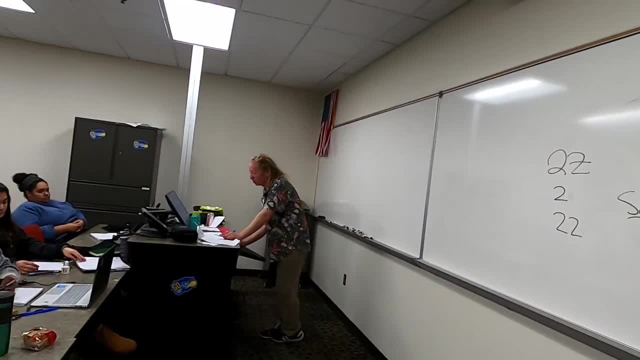 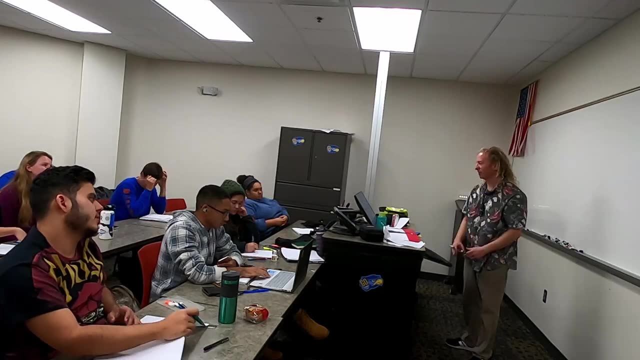 All right, All right, Let's do some more stuff. How about four? I think we should do four, because oh wow. Well, I definitely want to do five because it's easier, But maybe I shouldn't do that. Maybe I should do the harder one. 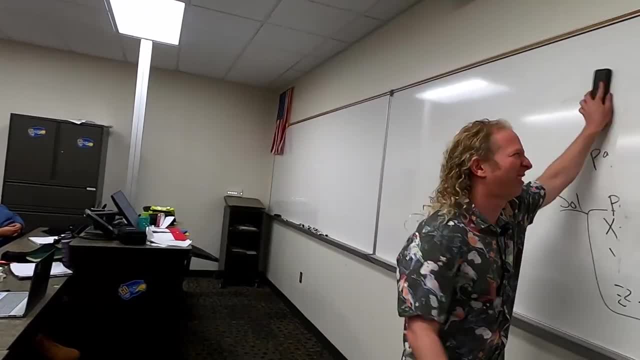 So let's do it. If you don't want to do the hard one, we should do the hard one, We should do the hard one. So four, All right, Let's do it. Let's do four. Four is a little bit different. 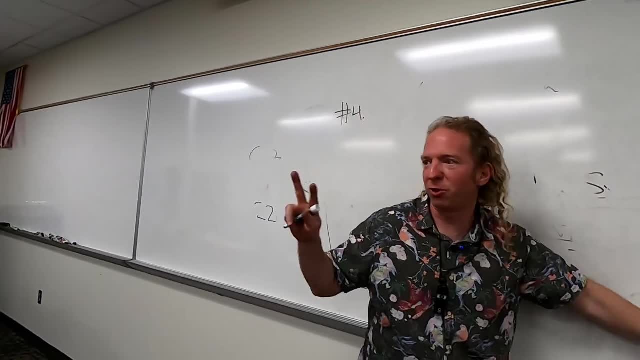 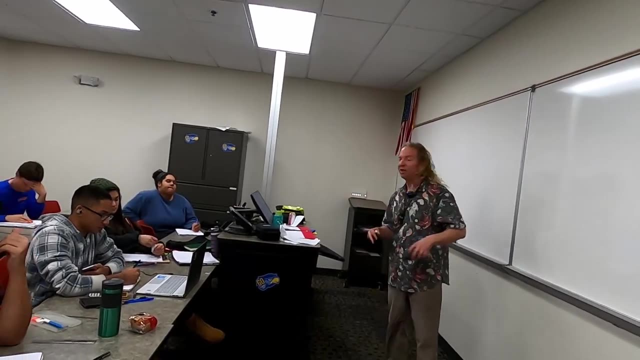 So on four, they give us two points And we have to find the equation of the line So kind of different. A new question. So they're no longer giving us a parallel line. Instead they give us points, So points. 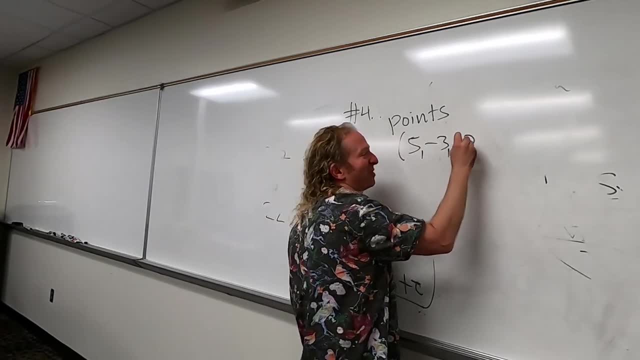 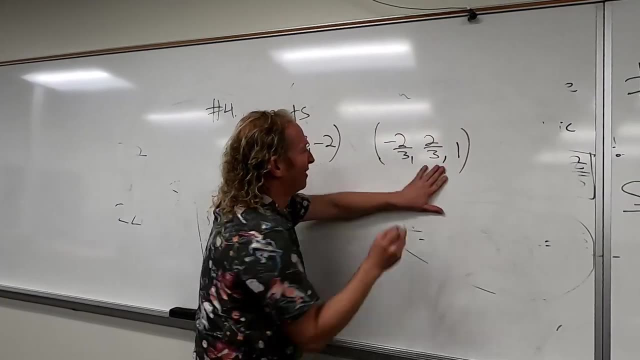 So the points are: negative 3, negative 2. Thank you, And negative 2 thirds, positive 2 thirds and 1. Thanks. Perfect, So we have two points on the line. We have to find the equation. It's kind of cool, right. 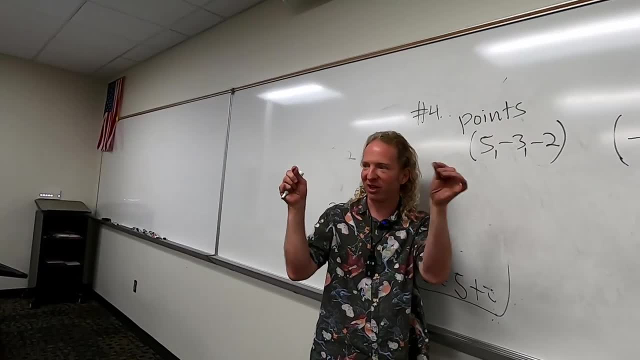 It's kind of like regular math, like a regular 2D, like giving two points on a line to find the equation right, So kind of cool. So if it was 2D you'd use the points to find the slope. 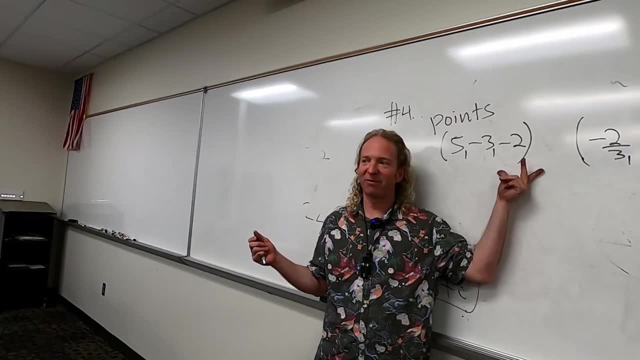 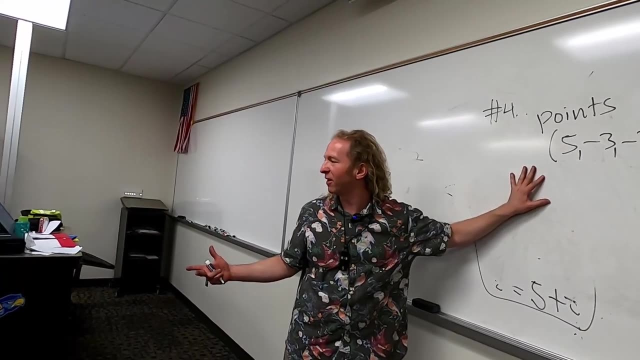 Since it's 3D, we're going to use the points to find the vector, because the vector tells us the slope. So if we have two points, we can subtract them to find a vector, right? So if you have a point here and a point here, 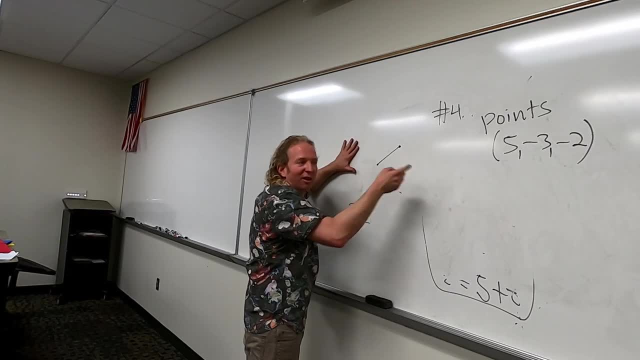 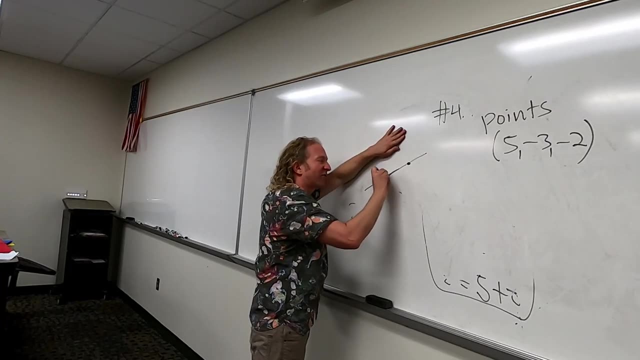 you can form a vector by subtracting the points right, And that gives you a vector. This is going to be a vector that's on the line, Because if this is your line- and here's one point, and here's another point- if you find this vector here, 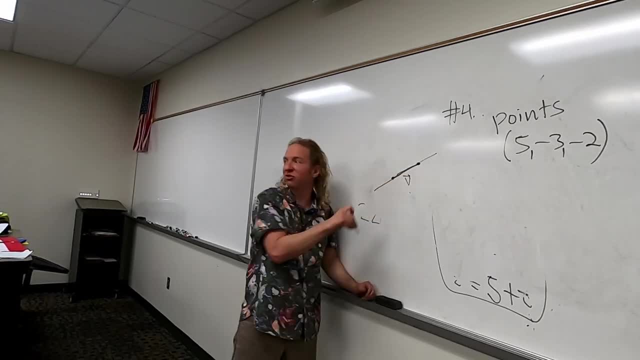 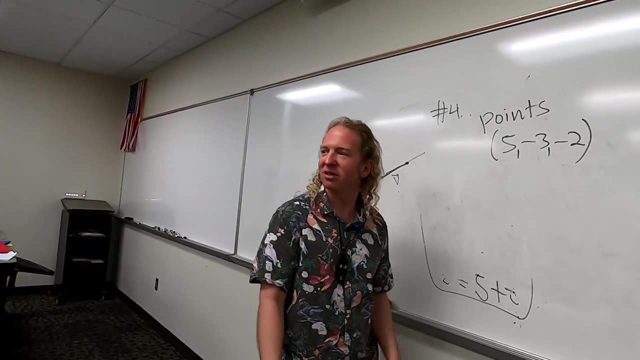 this vector, which we'll call v. it's on the line, So it's certainly a parallel vector, right? So all we have to do is subtract these to get our parallel vector. Does that make sense? OK, good, Let's do it. 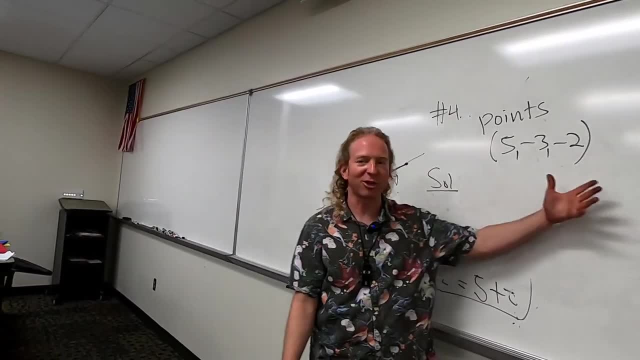 So the really bad part about this problem is what? Why didn't I want to do this problem? Because what, Yeah, the fractions. I'm like, oh my god. So we got this, though. This is calculus 3. Yeah, 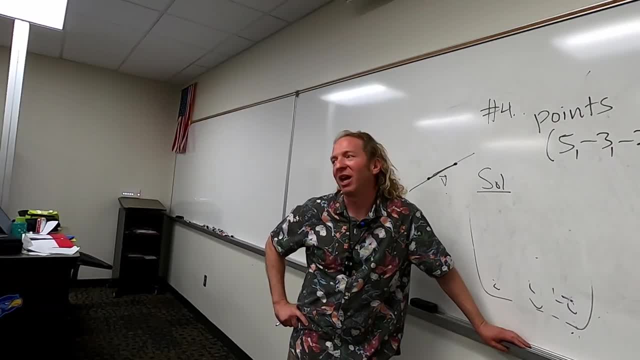 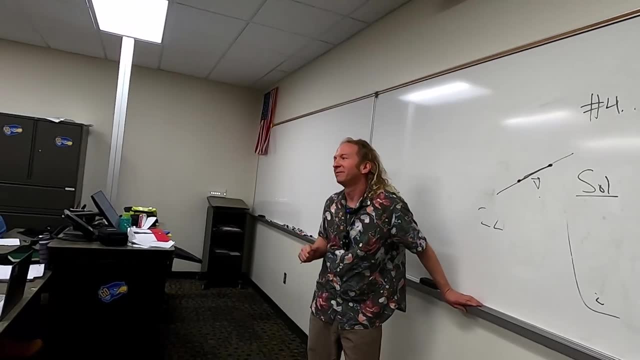 Can you? just, I don't think you can, because you're changing the point Like, let's say: Well, you can multiply the vector by 3. Right, so can you do that here? Not yet, Not yet. 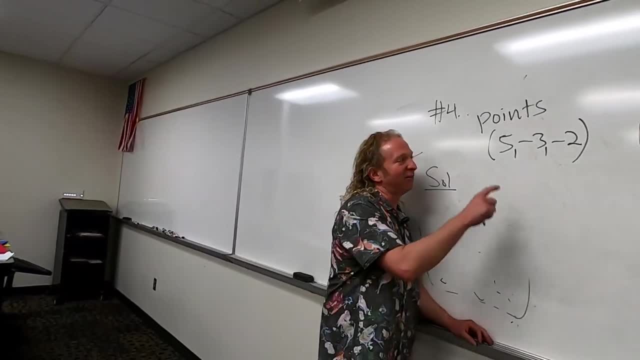 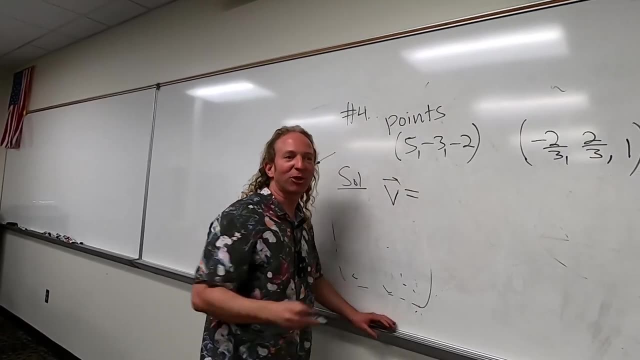 I think you've got to do the Oh right, right, right Right. Actually, if you multiply them both by 3, it'll work. But let me not go there. But you could. So v, Let's do terminal minus initial, I guess. 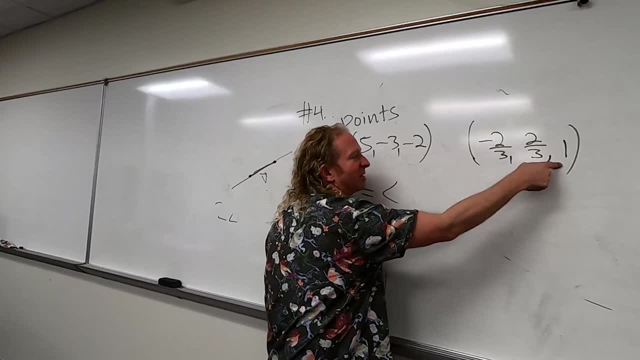 So we'll do this minus this, this, minus this, this minus this. We'll think of this as the terminal point or something You can just pick one. Yeah, you just pick one. I'm just going to pick this one first. 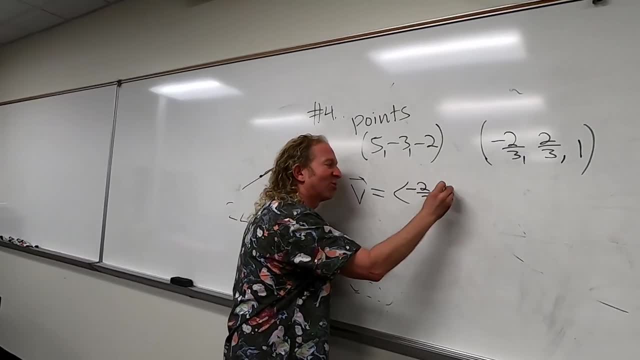 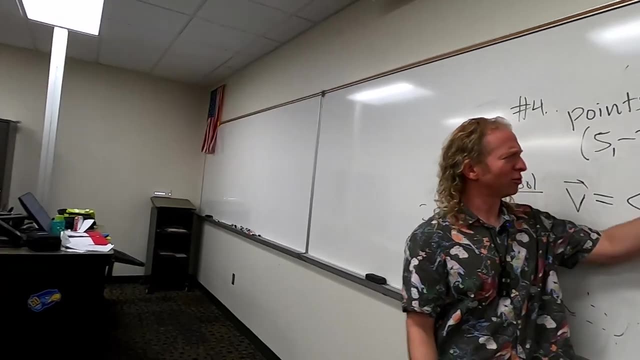 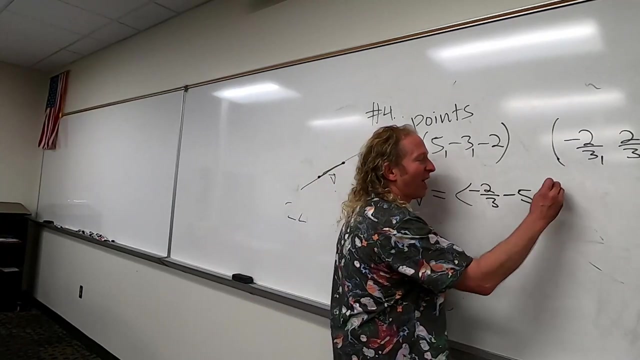 So negative 2 thirds minus 5.. This is horrible. Well, it's not that bad. We got this- It's college Back in the day there were no calculators. So 2 thirds minus this will be 2 thirds plus. 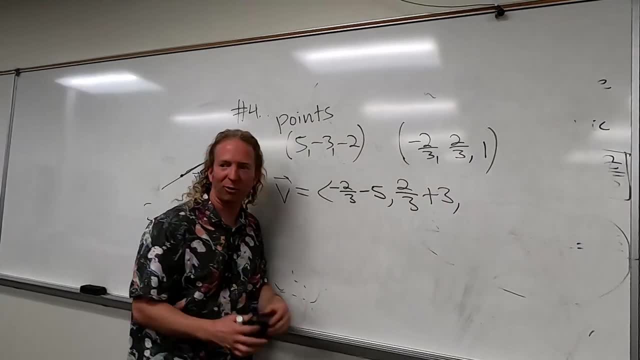 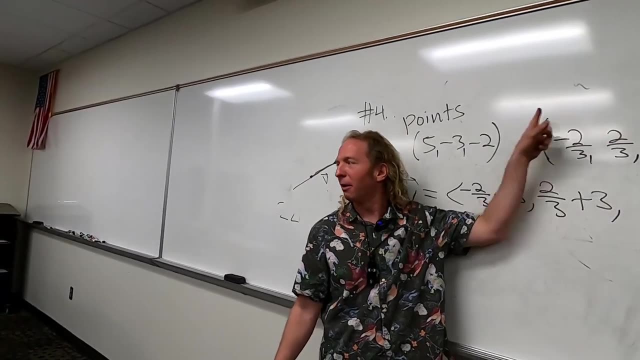 Yeah, I don't know if this is true, but I heard that when calculators first came out they were really expensive, like hundreds of dollars. But I don't know if that's true, I don't know. So 1 plus 2.. 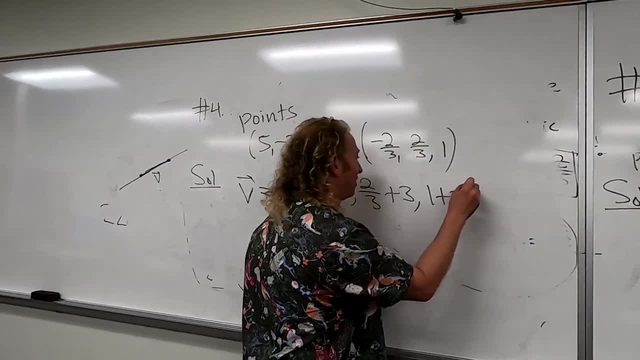 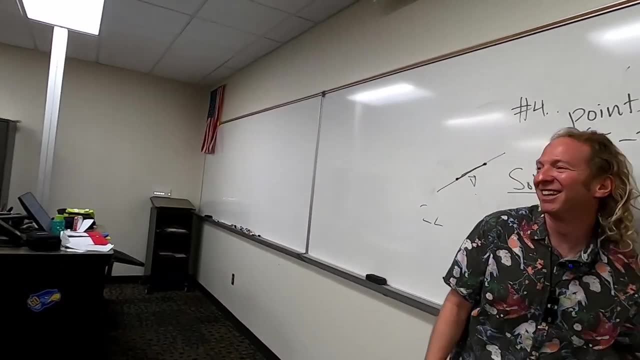 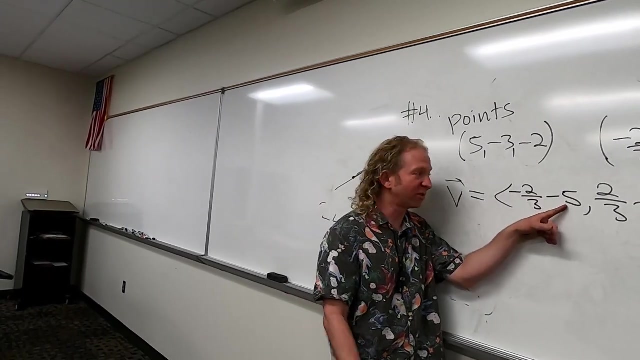 It's the variable, It is. It's the variable. It's the variable. Sarcasm, All right. So we want to think of this as a number over 3.. So 15 thirds, Yeah, 15 thirds. So this will be negative: 2 thirds minus 15 thirds. 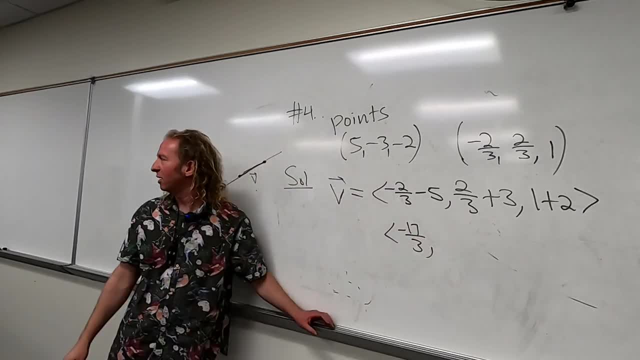 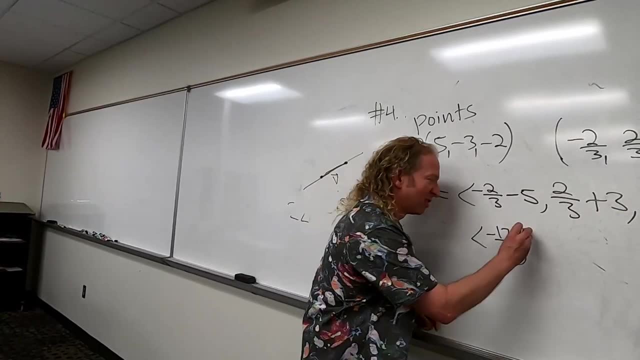 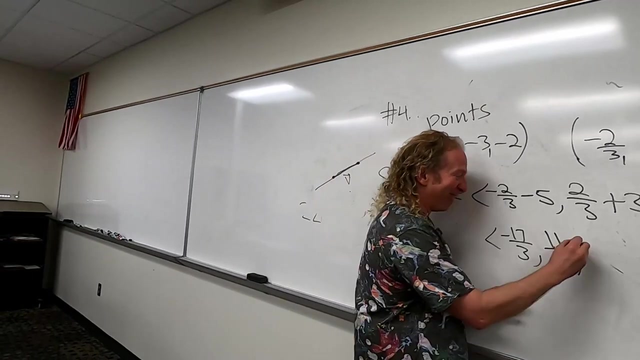 negative: 17 thirds. Yeah, is that right? 2 thirds plus 9 thirds 11.. It's 11 thirds. It's 11 thirds, 1 plus 2.. No, I know I laugh and I'll put 4.. 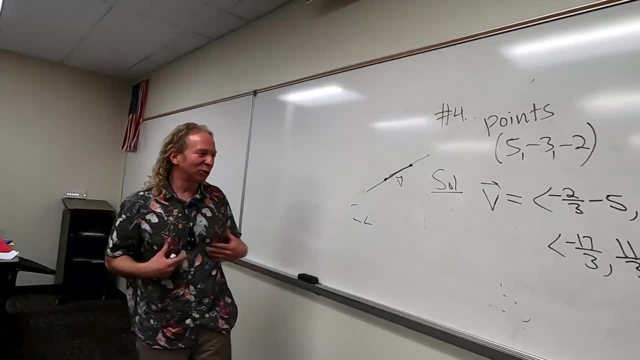 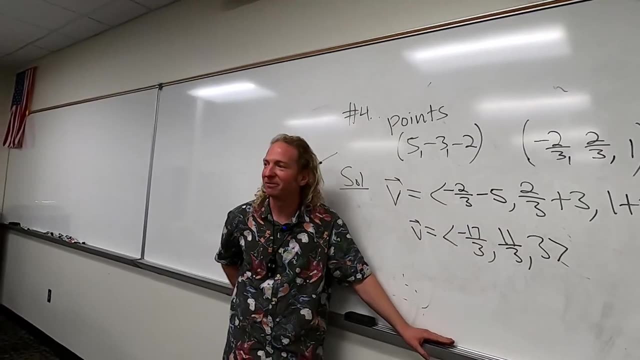 Like that'd be really bad, And I lose a point Like no. I don't know why I say lose. I don't really lose points, But it doesn't affect my life, So I don't know why it bothers me. 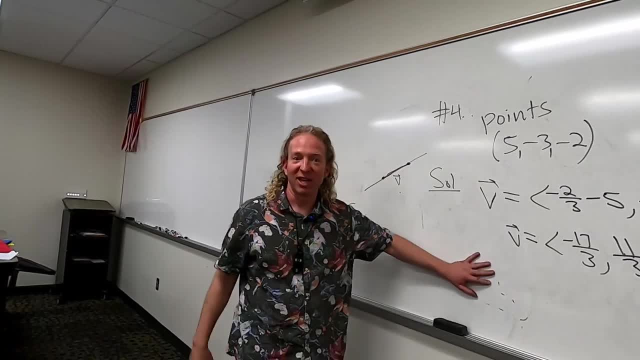 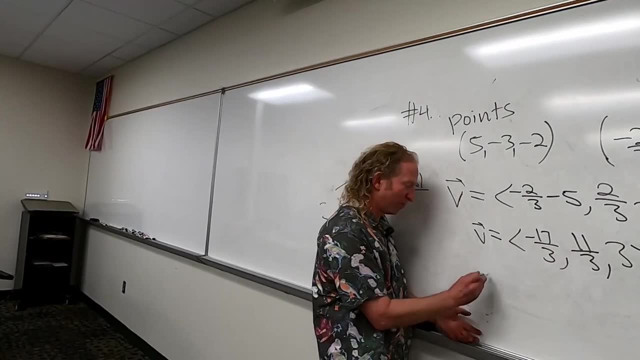 Huh, Now we can multiply it by 3.. Yeah, now let's do the Isaac way. So let's get rid of this. 3. By multiple, By multiplying by 3.. So I'm going to call it u. Why u? 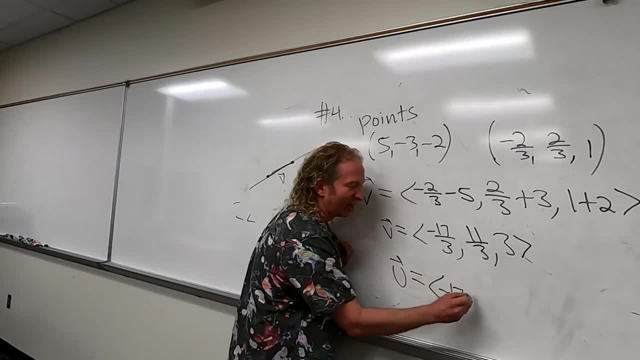 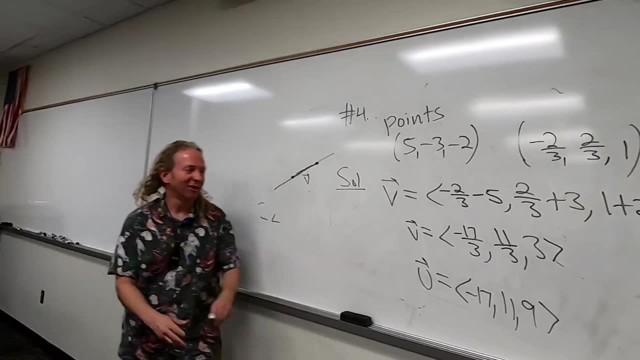 Because I just felt like it Just call it something else. right, So negative, 17,, 11,, 9.. Right, Right, 9.. So boom, boom, boom. Just multiply by 3.. You can do that right. 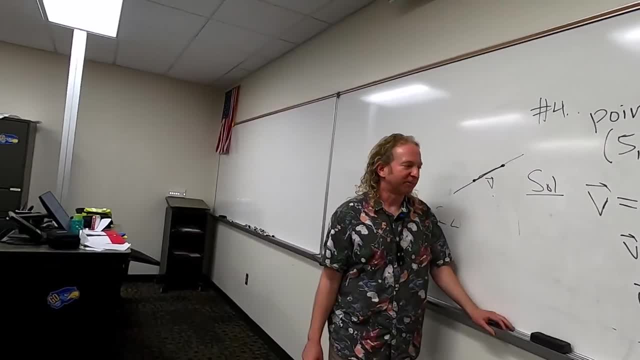 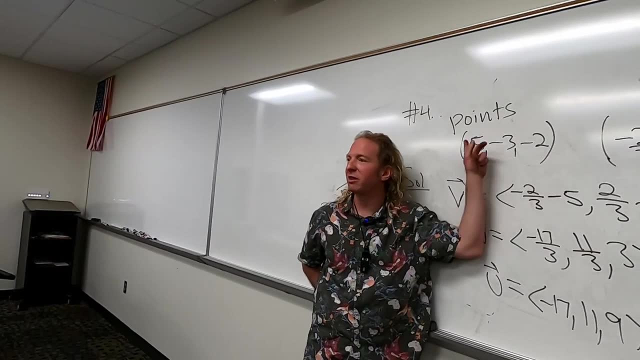 You can do that and it's still parallel, right? So Isaac was talking about multiplying this by 3.. I guess you could have done that, but you would have had to multiply this by 3 and this by 3.. Yeah, 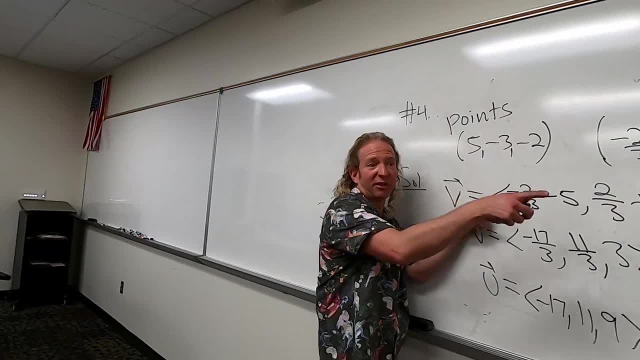 That's really clever. I just didn't want to do that because it's a little bit too clever. But we could have done that right. Because, look, if I multiply this by 3 and this by 3, what happens is you end up with a 3 here and a 3 here. 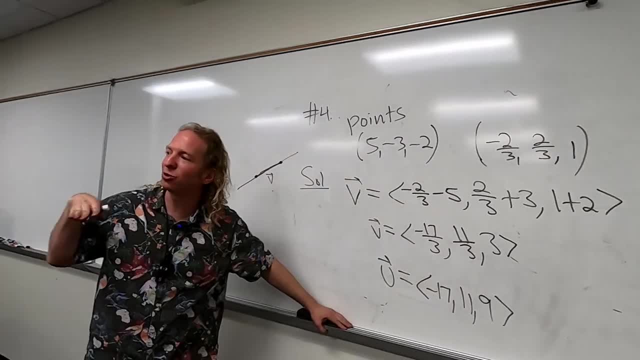 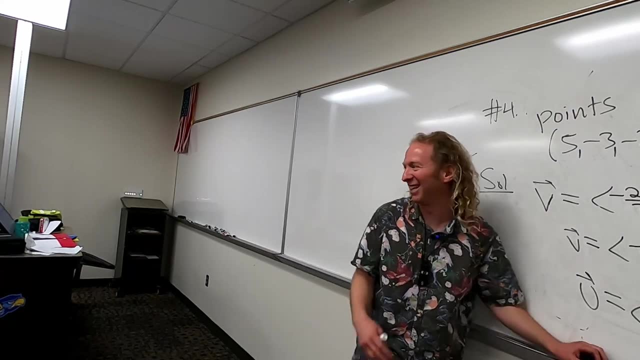 You essentially end up factoring out a 3. So you could have done that, but I just thought that was too slick of a move to do. So it worked. It was just too good, So I had to Yeah, So it was just too intelligent. 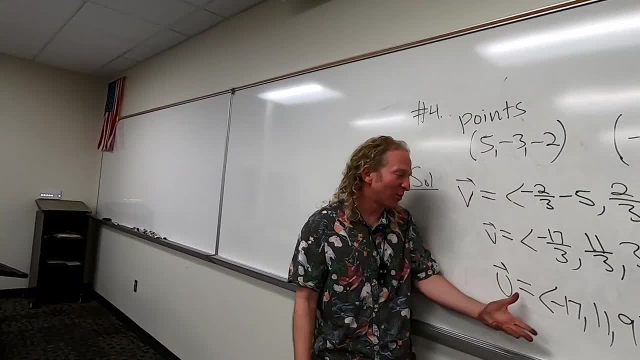 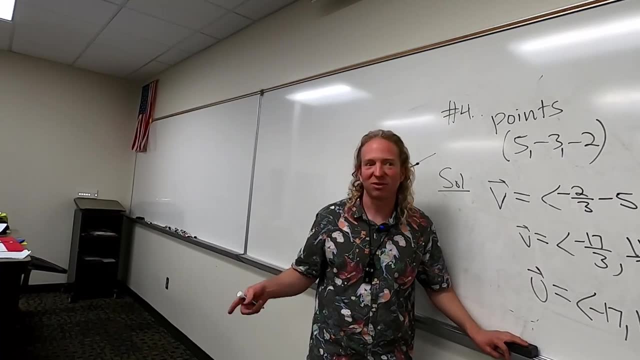 No, it's good. No, it's good, But you could do that right. Anyways, it wasn't so bad. So now we have to find the line, So we get to pick a point to use. So obviously we should use this one. 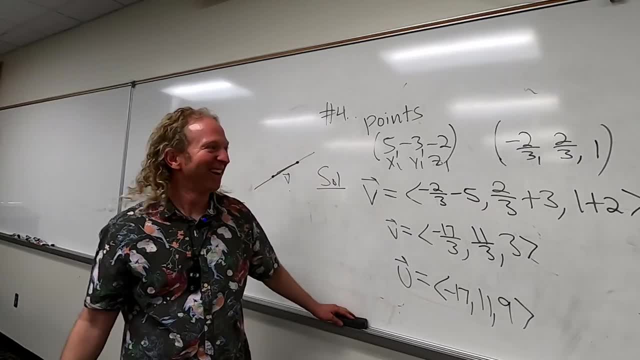 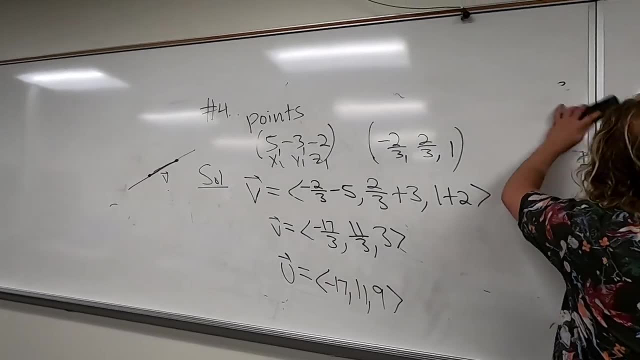 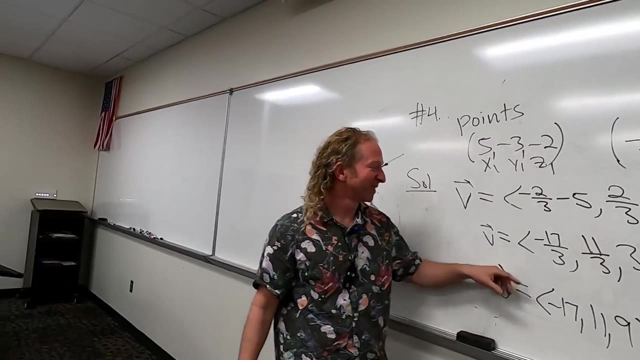 Yeah, The fraction. Yeah, yeah, You can't do that. Yeah, Torture. Yeah, Multiply it by 17 thirds. No, OK, So Put it on the test, see how long you get it. Yeah, So x is going to be. oh, so this is our. what are these? 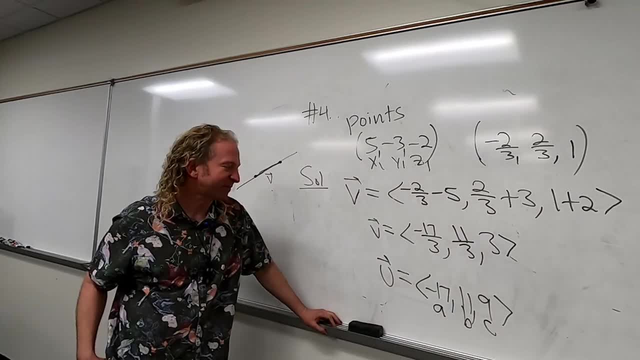 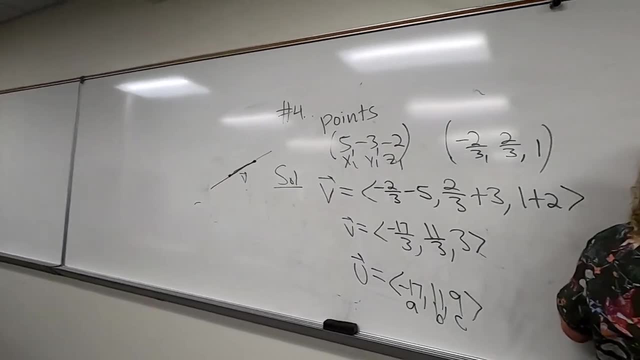 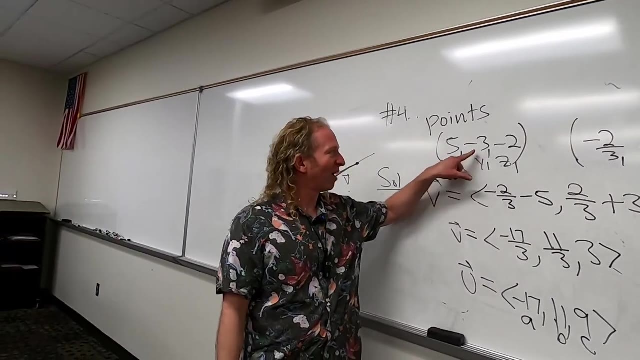 What letters are these? ABC, ABC. So it'll be 5, right, 5 minus 17t. That's the first one. That's x, Hey, Kenny, Yeah, y is negative, 3 plus 11t. 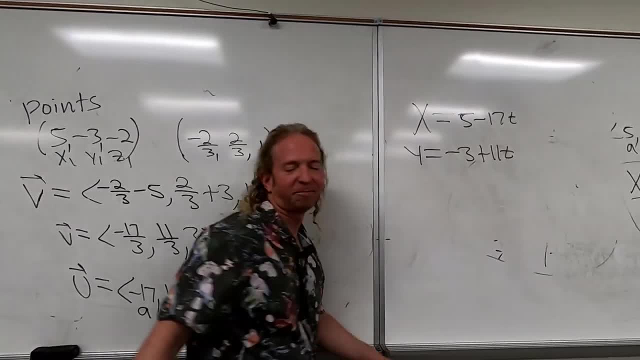 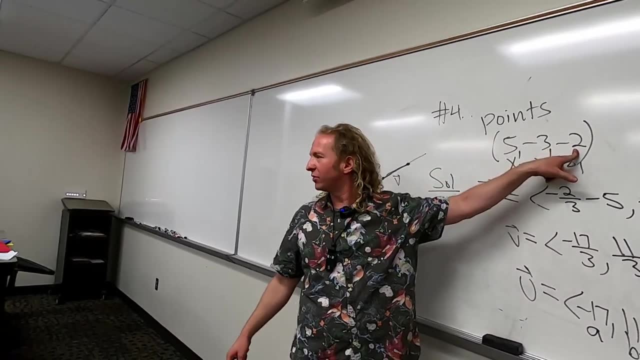 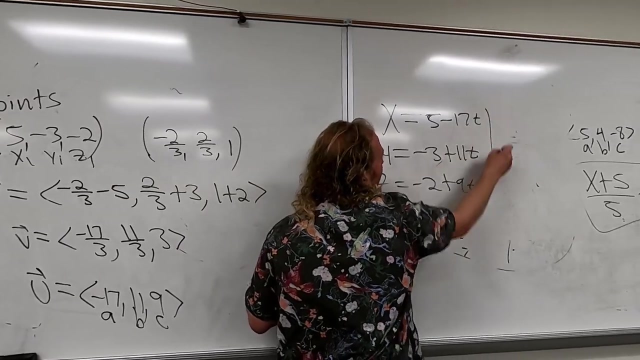 So negative 3 plus 11t. And the last one would be negative 2 plus 90, right, So z would be negative 2 plus 90.. And these are the parametric equations. Does that look right to you all? 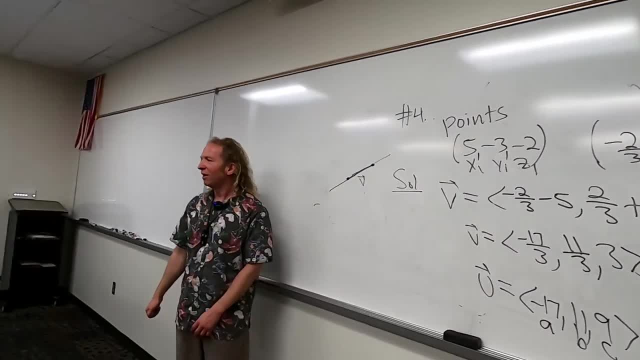 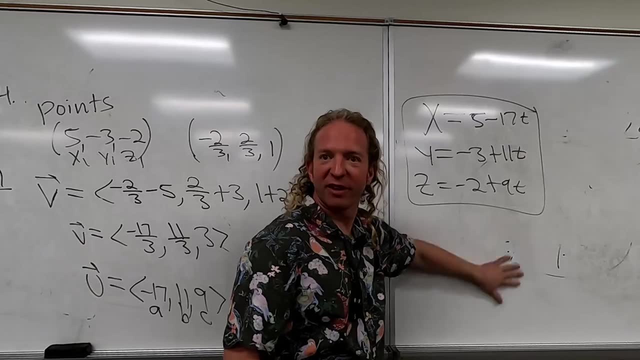 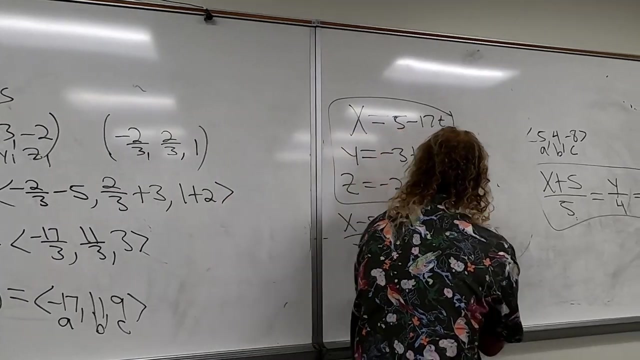 Does that look correct? Yeah, OK, And then we have to find the symmetric right. So the symmetric, you just subtract and divide, right, So it'd be x minus 5, x minus 5 over negative 17. And then y plus 3 over 11.. 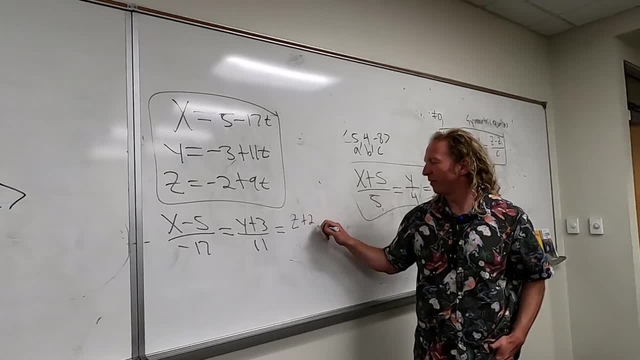 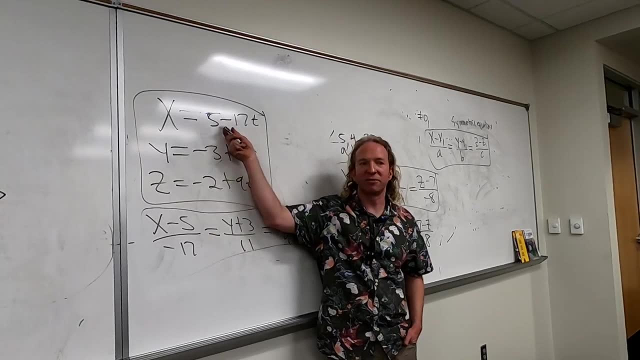 Going fast Because I think you got it And this is z plus 2 over 9, z plus 2 over 9, z plus 2 over 9.. So they're pretty fast. So it's just x minus 5 over negative 17,. y plus 3 over 11,. 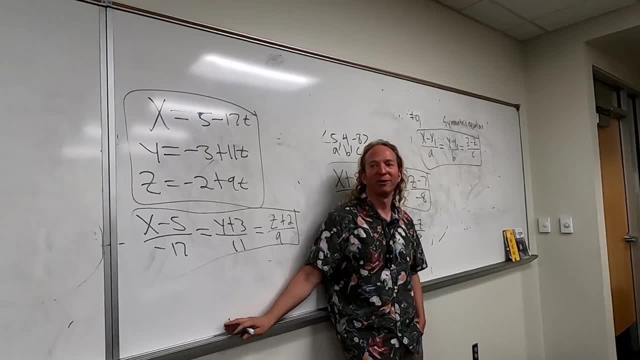 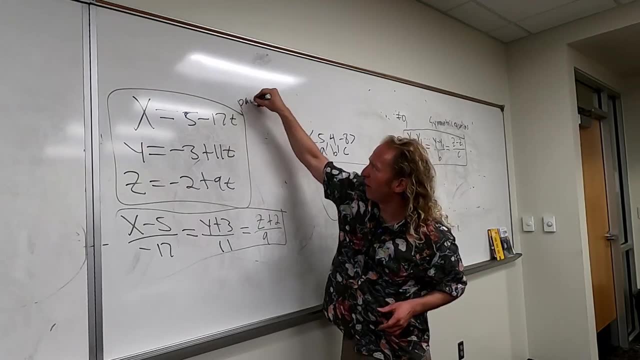 z plus 2 over over over 9, over 9.. So these are, what are these called? again, Do you remember Parametric? I'll just put para parametric. And what are these called? Symmetric? 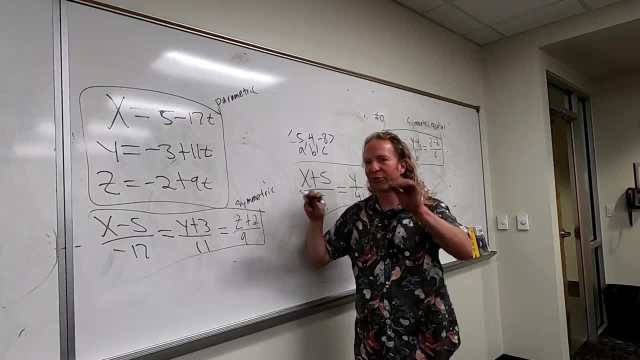 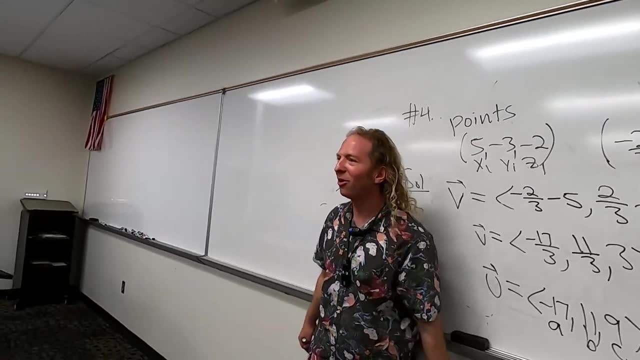 Yeah, symmetric. So this model is a path right in space that's traveling on a line right. So a key: hey, hello, are you in this class? Oh, OK, We just finished everything, but it's OK. 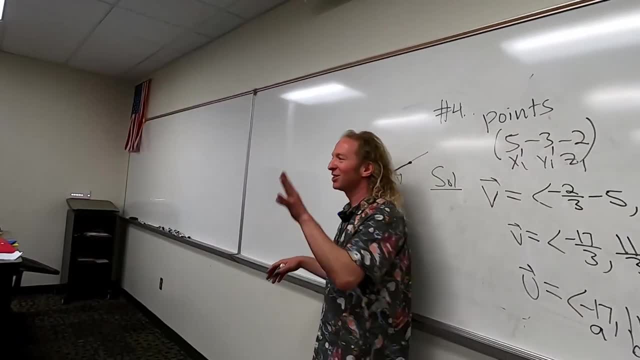 It's OK. No, it's all right. It's OK, You're good, Because we're going to do a worksheet and then I'll help you And you'll figure it out. It's like two formulas, right? No three, three. 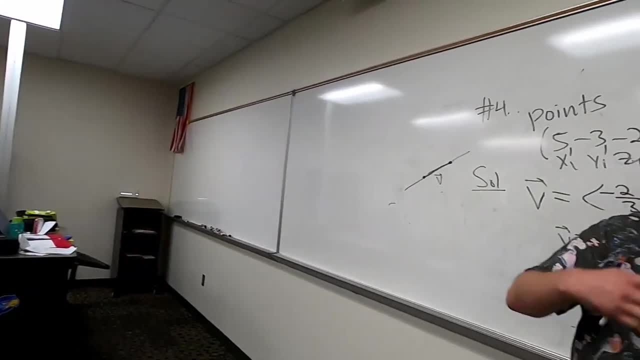 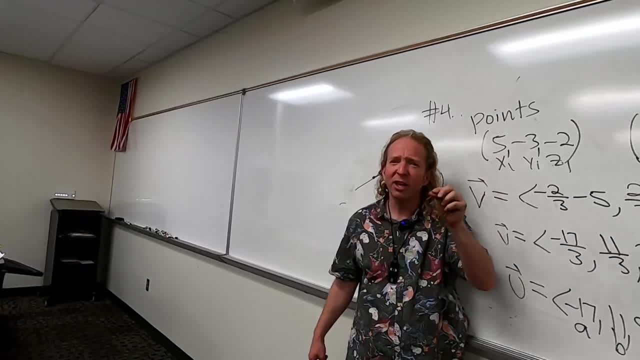 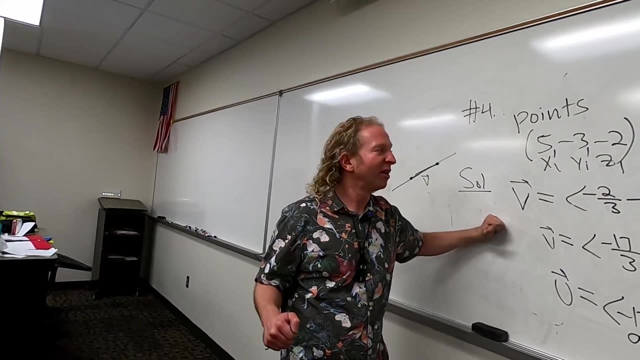 All right. So the original question is the hardest one we've done today. So we're given two points on a line. We have to find the equation of the line. So we need two things: We need a point and we need a parallel vector, right? 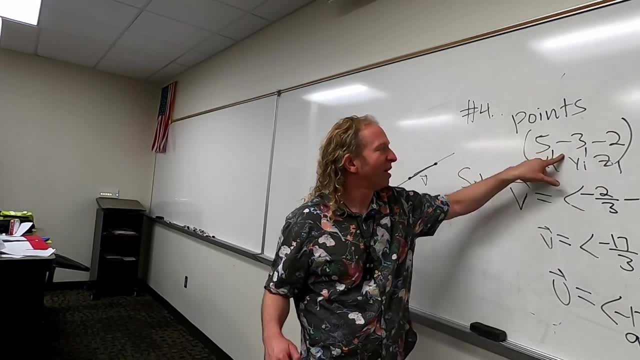 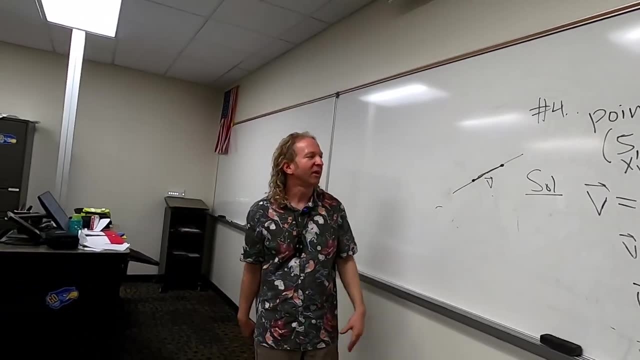 So the idea is we can use this as our point. If we have two points on the line, we can subtract them to find a vector that is on the line. Therefore, it is a parallel vector, right? So this is our ABC. 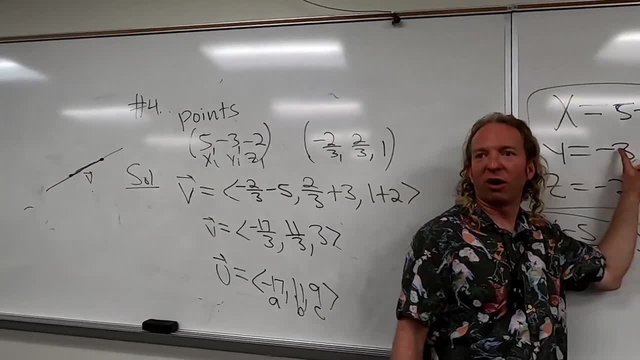 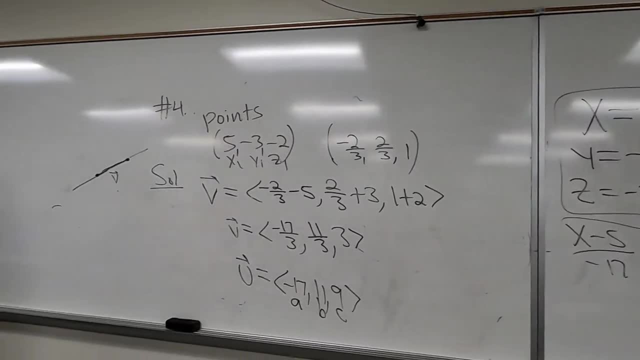 And then you just use the formula right: A plus BT, Y1 plus- sorry, X1 plus AT, Y1 plus AB. A plus BT, Z1 plus plus CT plus CT. Any questions on this stuff? Any questions on this stuff. 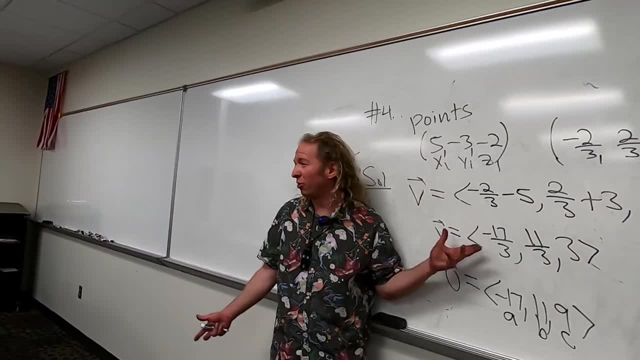 Any questions on this stuff? There was one more like this in the homework. Do you all want to try it? Do you want to do it? Yes, Okay, So I'll write it and then you try it, then I'll do it. 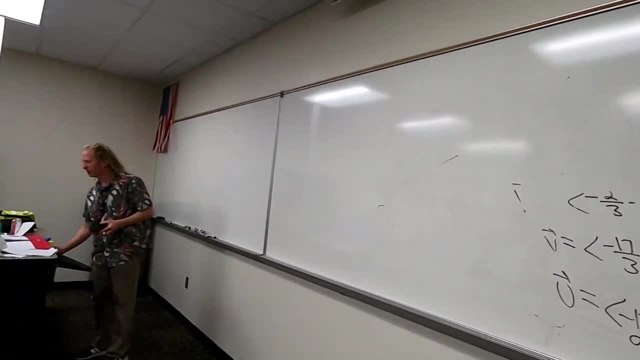 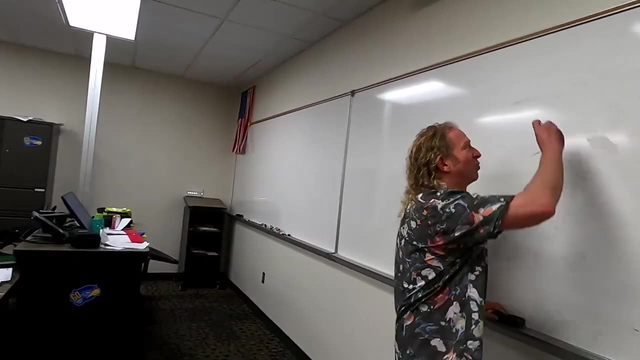 So it's number. I think it's number five. There's only six problems on this. Six is really easy, So five, This one's really easy. I didn't want to do this one because it was so easy, But let me just stop talking and do it. 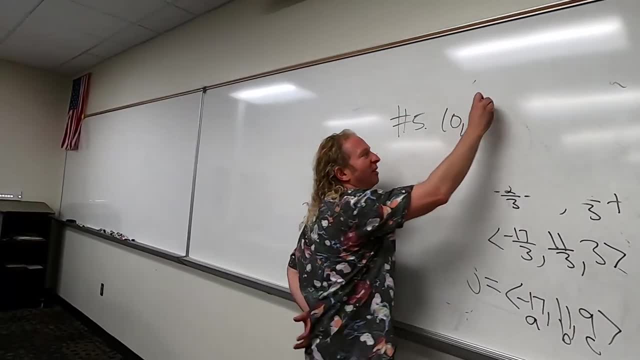 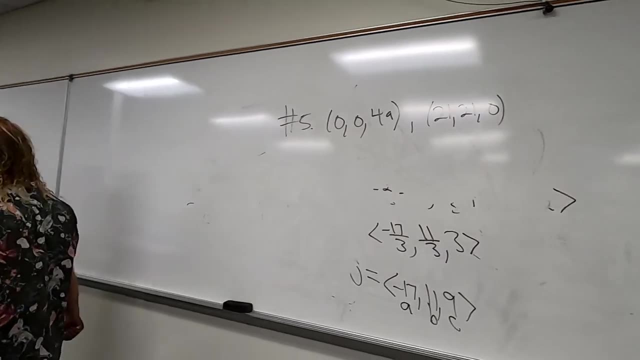 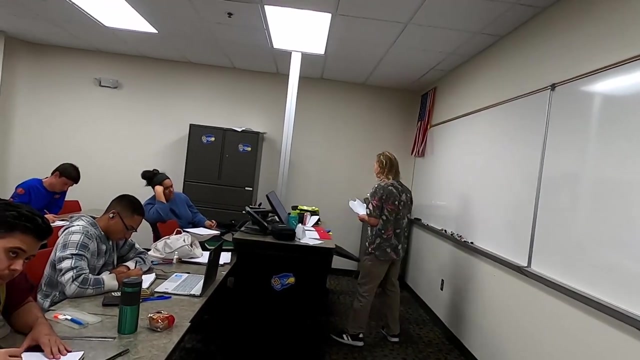 Maybe, maybe it's hard, All right, so 0049.. So try to do it. Find the. these are points on the line. Try to find the parametric and symmetric equations of the line. Okay, Here's my notes, if you want the formulas. 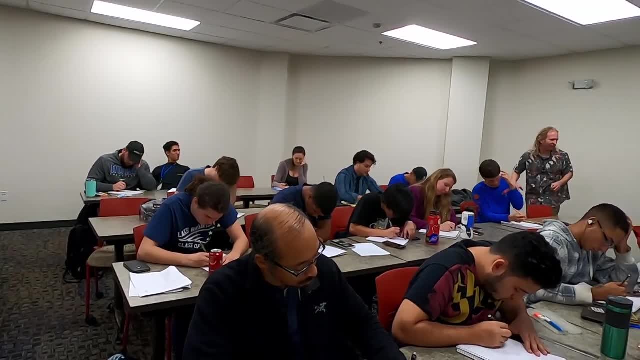 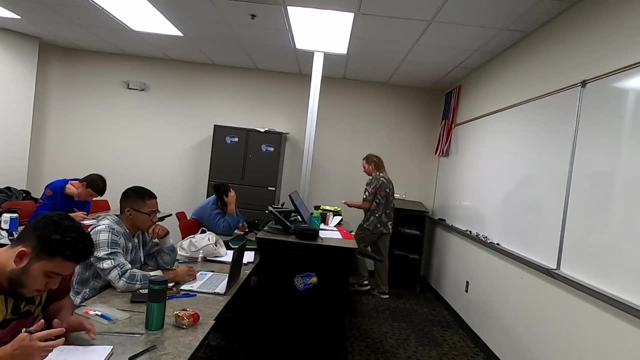 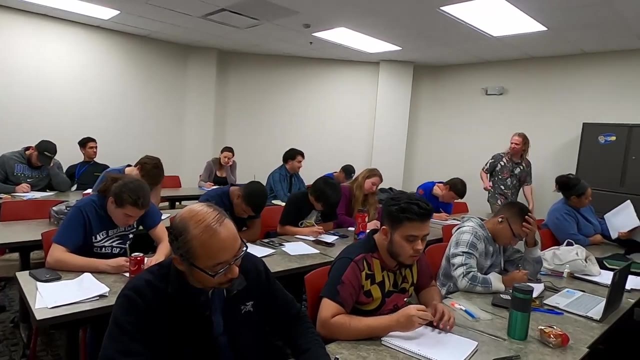 Just those things in boxes, okay, Boom, boom, Yeah, And then also this, And you'll be able to catch up during the worksheet time. Yeah, It's better to come. better late than never, right? Yeah, totally worth it. 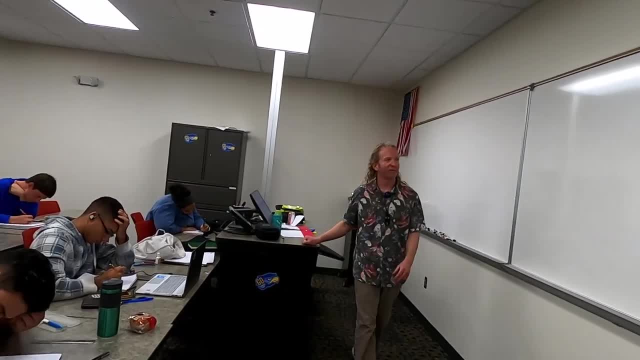 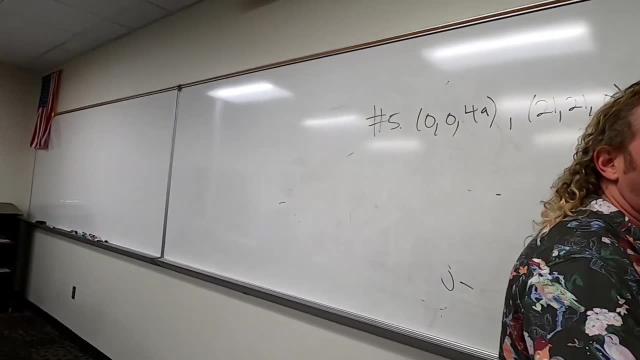 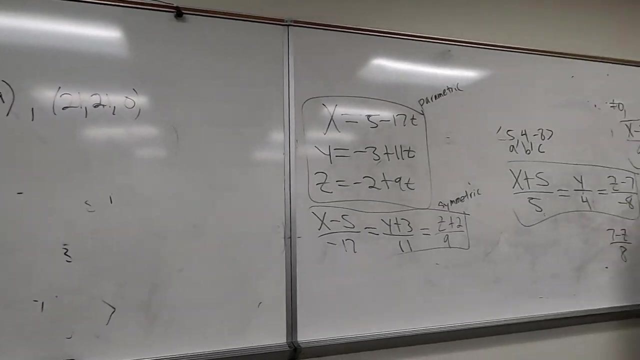 Yeah, That's not hard. like, yeah, You got it already, Kenny, No, I'm kidding, I'm giving you a hard time. I know you're not even- not even in the class. I don't know if I'm even gonna reach there. 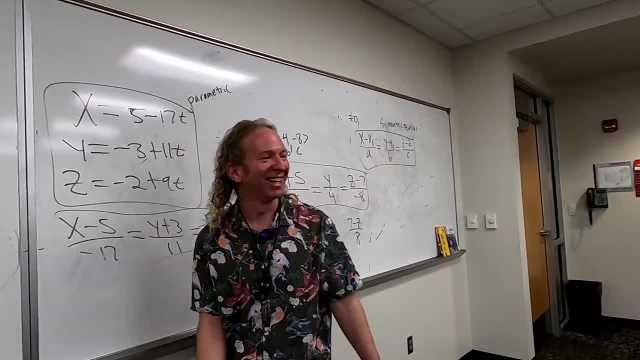 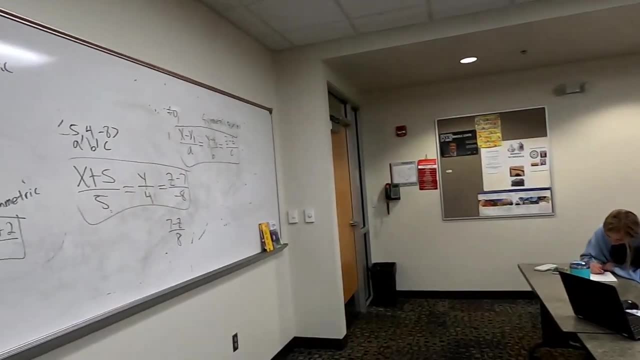 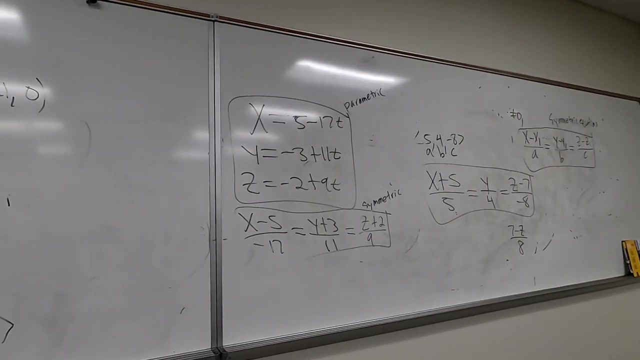 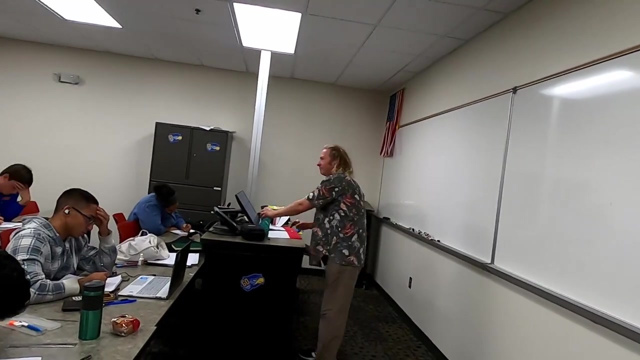 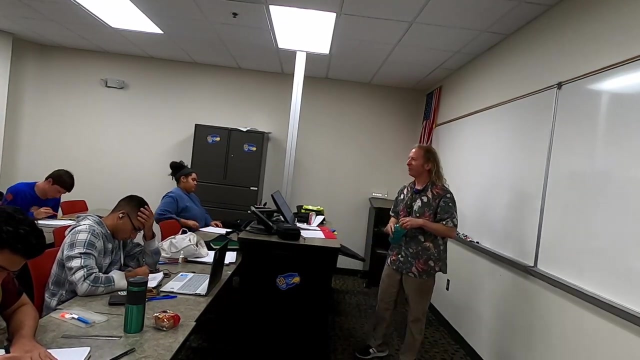 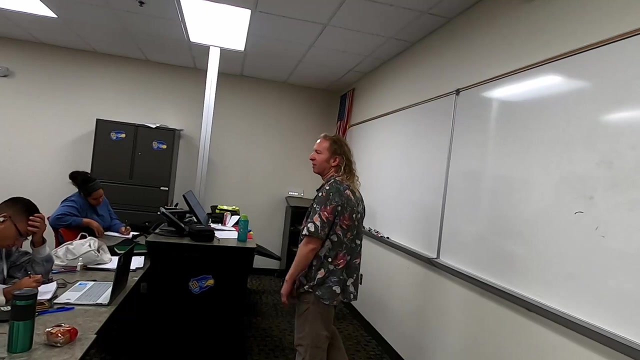 so are you going to be Isaac? are you going to be tutoring before class also sometimes, or no? maybe like before class also, maybe, 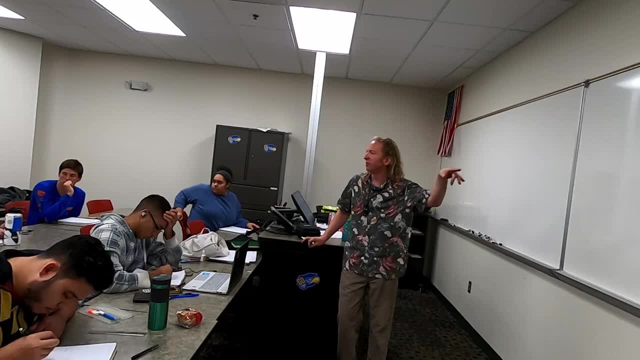 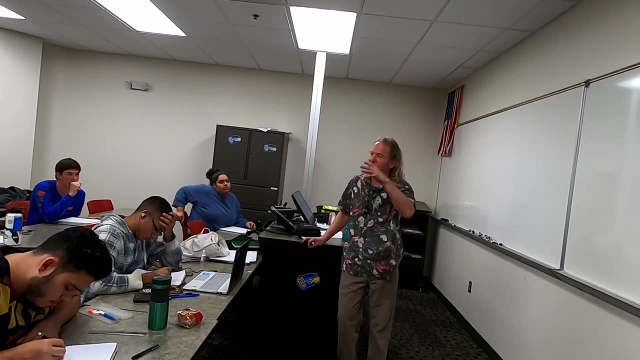 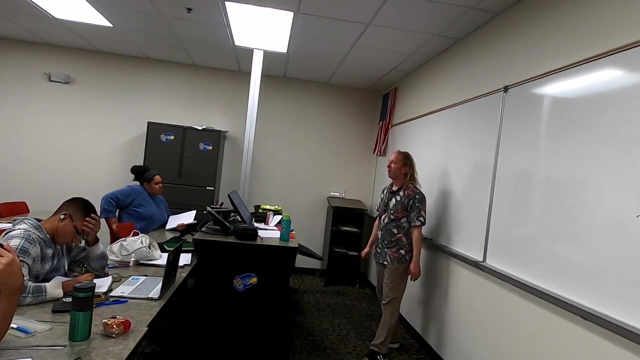 yeah, maybe on the tutoring center. cool, I had another idea. I was just I'm just thinking, I'm just talking here, but I was thinking like, if you do hold like tutoring sessions in here before class- I'm just just talking on Wednesday, but if you did it, 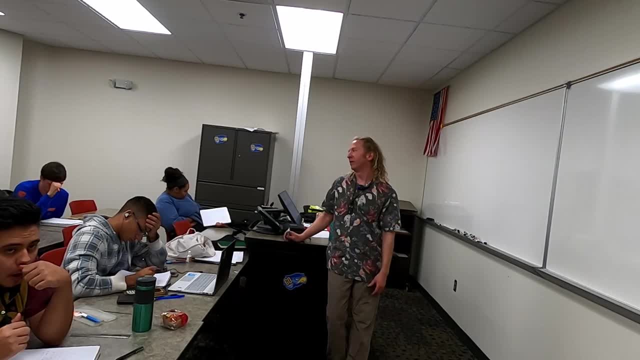 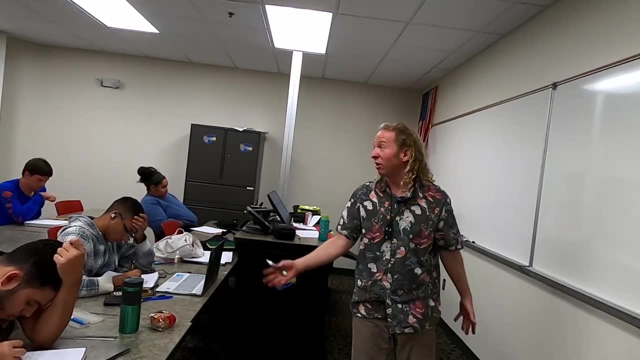 Monday though. yeah, and you have pizza parties. yeah, I was just thinking, yeah, you heard what I said. you had like a pizza party like in the future, maybe like before, not now, but like you know you could right. yeah, I'm just you know, but you have to. 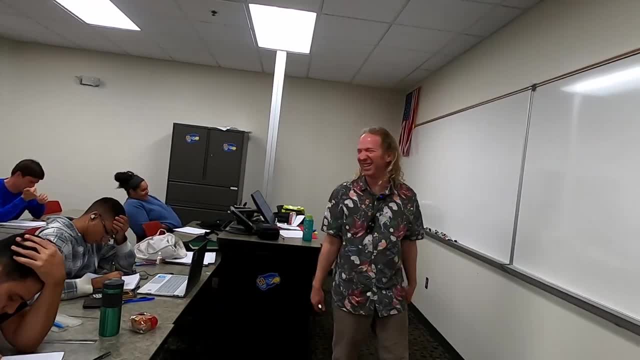 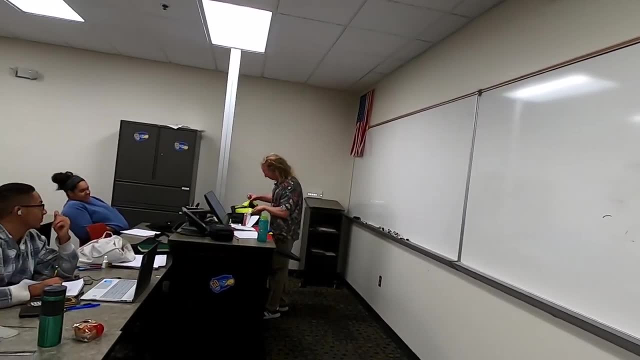 you know. so it's, it's food starving? no, I have. I have some apples, but I don't. I'm good, I just have to wash them and I'm not. I'm good. I ate like four sandwiches. I had two peanut butter and jellies and two ham and cheeses. 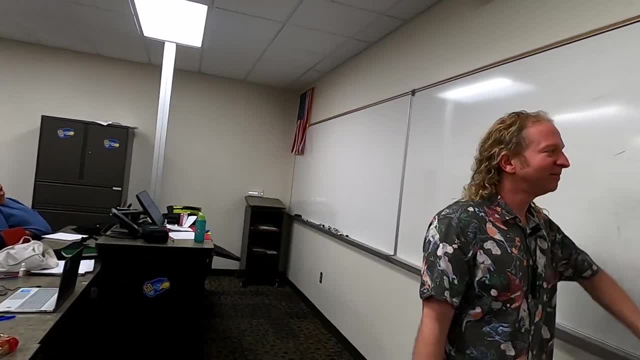 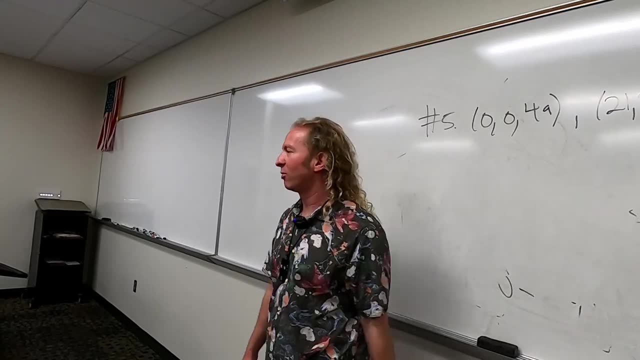 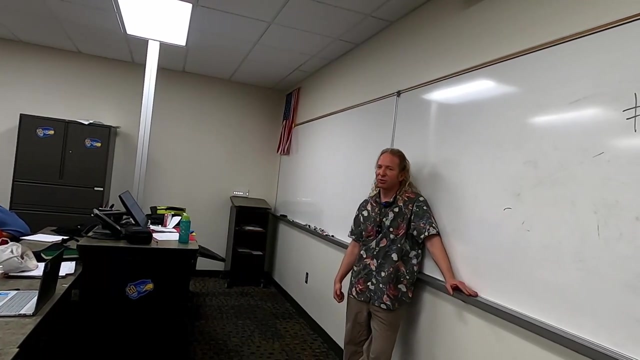 so I'm like sandwiched out for the day. I had eggs for breakfast. yeah, I had a summer where I actually had like a lunch break and so I would go to Publix every day and get a sub. it was an interesting summer. I met some interesting people. 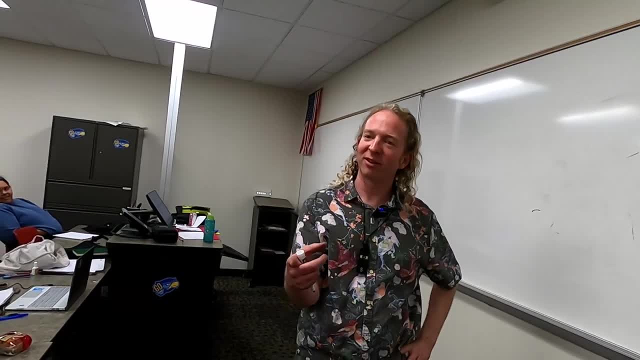 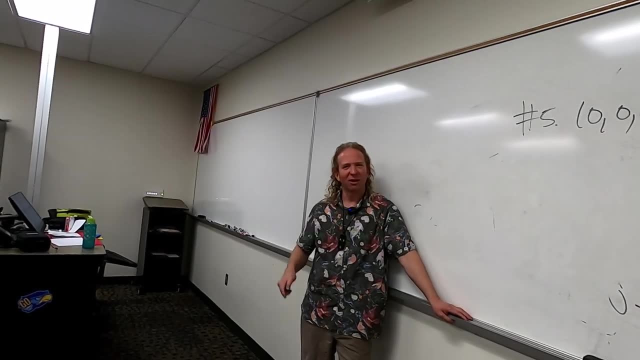 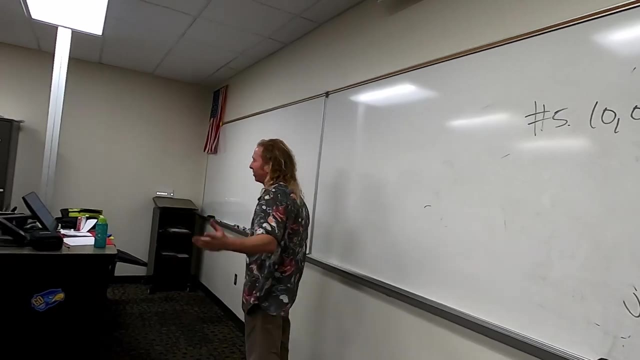 we didn't you go, did I? weren't you in my class that summer? we went to Publix together. oh, I was. what was that? it wasn't in the summer. it wasn't that summer where I had that break. okay, okay, okay, because I remember we went to Publix. 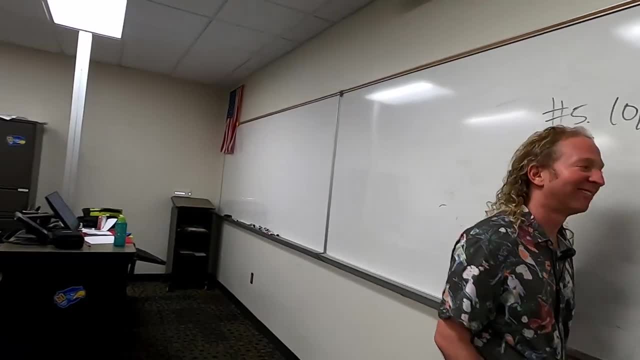 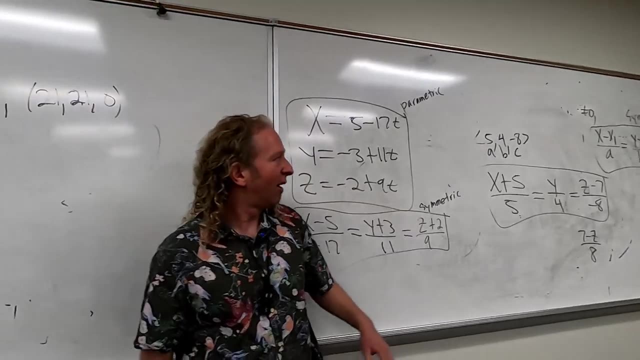 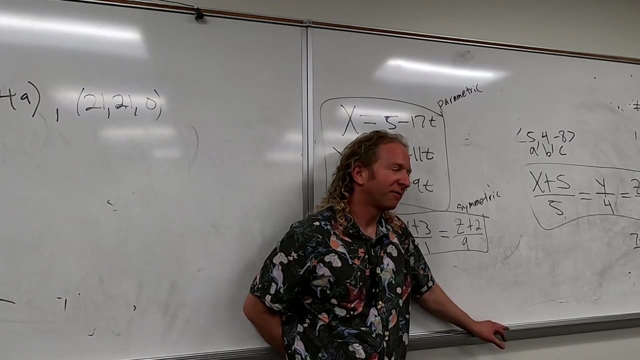 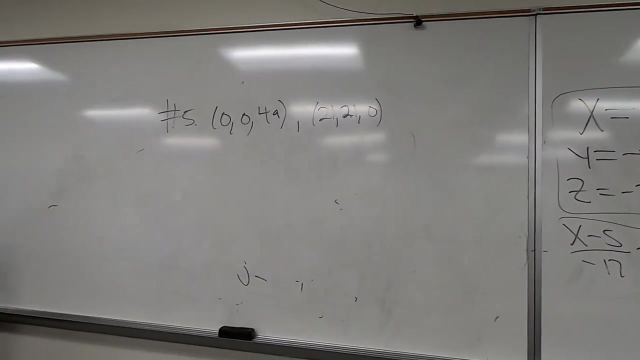 but yeah, yeah, Pub subs. yeah, it's a weird name, I guess. so I mean, I think so. I think that's why that's a good question. I think it's why, yeah, there's other symmetric stuff in math too, like there's like symmetric polynomials, like it's a thing. 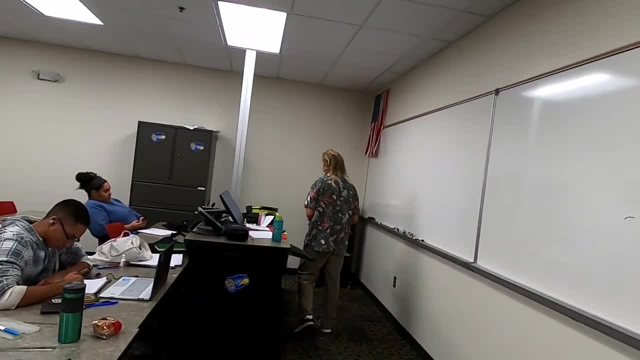 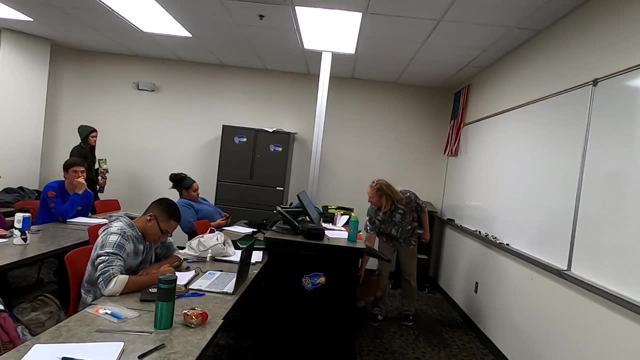 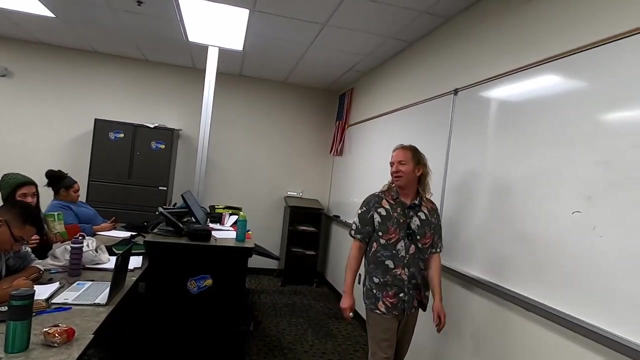 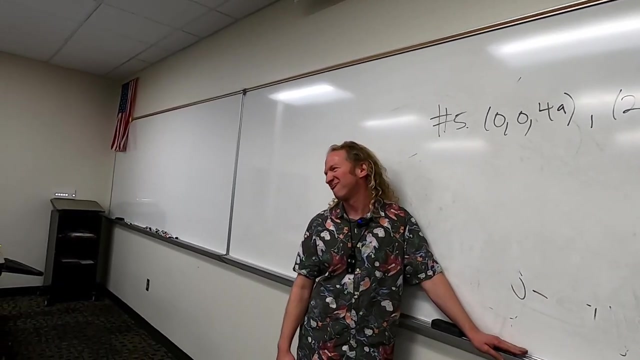 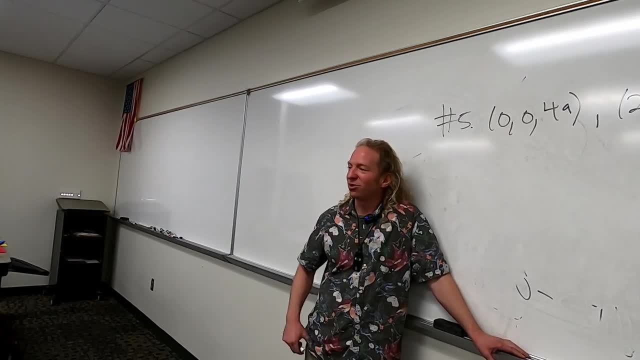 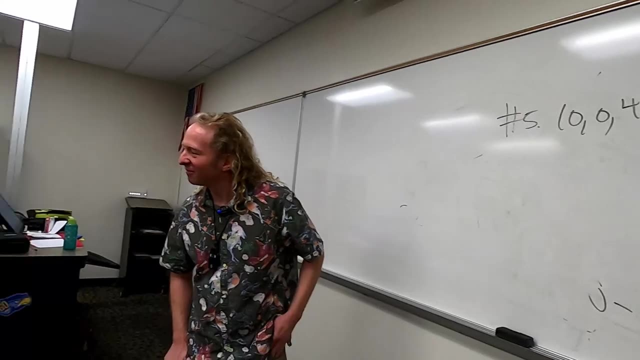 that's a cool shirt, thank you. I don't know what it says, but it looks really scary. it says ghost, oh, ghost, okay, yeah, it's a. it's a Swedish metal one. oh, you listen to metal? yeah, I used to listen to like Metallica and stuff. 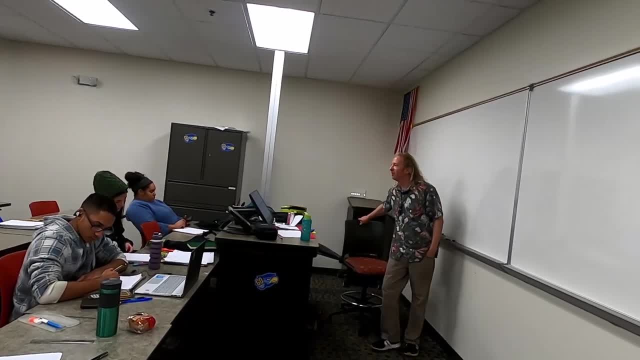 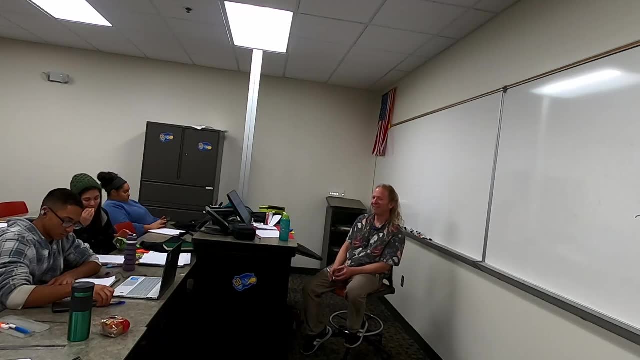 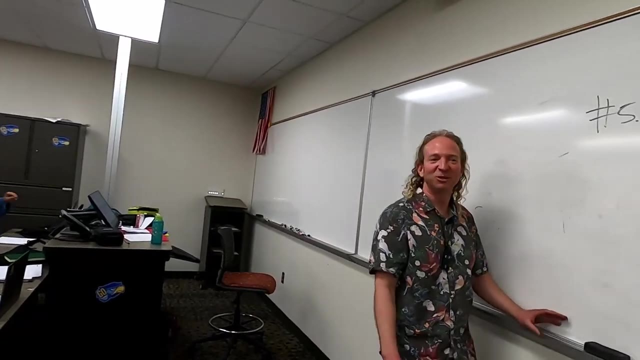 I play but I'm not very good. so you know, ghost, is there one now? you went to the one last year. you missed it. yeah, yeah, you went to the one in 2015. yeah, no, I said it was in. like I said, thank you, I know. 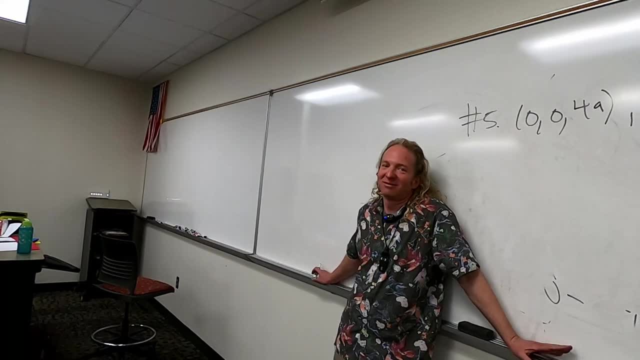 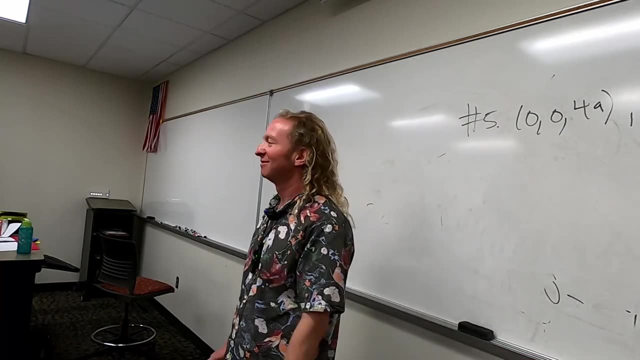 they're not going to be on tour this year or they're stopping- like they're going to stop the 20 questions. hey, we got a good two guys. yeah, did you get it, Roger? I should go ahead and do it. alright, let's do it. let's do it. 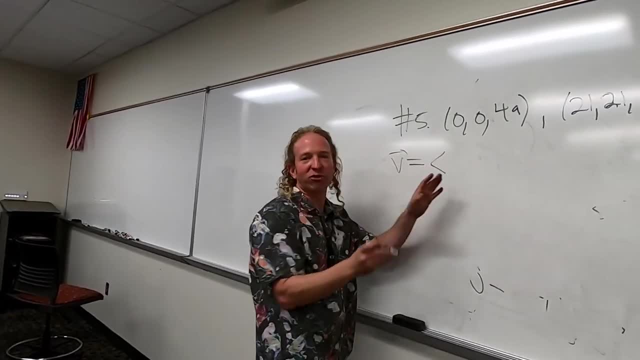 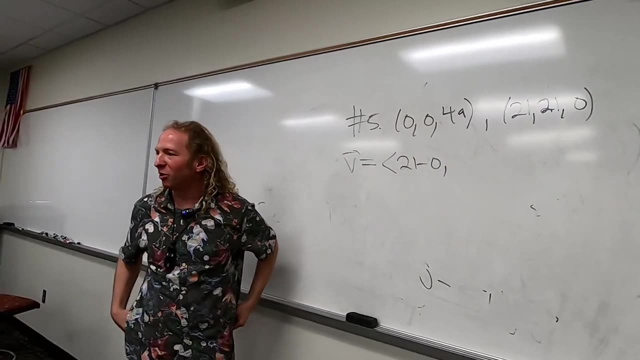 so V. so for V, you just subtract. I'm going to do this minus this. okay, so 21 minus 0. I'm going to write it as ridiculous as it seems. why not? right got to make it count. I'm going to see. if it's, I'm going to see it. 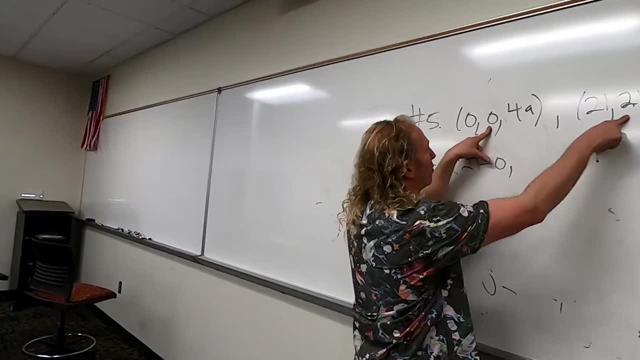 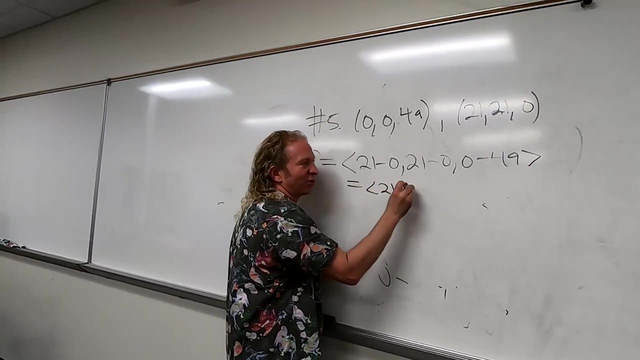 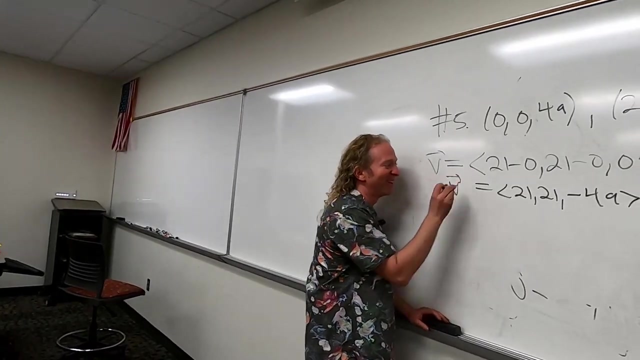 once a week. so 21 minus 0, boom. and then 21 minus 0, 0 minus 49, so that's going to be 21, 21. negative 49, negative 49. yeah, sorry, so V. so that's our V, that's our ABC. 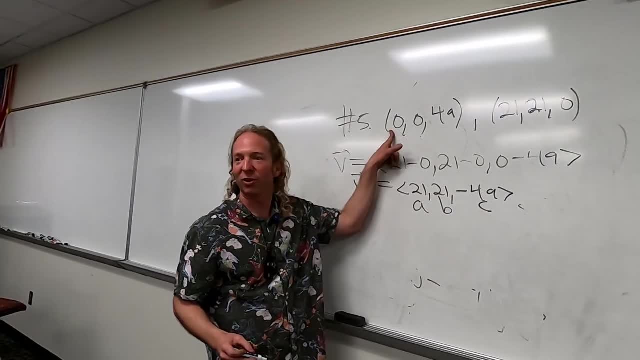 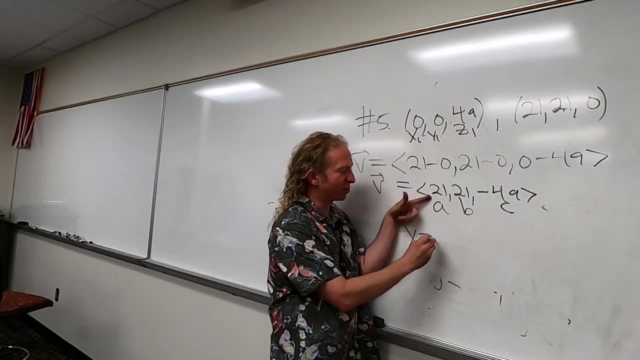 ABC, and then I'll just use this one. okay, so it'll be X1, Y1, Z1, so it'll be X1, so 0 plus 29, 21T, so 21T. Y equals Y1, so 0 plus 21B, so 21. 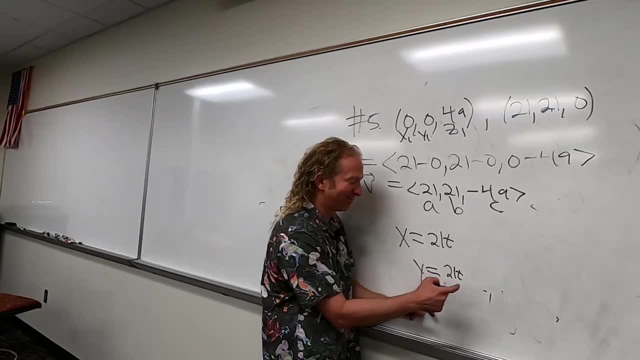 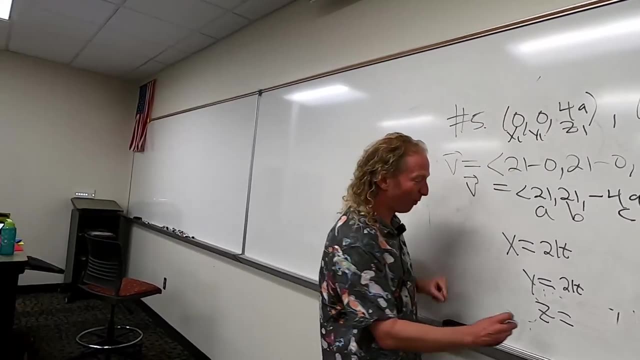 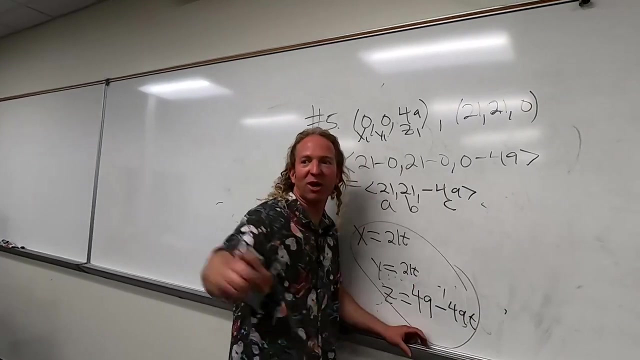 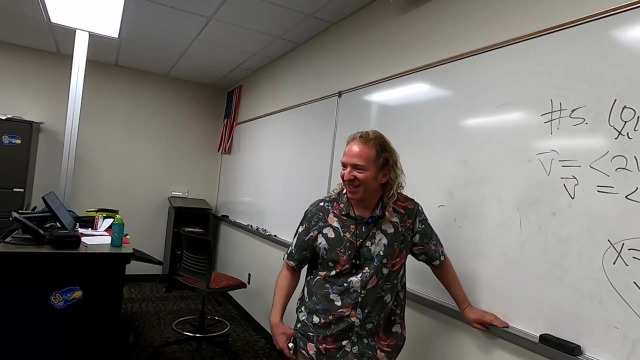 so 21T. so 21T Z is 49, 49 minus 49T. who got this right? I'm just curious. oh, you're ready for the test. it's so good. it's so good, huh, I got that. but what is a parametric line? 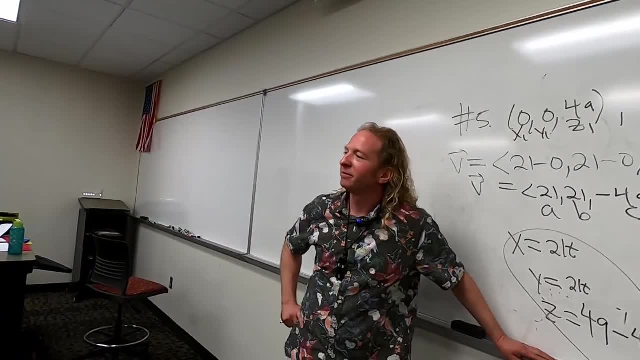 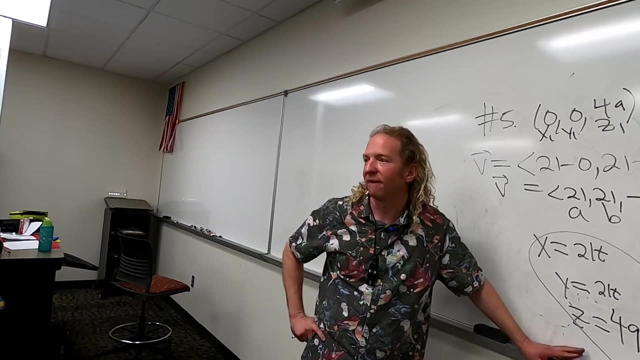 what do we say? I'll show you when we're done. I'll go over it. yeah, if you do it the opposite way and like switch the terminal and the initial, do you just get the same deal? just flip the signs? I think so. I think so, yeah. 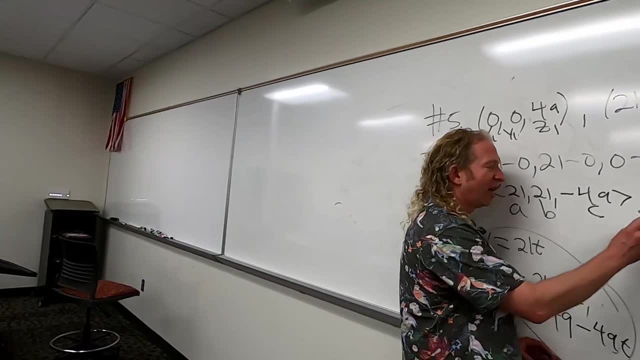 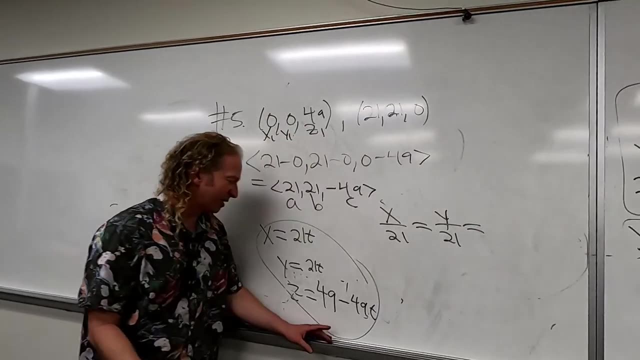 and then we can solve: solve here, so we get X over 21, let's solve for T, Y over 21. and then here we get Z minus 49 over negative 49. so Z minus 49. right, yeah, we get the same thing. but if you switch, 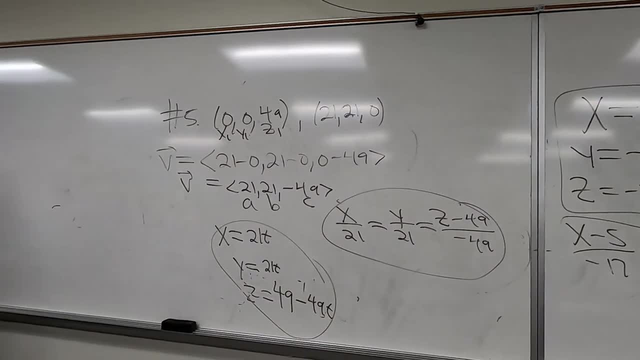 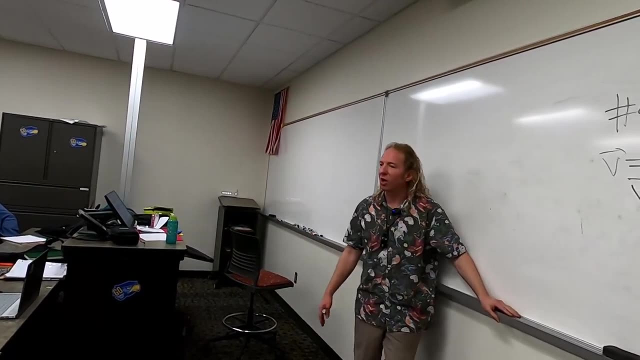 the terminal, it's going to lead to the opposite direction. yeah, yeah, also, if you use a different point, it looks completely different, but that's okay. there's infinitely many parametric equations, so Roger had a good question. this is something that someone else asked also, so let me just go over it again. 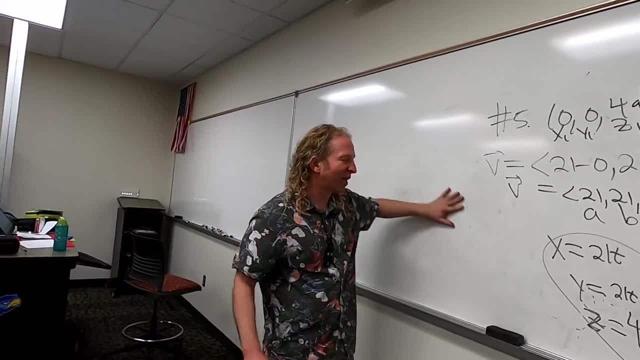 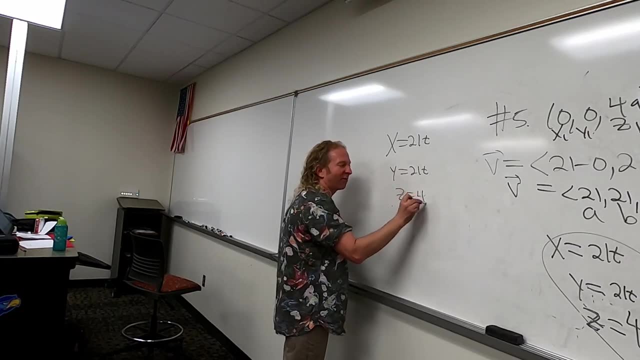 it's worth it. so what are these parametric equations? so like we have? we have this: it's hard to visualize it in this case because it's hard to graph it, but I'll give you another example. so like, when T is 0, we're going to have 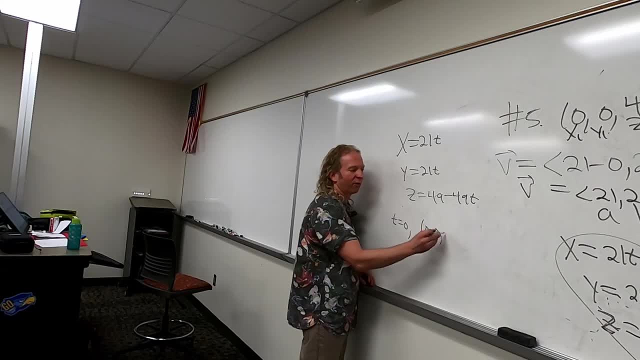 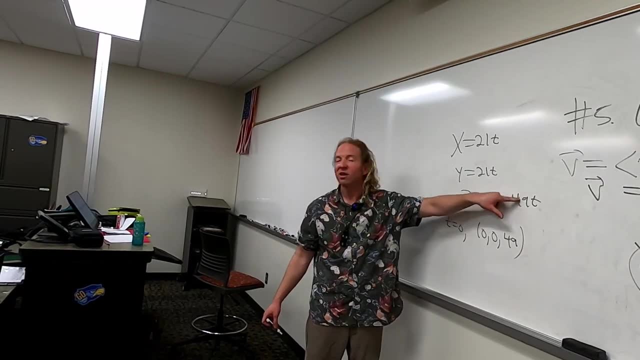 we're at 0, 0, 49, right. when T is 0, because you get 0, 0, 49, right. see how that works. so because these go away, when you plug in 0, you get 0, 0, 49. 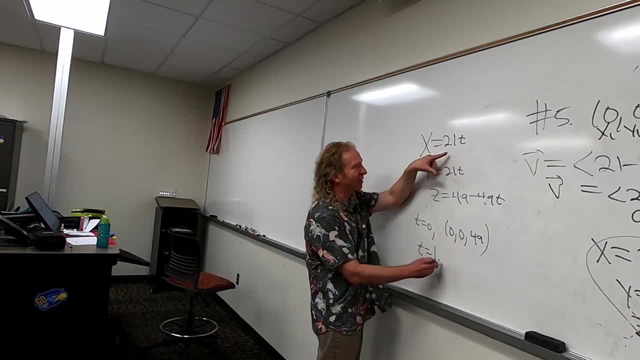 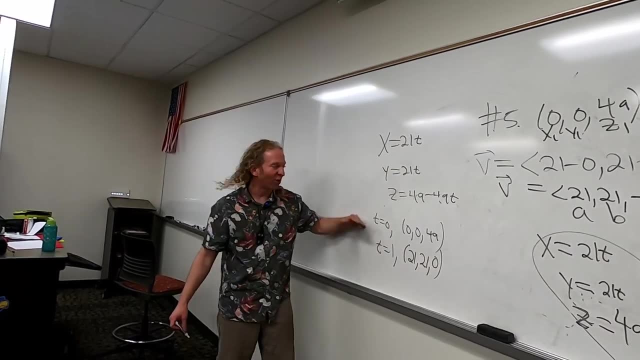 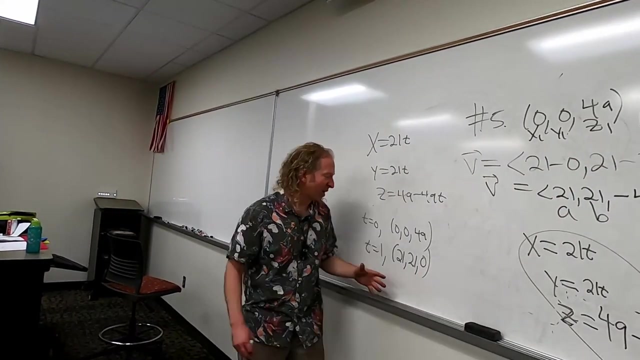 so like: then, if you do like, T equals 1, you're at 21,, 21, 0, oh, that's cool. so when T is 0, you're at this point. when T is 1, you're at this point, right. so then, when you're at, 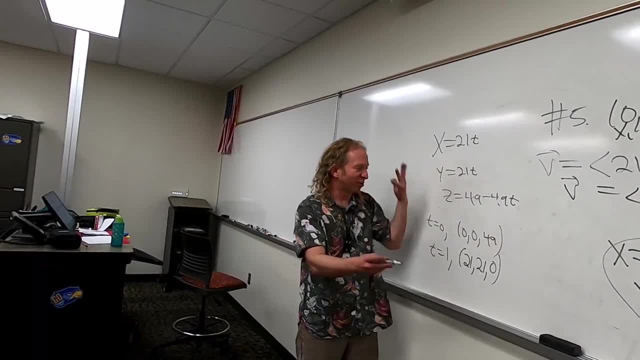 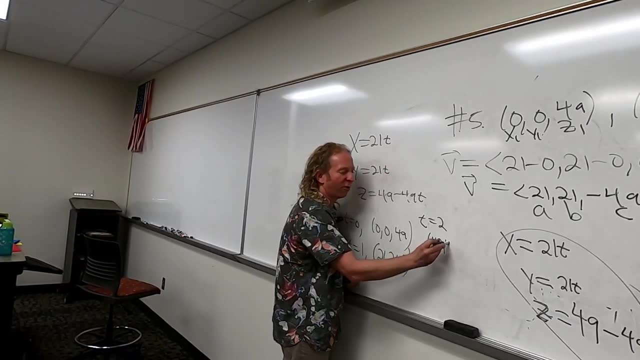 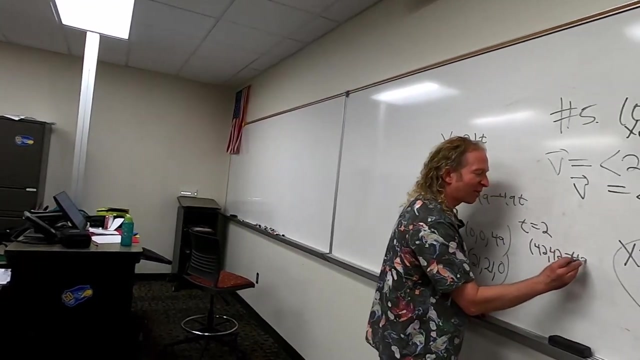 T equals something else, you're somewhere else. so like, if you do T equals 2, you're beyond this right, you're somewhere else. you'd be at 42, 42 negative 49, right negative 49, etc. so what happens is for each value of T, 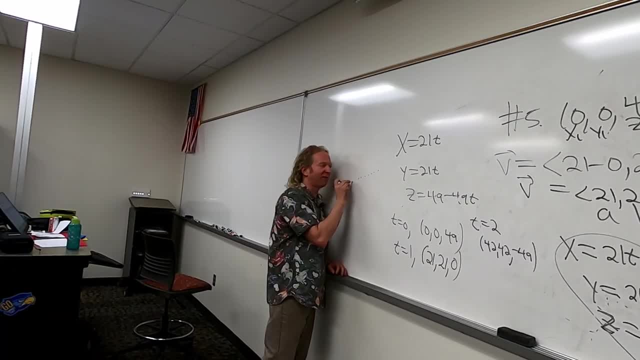 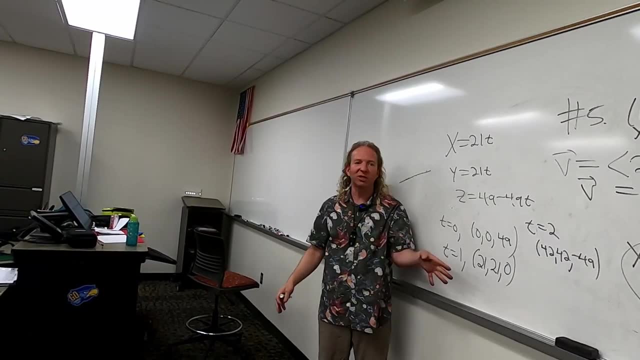 you're at a point on the line and so you have infinitely many values of T, so you end up getting a line. so as time goes by, it passes, it tells you where you're on the line. that's why we use T. someone asked: why are we using T? 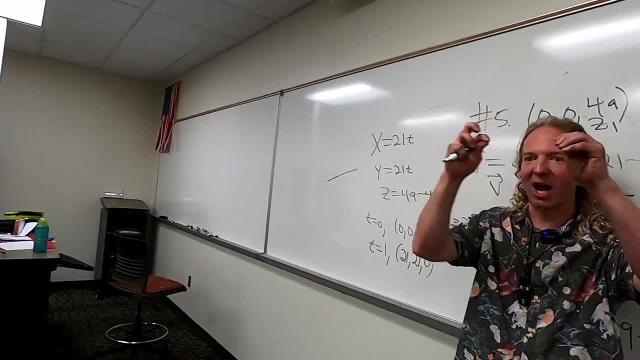 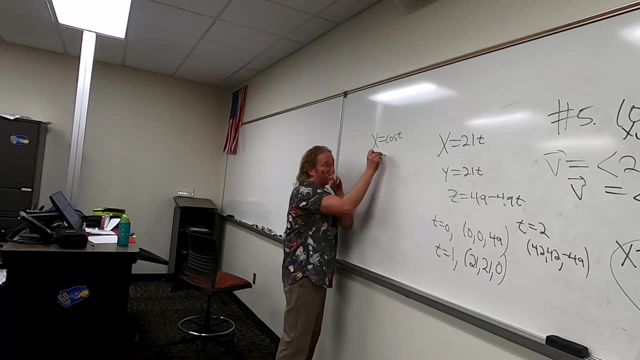 I forgot who that was. that was a really good question, because T represents time. an easier example- I hate to derail too much- would be something like this in 2D, like cosine T. this is later. this is the second test, because we're going to do it. 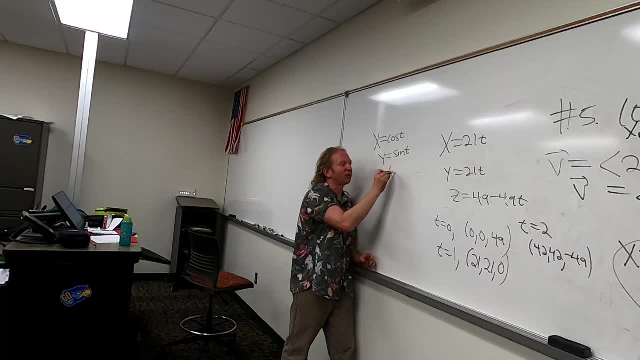 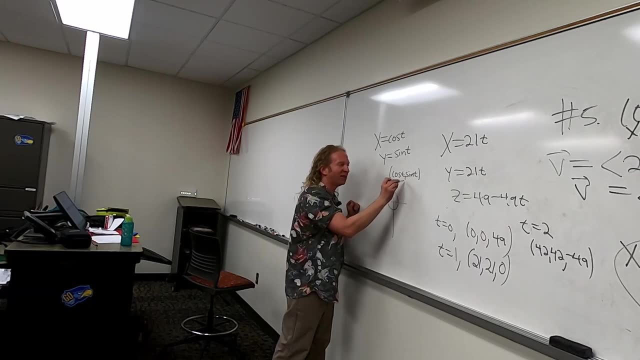 because it's awesome. this is a circle, right. so on the unit circle, it looks like this, right, every point looks like this: this gives you the entire unit circle right as T. if T is in 0 pi, 0 pi, 0, 2 pi, so as T varies from 0 to 2 pi. 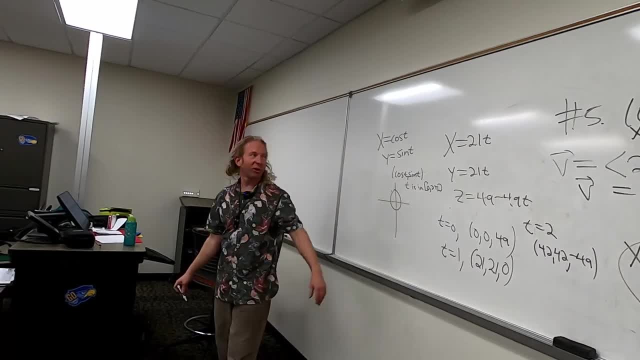 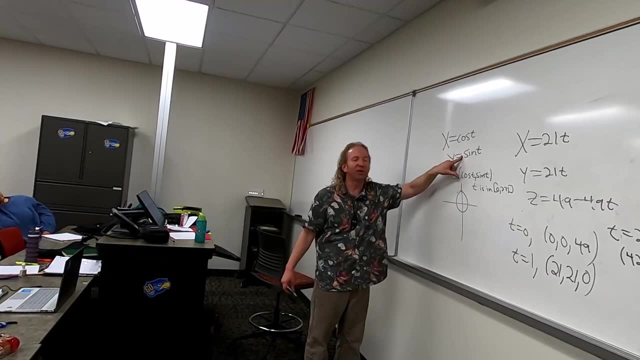 you end up getting the entire unit circle right. so, cosine and sine, parametrize the circle, in this case the unit circle. if I put like a 2 here and a 2 here, I get a circle with a different radius, a circle of radius 2. these parametrize 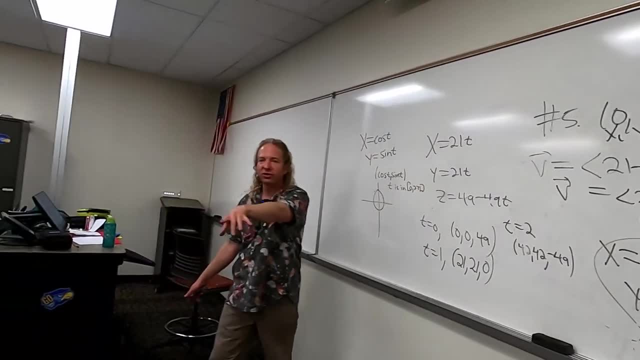 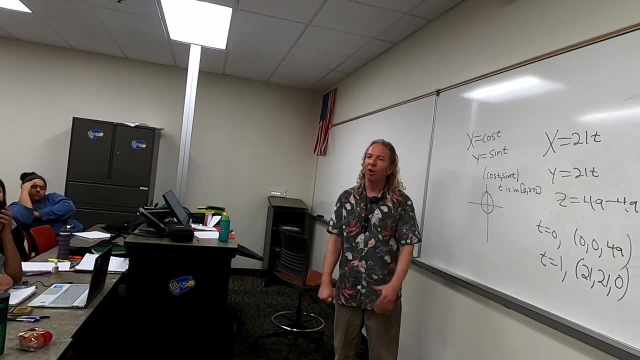 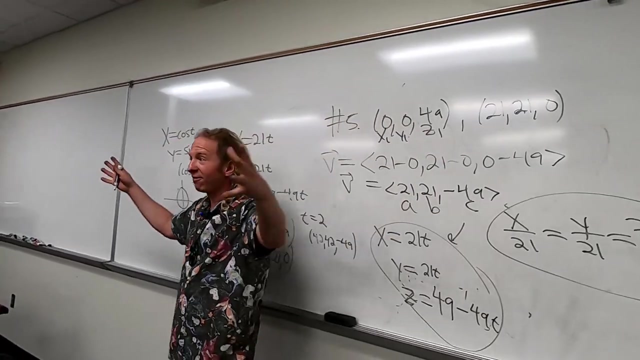 a line in space. the hyperbolic functions- remember cosine and sinc, remember those- those parametrize a hyperbola right, hence the name hyperbolic right. so we'll be doing a lot more stuff with these types of equations. so parametric equations describe something, a graph. 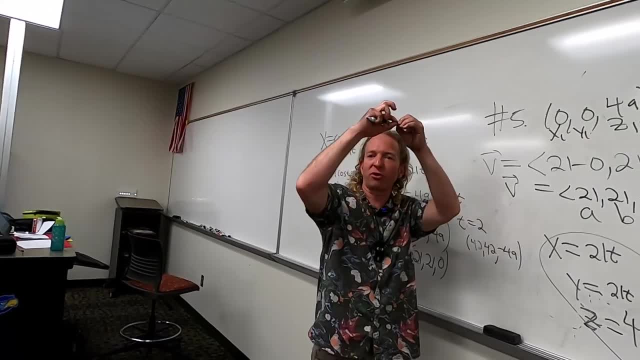 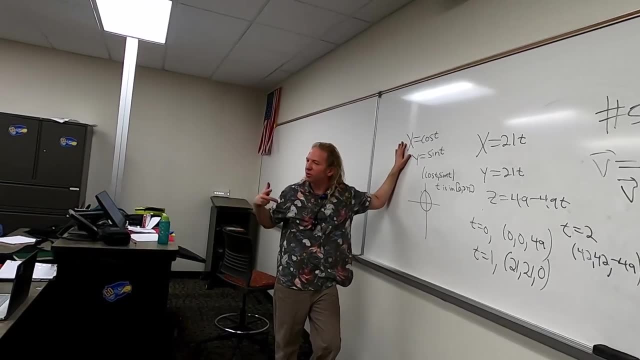 in this case a line, and they tell you where you are in the graph as time passes, just like these tell you where you are in the circle, or the hyperbolic ones tell you where you are on a hyperbola. so or later on, we'll have ones with a plane. 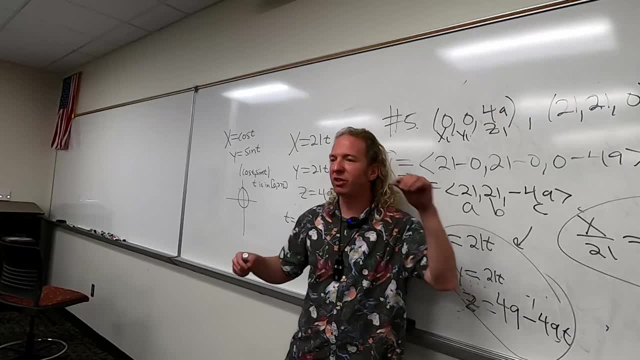 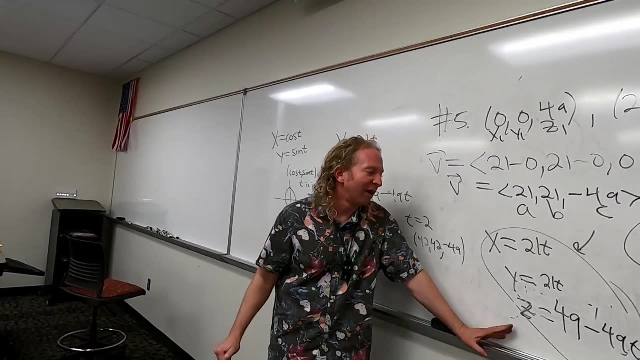 and stuff like that. so really important concept though, especially in 3D. so but it's just a line. unfortunately, it's just a line like it's not like a fancy curve, so you can't model like a flying saucer with this right, unless it's going in a straight line. 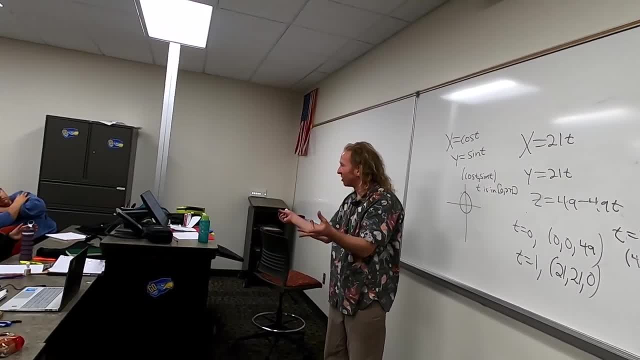 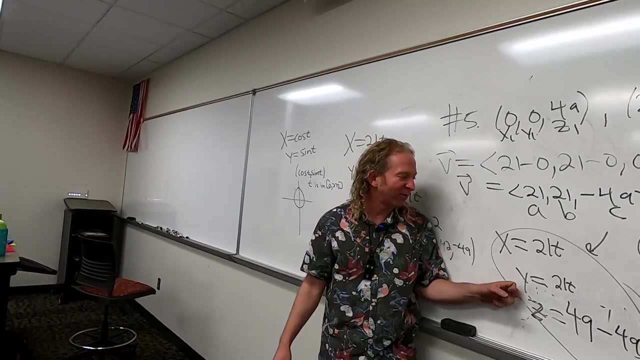 right, so like, but but what is the path of a flying saucer? right, if you could figure it out, if you could come up with parametric equations for stuff like that, you could model it. so really, really powerful. so t is usually time, so it gives you a point in space. 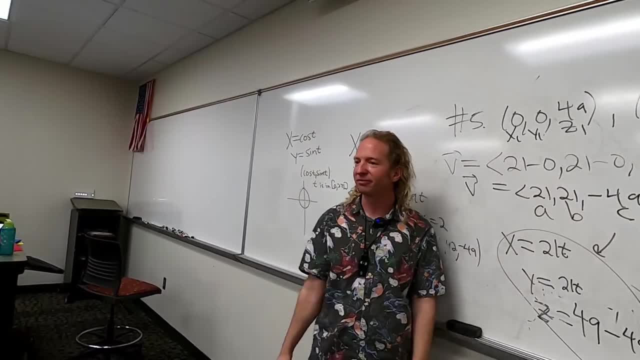 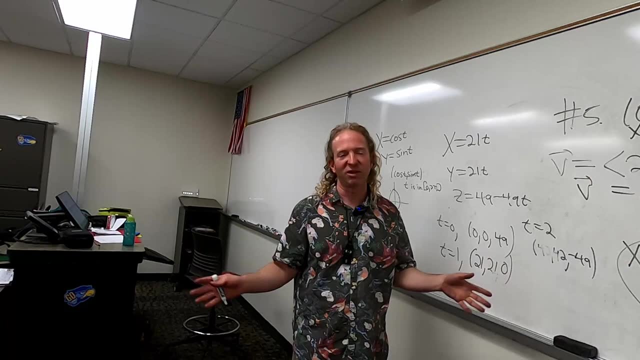 and x, y, z as time as time varies. does that help? yeah, really useful. I used to have this teacher a long time ago. he said that the most important concept in all of math- this was just his opinion right- was the concept of a path, because you can explain to anyone. 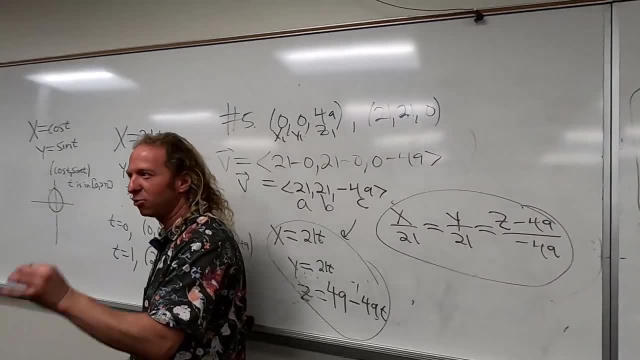 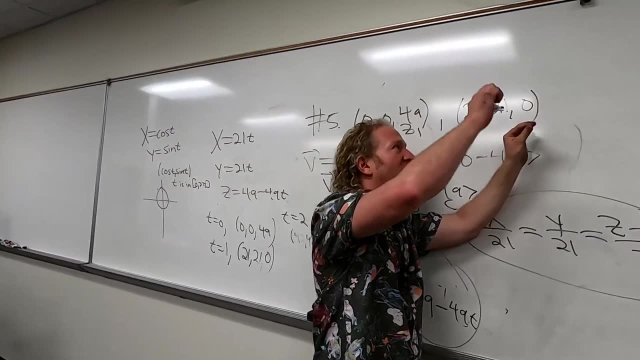 what a path is right, like you can go to a chemist, to a physicist, to a mathematician. most people in the world will understand if you tell them: hey, I'm trying to get from here to here. so to get from here to here, I have to travel along a path. 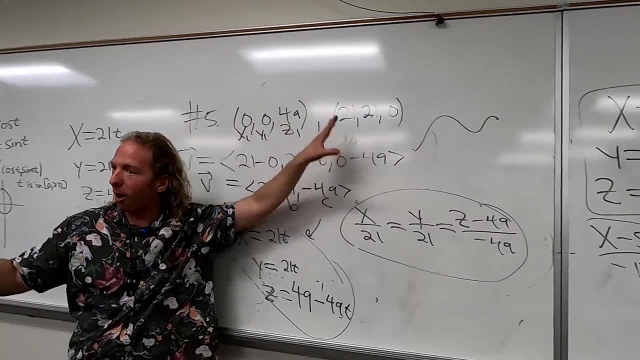 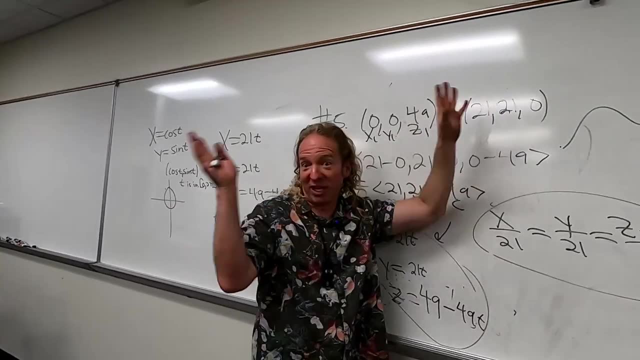 that's called the path. paths in mathematics can all be modeled in theory by parametric equations. so in theory, according to that guy, this is related to what he thought was the most important concept in math. I don't know if I agree with him, but that's. 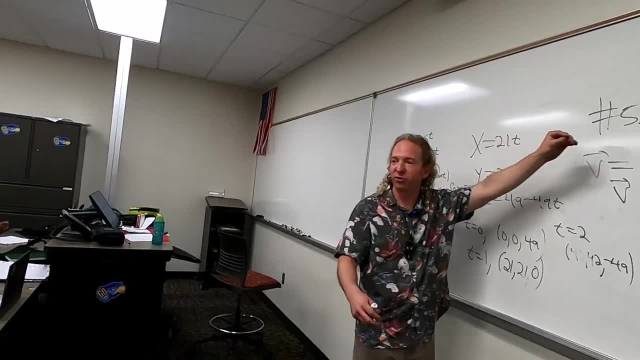 that's kind of cool, right, so kind of interesting, because you use it in all fields, right, and you use it in the real world too, right, like, if you're trying to fly to the moon, you have to take a path to get there, right, you can model that path. 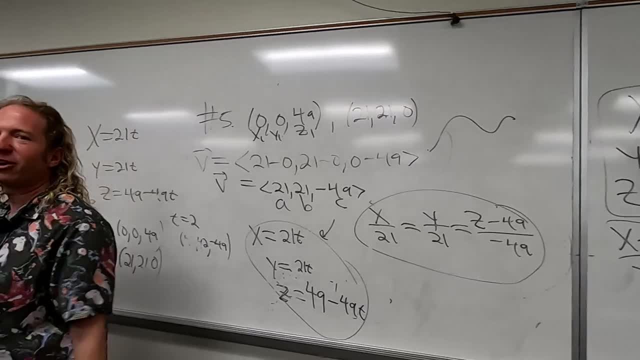 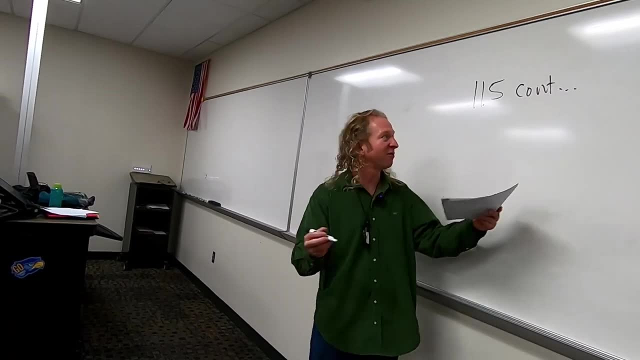 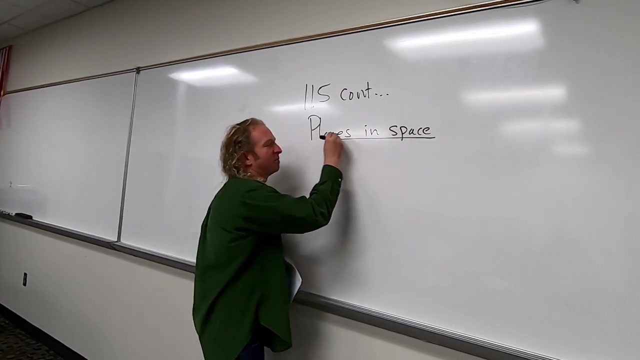 with parametric equations. so kind of good stuff. sorry, rent. it's good, though it's good, it's good stuff. today we're going to talk about planes in space, so let's go through and derive the equation: so planes, planes in space, planes in space, planes. so 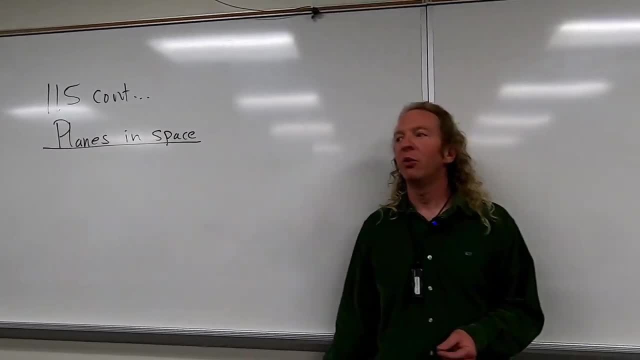 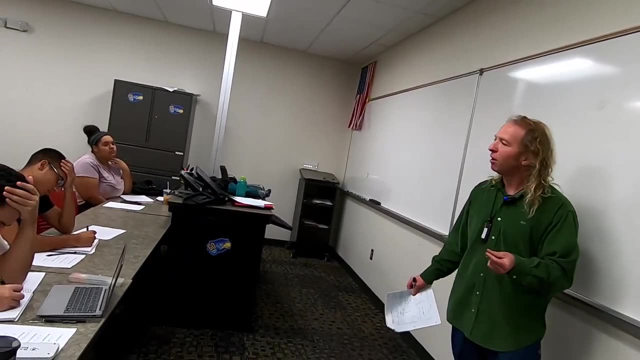 when we were talking about lines, to find the equation of a line, we needed a point on the line and a parallel vector and that gave us the equation of a line. when we're finding the equation of a plane, we're going to need a point on the plane. 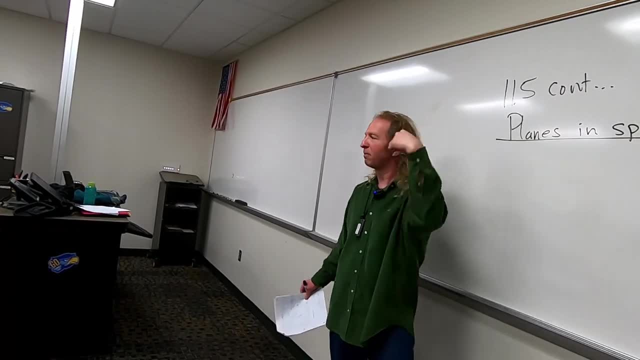 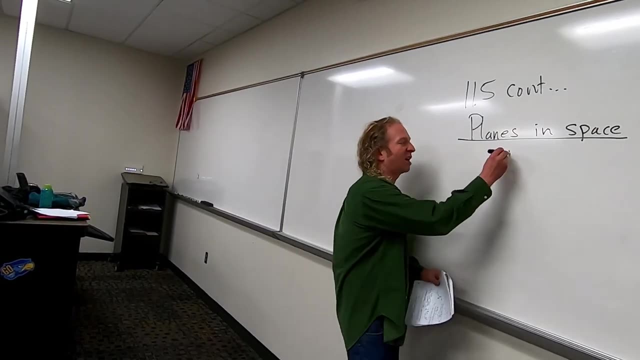 and a perpendicular vector. so, given a point on the plane and a perpendicular vector, we have the equation of the plane, okay, so I'm going to derive it really briefly. so here's: here's the z-axis, and and then here's the x-axis and here's the y-axis. 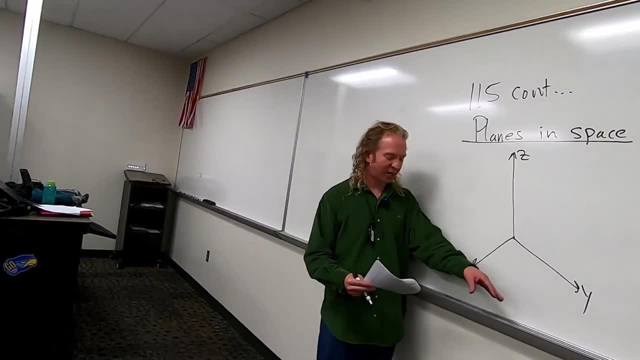 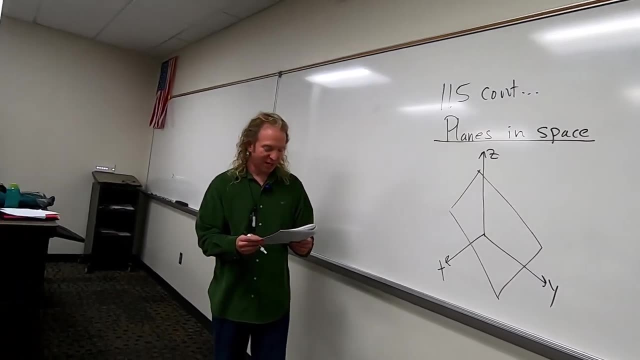 okay, so z, x and y, okay, and then I guess this is the plane. this is my really bad plane. there's my plane, there's my plane there, and I guess we need a point on the plane. I'm going to stick to my notes very carefully. 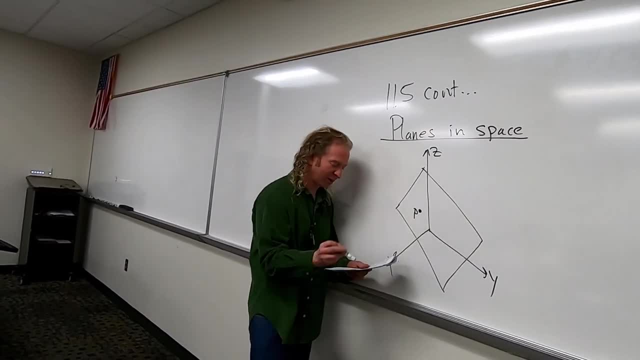 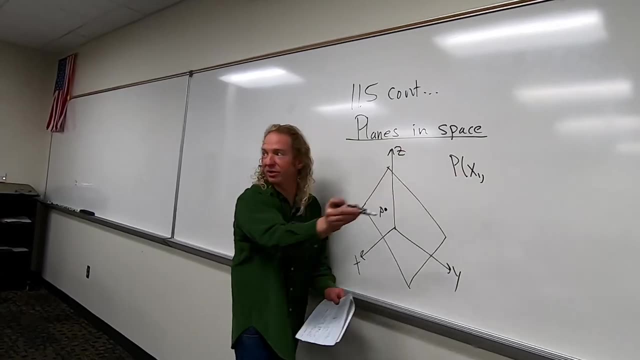 I'm going to call this P, so big P is my point on the plane, so P. I'm going to write it over here and write it as x1, y1, z1. that'll be P in the book's notation they tend to use. 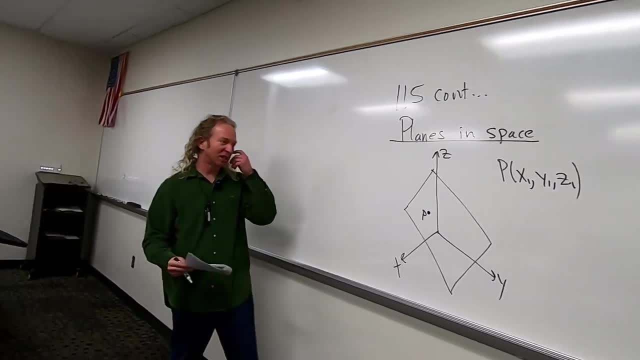 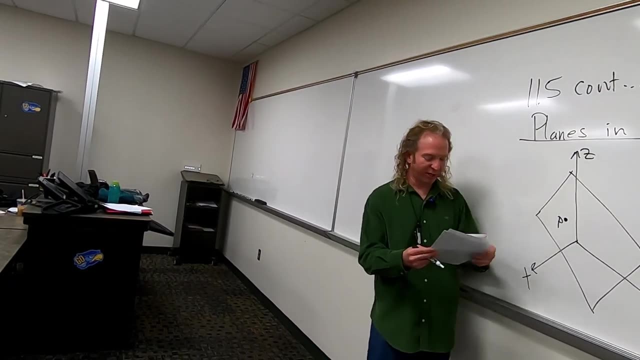 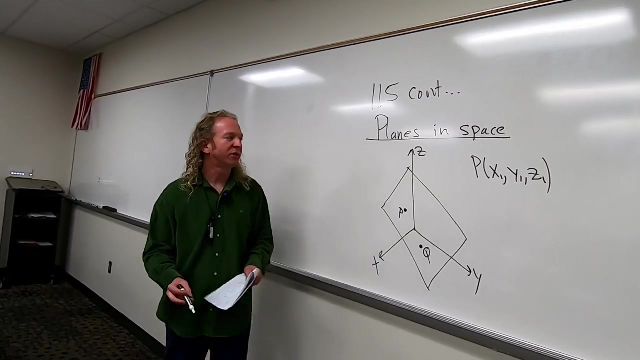 they tend to use notation like this, so x1, y1, z1 with the big P. okay, then we need another point on the plane which I'll call maybe q, q and so q. here I'll call that x y z, x y z. 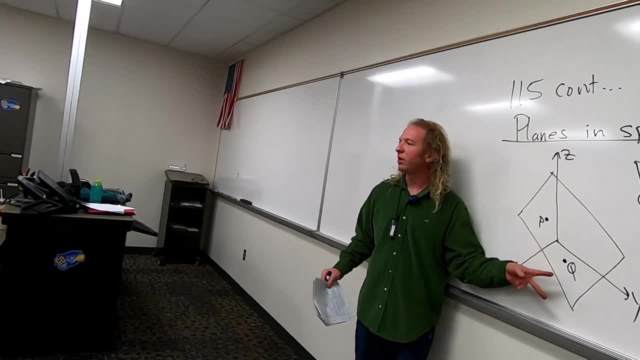 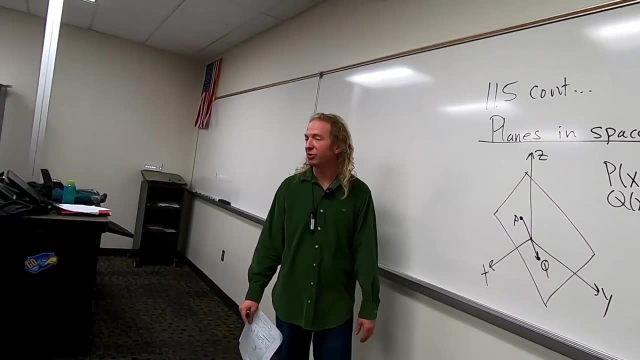 x, y, z. so whenever you have two points, you can form a vector, we can form a vector. so that'll be our vector Pq, which is on our plane, which is on our plane going really slow following my notes, don't want to mess up. 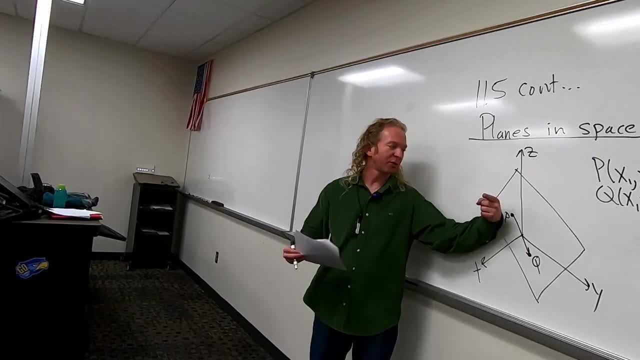 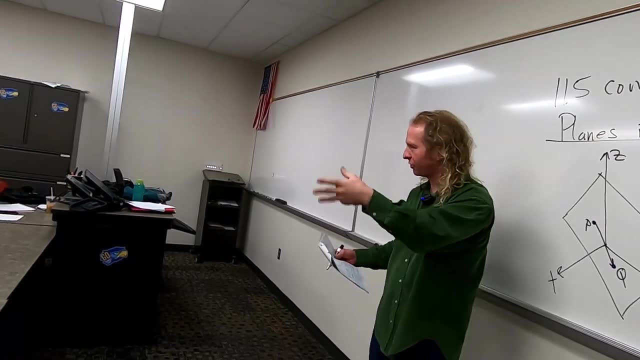 and then what happens is you need a vector that's perpendicular, so orthogonal. another word for perpendicular or orthogonal is normal, so normal, perpendicular, orthogonal, all the same thing. so we're going to call that n and put a little arrow on it. so this makes a 90 degree angle. 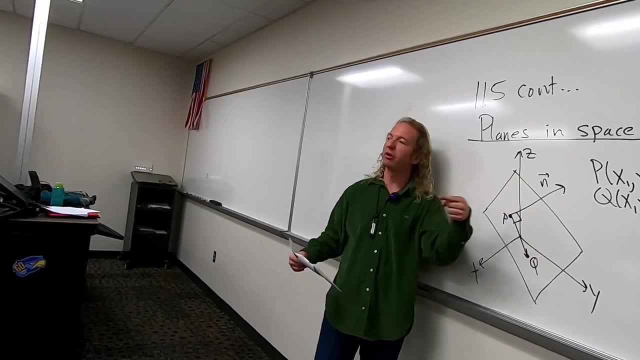 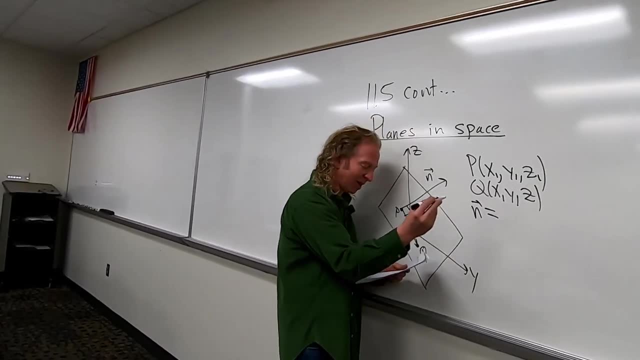 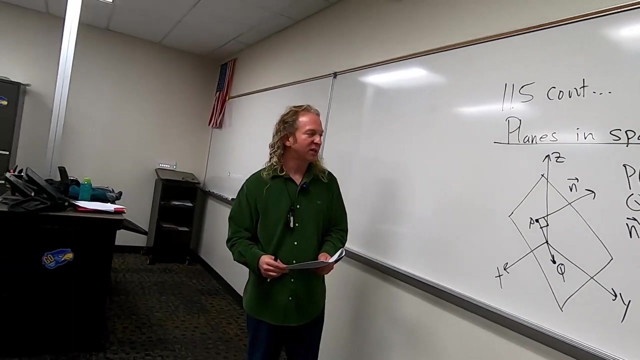 with our plane. so this is coming out of the board. this vector here lowercase n. so n here, n here we're going to call that abc. n is abc and here's the key. so x1, y1, z1. this is given to you in the problem. 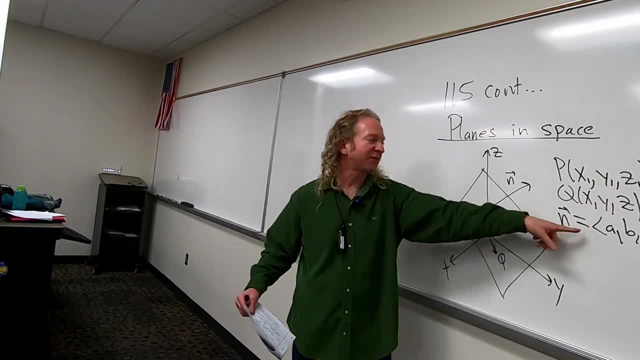 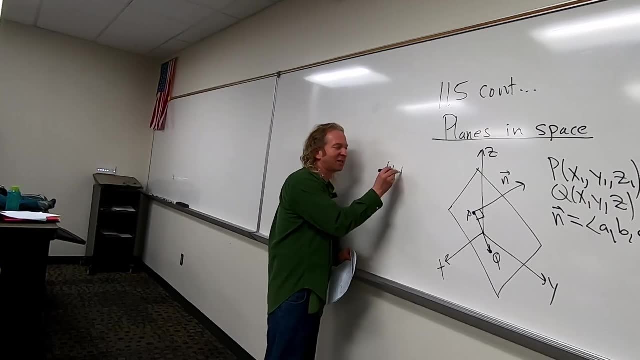 like 2,, 3, 4. they give you that pretty much always this you have to figure it out or it's given to you. this is like your variable, you know, like when you before, like when we have like the equation of a sphere, you have like x minus x, not squared. 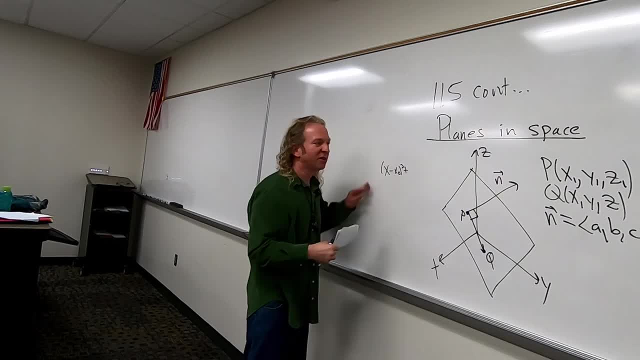 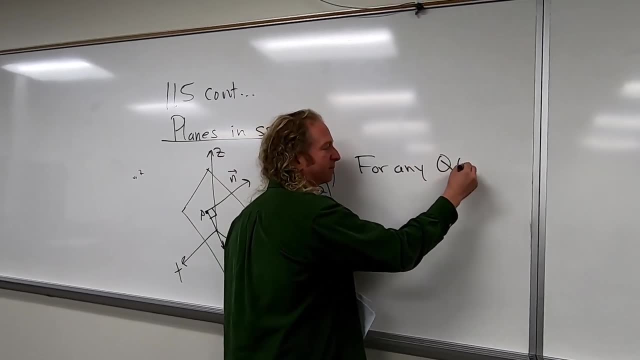 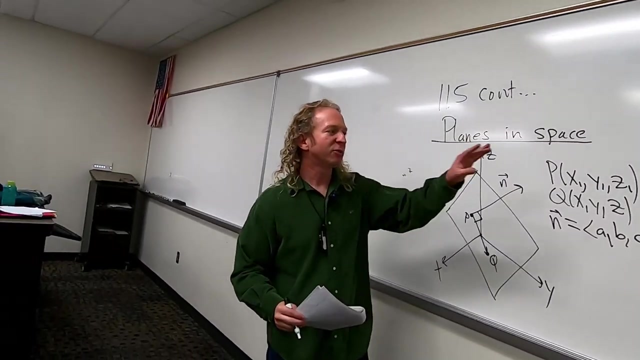 plus, etc. this is given, this is the variable. okay, so this is the variable. okay, so this is the variable term. so, for any q, for any q, just to be really perfect and correct, 100% correct, we got to be correct, it's math. so for any point q on the plane. 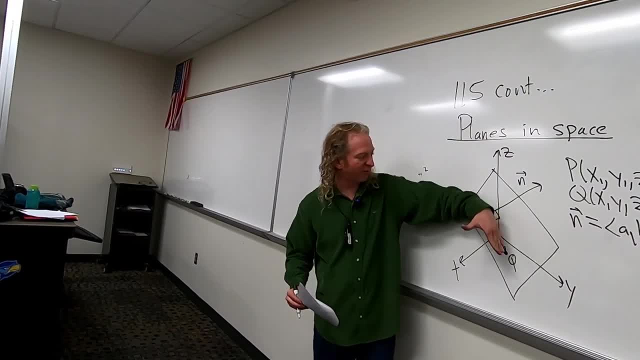 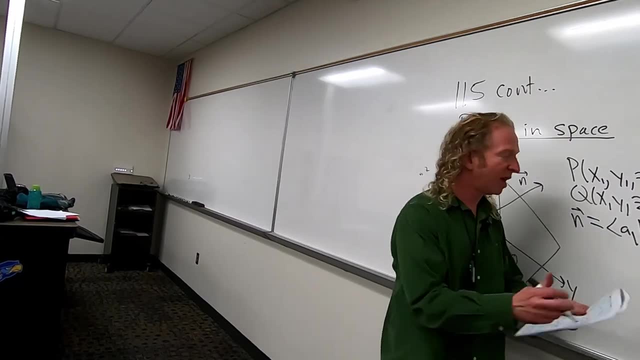 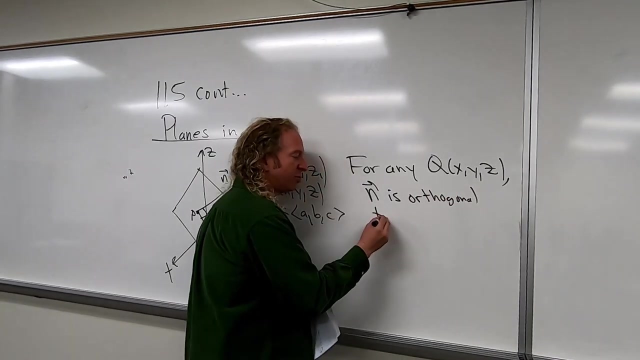 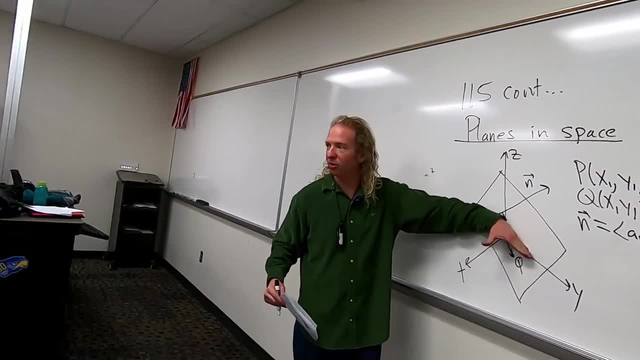 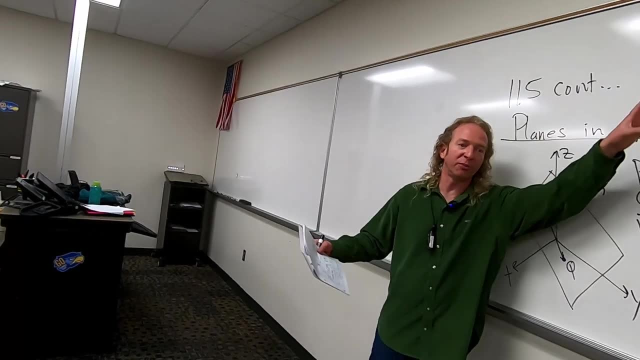 so I can pick any q. I pick a q. here I get a vector, pq, and n is perpendicular, right, because n is perpendicular to the plane, right? so it's perpendicular to all vectors, pq for all q. so what happens when you have two perpendicular vectors? what happens? 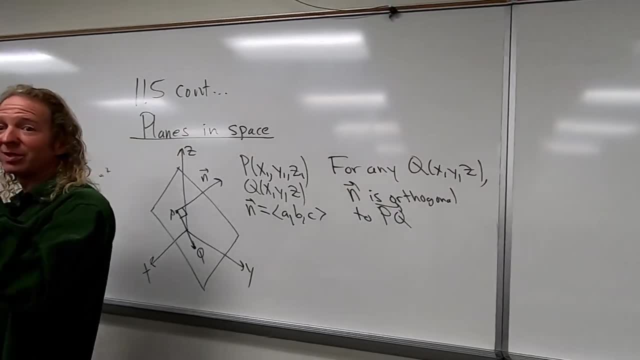 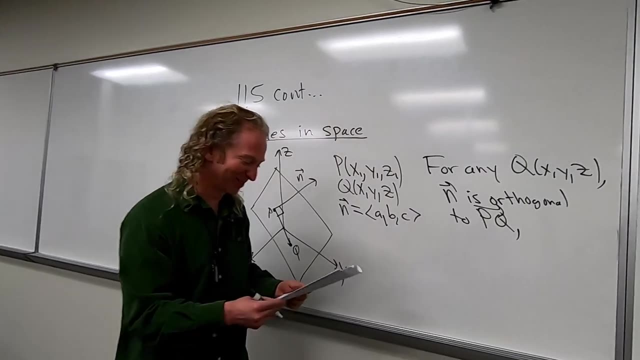 when you take their dot product, what do you get? do you remember zero? yeah, good Luigi, you get zero, right? so this means that for any q- very good Luigi, extra credit. no, I'm kidding, you don't need it. so n dot pq is equal to zero, the number zero. 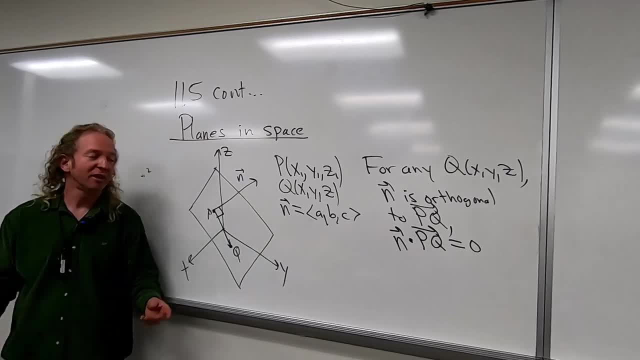 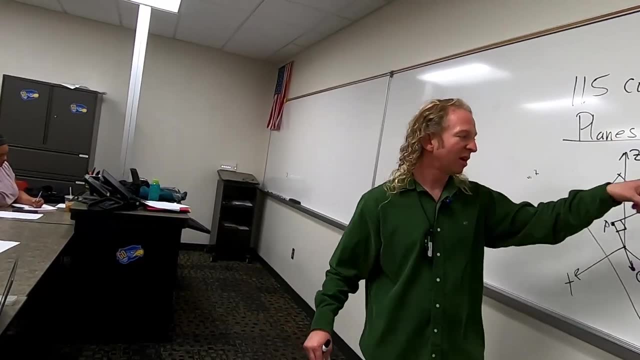 not the vector zero right. so the dot product of our normal vector and our vector pq is zero. so for any point q on the plane, n dot pq is equal to zero. right n dot pq is equal to zero. right n dot pq is equal to zero. so let's write that down. 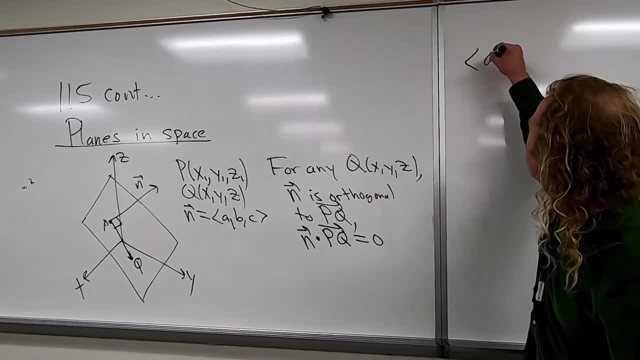 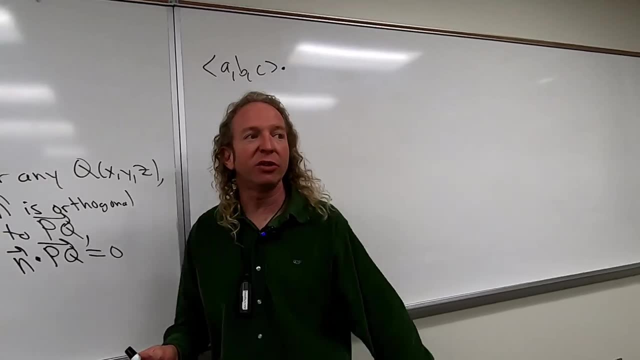 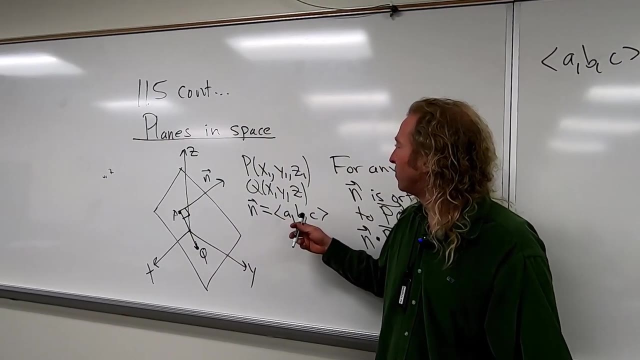 mathematically. so n is abc, so we know that. so abc dot and we can find the vector pq using some math from before. to find the vector pq we have to subtract them. do you remember the trick? it was something minus something. final minus initial. yeah, final minus initial. 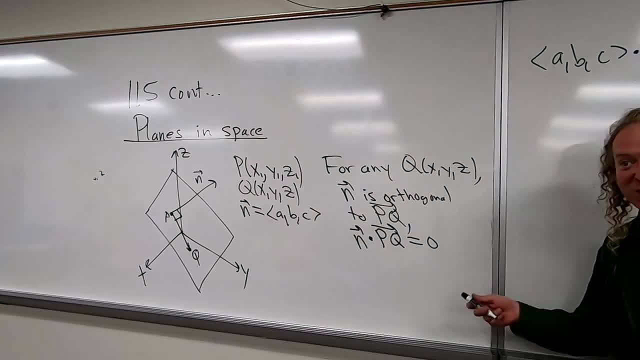 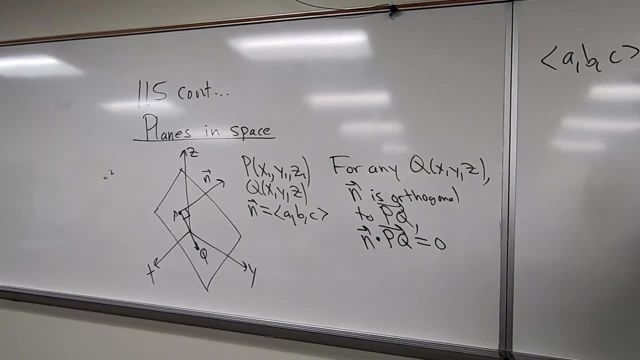 terminal minus initial. yeah, very good, so it'll be this minus this right, this minus this right, so it'll be x minus x one. i love when we can derive stuff and it makes sense, like it just makes me feel good, like i don't know, it's just. 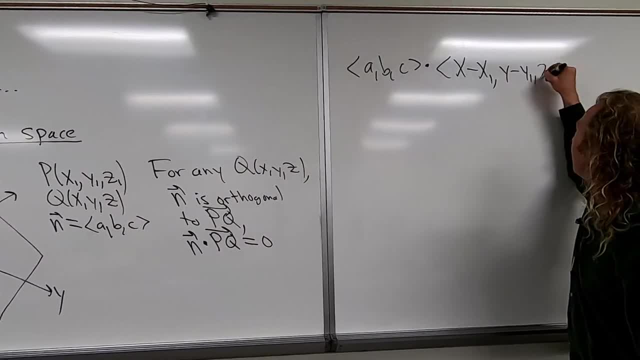 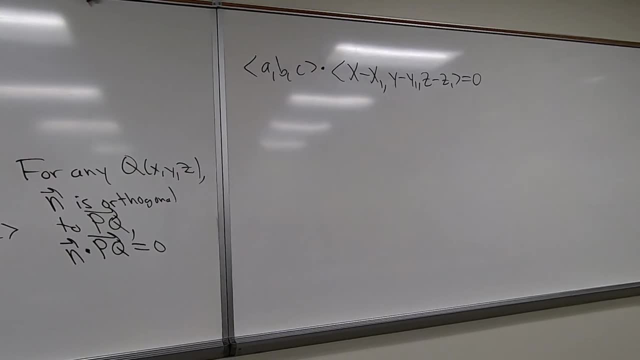 it's great. so y minus y one. if it doesn't make sense, it's okay. um, and that's equal to zero, right? so it's just terminal minus initial. that's the key, right? so the dot product is equal to zero, because they're perpendicular for any q. 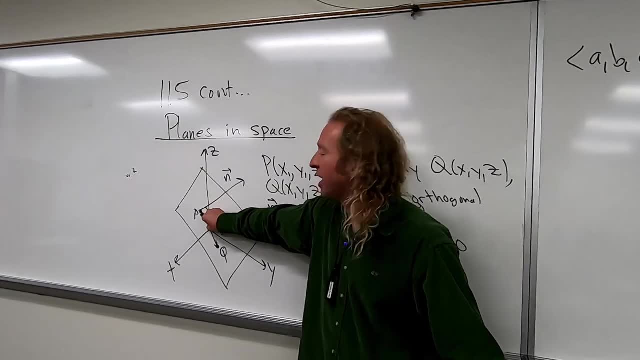 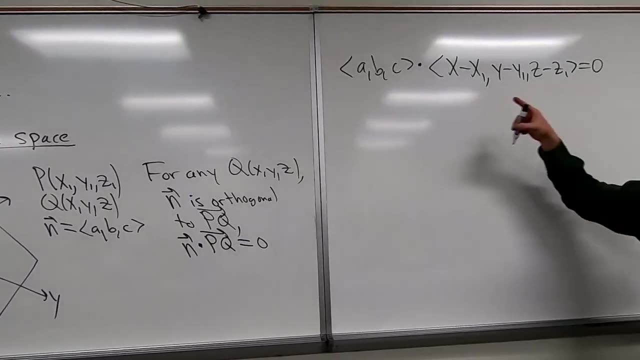 right. so q is. so for any point q, i get a vector on the plane and n is orthogonal to the plane. so the dot product is always going to be zero for any q. so this is true for all x, y, z on the plane and then the dot product. 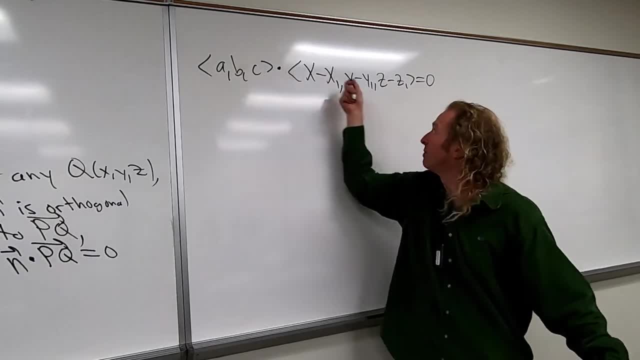 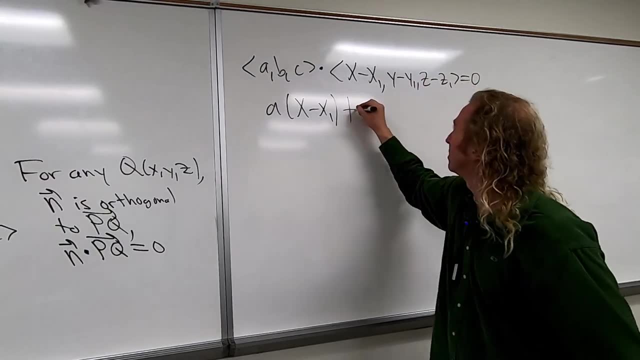 basically says: you multiply these, right, you do this times this plus this, times this plus this times this. so we get a times x minus x, one plus b, times y minus y, one plus c, times z minus z one, and that's equal to zero. and that's the formula. 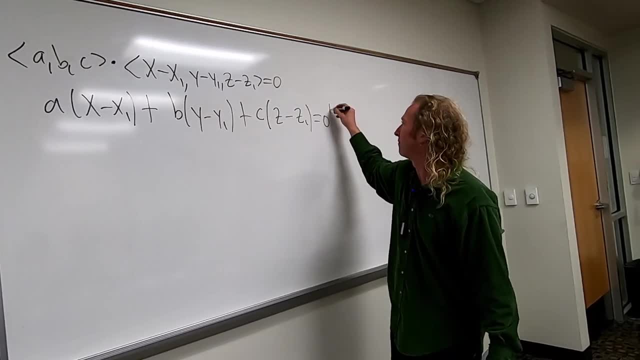 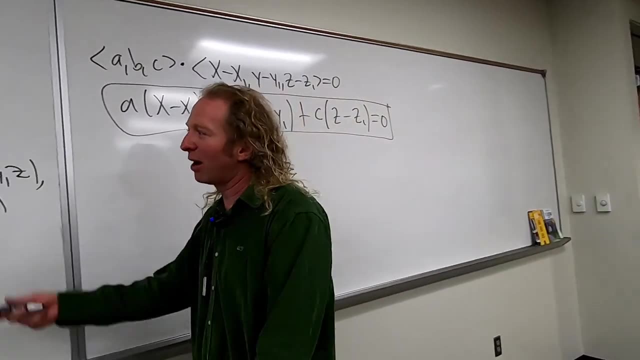 right, you want to memorize that for for the test. that's the formula. i could have done that for the test. that's the formula. i could have just started with this. i thought about it when i, when i, when i was over here, i was, i didn't say it. 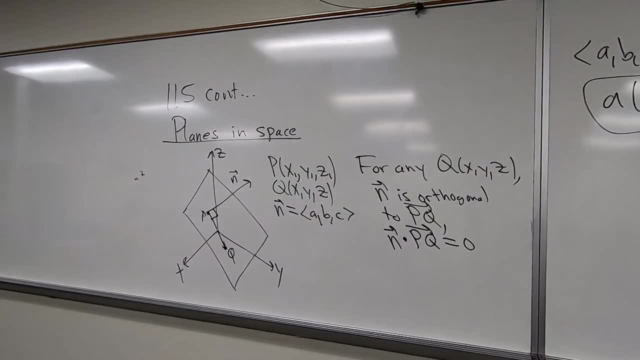 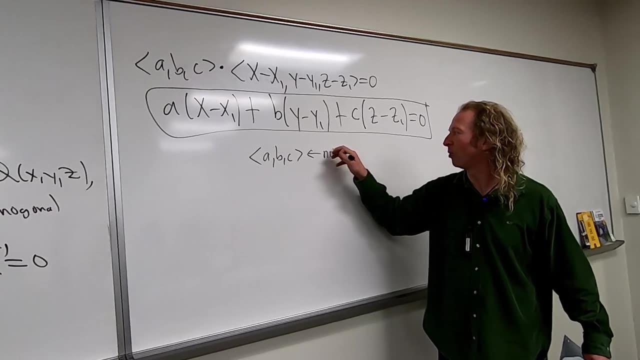 but i thought i thought maybe i should write the formula. no, it's good, it's good, it's good to go through it. so that's the formula. so what is what is a b c? a b c. this is our normal vector. okay, this is our normal vector. 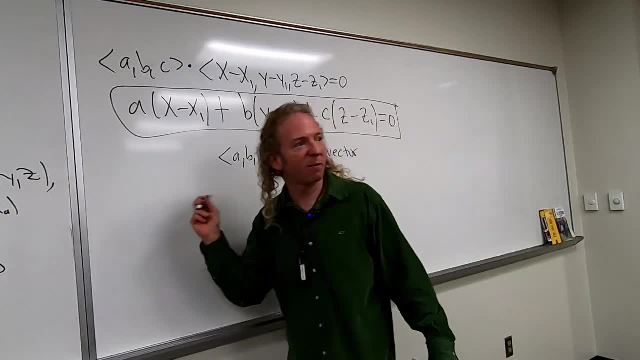 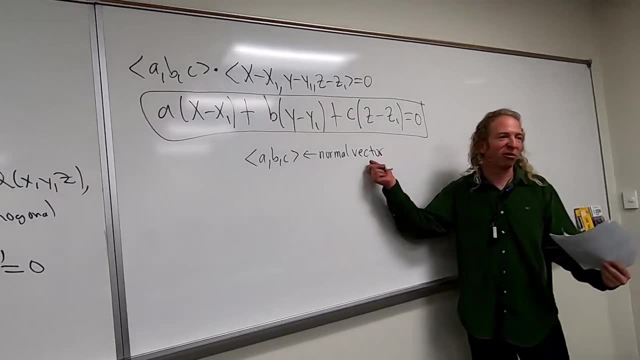 this is normal to the plane. i'll call it normal vector. this is perpendicular to the plane, always, right, it's perpendicular to the plane. so that's the problem. sometimes you define the equation of the plane. the goal is to find this. that's the hard part. sometimes it's given to you. 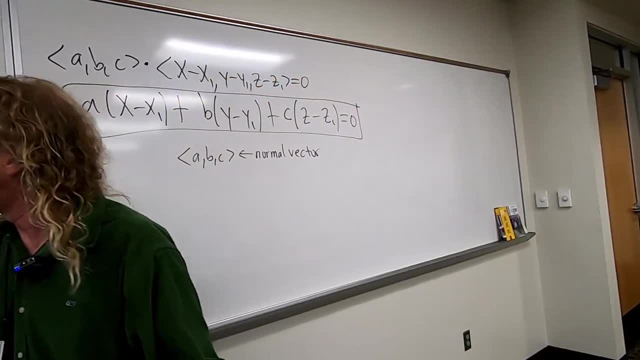 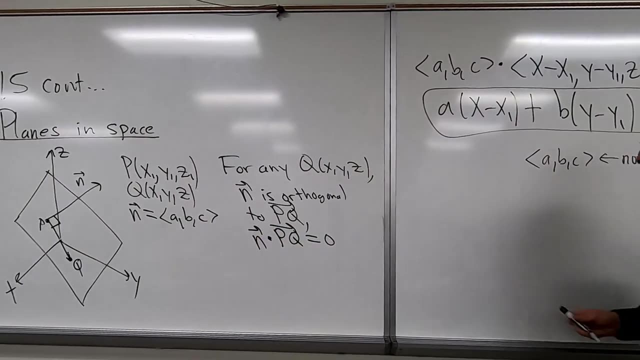 all right, there's easy problems too. and then x1, y1, z1, oh, oh, oh, look, oh no, i didn't mess up. i thought i messed up. i thought that was supposed to be a z1, but it's not that, that's a z1. 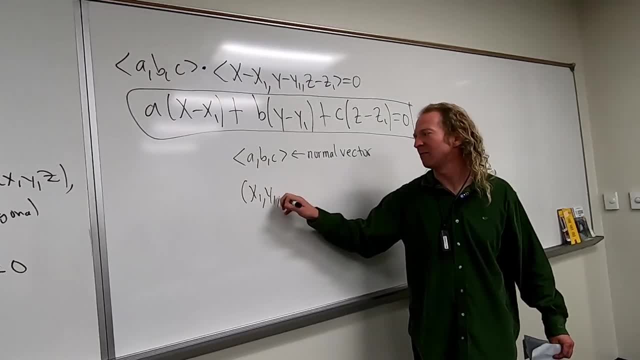 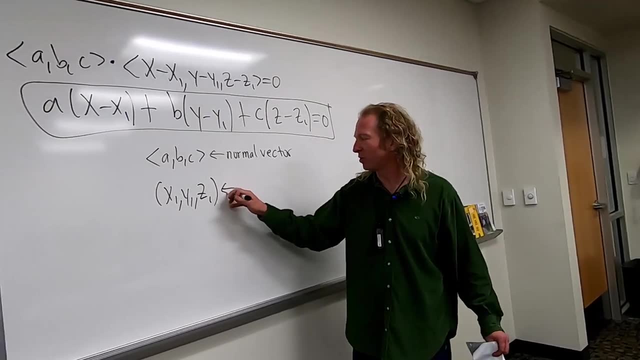 right. so this, this is our point on the plane. have i made any mistakes in this class at all? like, have i made? i have maybe one or two. maybe one or two. i'll check, okay. okay, february is a good month usually, so this is a point. 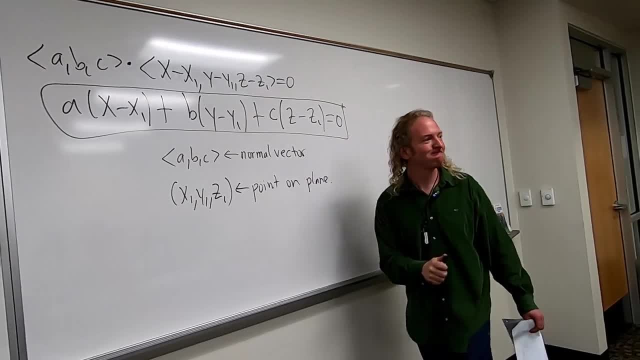 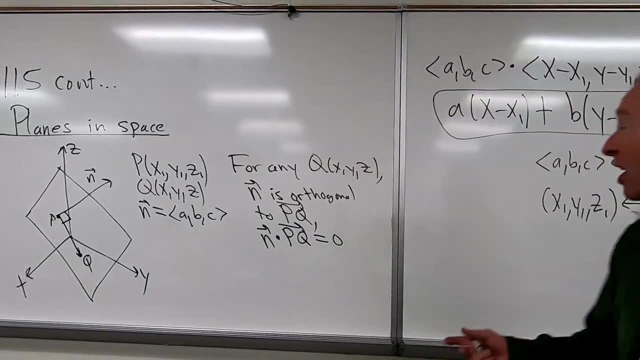 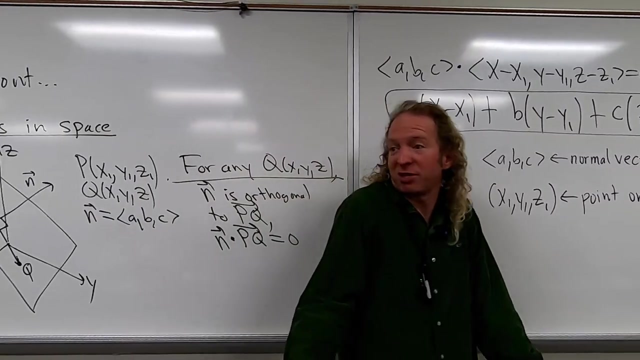 on the plane. point on the plane. yeah, all right, that's it. that's it. q is also a point on the plane. yeah, q is the variable point, though, right, yeah, that's why i said it like this. yeah, it's also a point on the plane. they're both points. 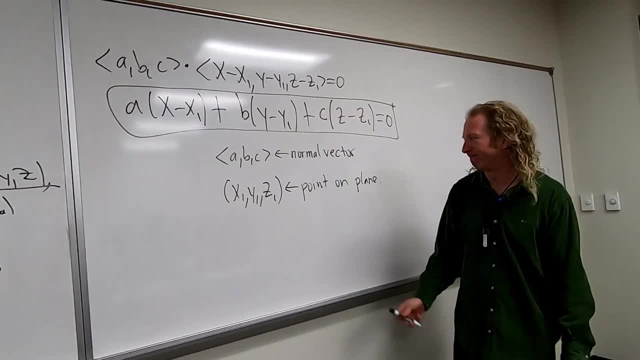 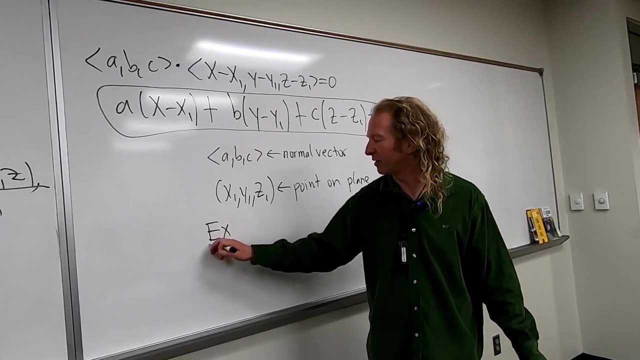 on the plane. yeah, this is the one we usually talk about: um, what else, what else, what else? sometimes they're not written this way. it's like, let's say, let's say you're looking at a plane, like say you're on the street and you run into someone. 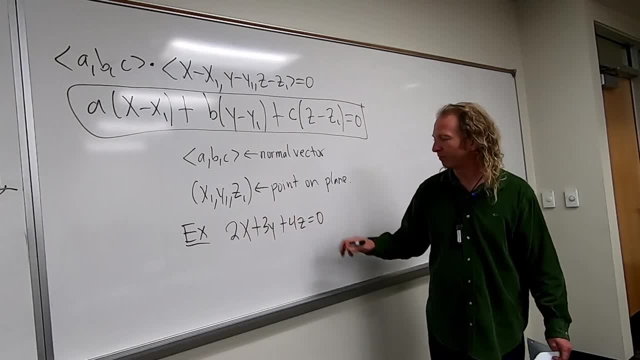 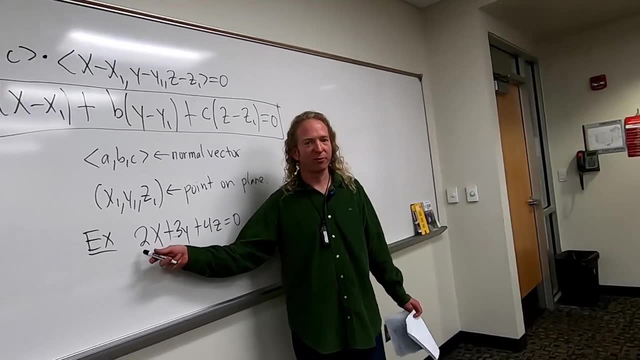 and they say: hey, you know, 2x plus 3y plus 4z equals zero. that that's what i got right. and they say, well, what's? what's the? what's the normal vector, so you can just get it straight from here. so it would be. 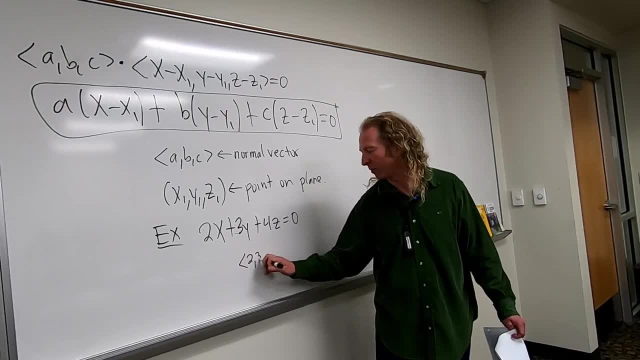 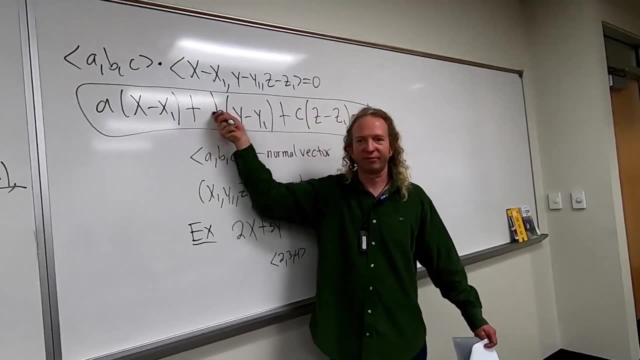 two, three, four. so the normal vector here is, so you can get it from here. you might say it doesn't match that. yeah it does. you can distribute all of this right and you still get ax plus some stuff by plus some stuff, cy plus some stuff. i just put a zero. 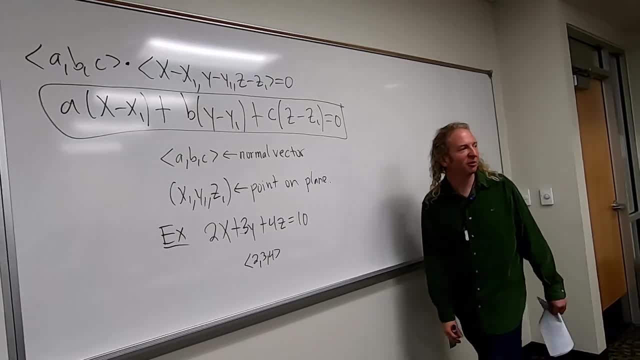 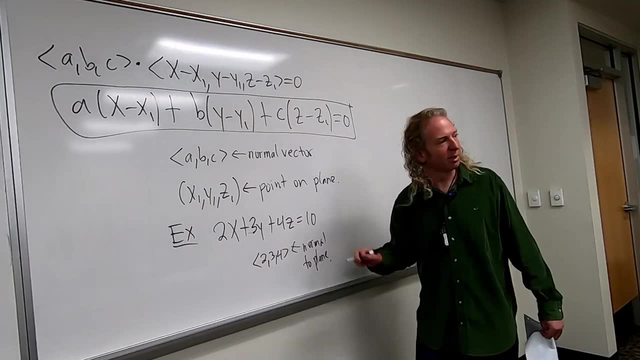 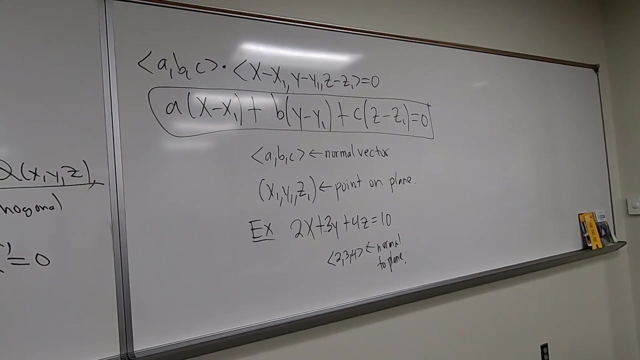 i don't have to put, i can put ten here, it doesn't matter, right? so this is normal, normal two plane, normal two plane. so you can get it from that. okay, you can get it from that. that's the point, okay, all right, we're done. all that's left. 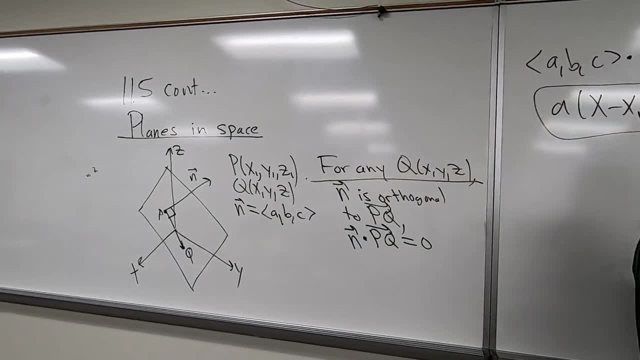 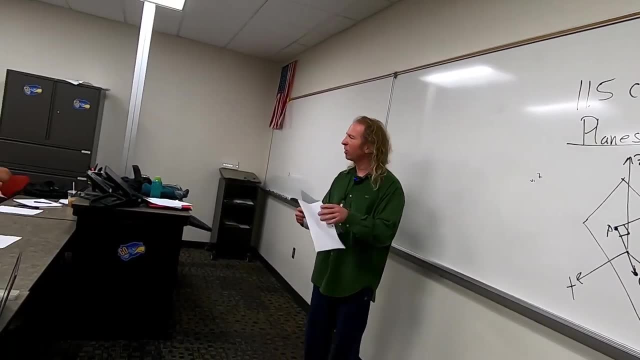 is problems to do. this is called the general form, by the way. so let's just do homework right, let's just do homework problems. that's all the theory there is. anyone have the homework up, anyone have it up, anyone have it up, you do, you do, rafael. 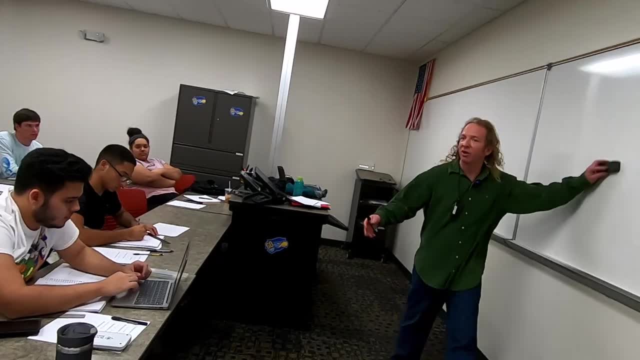 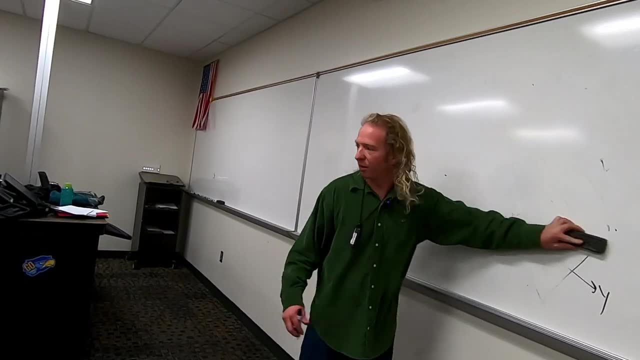 rafael, let's just do all of them. if that's okay, if you all, let's just do all the problems. what's what's the first plane problem, rafael? which number is it second? 1.7 is also in the homework. yeah, yeah, i know. 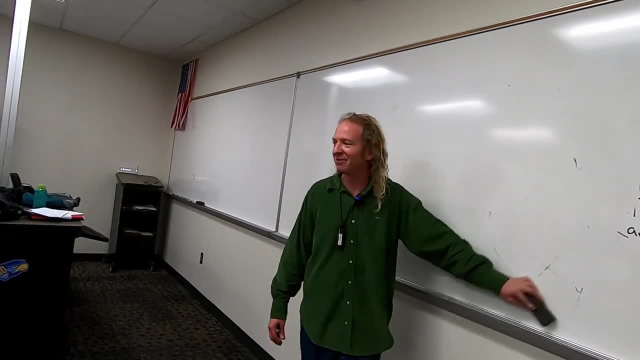 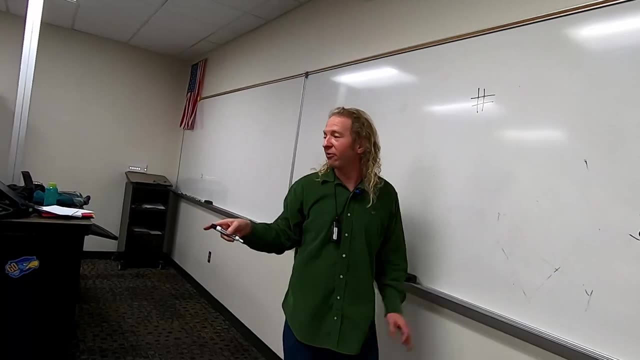 yeah, yeah, it's easy, it's easy, okay. so number one is point zero, zero, zero. wait, what problem is this number one? no, no, no, eleven, five, right, yeah, what's the first? the first plane question? oh, mm-hmm, yeah, i think it's like seven or eight or something. 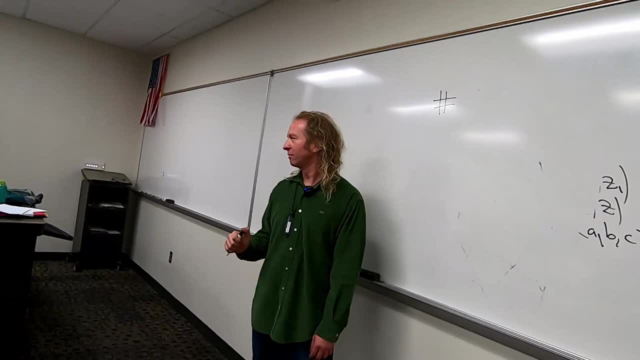 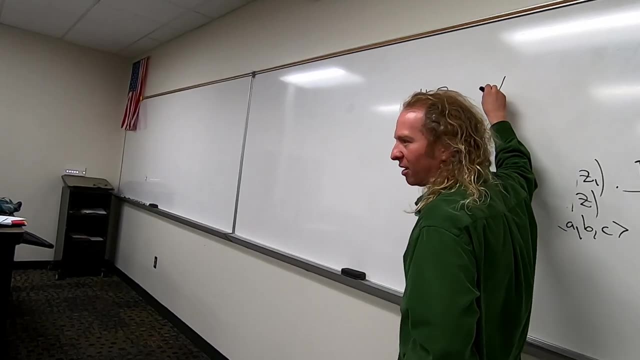 seven. was it seven because i was doing it last night? i think i remember that six. yeah, it is okay. so, thank you, michael. that's plus four y, what's it say? uh, determine whether the plane passes. no, not that one, that's eight. that's eight the next one. 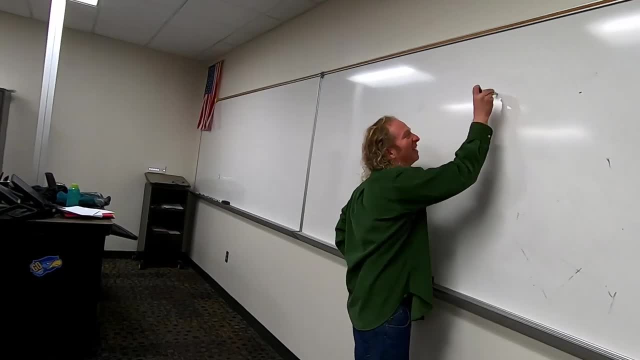 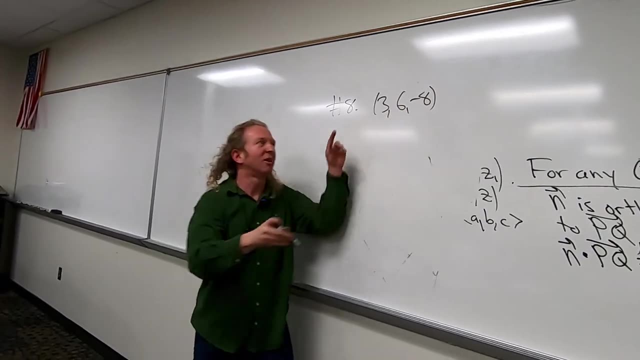 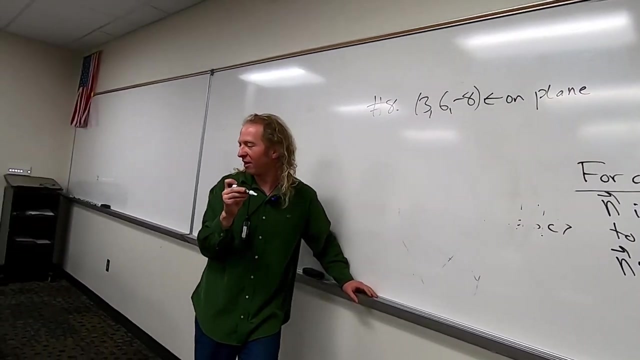 okay, okay, point is three, six and negative eight. and what does it say? this is, on our plane, an equation of the plane that passes through the given point. okay, the given point from, and it's perpendicular to the given vector. what's the vector? um, it's perpendicular to. 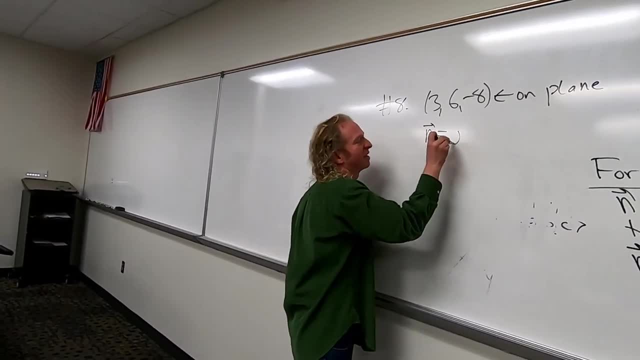 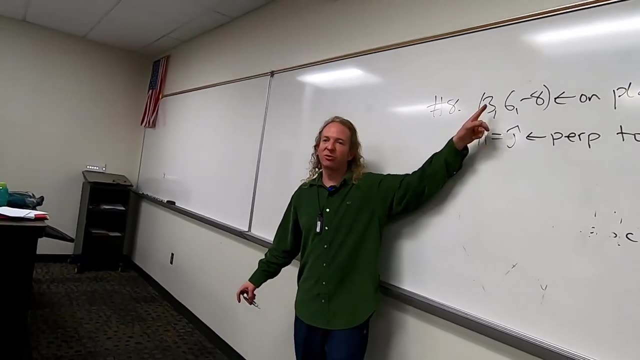 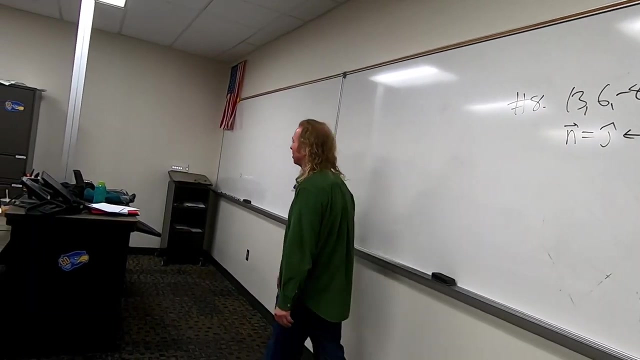 n equals j, j, j. okay, so it's this. thank you, rafael. so it's perp two. okay, so the plane, the question says that passes through this point and it's perpendicular- hey, is perpendicular to this vector. okay, that's the. that's the question. 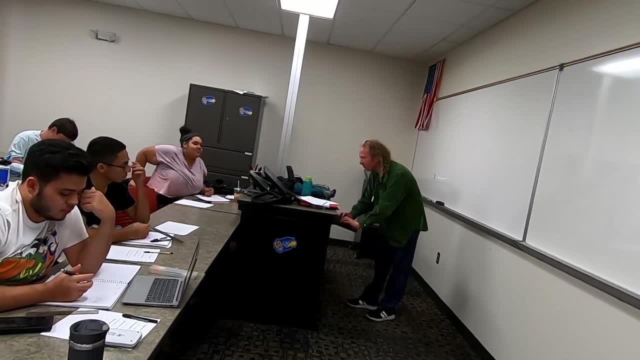 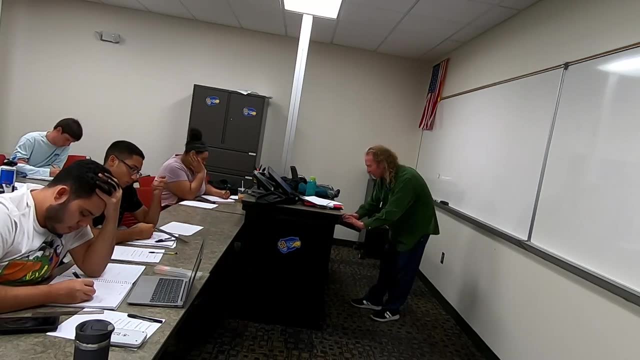 i'm going to sign in too. look at the homework also, so find the equation of the plane that passes through that point and is perp to that vector. so this is the easiest possible case. um, because they give us everything right like, so all we need to do? 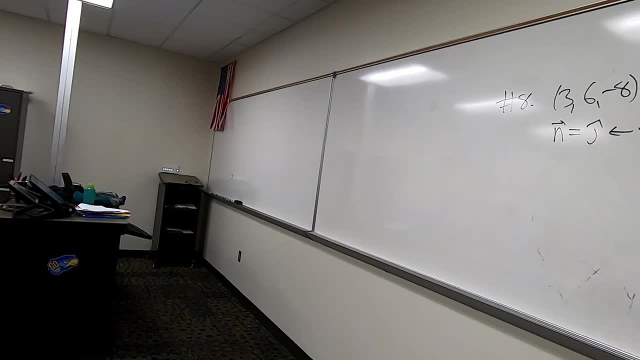 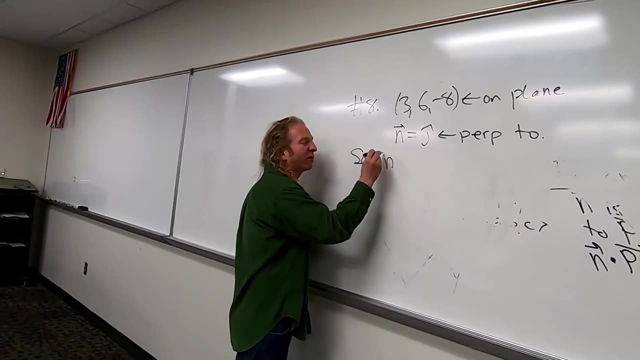 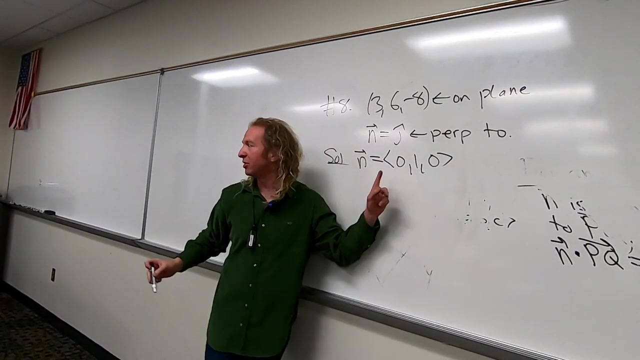 is figure out the stuff. so they're telling us that this is this, right, right. so we just have to write this in component form. so, in component form, what would the component form be for? j hat, do you all know? zero, one, zero, zero, one, zero. very good, michael. 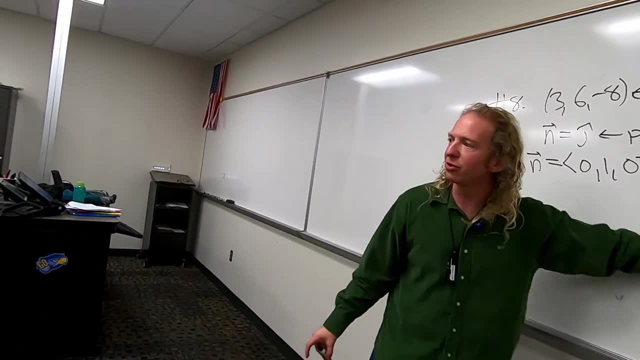 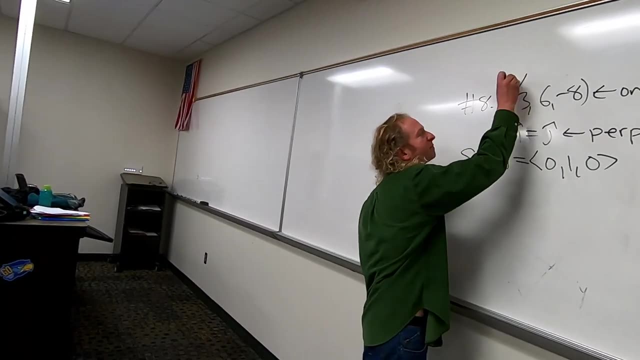 yeah, zero one, zero. it's one of the unit vectors. right, it's one of the standard unit vectors. so our plane is perp to this and this is uh on our plane. so this will be our x one, y one, z one, and then this will be our. 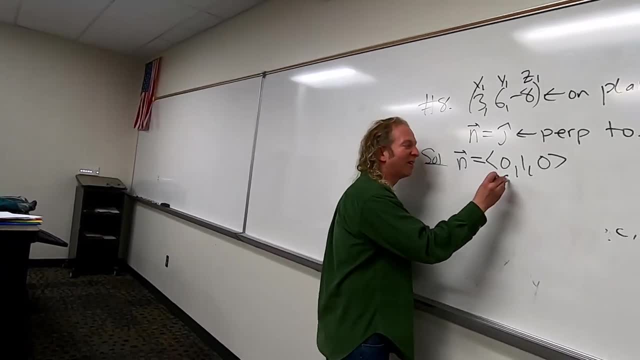 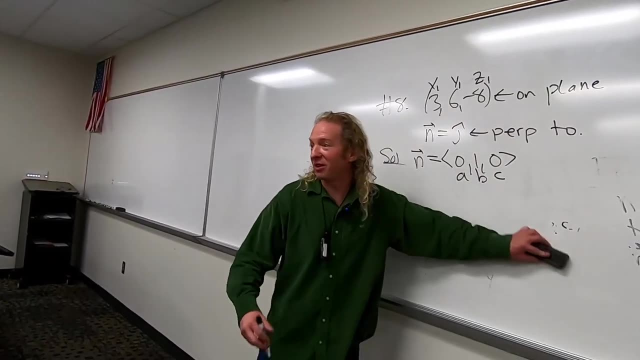 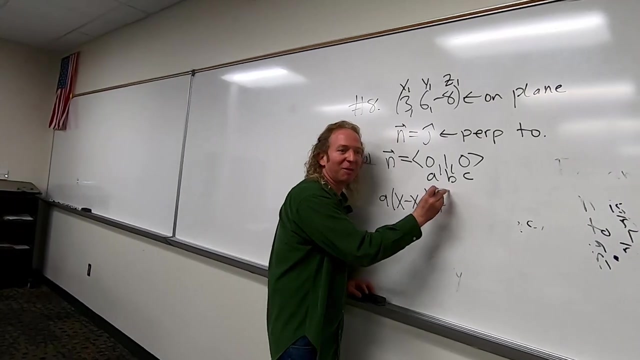 a b c, right. hey, what's going on here? a b c, my shoes awesome. a b, c, all right. so then we choose the formula right. so i'll write the formula down, just in case. so it's a x minus x one. it's over there, but why not? 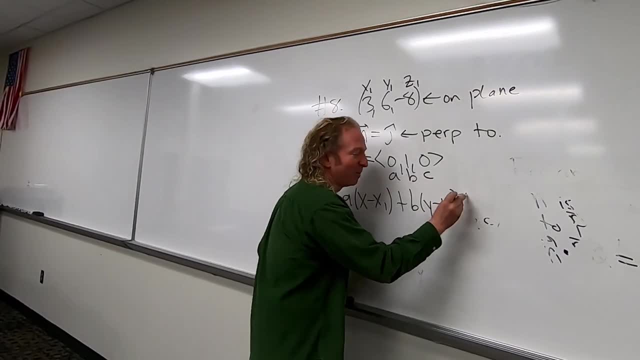 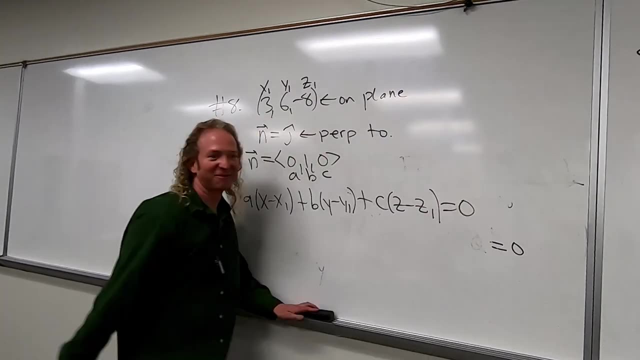 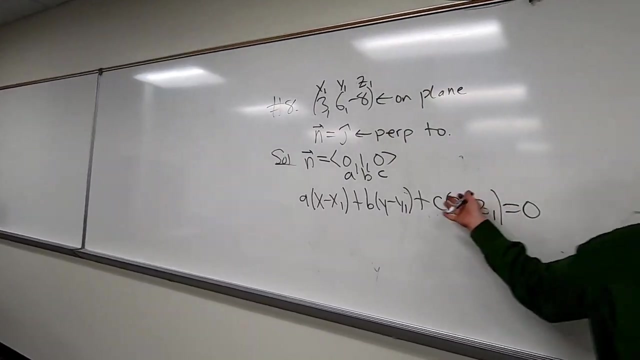 plus b y, minus y one, i don't know, it's just making it seem longer- plus c, see you, see you later. bye, you can skip this step. i just wanted to to show you this step. so any questions, any questions? this one, yeah, can you assume it's equal to zero? 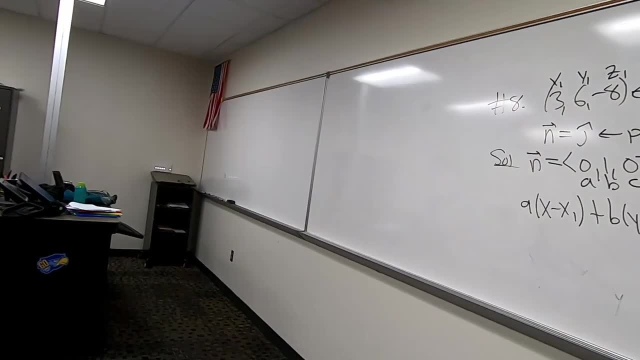 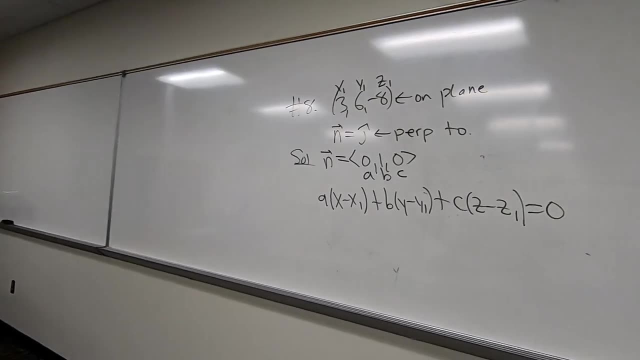 the equation on the bottom: yes, yes, this is the formula. okay, so what about when it's equal to ten? ah, so this is different. so, basically, how do you get this? if you were to multiply all this out, you would. you would get a number over here, right? 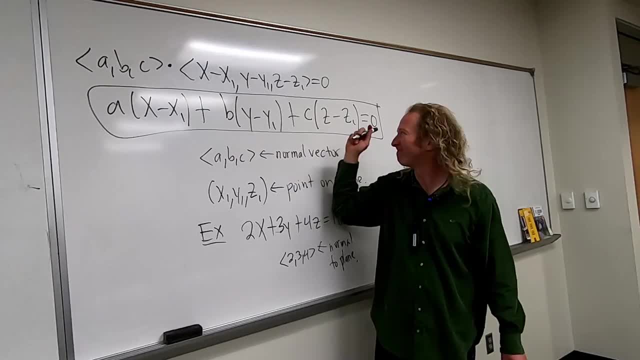 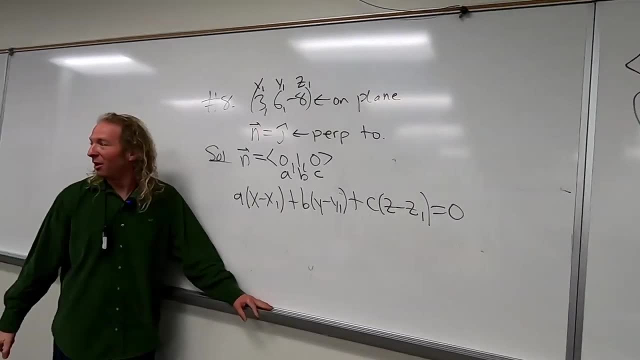 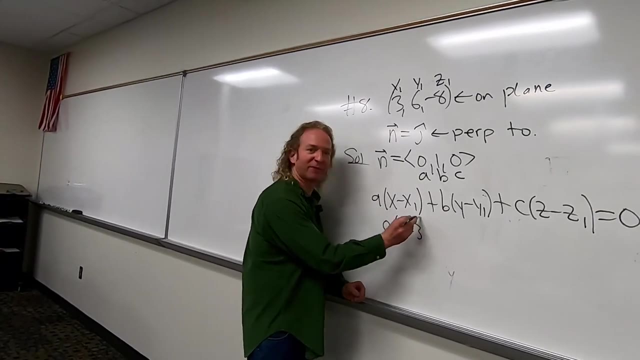 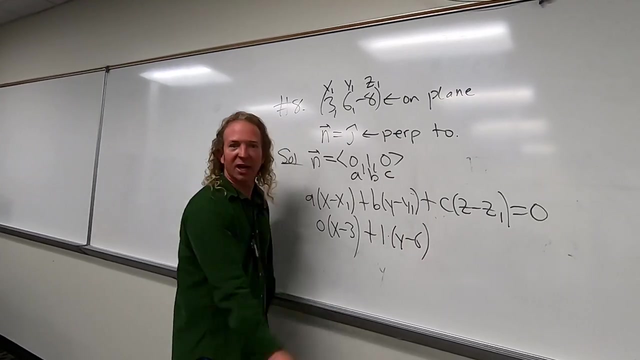 because you would get like a, x one, b, y one. good, uh, tony, no, josh, good, good, yeah, so right, okay, um, oh, so a is zero, right, so it'll be zero times x minus three plus b is one, so one times y minus six, and then c is. 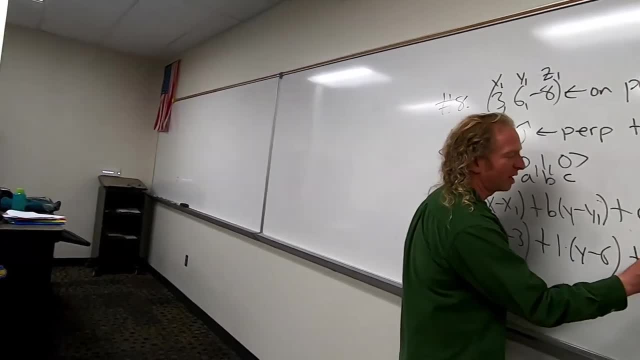 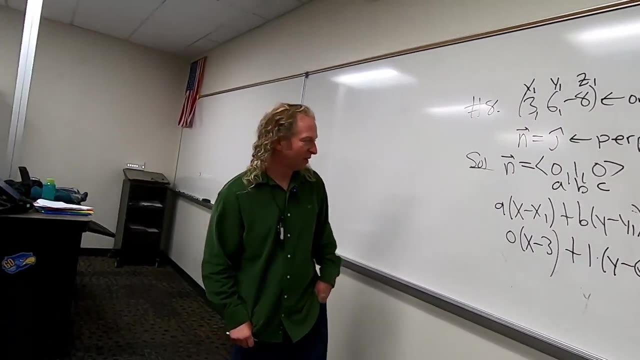 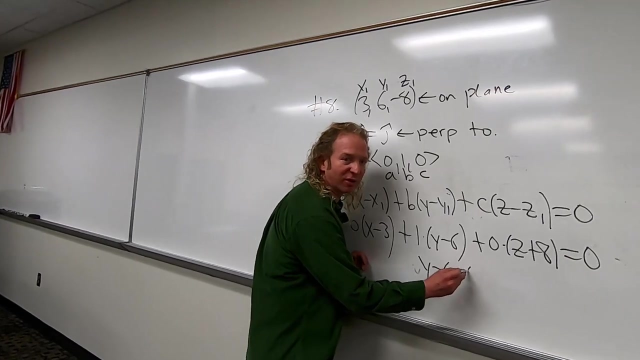 uh, zero. so zero times z plus eight, and all of that is equal to zero. so when you multiply anything times zero, you just get zero, right? so this is going to go away. so you just get y minus six equals zero. oh, that's pretty cool. so now you just add six to both sides, right? 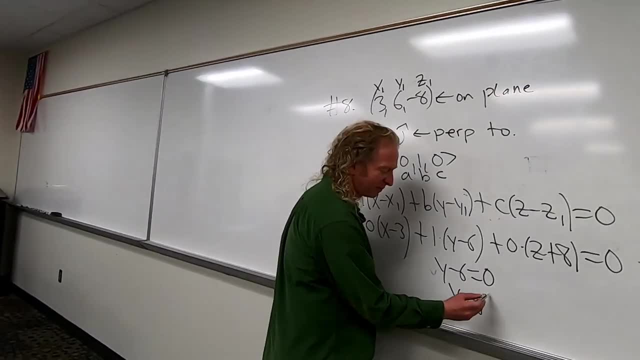 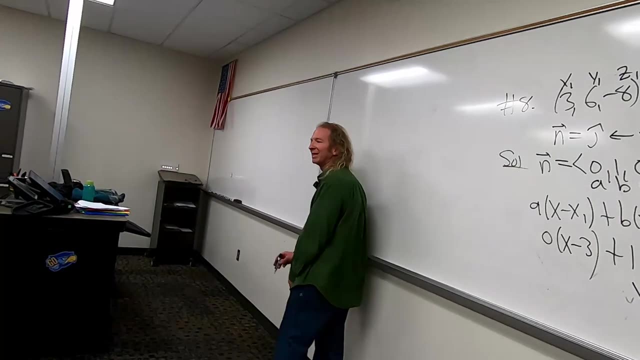 you just get y equals six. that's a plane: y equals six. you can leave it as y minus six equals zero and i would. i would mark it correct. so that's it, that's number. that's number eight, number eight from the homework. i'm going to sign in so i can look at it too. 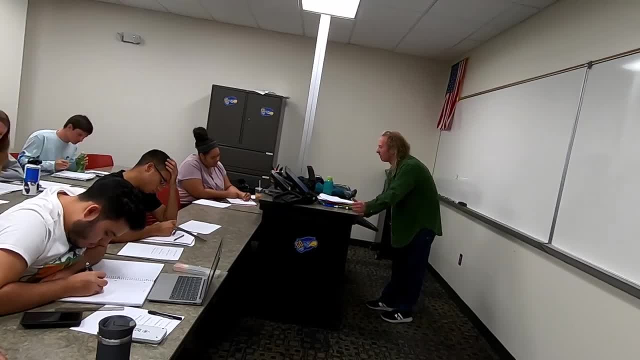 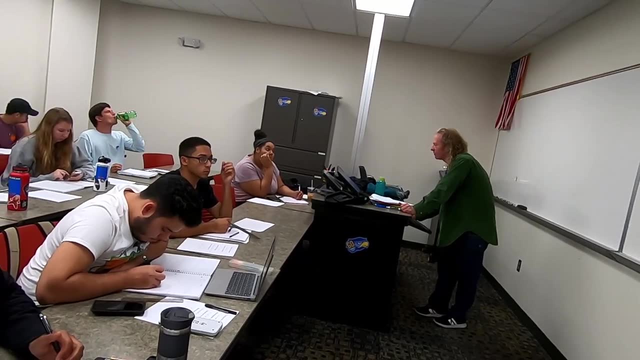 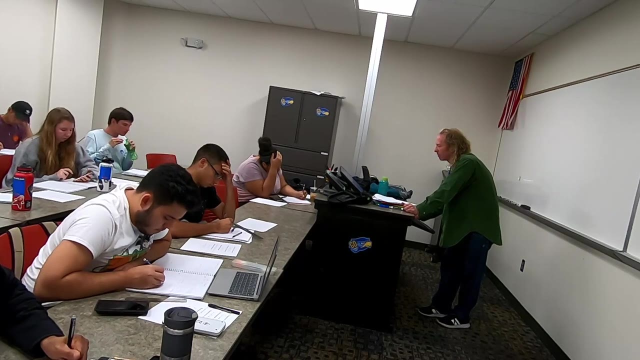 so i can read the wording. wording is really important. ah, password. any questions on that one? any questions? all right, so let's do number nine, number nine from the homework. i'm going to read it because i want to make sure the wording, the wording, changes slightly when you're taking the test. 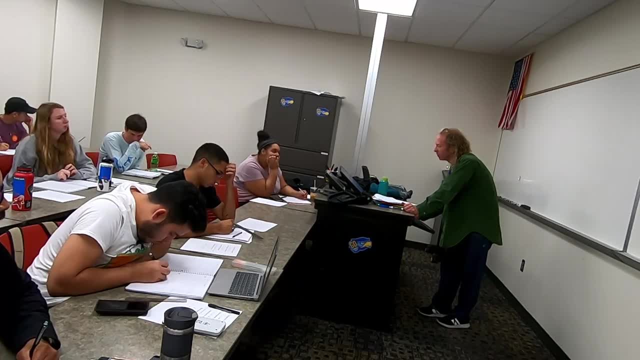 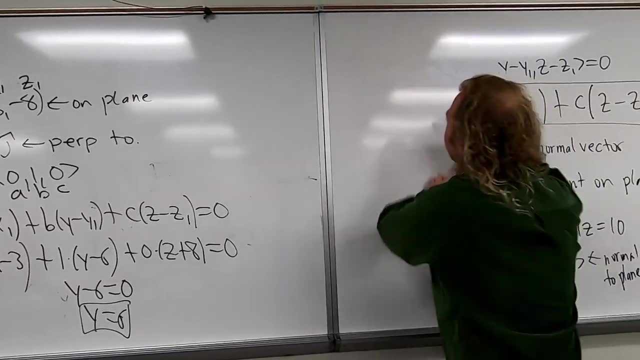 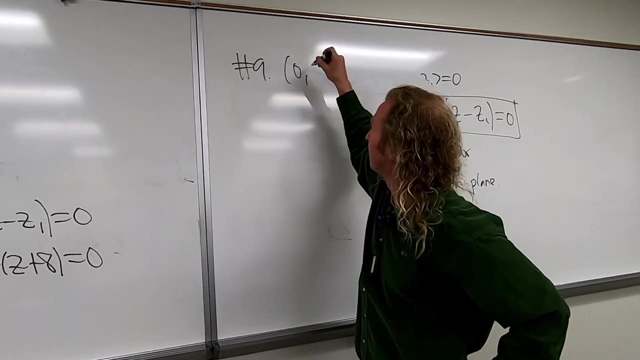 um, read the questions really, really carefully, because they'll change slightly. okay, nine is exactly the same. um, maybe we should do it, though for practice, just because we can. so number nine right, can you? can you read me the point? yep, that's uh. zero comma five comma zero. 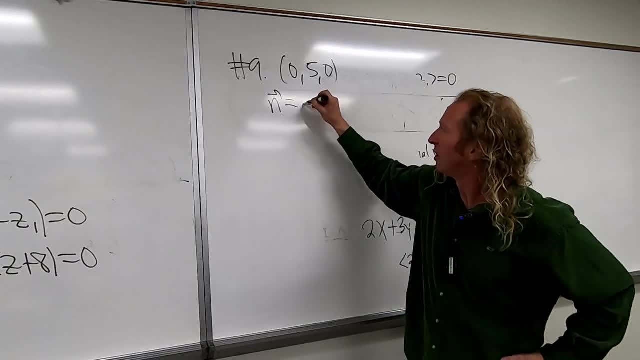 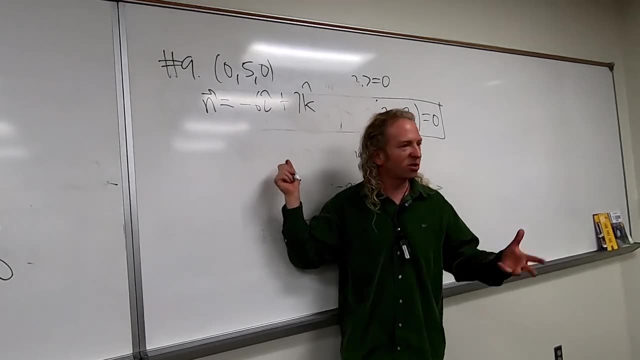 and what's the vector n equals negative six, i plus seven k like that. okay, do you all want to try this one on your own really quick, see if you can do it. yeah, try it. try, i mean, it's good one. you will have easy ones on the test too. 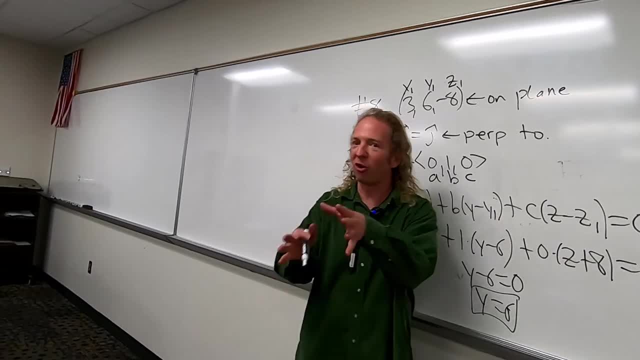 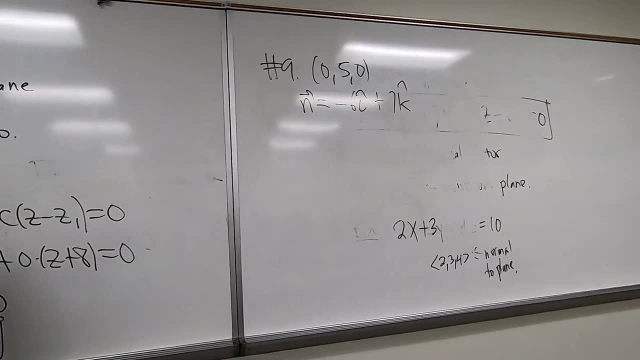 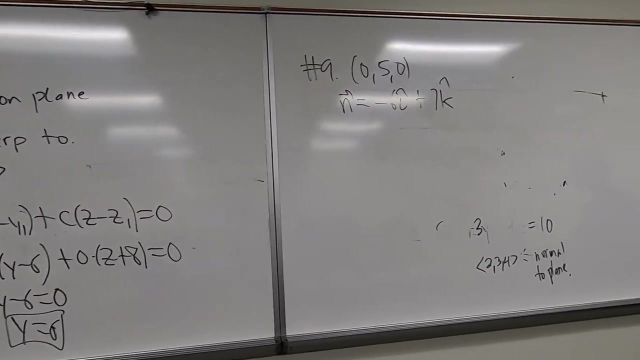 every single one is on there actually, so. so all all the varieties of the playing questions i figured you know make it interesting, just so you have all the easy ones. there's a there's a tricky part to this. maybe i don't know. it's not tricky, no, okay, well, not yet. 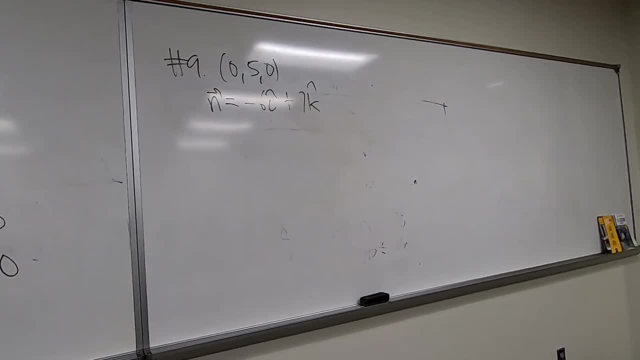 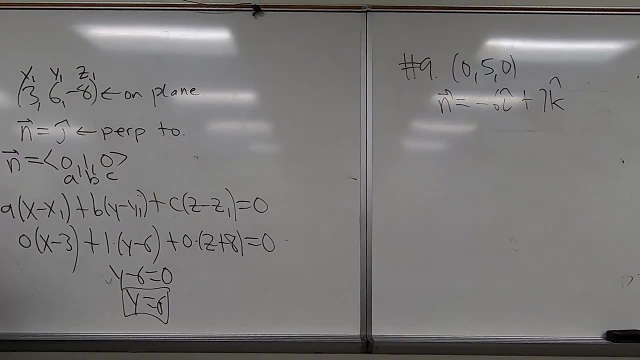 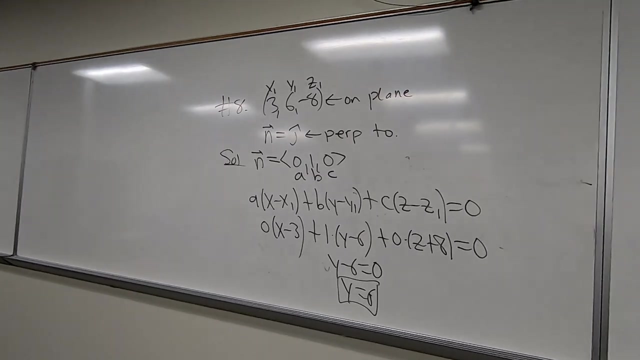 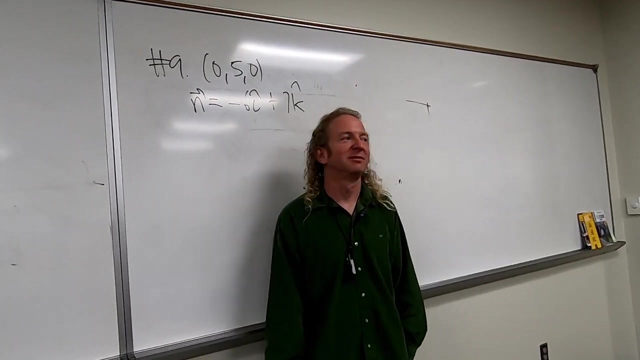 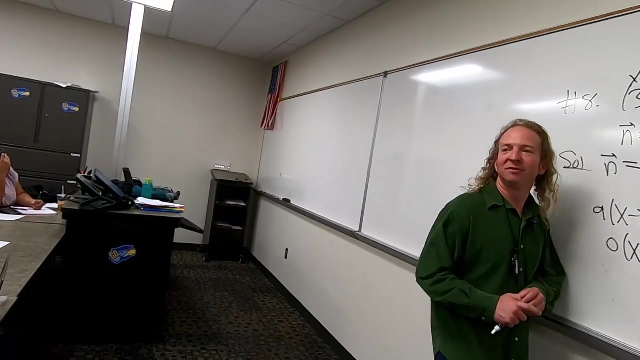 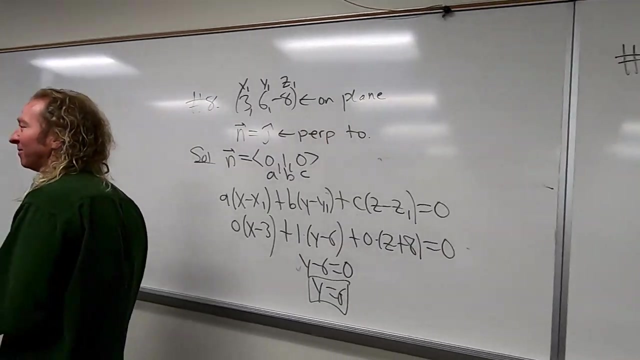 wow, it's really full in here. it's like a full class. um, it's a full class, so it's like a full class. yeah, you got it already. got it, michael? yeah, it's pretty easy so far. it does get a lot harder, like, trust me, it's like i know i said that it doesn't seem that way yet, but 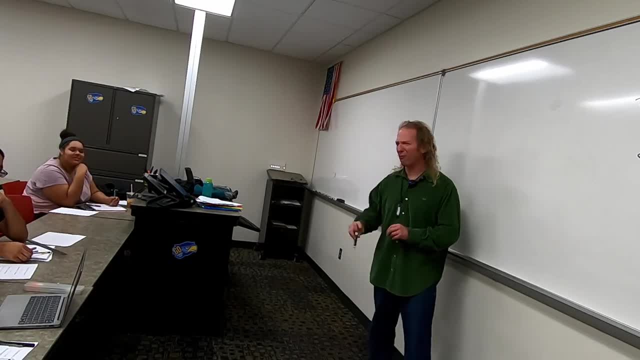 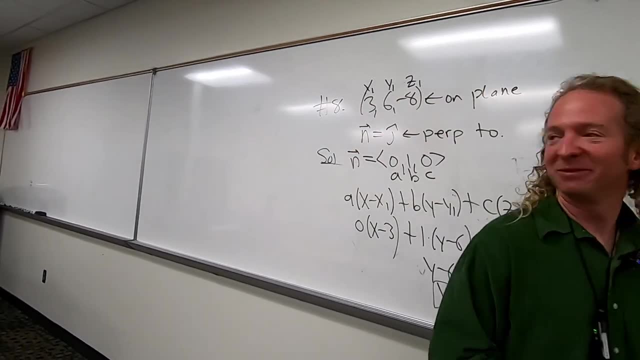 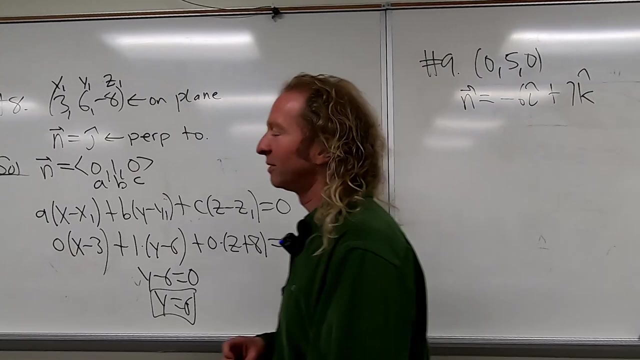 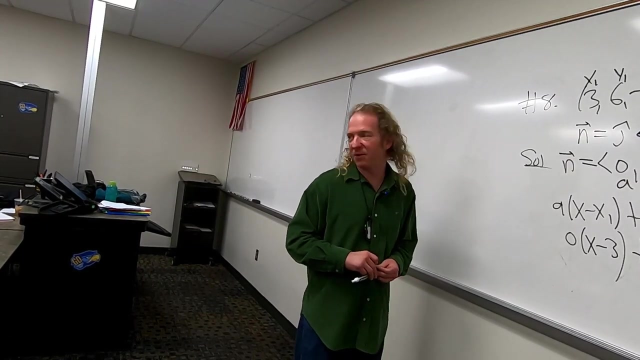 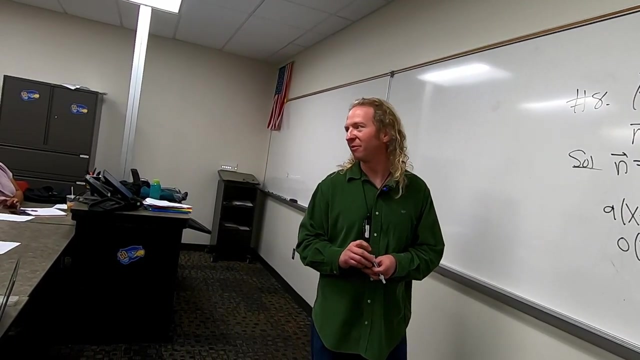 yeah, it will. oh, just wait for it. yeah, oh, totally, it's really conceptually difficult. did you all get it right? the same answer: yeah, well, it is. if it's perpendicular, yeah, that equation will be zero. yes, it's true. no, they tell you it is. this is given. 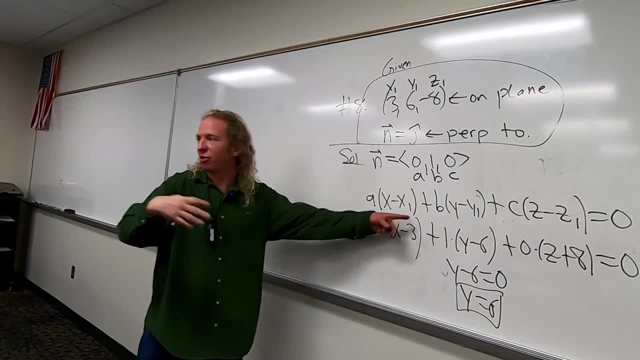 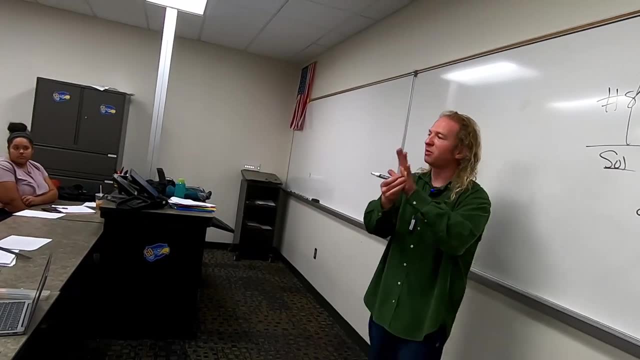 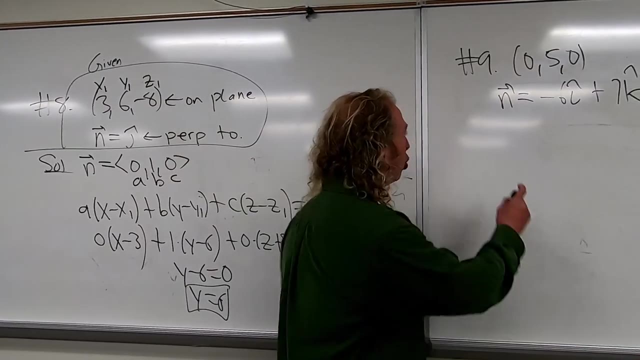 oh, for the equation to work. so, yes, yeah, yes, that's where. that's where the equation came from, right, the equation came from the fact perpendicular. yeah, yeah, that's yes. good, can I do it or I can do it? okay, solution. so the first step maybe is to rewrite n. 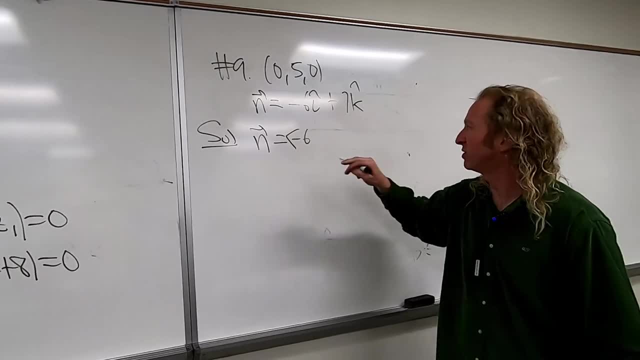 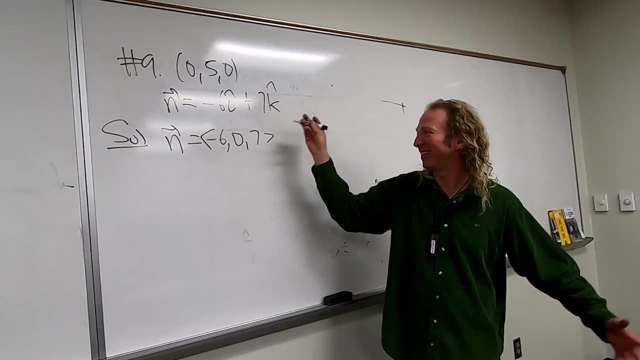 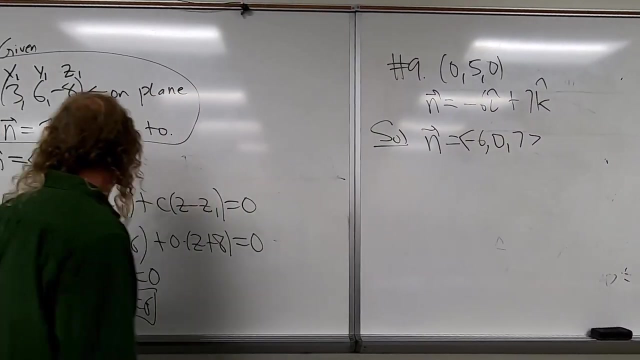 so that would be negative 6, whoa whoa, whoa, whoa whoa. negative 6: uh, zero. very good, that's the tricky part. it was supposed to be tricky. um okay, so now you just use the formula I'm gonna, I'm gonna make a leap here. 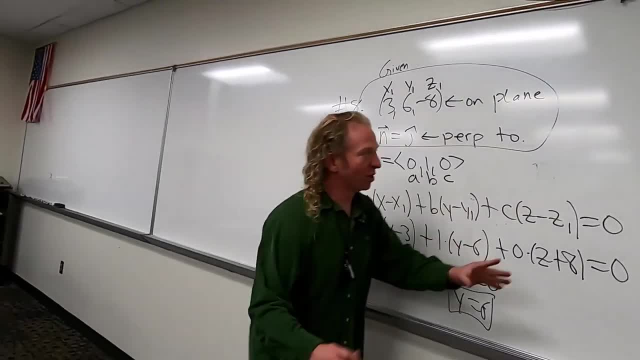 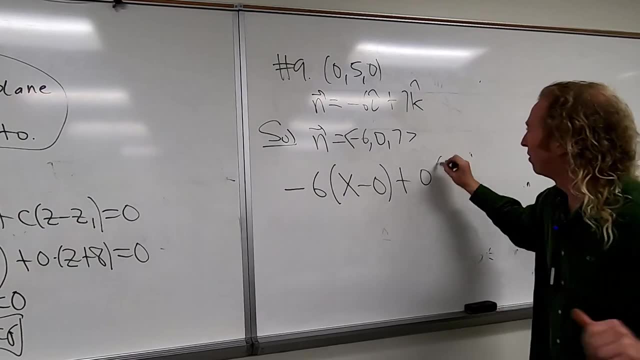 and I'm not gonna write the formula down again. okay, alright, so let's do it. so it'll be so. so, negative: 6 x minus 0 plus 0. oh, I should write these down. this is x1, y1, z1. right, that's those. 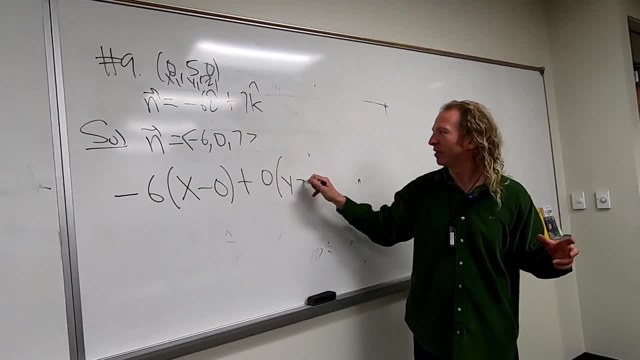 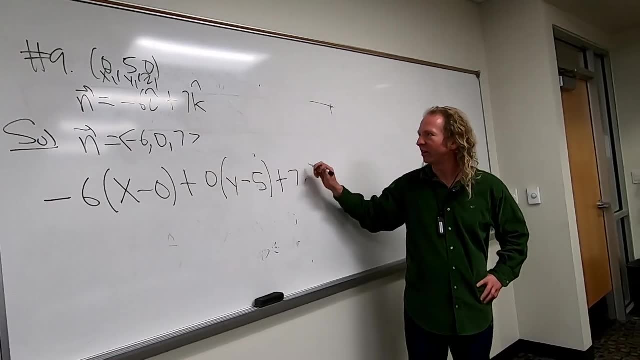 so x minus 0: 0 y1, y1, y2, y1, y2, y3, y3, y4, y5, y6, y7, y8, y9, y9, y10, y11, y12, y13, y14, y14, y15, y16. 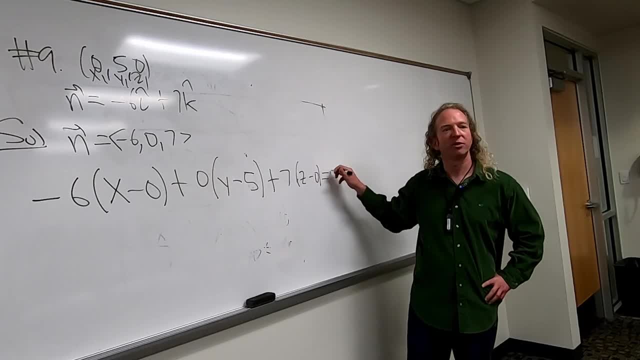 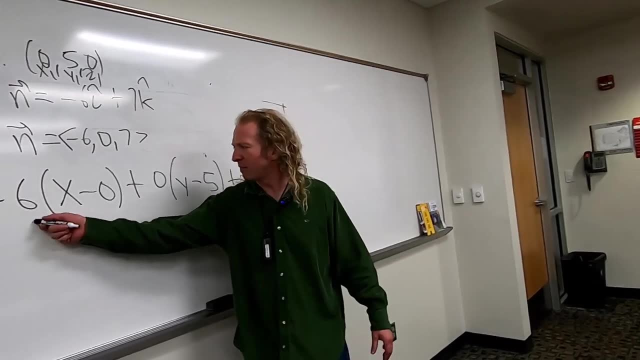 y17, y18, y19, y20, y21, y22, y23, y24, y25, y25, y26, y27, y28, y29, y30, y30, y30, y31, y32, y33, y34, y35, y35, y36, y36, y36. 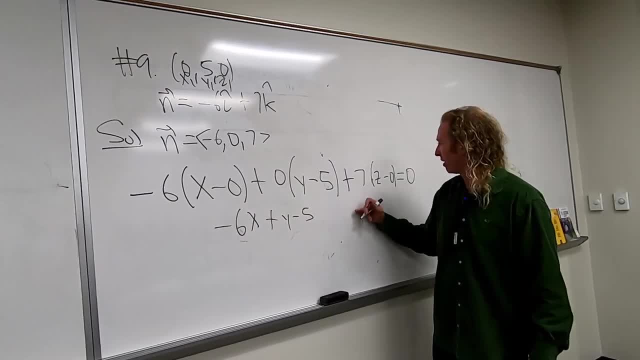 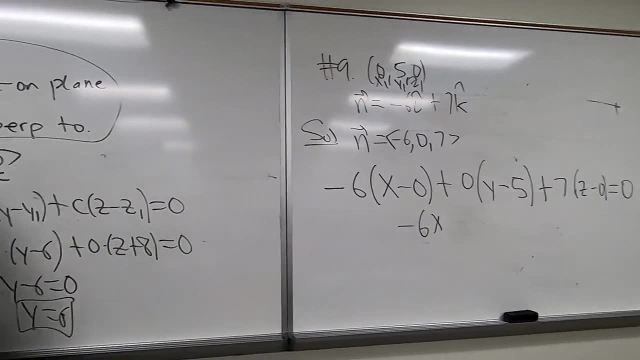 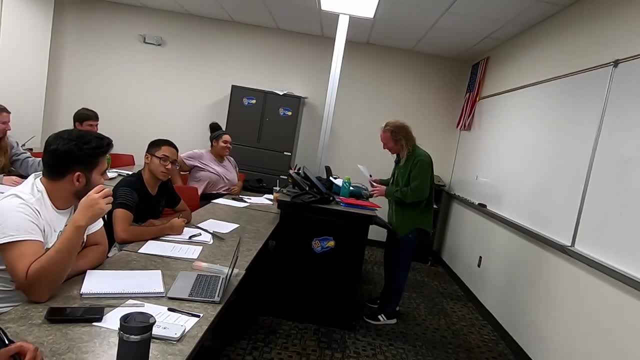 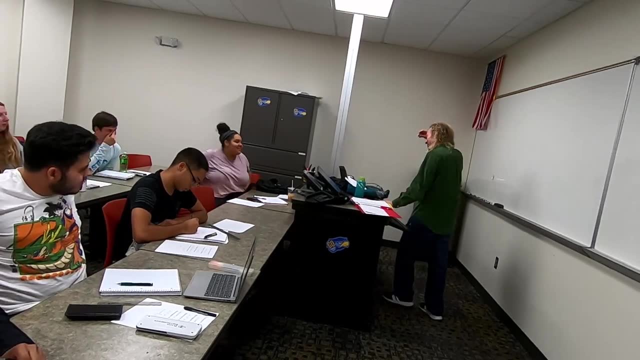 y56, y57, y58, y59, y59, y60, y61, y62, y64, y65, y67, y68, y70, y81, y71, y62, y20, y21, y23, y24, y24, y26, y26, y26, y27, y28. 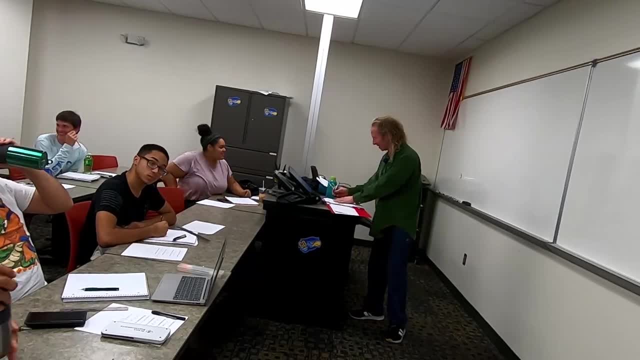 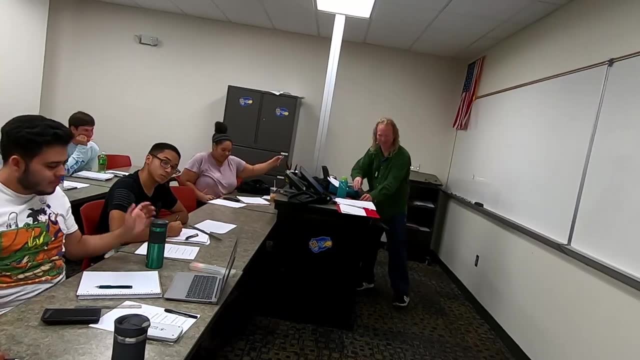 y29, y30, y30, y30, y31, y34, y34, y35, y36, y36, y45. I'm using the dummy. Is everyone looking at me? All right? So, yeah, what happens to all of this? It becomes what. 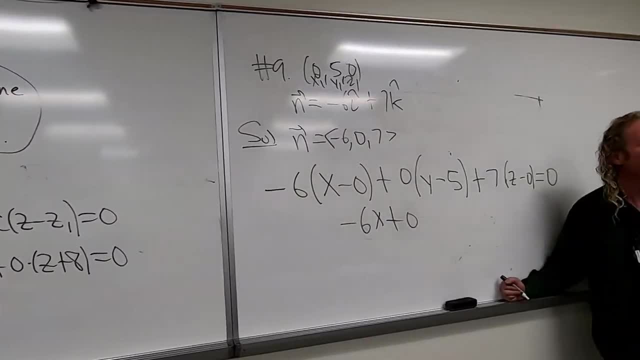 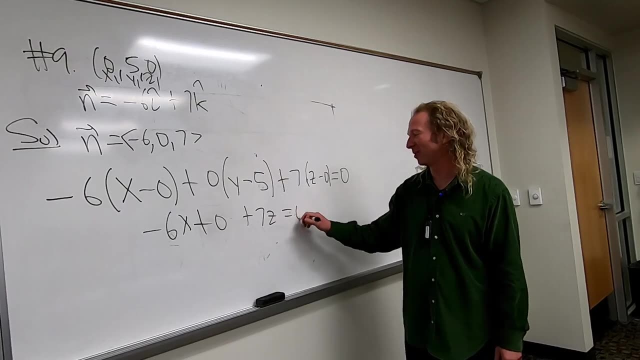 Zero. What a weak move. I can't believe I did that. You know what happened. I was thinking about something else. That's what happened, So bad. All right, that's equal to zero. Huh, This should be it. 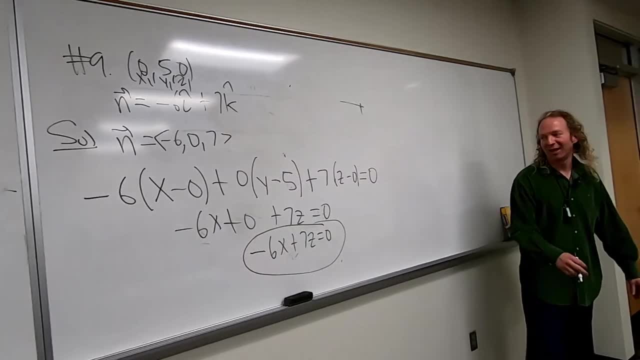 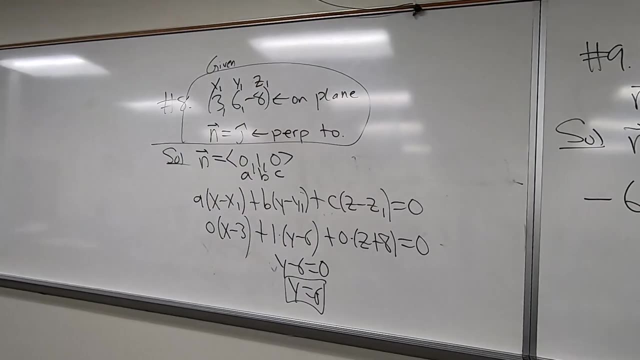 Is that what you all got? Yeah, it must be right. then, Yeah, it must be right. Okay, I was thinking about something else. Sorry, It's related to your test. I was thinking like, if you're taking the test right, 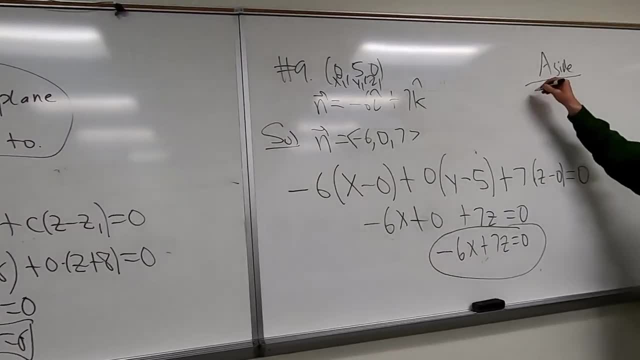 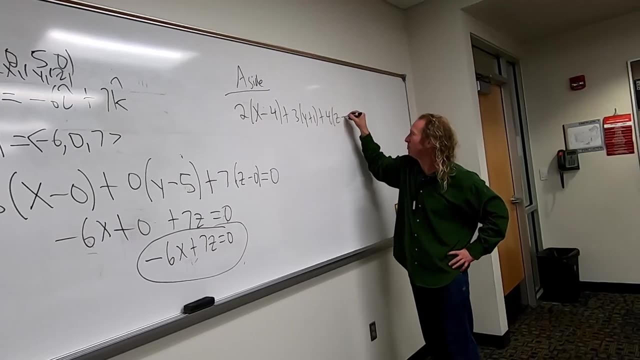 Just aside, This is important. This is what I was thinking about. I'll show you. Say you're taking the test and you get this. This is useful. Say you get this. I used to people always ask like, oh, do we have to multiply it out? 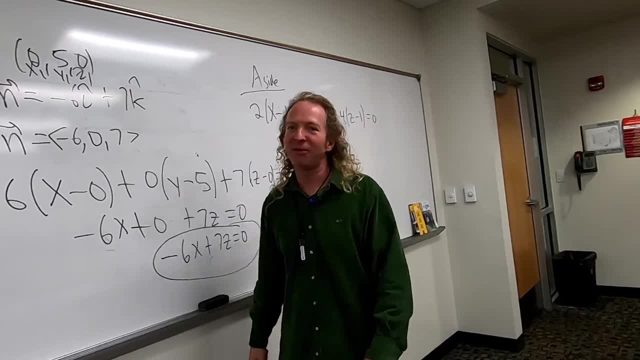 So I used to always say, yes, Oh, yeah, multiply it out. But then there's always some people who don't do it right And then I feel bad taking off points, So don't worry about it, Just leave it like that, if you want to. okay. 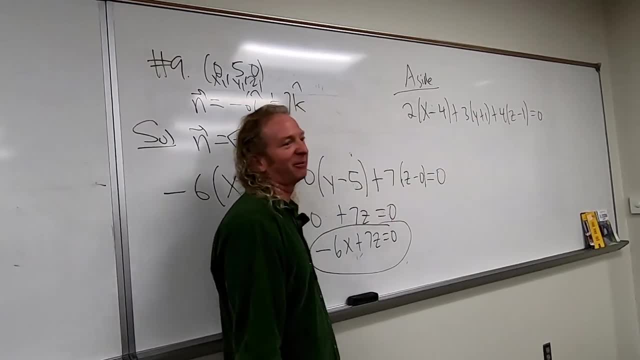 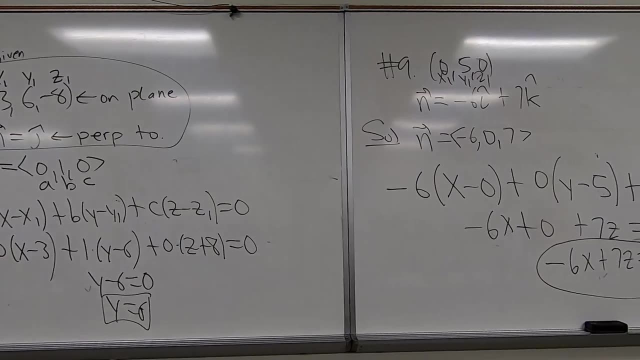 So you don't have to multiply it out. okay, That's what I was thinking about. That's why I messed up. I know right. Yeah, So will it always give you the three points and then like one vector? 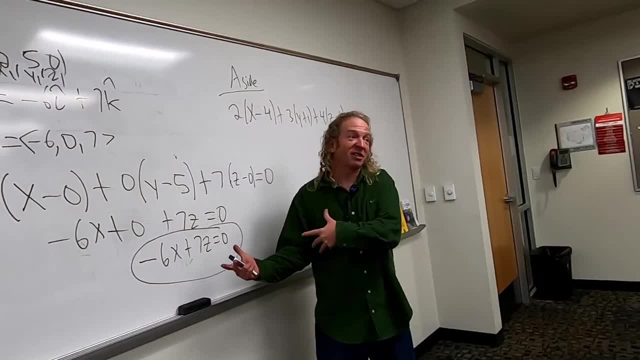 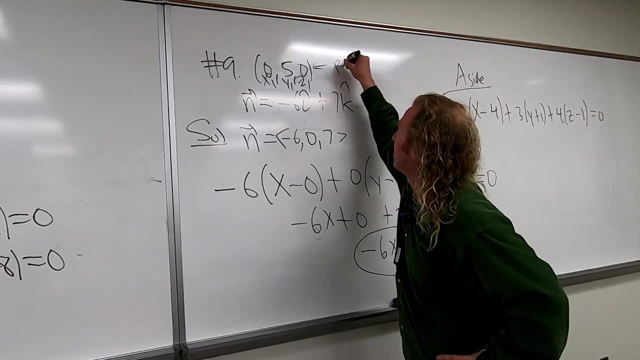 No, No, it won't These, it does. And this problem, You just know to set those first ones to X, Y and Z. Yeah, and this problem, Udash. it said this was thank you, no, thank you, Udash. 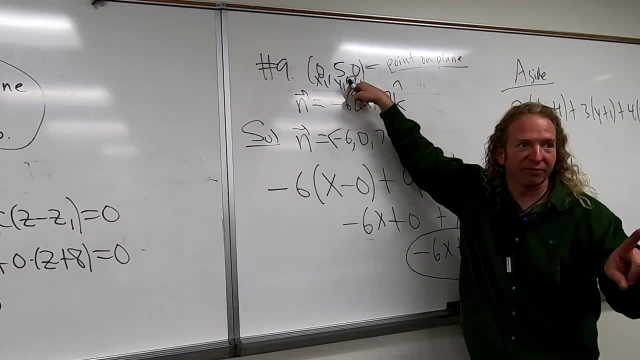 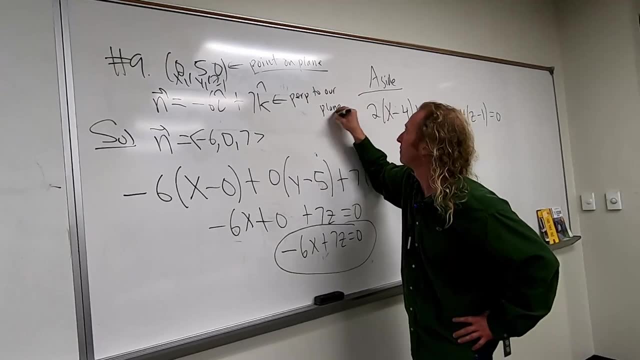 In this problem. it said that this was a point on the plane, okay, And it said that this was perp. No, it's super important, Udash. Thank you for asking, because I didn't write it. Yeah, good. 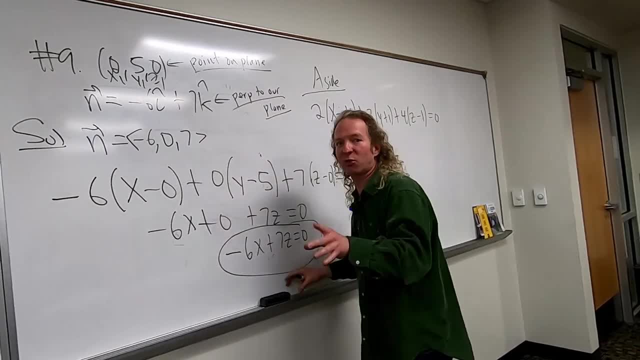 Good, Okay, so in this problem, that's what it said. okay, I think the next question is different now, Okay, good. What makes this so difficult is what Udash was asking about: is that it changes every single time. 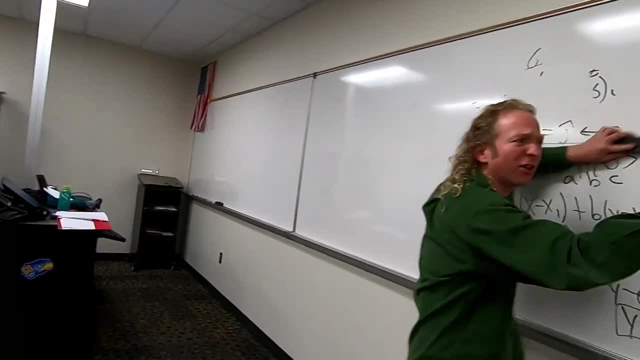 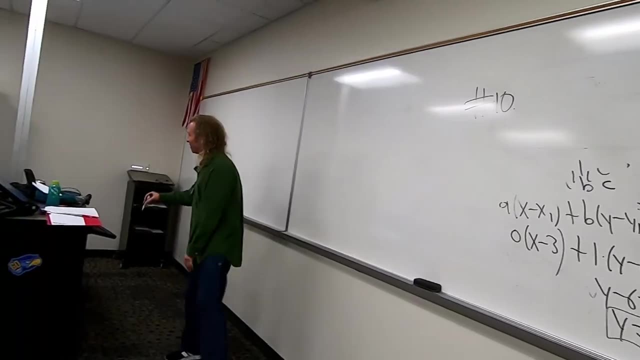 So watch Number 10, it's different, It's already harder. Hey, Anna, you made it. Oh good, Number 10.. Number 10.. Oh, exciting times. 8,, 5,, 5.. Yep. 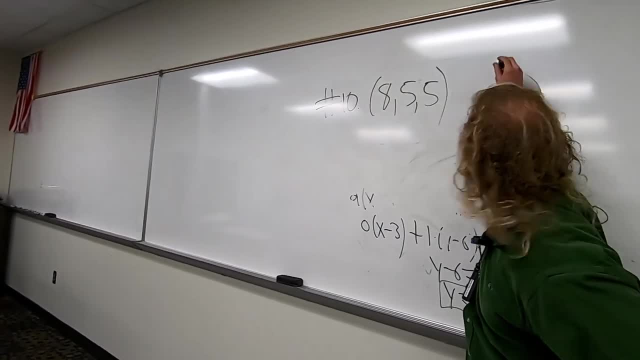 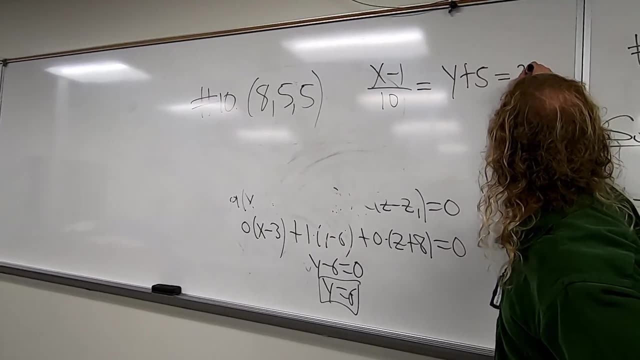 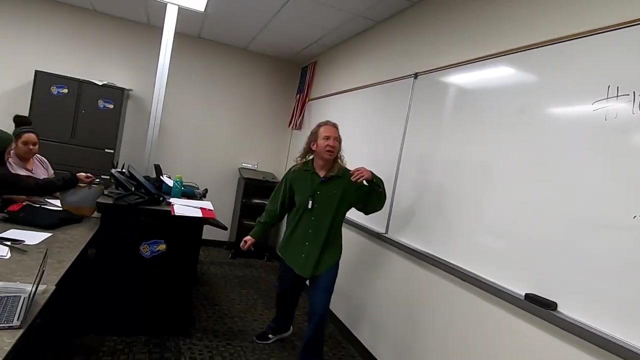 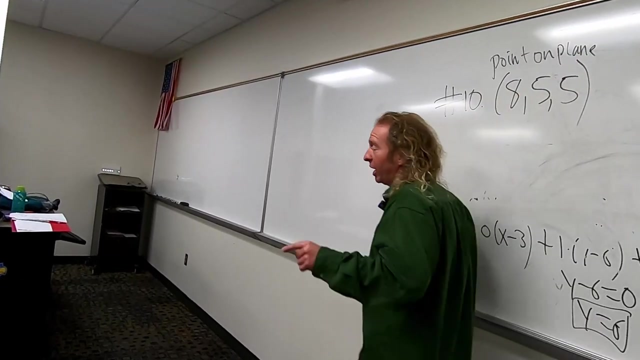 And can you read me that equation? Yeah, that's minus 1 over 10, equals y plus 5, equals c plus 8 over negative 8.. Okay, So it tells us some stuff. It tells us that this point is on the plane, okay. 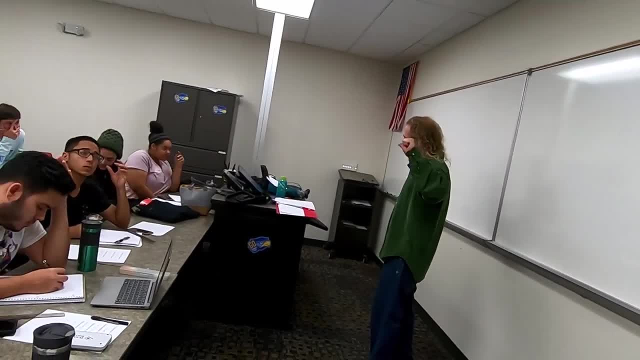 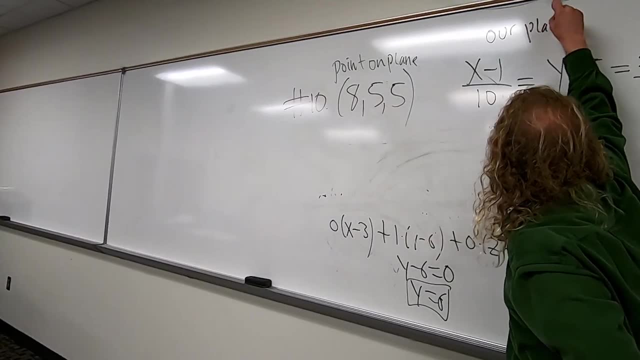 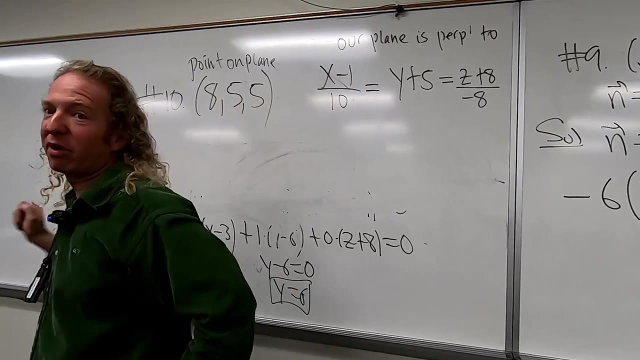 And it tells us. it says: find an equation of the plane that passes through the given point and is perpendicular. So it's perpendicular to the given line, So our plane is perp to this line. okay, Let me pause here and let you catch up. 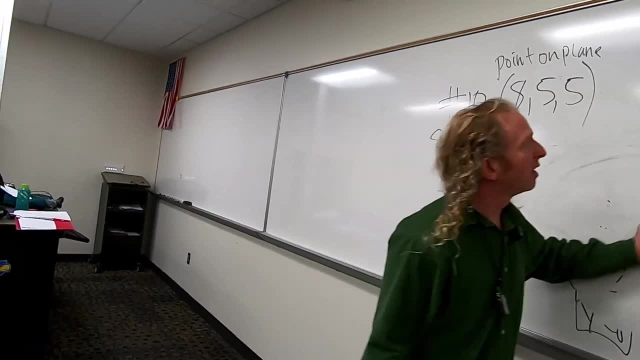 I'll let you write it down And then we're going to go. Huh, It's a 5.. It's a 5.. Someone else asked that. this morning in my Calc 1 class They gave me a tip for writing 5s. 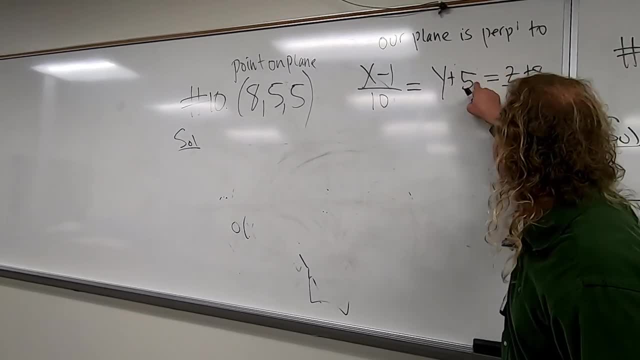 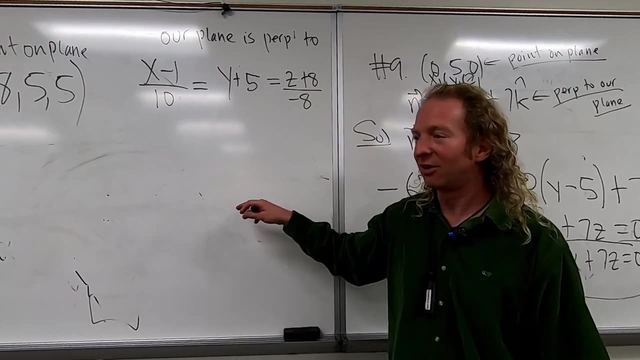 They said to do this. They said: do this and then do that. I don't know, Don't do that, Just do it straight. I don't know, I don't know, I don't know. What do you mean? Just go right to left. 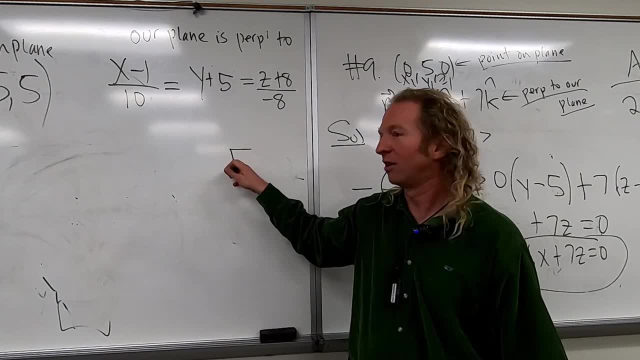 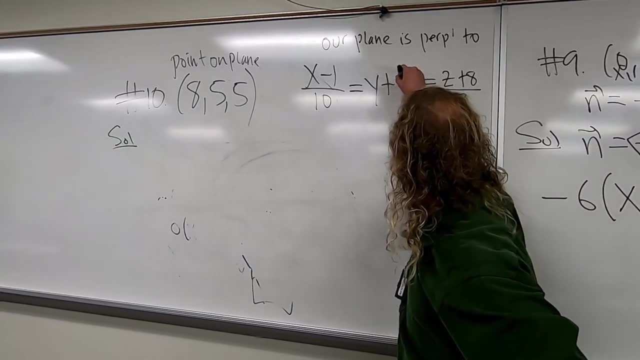 Just do a straight line, Accentuate the curve, Bring it up. Okay, All right, Here we go. Here we go, Here we go. It's about the curve. We know it's a 5. There you go, Woo. 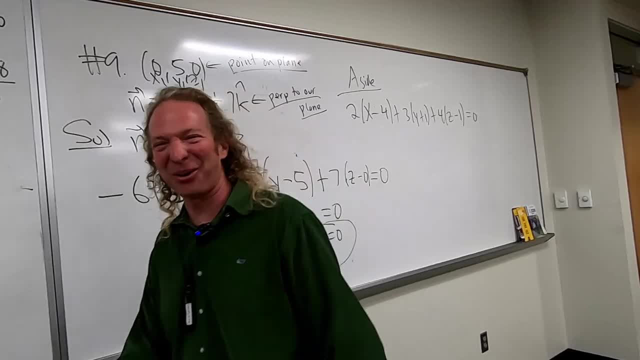 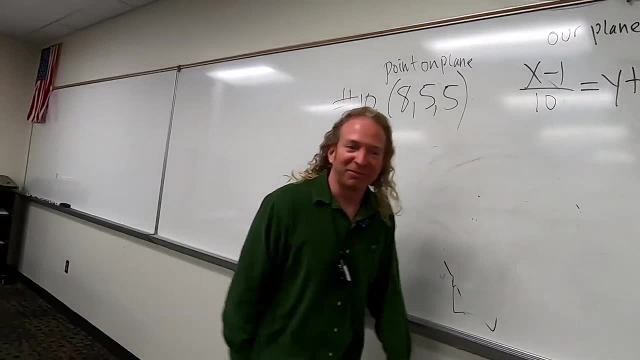 That takes a lot of work. Oh, okay, Yeah, Wow, Yeah, those are 5s too, But okay, I'll let you write it down. This problem is harder because what Udash was asking was very important, So let me just recap what Udash said. 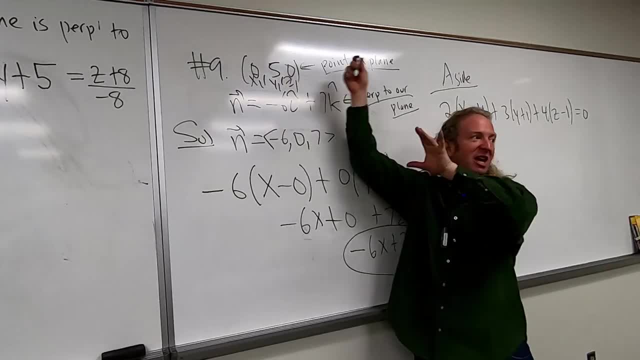 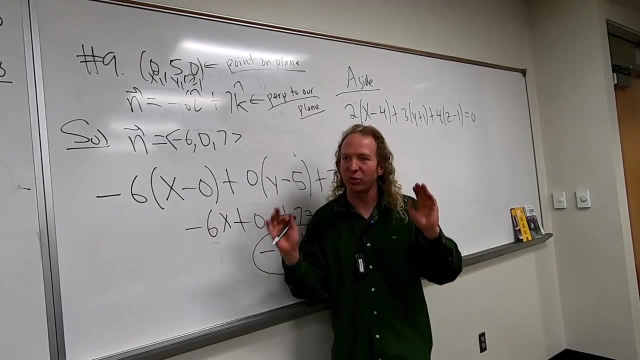 In the previous question, they gave us this point on the plane and they told us that this was perpendicular. Whenever that happens, you're good to go right, Because all you need is a perp vector, A point and a perp vector, and you've got it. 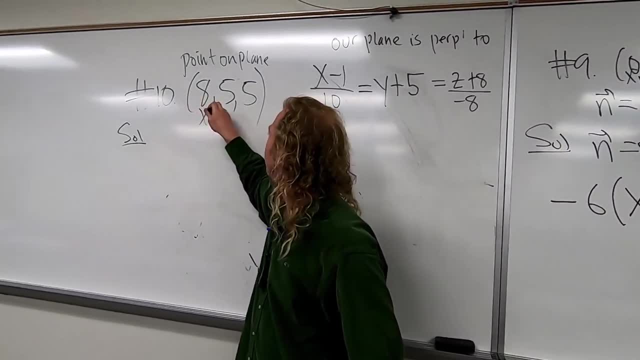 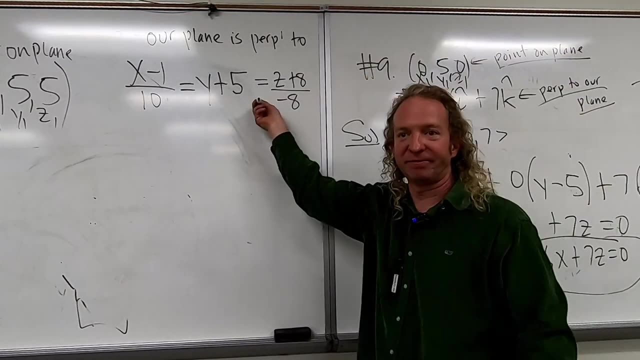 Okay, This one. we've already got the point, So we know that's x1, y1, z1.. And I actually don't know how to do this problem yet, so I have to think. So our plane is perp to this line, right? 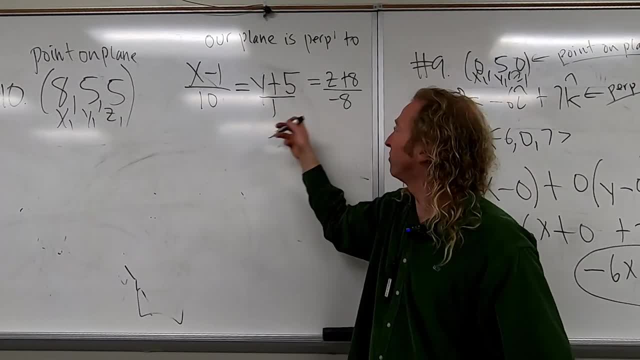 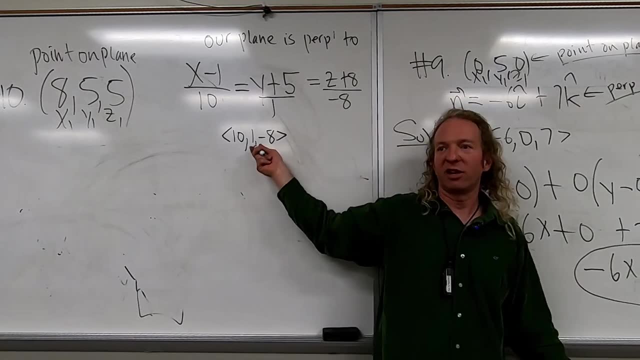 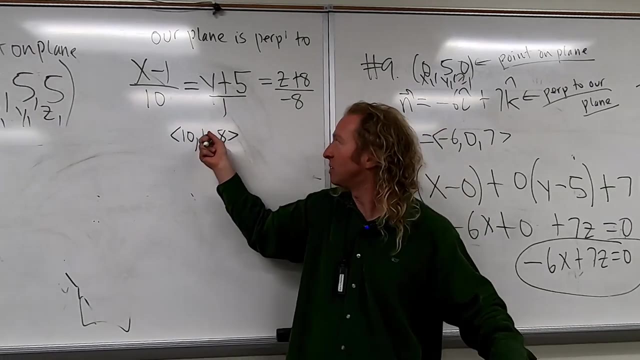 There's a vector here: 10, 1, negative 8.. 10, 1, negative 8.. This is called the direction vector. This vector is parallel to this line. Remember from last time. So this vector is parallel to the line. 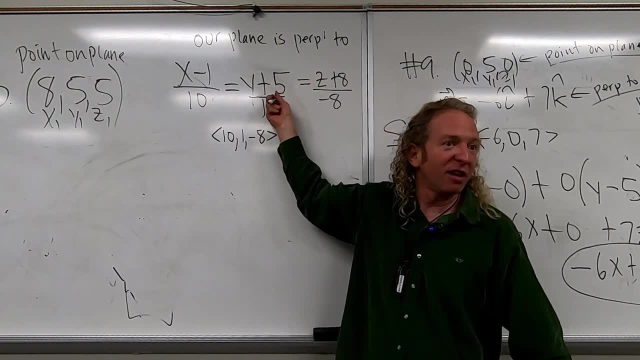 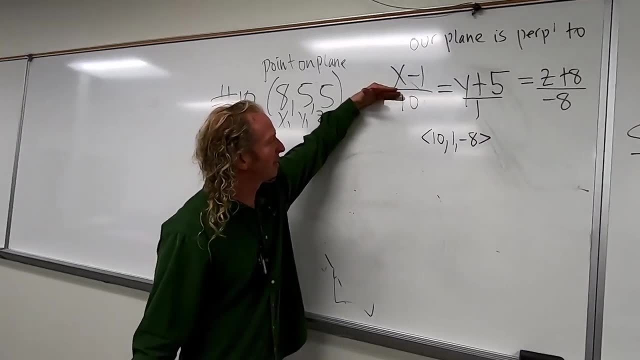 Okay, Our plane is perp to the line. Therefore, our plane is perp to this vector. Let me explain that again. So this line Is parallel to this vector. So they're parallel, right? So let's say: this is the plane. 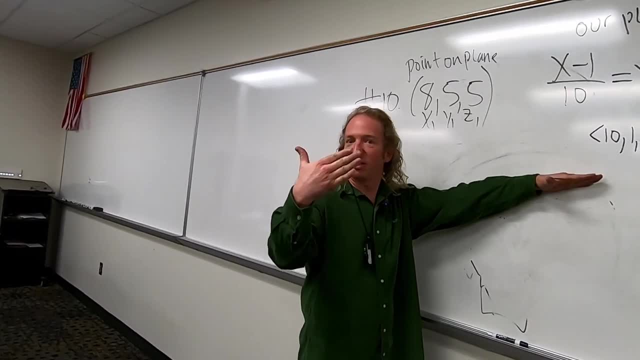 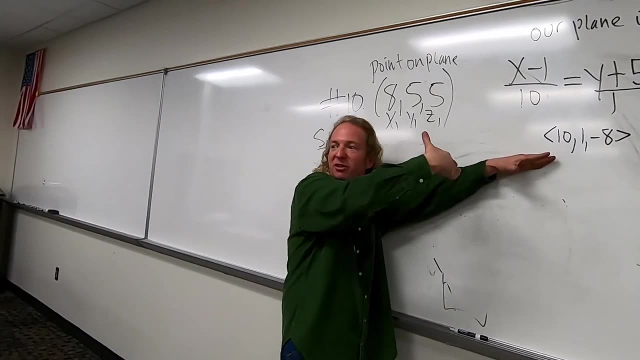 And let's say: this is the line right. So the plane is perp to the line right, But this vector is parallel to the line. That means the plane is perp to this vector. Okay, So the plane is perp to the vector. 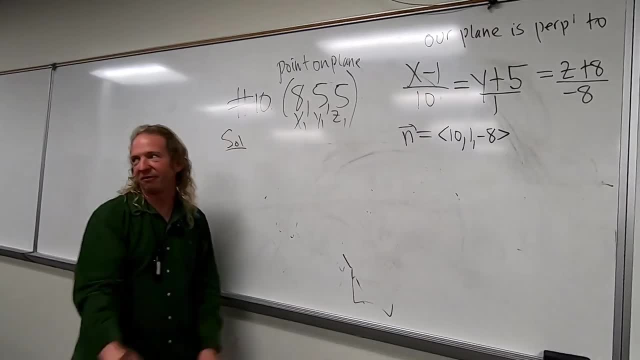 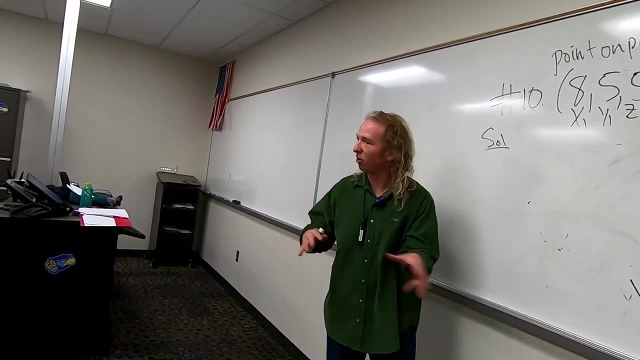 So that's our normal vector, That's our n Deep right. So it requires thinking, which is why I love this stuff. right, And they're all different. right, They're all different In the previous problem, they just gave it to us. 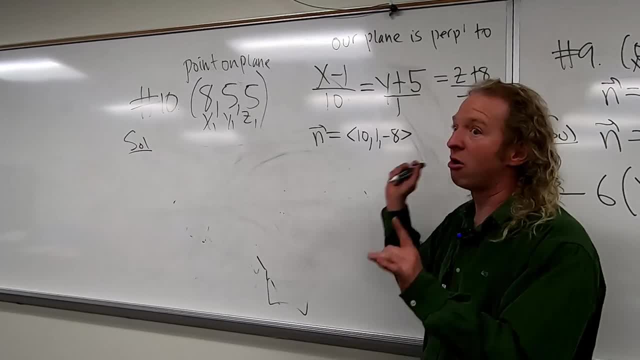 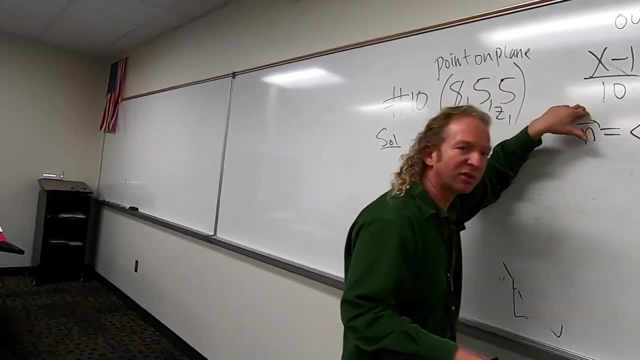 So you may be saying, oh so anytime they give us something like this, it's always going to be that. No, It depends on what the question says, right? The question is saying that our plane is perpendicular to this. So, because this is parallel to this, 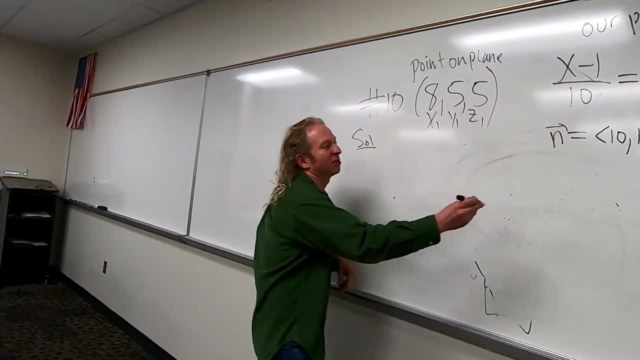 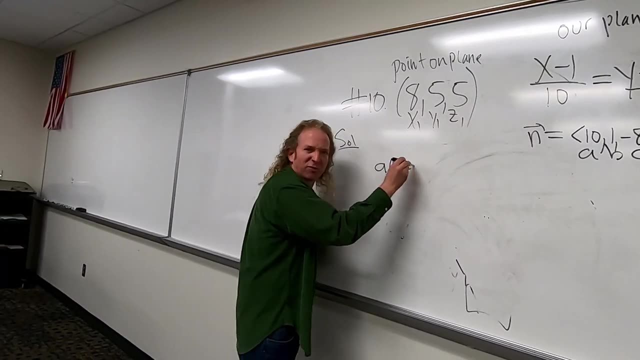 our plane is also perpendicular to this. So now we're good to go. So this is our ABC. It's beautiful, It's math, So I'll write the formula down again this time, just because I feel like this problem deserves it. So A x minus x1.. 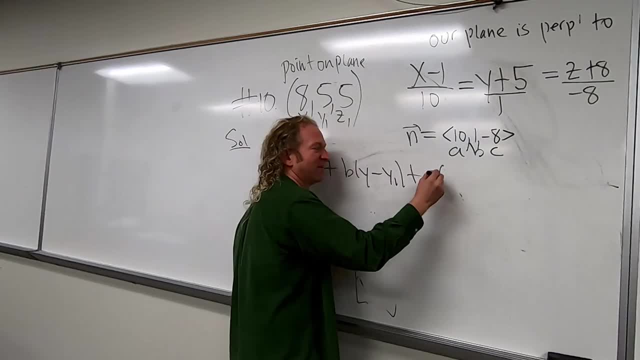 And I don't want to mess up anymore. Those days are gone. Never going to mess up. I'm going to mess up again. This is it Not never. We'll see So double points next time. That's fine, OK. 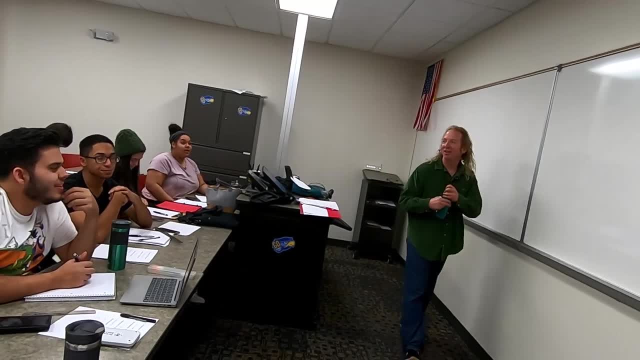 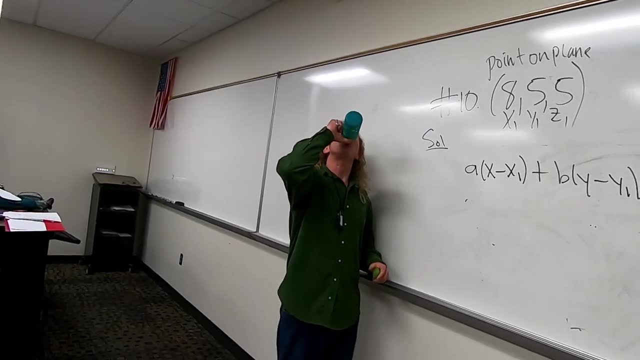 We can do double. I'm not going to mess up, It's on. All right. Double points, Let's do it. Let's do it. Double points. Yeah, You got it. It's challenge accepted: Double or nothing. 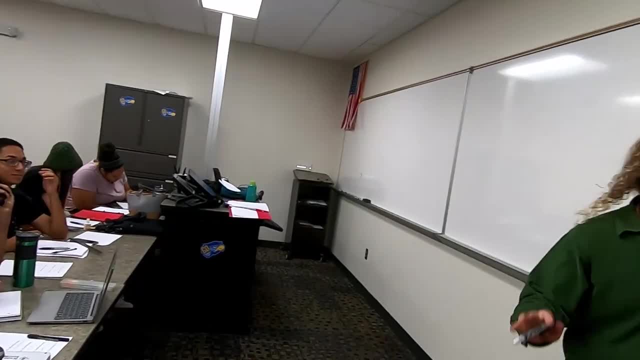 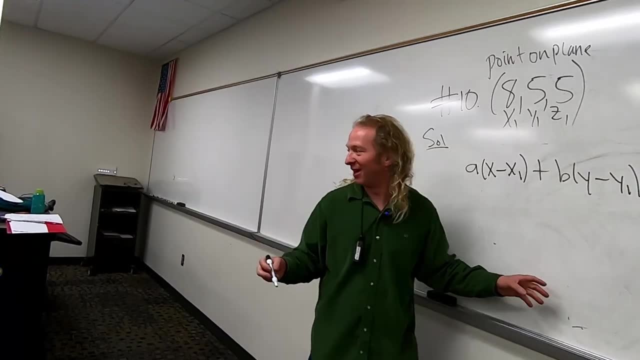 Oh yeah, I know I'm a really bad gambler, But I'm not going to lose. Calculus, not a statistics teacher. I actually do teach statistics. so yeah, I've done a lot of stats. So 10, x minus 8.. 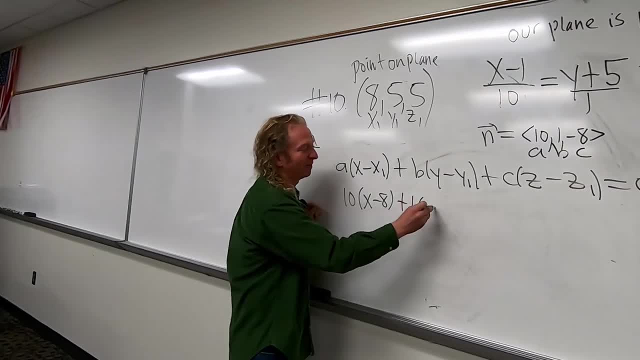 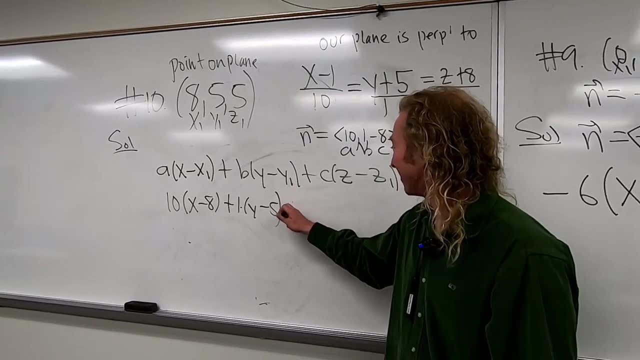 The first stats class I ever taught. a student from that class just came to see me like just now. Yeah, it was really creepy. I know it was really creepy. Yeah, I was like, oh my God, I couldn't believe. I was like, oh, z minus 5 equals 0. 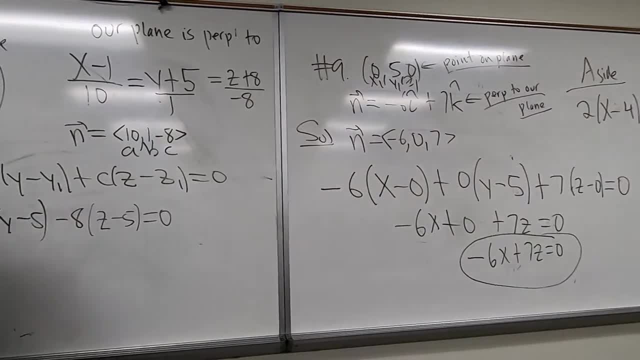 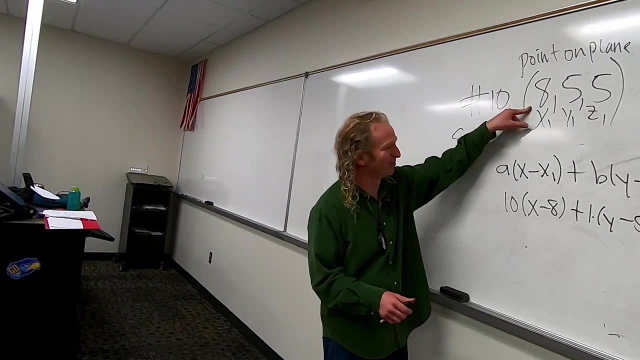 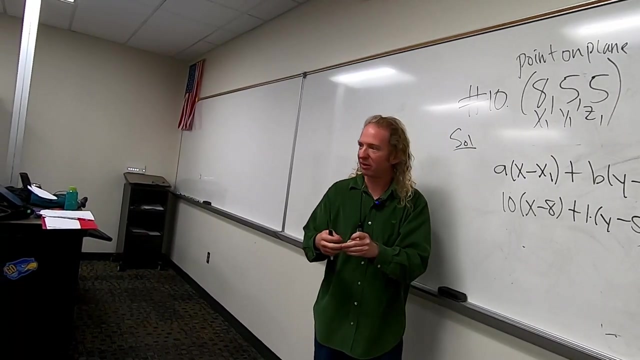 There's an easy way to never lose at casinos. right, I shouldn't tell you this. I'll have to delete this. You always triple your bet, right? Huh, Then you lose. But if you do the math, if you always triple your bet as long as you win, double when you win, you'll never lose mathematically. 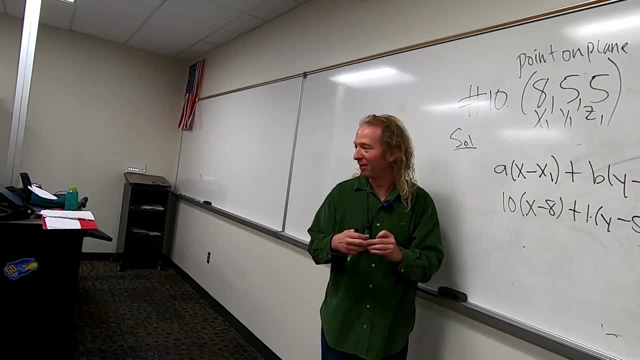 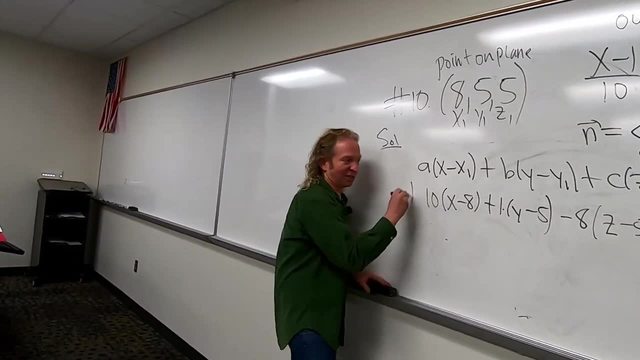 This guy I used to work with taught me that He was really shady. Huh Well, eventually you will win. right? If you have an infinite amount of money, eventually you'll win. Okay, so let's just leave it like this. 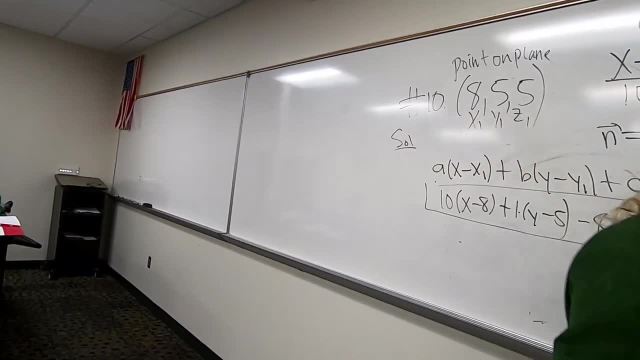 That's it. Let's just leave it like that. Yeah, you can take a bunch of pennies and try it Like: okay, bet three pennies and then you lose. So triple your bet, Bet nine pennies, you lose. 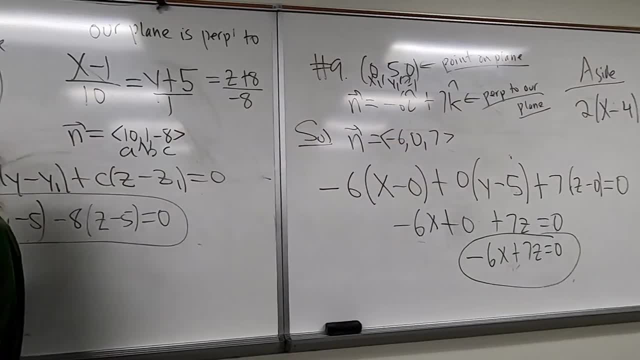 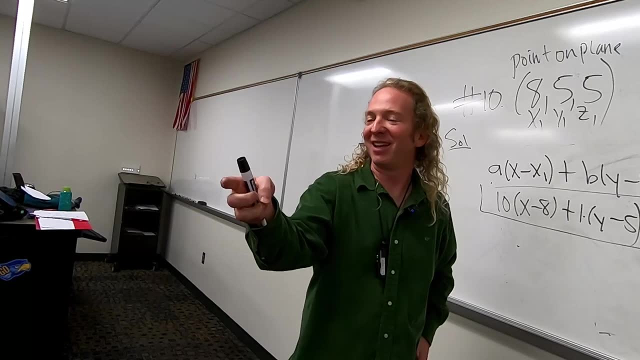 Triple your bet, Bet 27 pennies, and then you just keep doing it And then when you win, you win double and the math works out and you always end up winning. I think What's that? No, you need to have real money. 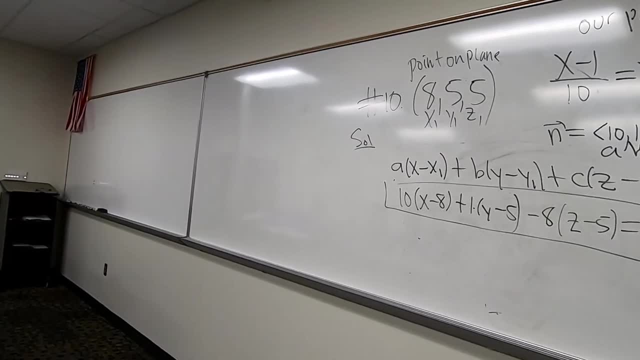 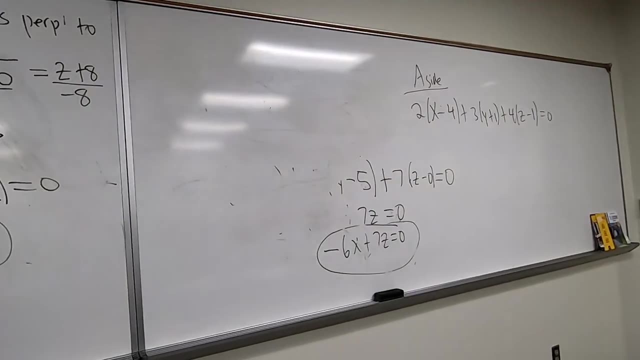 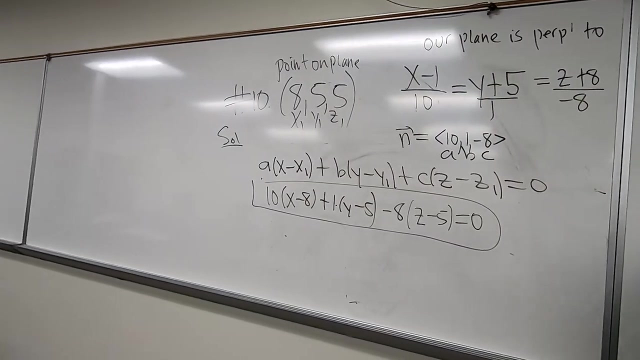 Yeah, No, and they have limits at tables, right, Don't? the tables have limits And they check for stuff like that. But I think they kick you out. so if you get caught doing that, There was a movie where the guy was like 60 or 70,000 dollars in the hole from doing that. 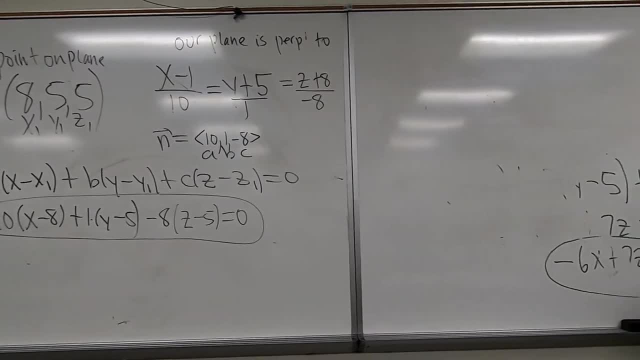 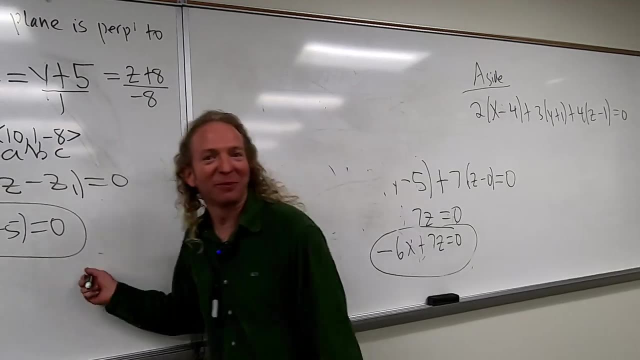 Really, Was that Rayman? No, Rayman, He won. No, no, no, He cheated, Cheated, He cheated. well, Any questions on this one? All right, let's do 11.. Keep going. Let's keep going. 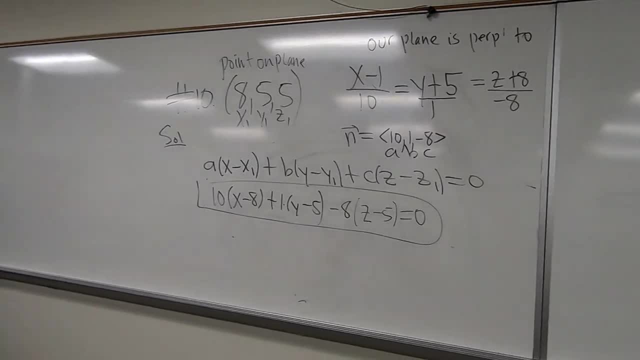 11.. Oh, I like 11.. 11's not that hard, but let's do it. We should do it because it's probably going to be on your test, Number 11.. Do you want to take this answer though? 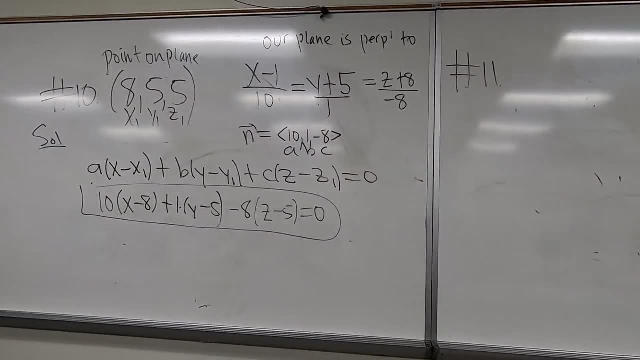 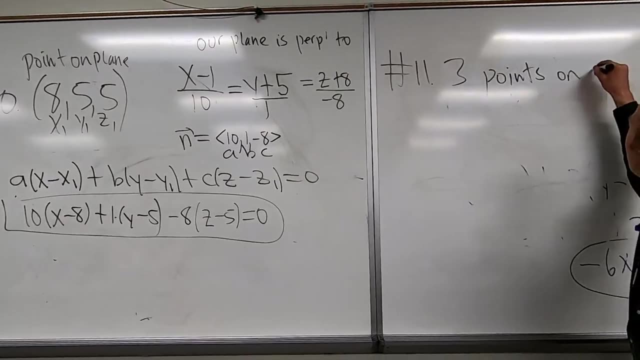 Try it. Try it Only when we find out right. So 0, 0, 0.. So we have three points on the plane, in this case Three points on plane. So we have 0, 0, 0.. 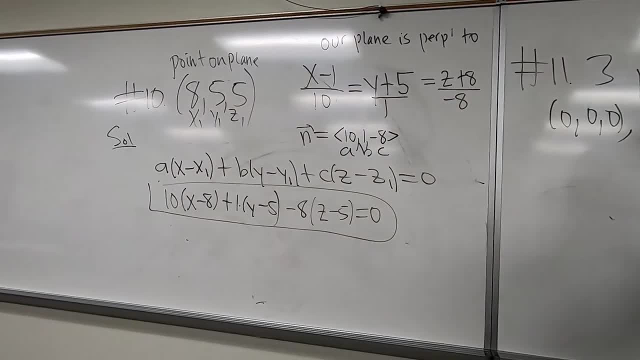 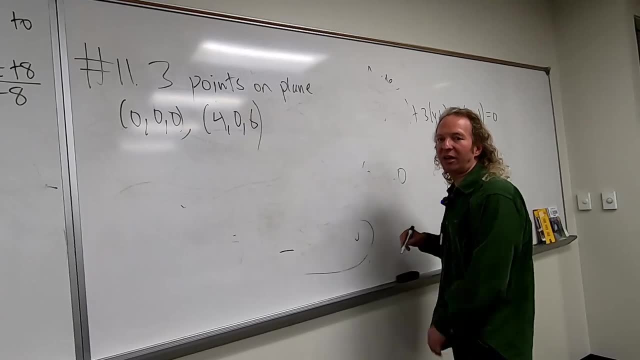 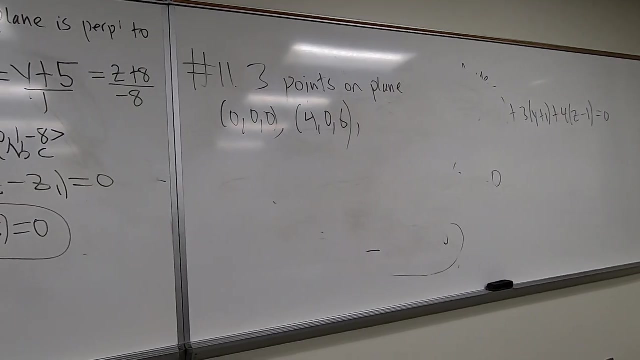 4, 0, 6.. This one's pretty easy, I think, compared to some of the ones that are after this. And The last point is negative 3, negative 1, 6.. Negative 3, negative 1, 6.. 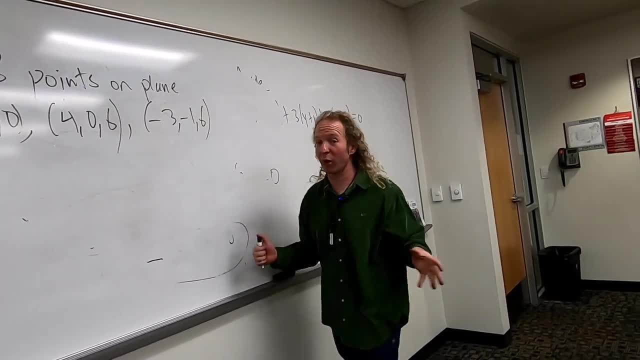 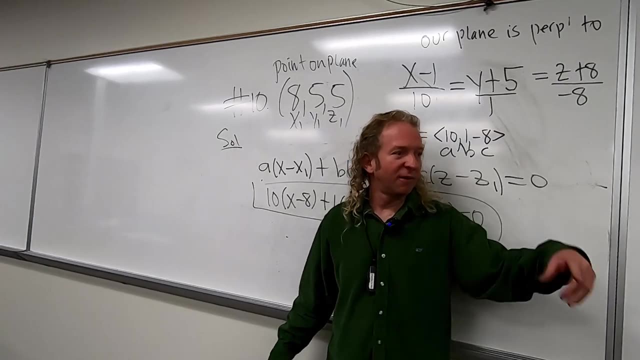 Okay, so you have three points on the plane. We have to find the equation of the plane, Any ideas? It's kind of a hard Terminus initial. What's that going to give us A vector? That's what? Parallel. 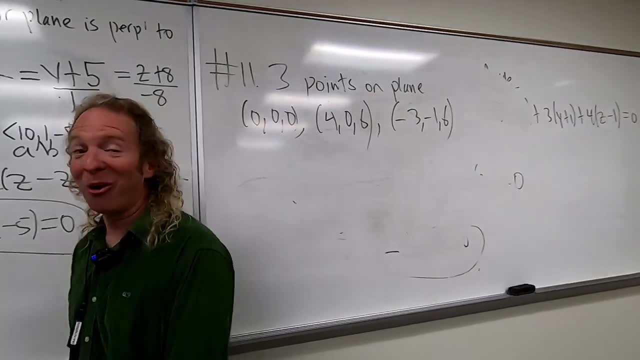 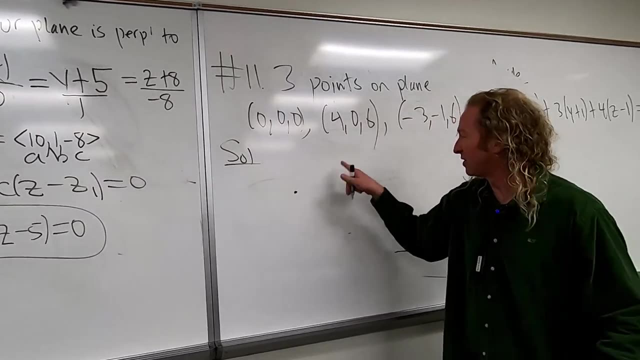 Parallel Mm-hmm. Okay, Okay, all right. So I'll just tell you: Okay, So solution, So good idea. So okay, Here's the idea. So you have a point here. Say: this is the plane, the board. 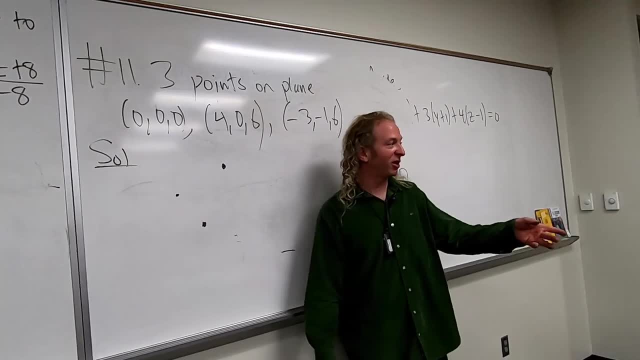 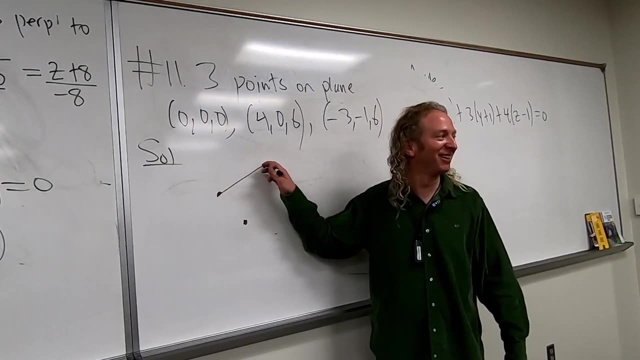 You have a point here and you have a point here. Okay, So, given two points, you can do what Samantha said And find a vector right, And then you find another vector. So you have two vectors on the plane. 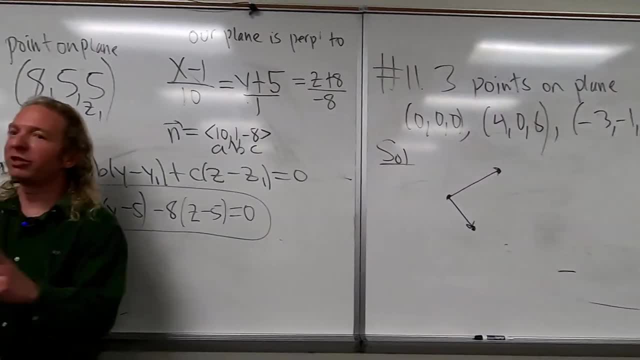 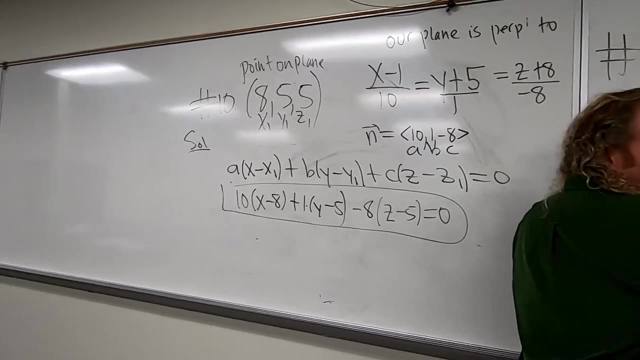 If you have two vectors on the plane, how do you get a vector that's perpendicular? What do you do? You take the y. What's that called Cross product? Very good, So you can use these to find two vectors and take the cross product. 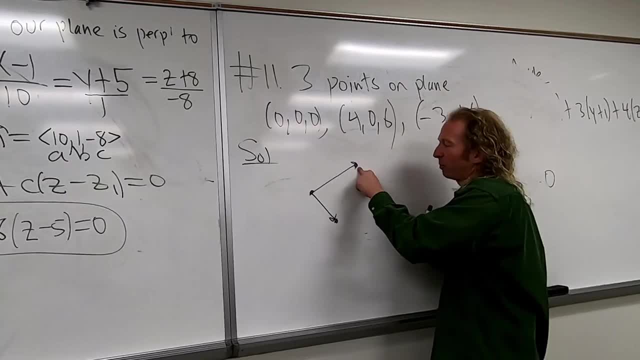 Right, Super simple. So you have three points on the plane. So do terminal minus. So just find two vectors on the plane, Find the cross product and that's your n. Could be any two, right, Yeah, any two. 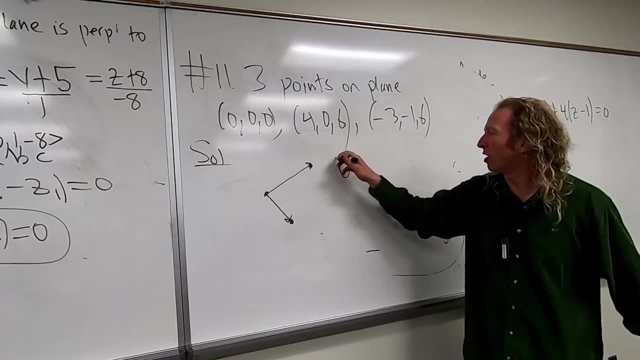 Any two, So let's do it. So let's just do this one first. So let's find u, I'll call it u, So I'll write it over here, So u So do. terminal minus initials. 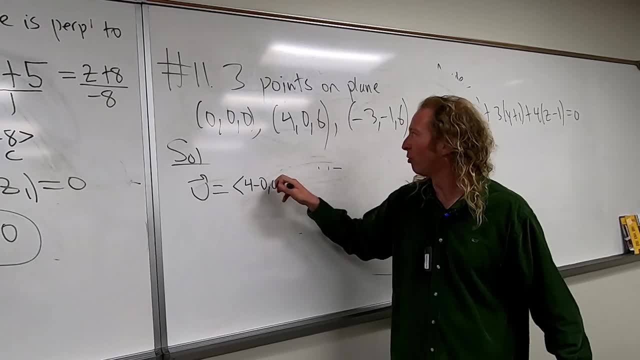 I'll even show the step. Look, it's 4 minus 0.. So 0 minus 0.. 6 minus 0.. You might say: why are you doing that That way? when you go home, you know what's going on. 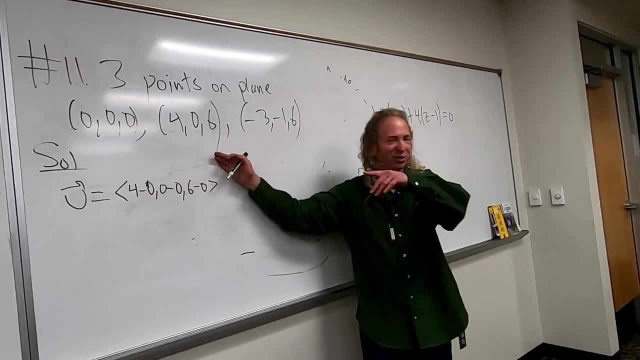 Right, Like, why did the points become vectors? Like no, no, I'm actually doing like subtraction, Right? So 4 minus 0.. 0 minus 0.. 6 minus 0.. So that's u. 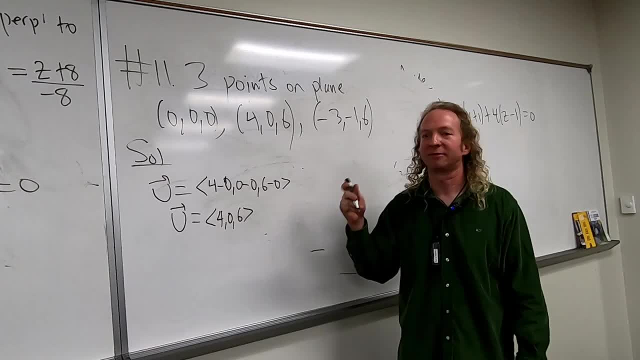 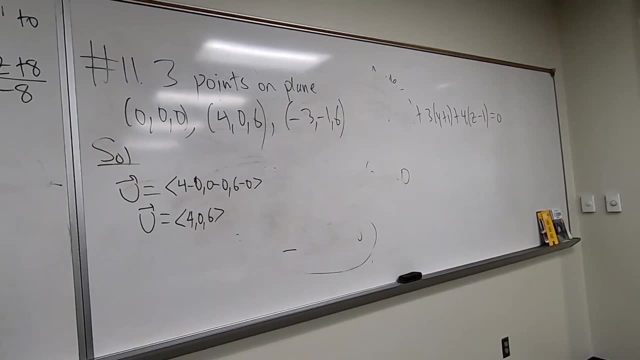 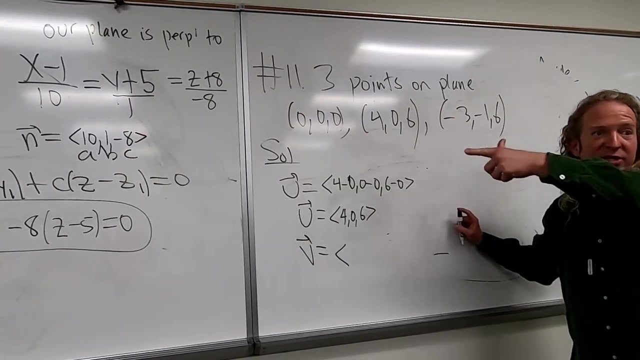 That's 4, 0, 6.. That's our first vector. It's on the plane, so it's parallel to the plane, Right? Let's find our other vector. We'll call it v, So I'll just I like using 0, 0, 0, because it's easy. 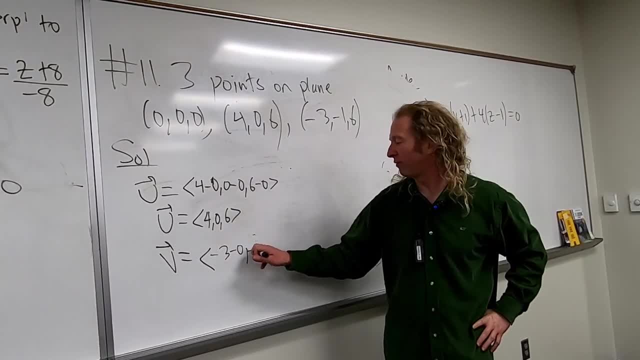 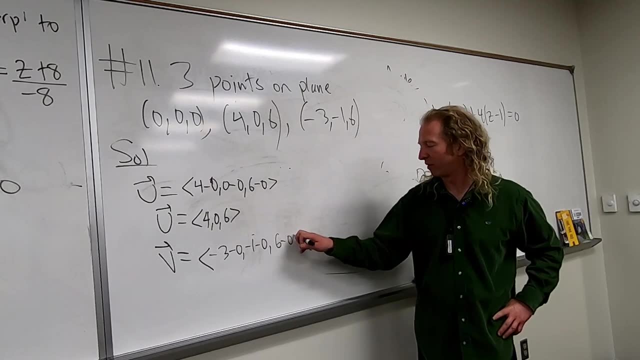 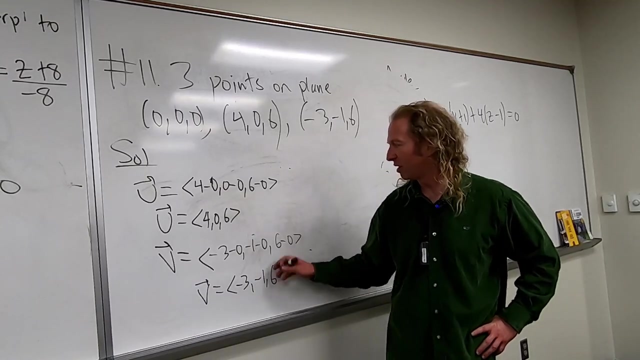 So negative 3 minus 0, negative 1 minus 0, and then 6, 6 minus 0. So v is negative 3, negative 1, 6. So these two are on our plane. 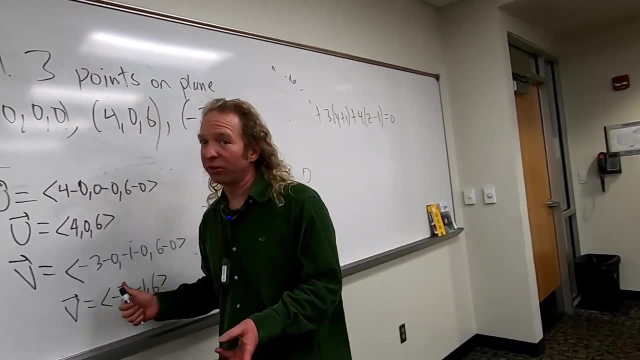 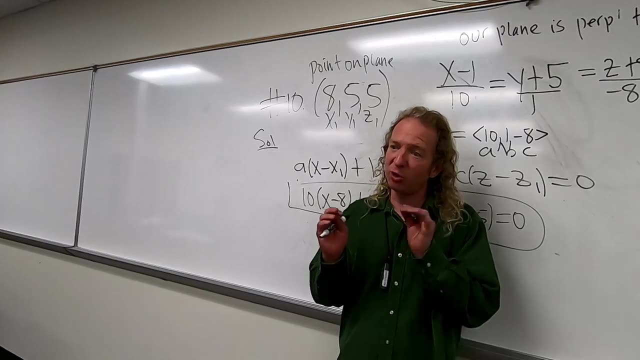 We have two vectors on our plane. Okay, In general, Whenever you have two points on the plane, you can always find a vector on the plane. In other words, whenever you have two points on the plane, you can always find a parallel vector. 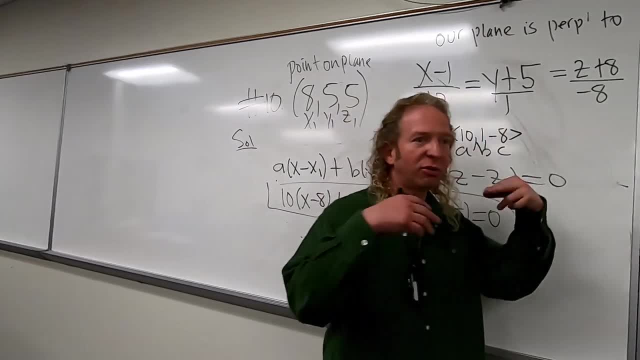 That's useful because if you have two parallel vectors, you can always take the cross product and that will give you n, and then you're done with the problem. Right, Because the goal is to find n. Right, So you can plug it into the formula. 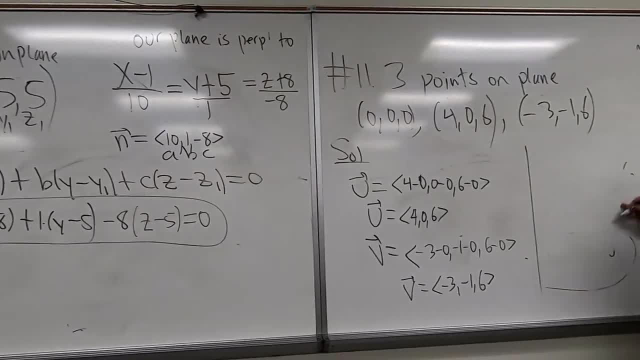 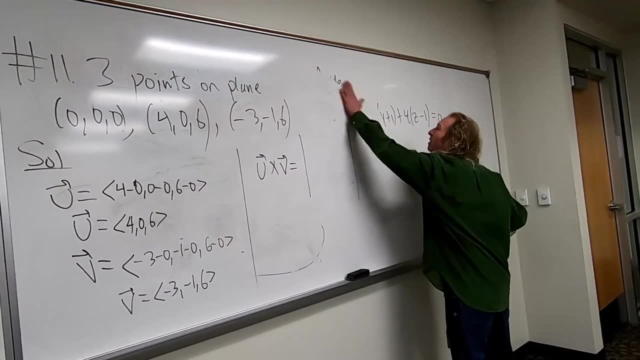 Right, Okay, So let's do it. u cross v. Blast from the past, from last week. u cross v. It's been a while. It's been a while, So you put the determinant. Do you remember what goes in the first row? 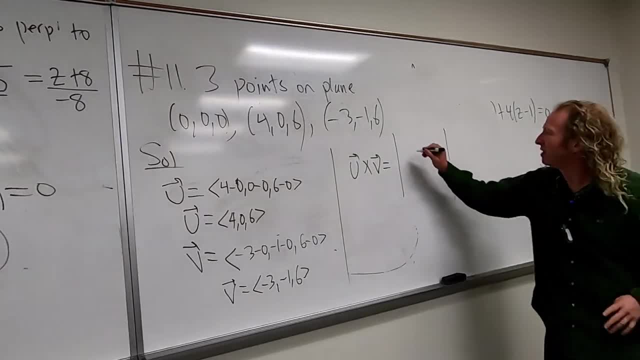 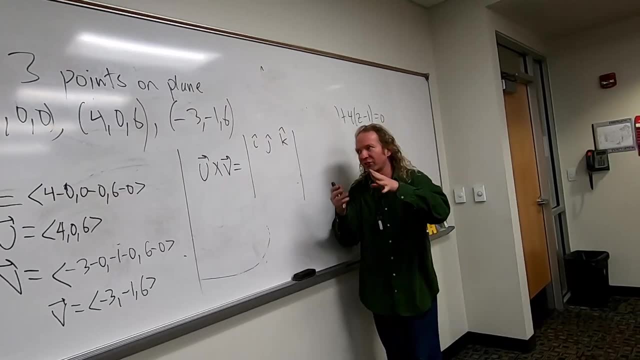 IJK. Yeah, Good, You know, You remember stuff. Good, So it's IJK, IJK. This comes up a lot Right? You only have one question on your test, just where it actually says: find the cross product. 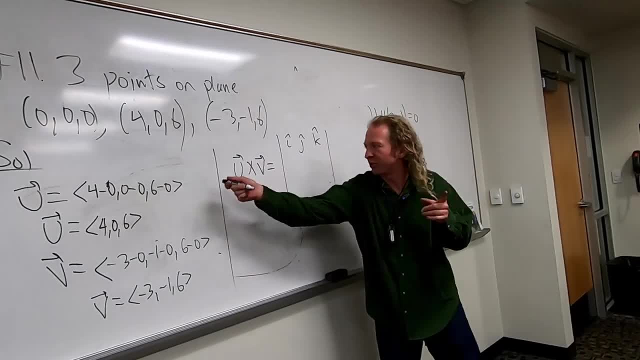 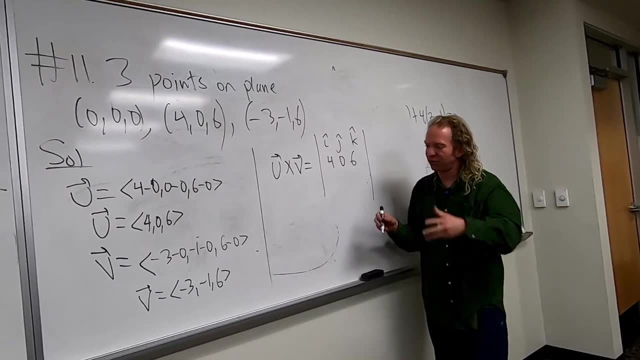 But it comes up in other questions And then you put the u first because the u is written first. You could have done v cross u as well. It's okay, Same answer. At the end it's the same answer Like when you finish the problem. 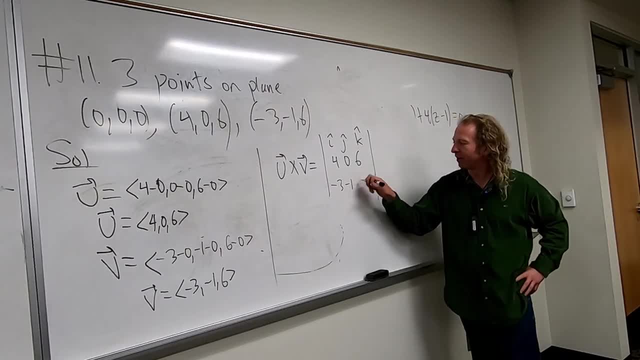 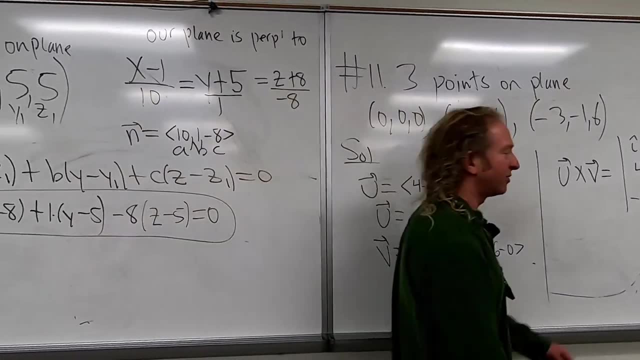 Okay, And then negative 3,, negative 1, 6. Good stuff, So this is equal to. So I like to put the i hat first. I have a habit of that, So i hat It's plus minus plus. 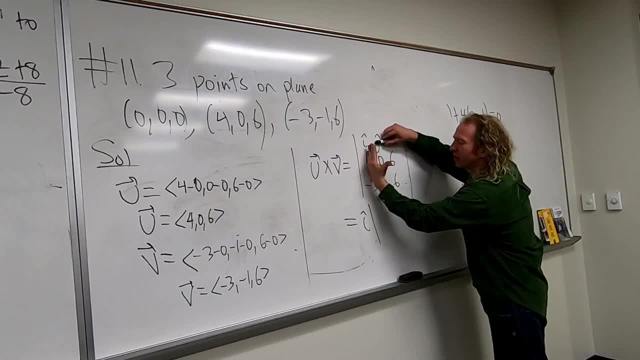 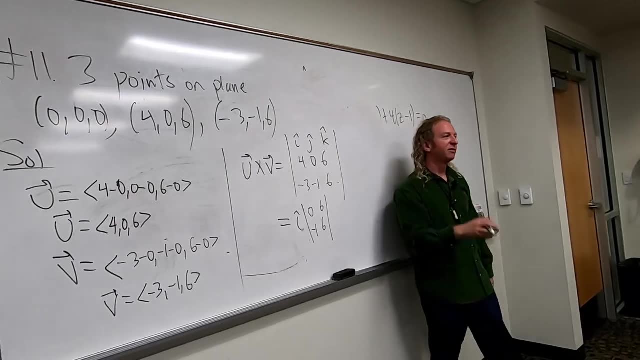 So you cross out the corresponding row and column right. So 0, 6, negative 1, 6.. So 0, 6, negative 1, 6.. I'm not going to mess up. 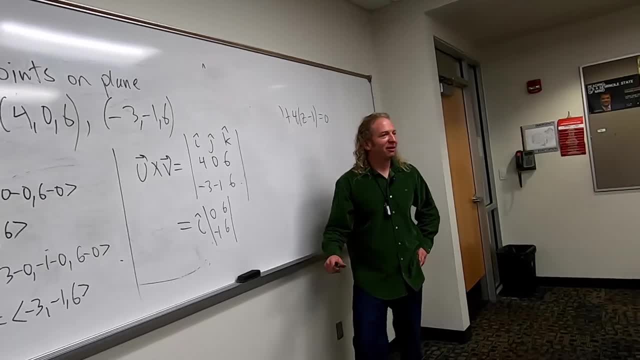 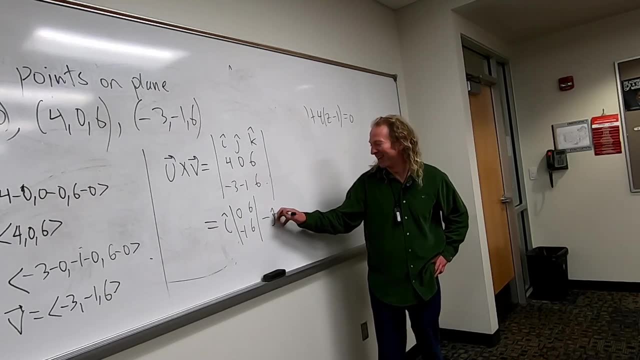 It's double. I'm going to mess up all the points, right? So all right. Is it plus or is it minus? It's minus. Very good, It's minus, It's minus. So you cross out the corresponding row and column. 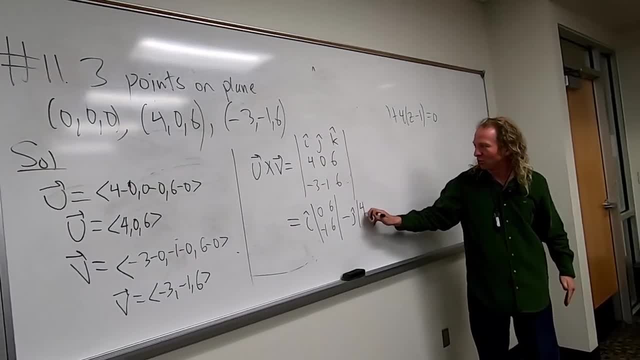 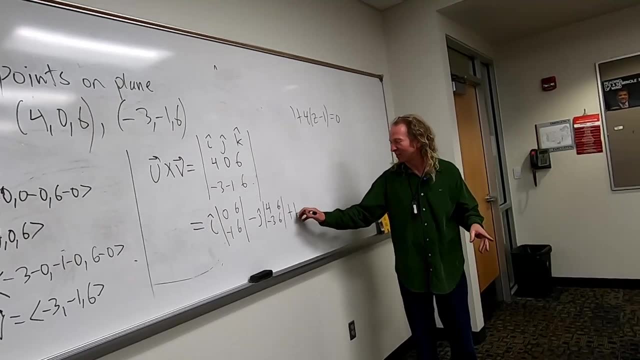 So 4, 6, negative: 3, 6.. So 4, 6.. It's really hot in here. Negative: 3, 6. And then it's plus. It's this long-sleeved shirt. 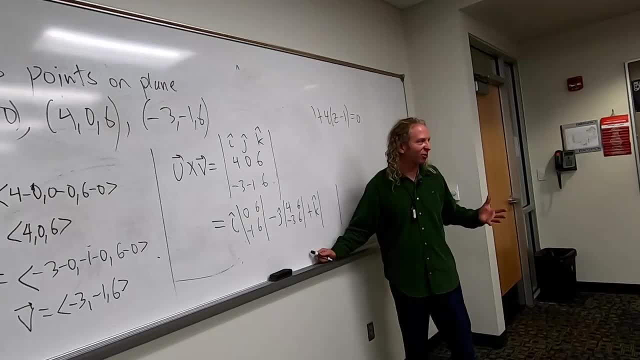 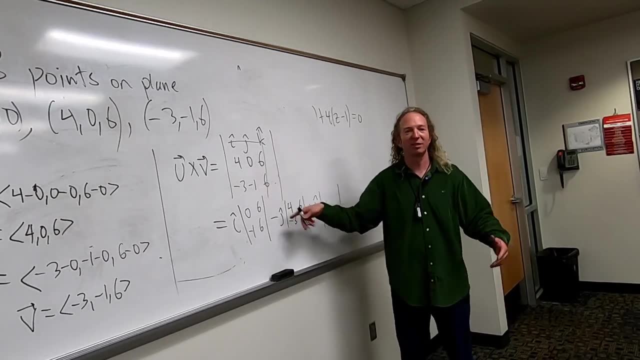 It was cold outside, but it's not cold in here. I'm finally going to do what I've been wanting to do this whole time. All right, Because you can cross them out. That's what you're doing mentally, right In your mind. you're doing that when you're finding these. 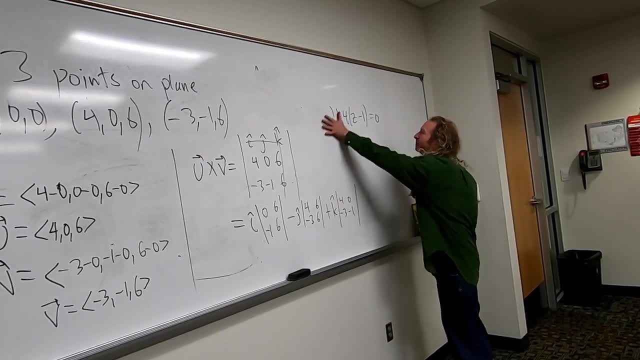 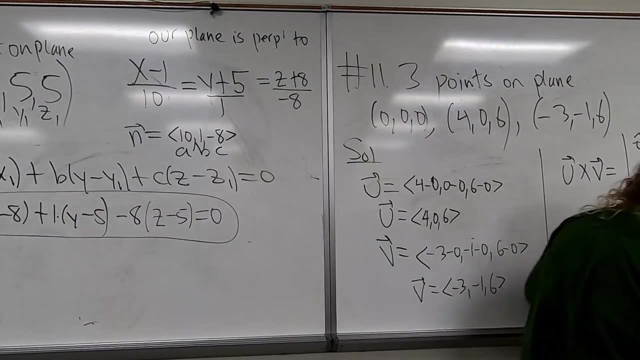 So 4, 0, negative, 3, negative: 1.. Any questions so far? Any questions, All right. So this is equal to. So now we can figure out these determinants. So I'm going to skip some steps here. 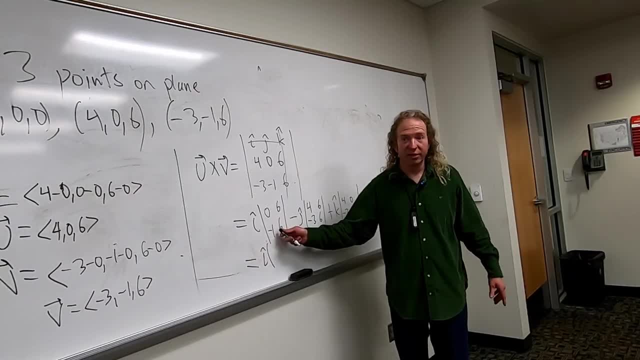 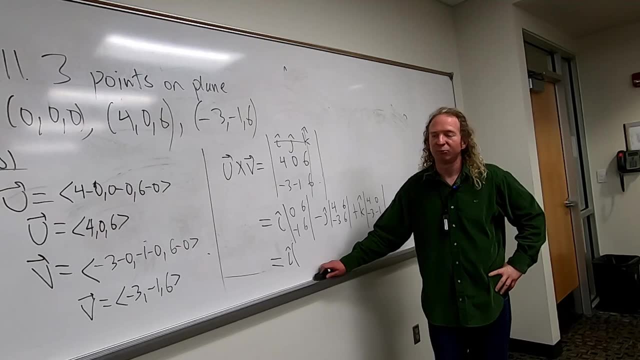 So i-hat. So 0 times 6 is 0.. Yeah, I just have a question: How do you figure out which one is 0? It doesn't really matter, Okay, Mm-hmm Right. 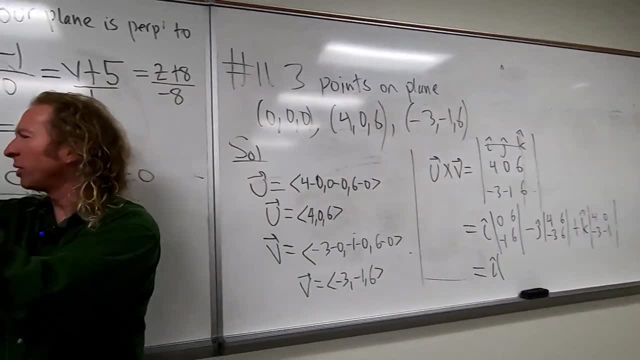 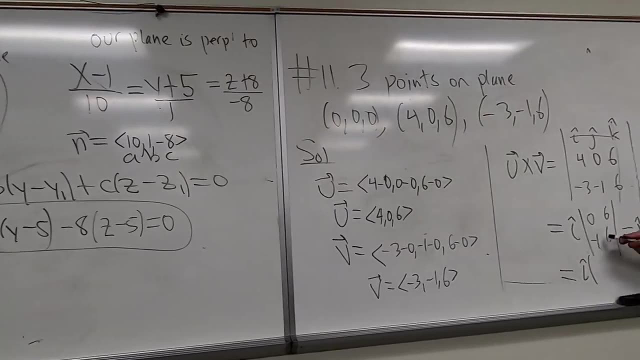 Because you can get. Yeah, Because if you subtract them the other way, it's just a vector going the other way. I'm just paying attention to the points of the right angle. Mm-hmm, So 0.. And then minus negative 6 becomes a plus 6.. 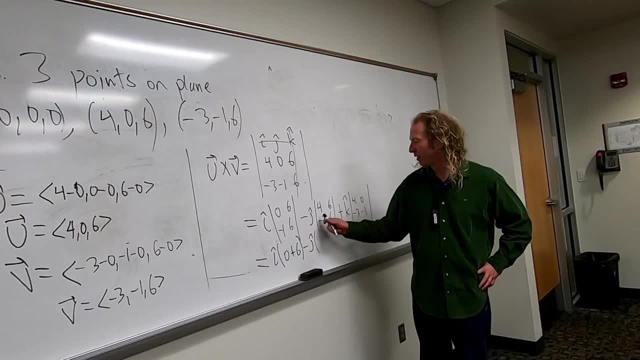 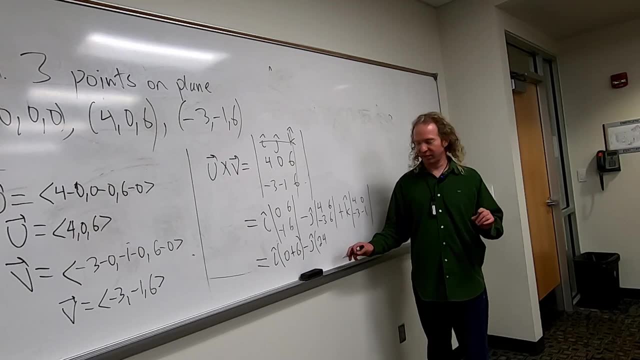 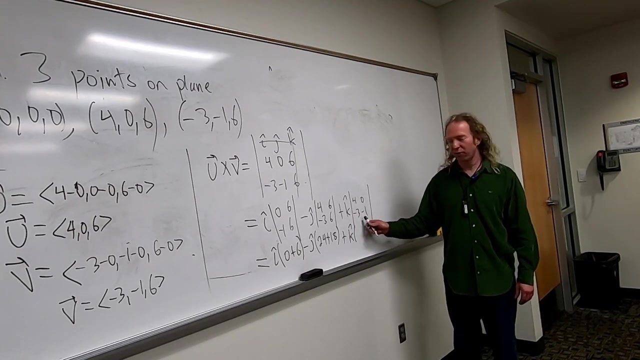 Right, So plus 6.. Minus j-hat 24.. Minus negative: 18 is plus 18.. Good, Plus 18.. Plus k-hat Negative: 4 minus 0.. Right, Because you do this times this minus this times this. 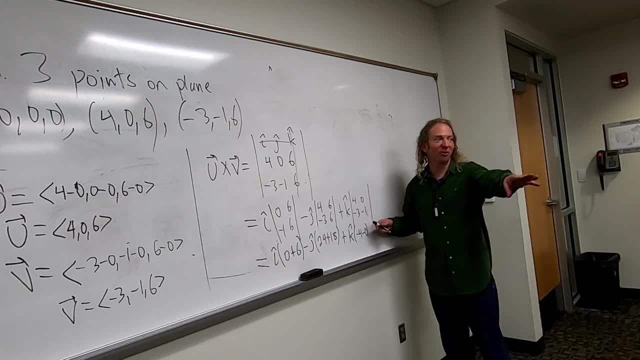 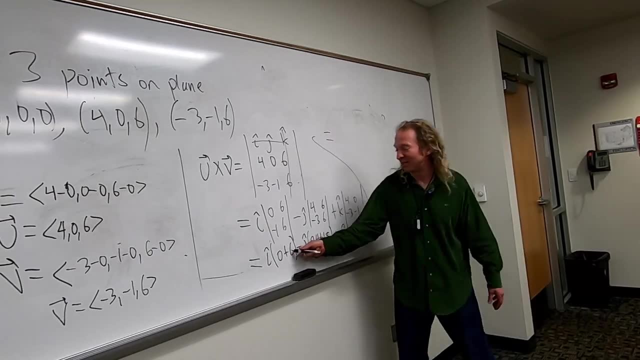 This times, this minus, this times. this Does that make sense? Oh, you weren't here. Oh, I remember. Does that make sense? Yeah, Good David. So this is 6, i-hat, Oh 24 plus 18.. 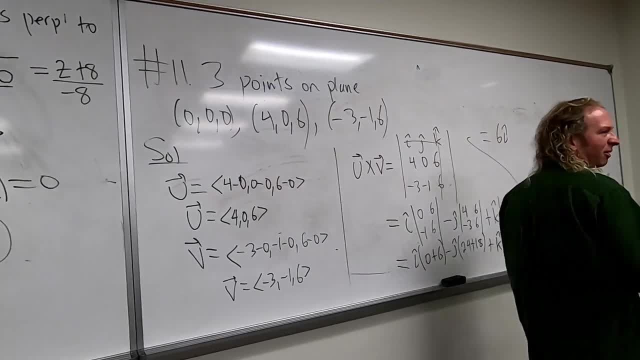 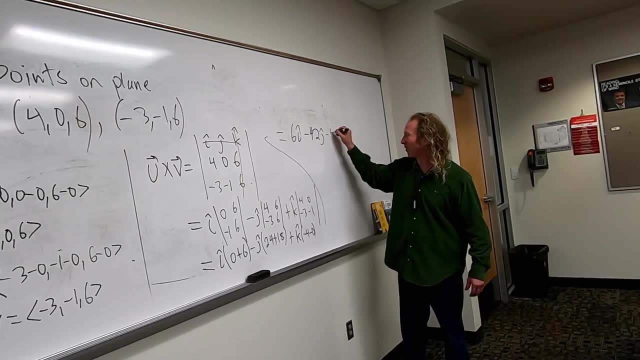 Anyone know what that is. Is it 42?? Okay, What it is right? 42 j-hat minus 4 k-hat. I'm going to write this in a better way, with the angle brackets. Do you remember what it's called when you write it? 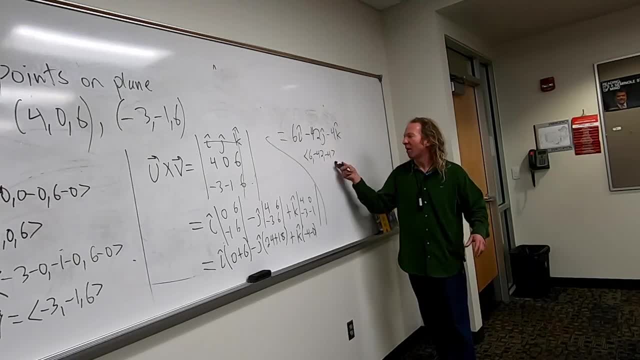 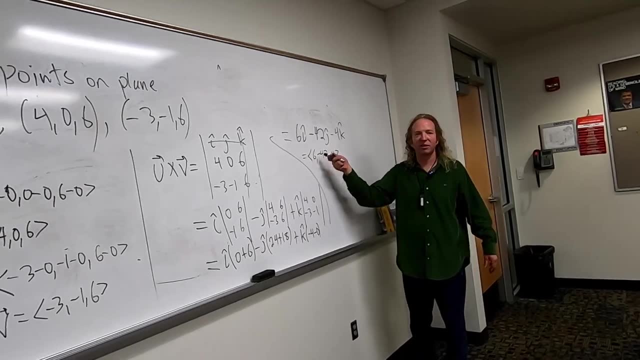 What's this form called? Yeah, component form. So I'm going to write it that way. It just seems a little more clear. You don't have to make that leap, I just prefer component form. And what are these? These are our what. 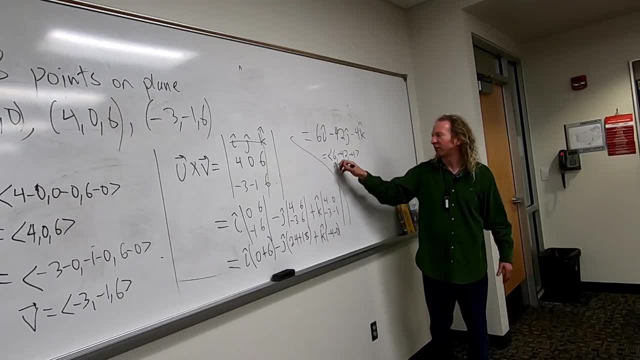 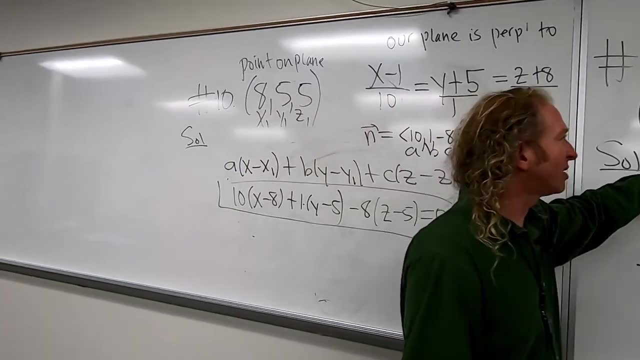 This is our what ABC. This is our normal vector. Good, This is our ABC. Mm-hmm. Any questions so far? Now we're going to finish it, But I like this one because it's not too hard conceptually. 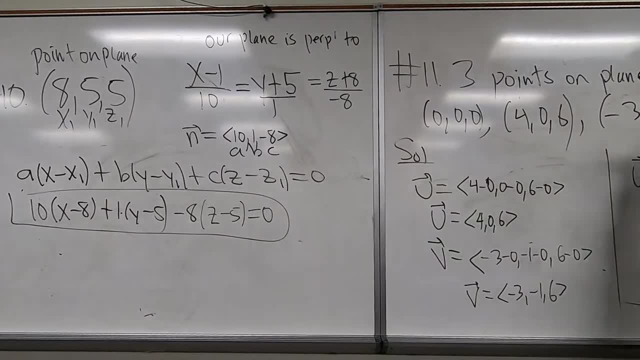 You have three points and then it's really easy to visualize it. Say: the board is the plane right, So 1, 2, 3. Draw a vector. Draw a vector. You have two vectors that are on the plane. 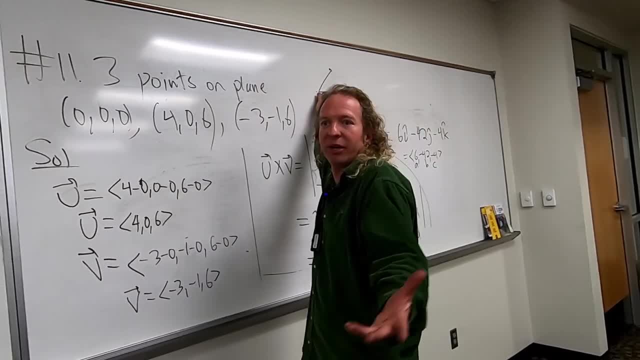 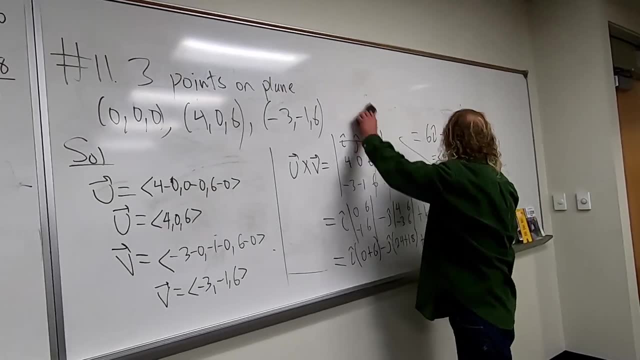 Take the cross product: Boom, And you get a perfect vector. That's your n right. So it's really easy to visualize this one. Let's finish it. I guess I can squeeze it in up here, So ABC. 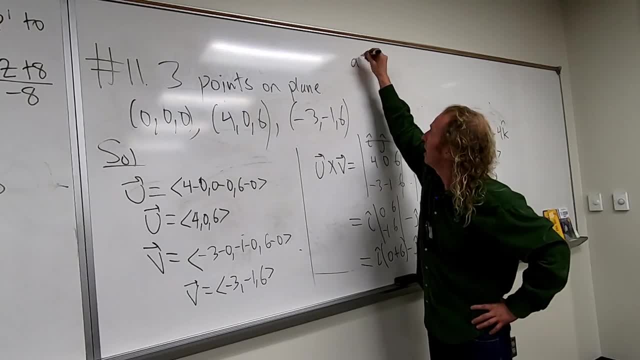 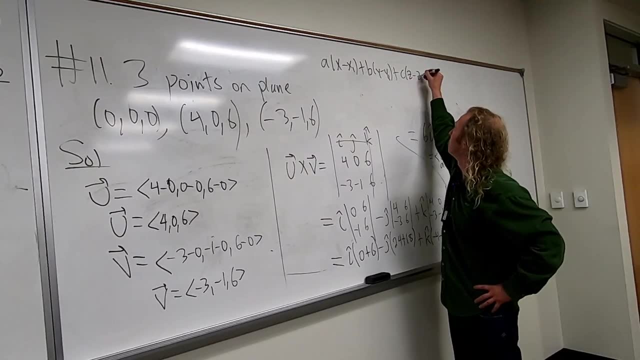 It's 6 negative, 42 negative. So the formula was A- X minus X1, plus B- Y minus Y1, plus C- Z minus Z1, equals 0. It's always equal to 0 in the formula. 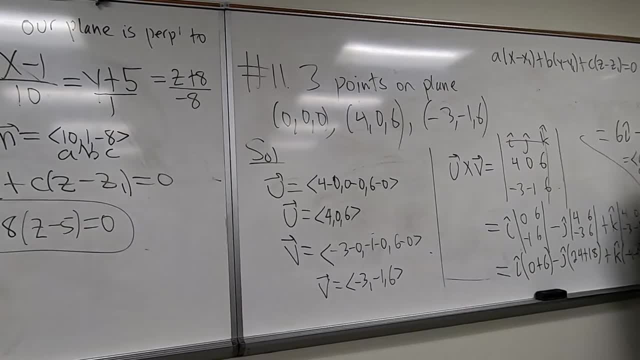 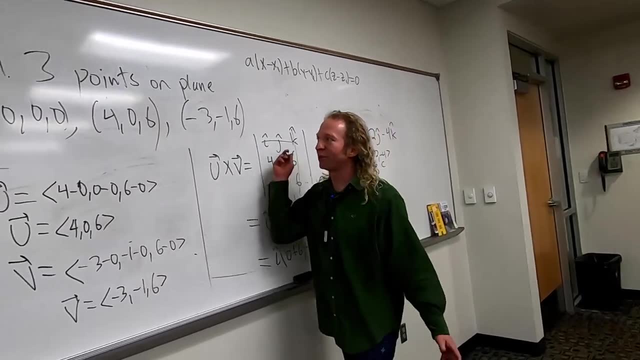 Always These pamphlets and stuff, Beautiful stuff. So then, A is 6.. Oh, oh, oh, oh. What's the best point to use here? Yeah, Let's use this one. Oh, yeah, Yeah, this is. 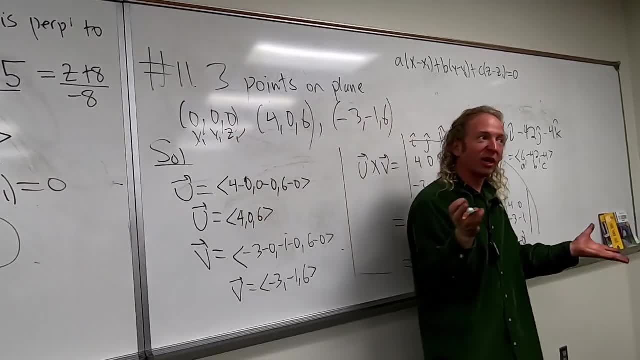 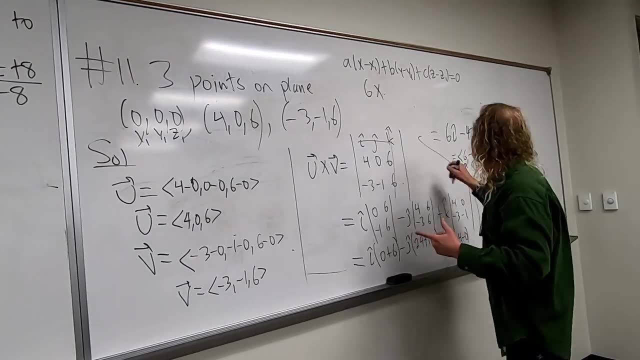 It doesn't matter which one you use. okay, It doesn't matter. So I'm just going to go to the answer, because these are all zeros, They're all going to go away, So it'll be 6X and then minus 42Y, because this is 0.. 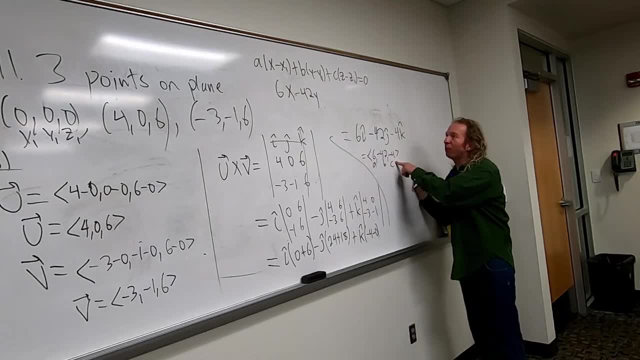 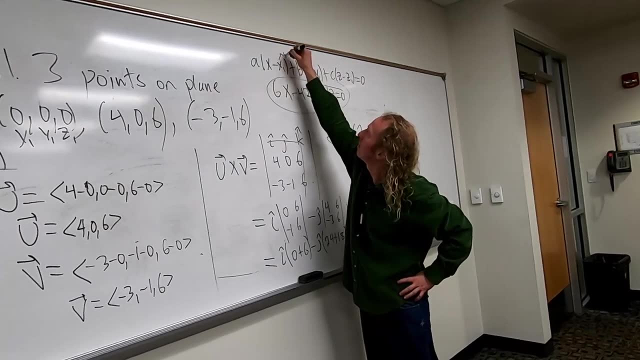 Because this is 0,, this is 0. And then C is negative 4, so minus 4Z And that's equal to 0.. That's it Right there. Because these guys, this is 0,, this one is 0, and then this one is 0 as well. 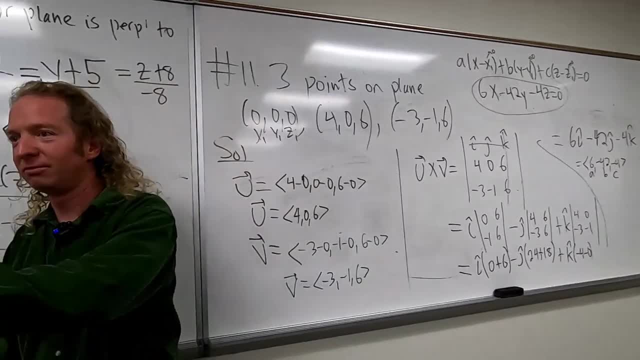 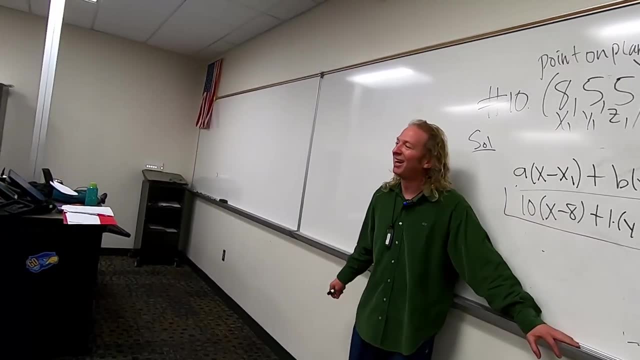 Those are all zeros. Yes, Jamal, So the N vector Come on. Yeah, Oh, my God, I'm sorry. So the N vector isn't on the plane. It's just perpendicular to the plane, Right, Thank you. 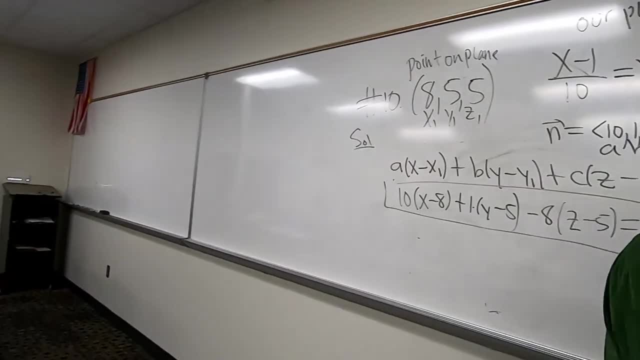 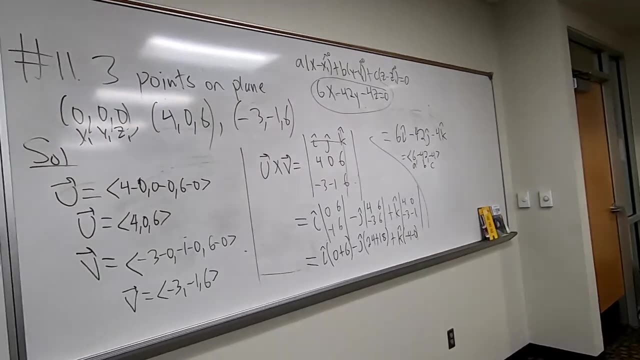 It's come on And I'll just call you Cabal. I'm so sorry, I'm so bad. Any questions? on that one, Yeah, the N vector is always perpendicular to the plane. It doesn't have. Yes, perp. 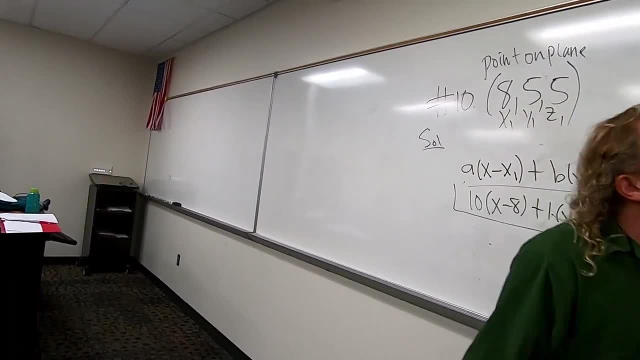 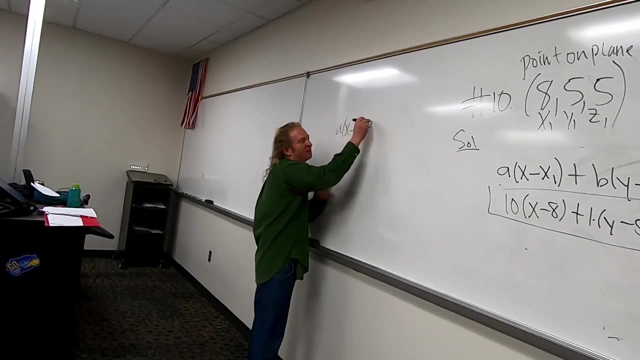 Yes, What equation is that? What's the name of that equation? Oh, very good, Yeah, because you, yes, So I'll write it over here for you. So this, this is the formula. Yeah, you missed the derivation, but it's okay. 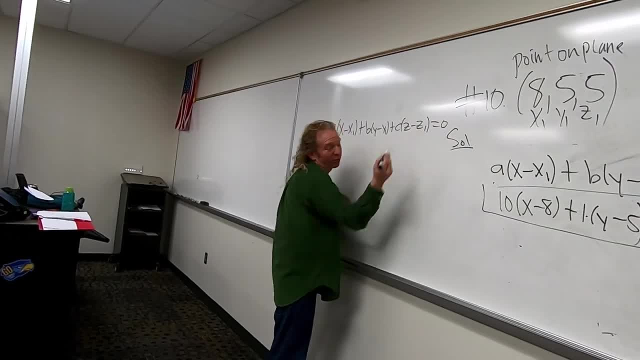 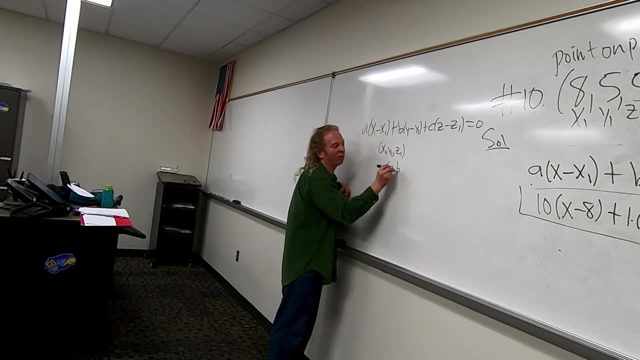 So, yeah, yeah, it's really cool. It's a really cool derivation. So, basically, this is the equation of a plane And this is a point on the plane And this is your normal vector. This is perp to plane. 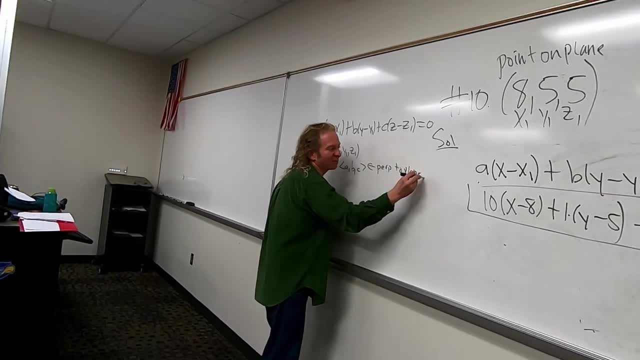 So that's the equation of the plane Mm-hmm. Okay, And the goal in all these problems is to find the ABC, the normal vector. That's the hard part, Because they're all different. right, They're all different. 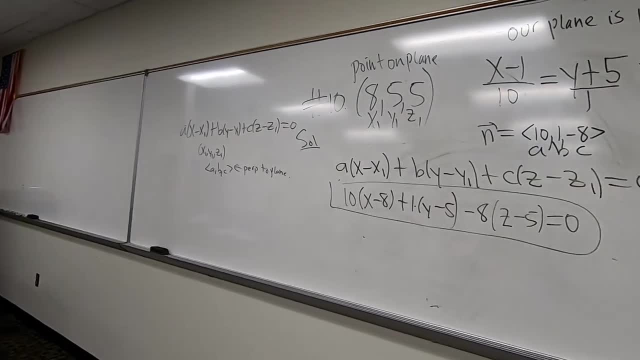 And they can. they get harder. Each one's a little bit harder, The next one's a little bit harder. So Yeah, All right, let's do it. Let's do it. That was number 11.. Any other questions on 11?? 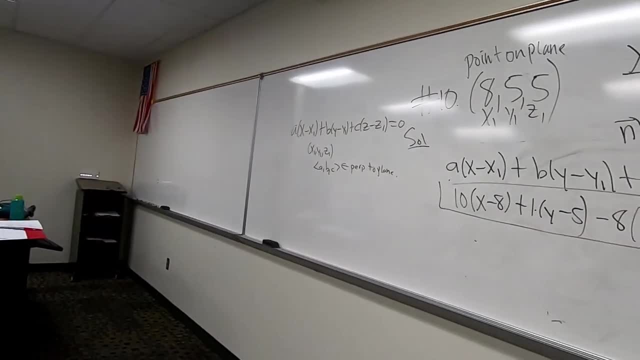 So I think you can do it again on Monday. If, like, if it showed up on a test, like, could you do it? Yeah, Yeah, Yeah, Yeah, Yeah You will. I'm going to remember. No, I'm kidding. 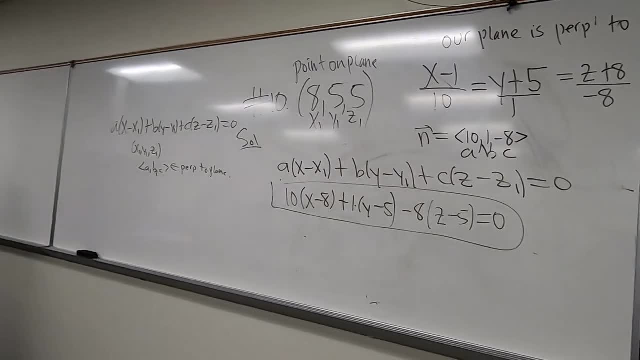 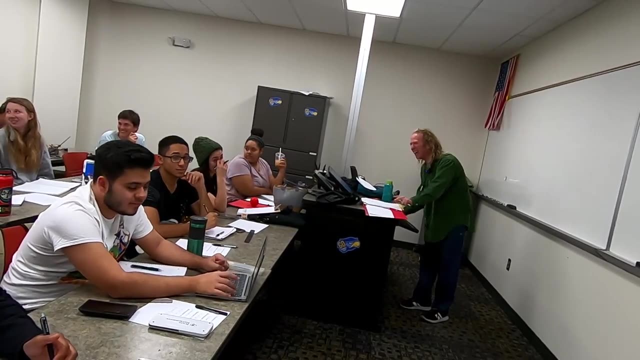 Like, who said you would do it? No, no, You did it wrong. Like some comments on your test, You lied to me. No, no, I'm kidding. I'm kidding. Just write that on every test and write it away. 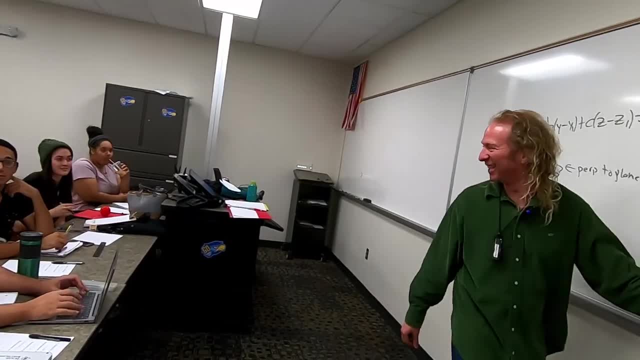 Yeah, No, it's so bad. I think you stopped after the first one. Yeah, No, I don't Yeah. I don't Yeah, No, I never did I just Well, actually, no, No, that's actually. 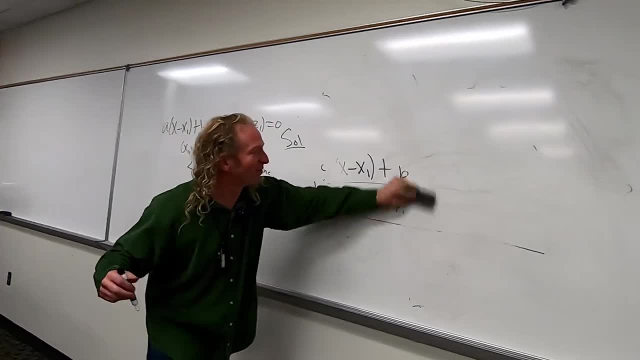 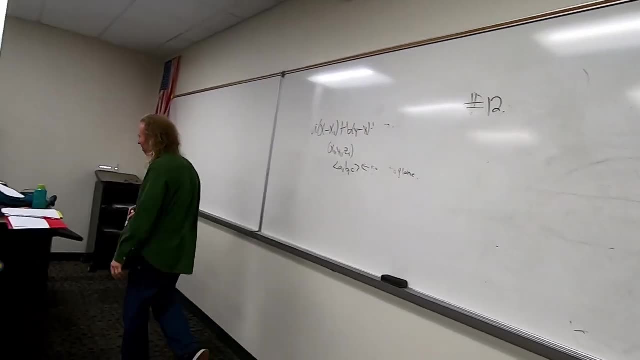 So never mind. Number 12.. Number 12.. I try to grade the test as fast as possible, So I don't even look at the names a lot of times. Find the equation of the plane. Okay, They give us the point. 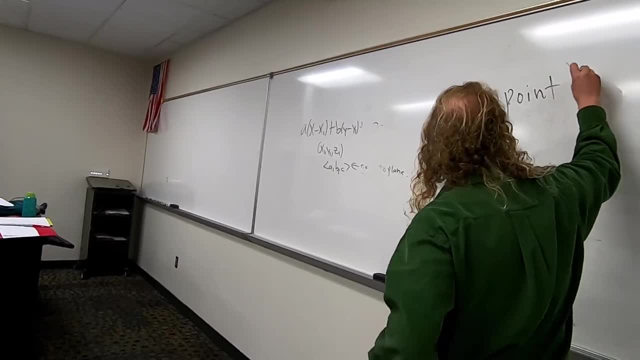 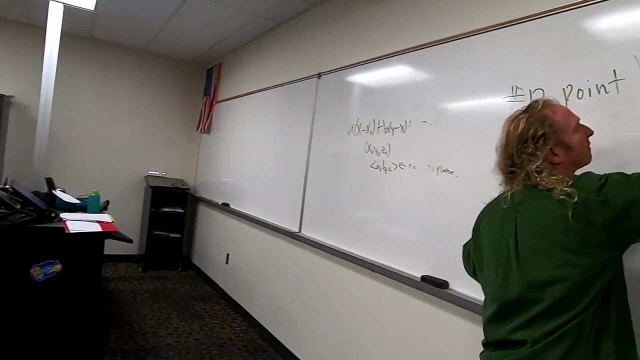 So that's good. They always give us a point Which is: Which is nice, So 10.. I signed every single possible plane question that was in the homework: 10, negative 8, and 5. That's good. 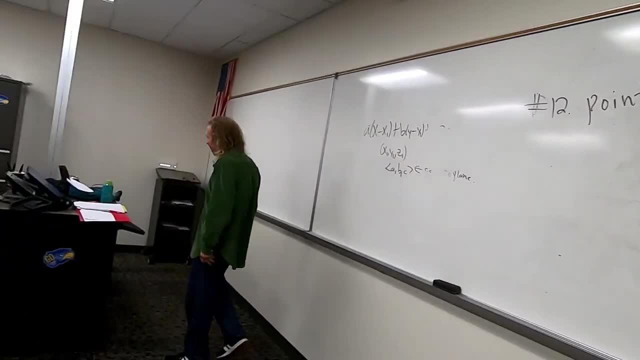 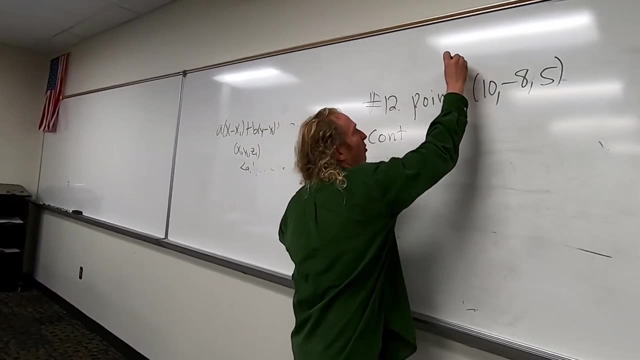 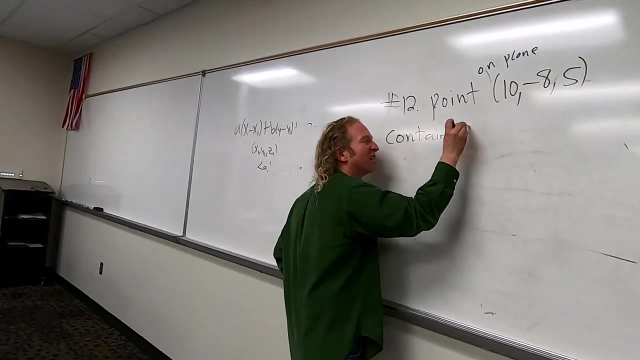 That's our X1, Y1, Z1.. Success, We've got some progress. Then they say it contains the line Interesting, So contains. So this point- This is a point on plane Plane- contains the line. 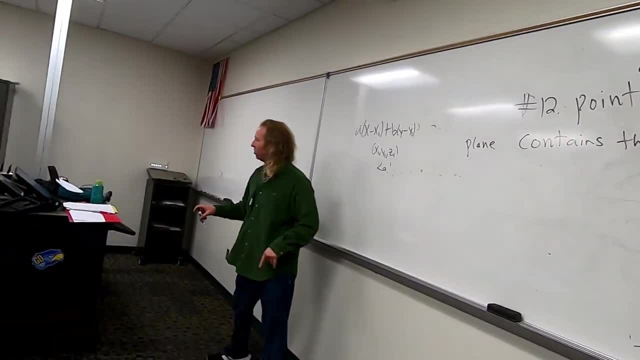 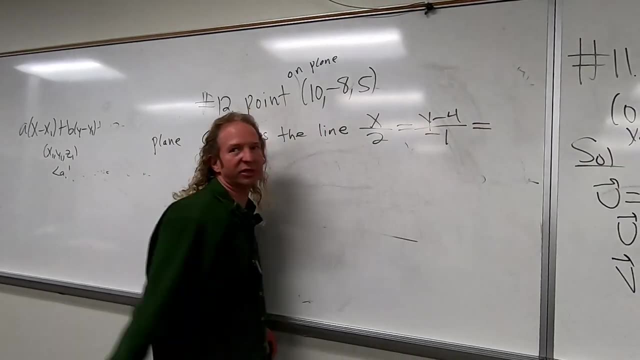 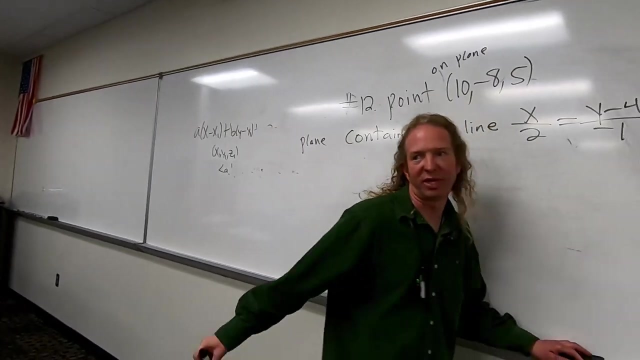 This is pretty deep. I like this problem: X over 2 equals Y minus 4 over negative. 1 equals Z equals Z equals. I'll give you some time to write this one down. Take your time, We've got tons of time. 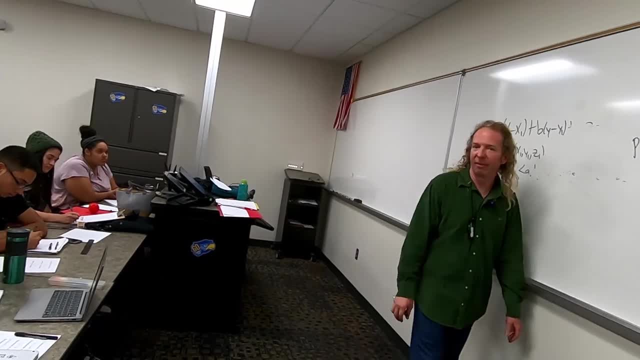 After we finish all this homework, we're just going to do the next section. It's not bad at all, It's like just We're just going to touch on it. I'll derive some, I'll show you some stuff and we'll do some problems. 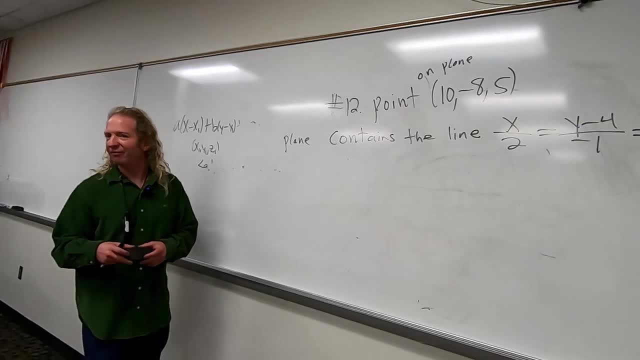 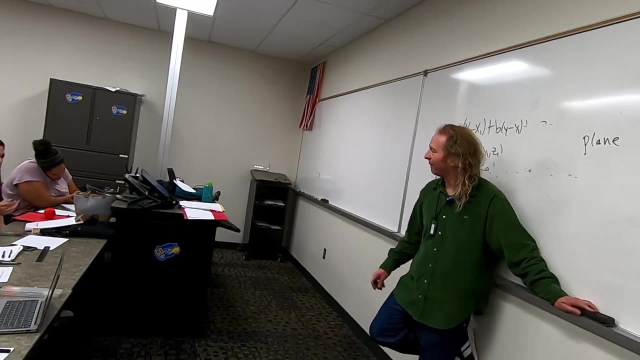 I'm not really going to derive it, Okay, So yeah, No, no, Go ahead. Do you have an idea? No, no, no, Do you have an idea? I was going to ask an abstract question, Oh, no. 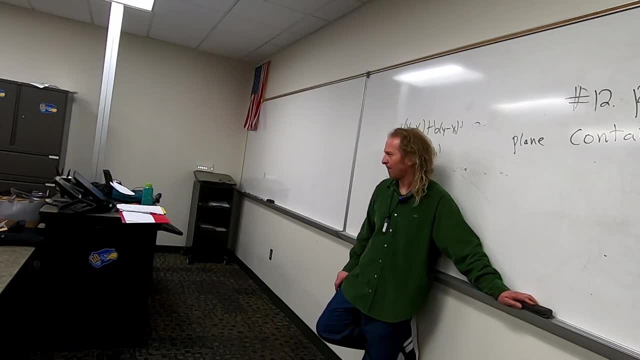 Ask: That's okay, No, it's good. So we're finding things that are orthogonal. What place does derivatives have? Because derivatives are technically also perpendicular, So tangent. But it's going to come up right, Right. 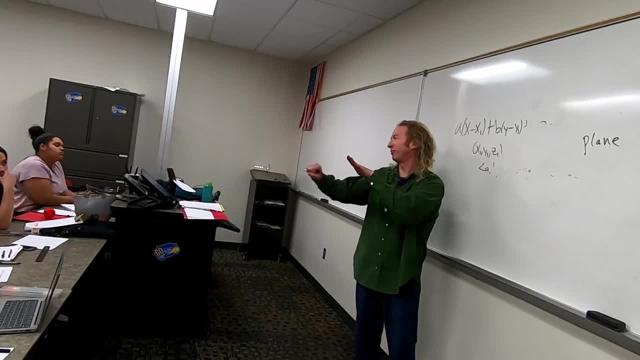 Because later on we're going to have vectors that are tangent, So tangent to functions and orthogonal to functions- Vector-valued functions. Yeah, Yeah, So we're going there. Yeah, we are going there, We're going to get there. 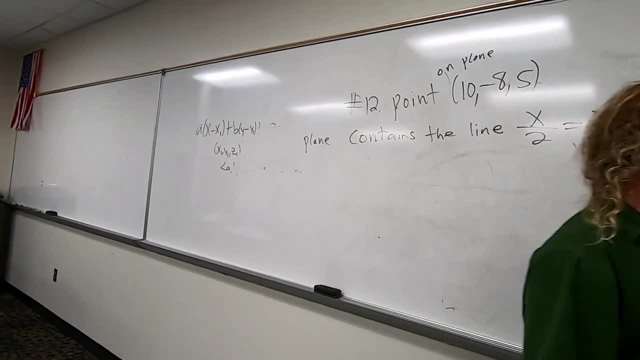 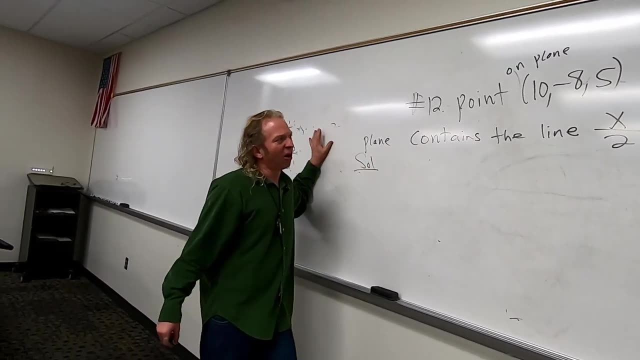 We're going to be having stuff like this: cross products later on are going to have functions inside them and stuff. It's really cool. Yeah, Yeah, it's exciting, Exciting times. Okay Solution, Good question. All right, So let's pretend that the board is the plane. 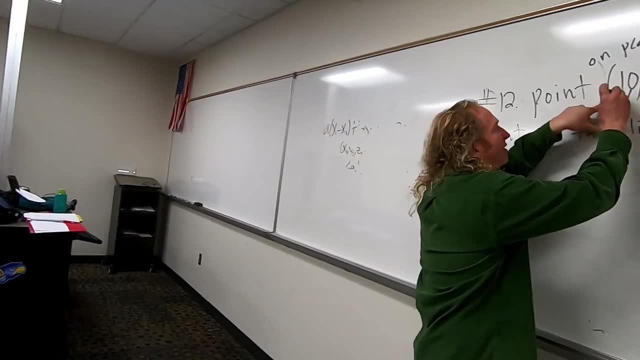 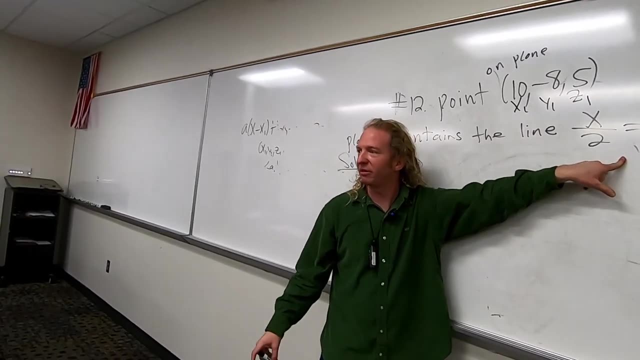 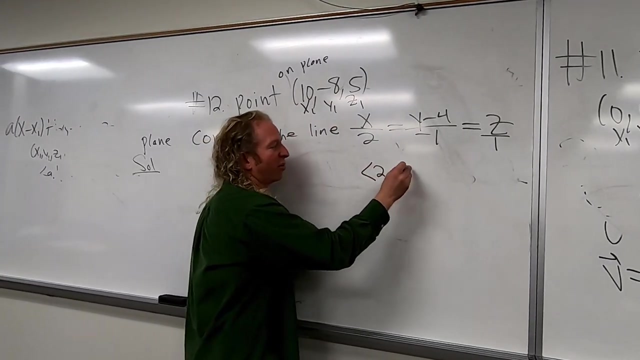 Right. So this point is on the plane. So we've got that. This line is on the plane Right. There's a vector here, The vector 2, negative 1, 1 is parallel to this line, Right. 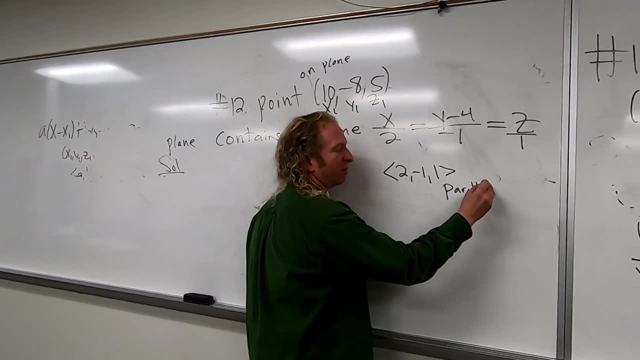 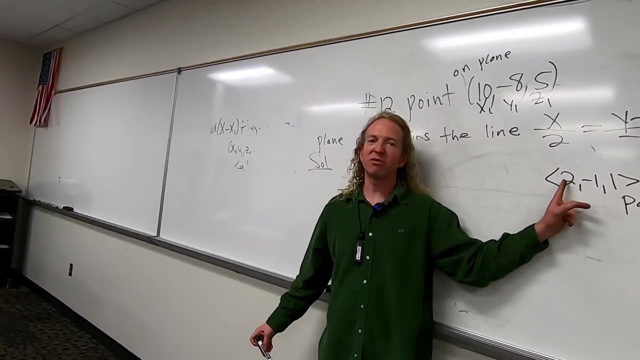 This is parallel to- and I'll put an arrow here, So this is called the direction vector Right. Remember these numbers? They had a name too. Remember what the numbers were called? Do you remember Direction numbers, Direction numbers. 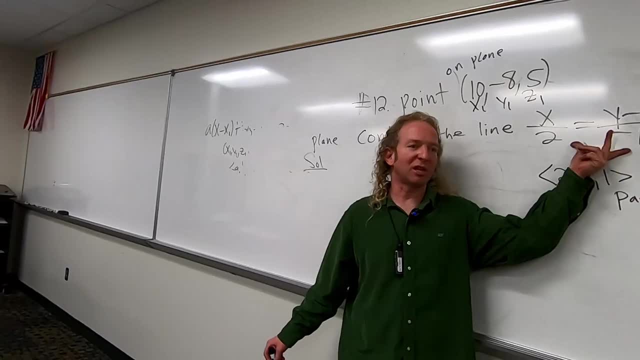 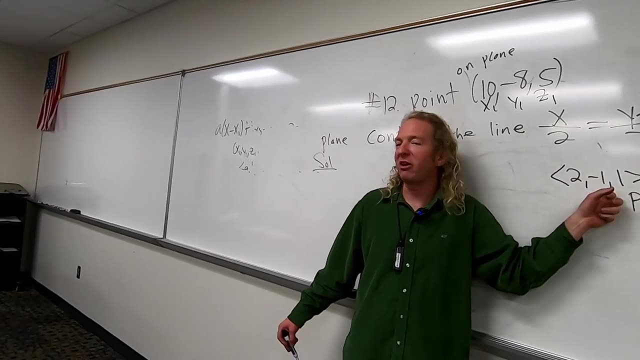 The extra knowledge. Yeah, So this vector is parallel to this line, But the plane contains this line, So this line is on the plane. That means this vector is parallel to the plane, Right, Because this is on the plane. 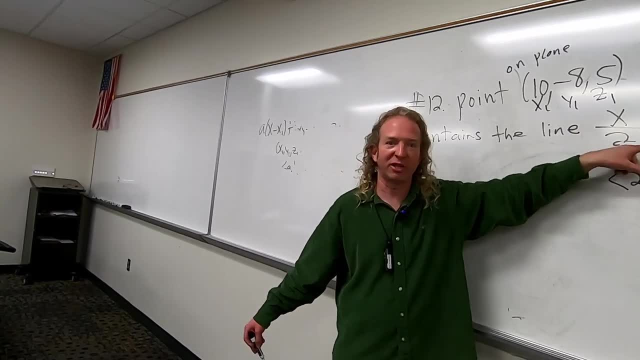 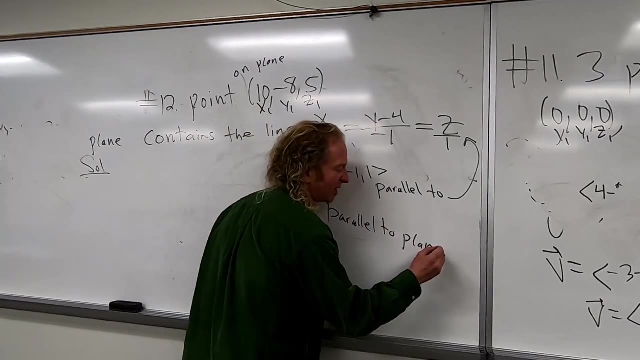 This is parallel to this. So it's parallel to the plane. So this is parallel to our plane. Does that make sense? Everyone understand that leap Parallel to plane. Let me explain it again, just in case. So this line is on the plane. 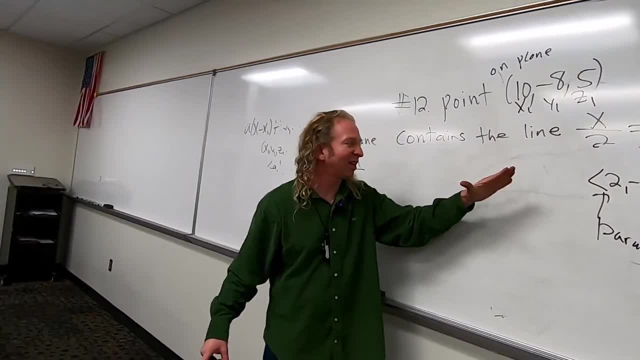 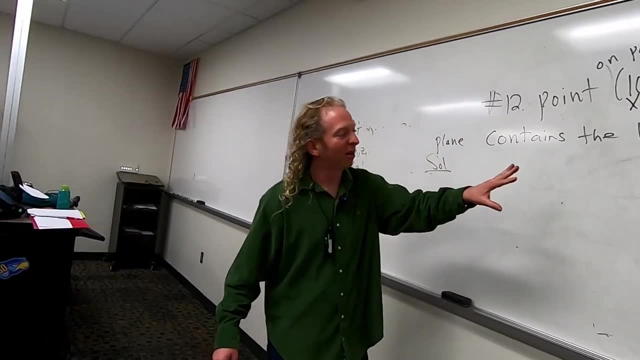 Like say, it's this, This vector is parallel to this line. Therefore it's parallel to the plane. Okay, So we have a parallel vector to our plane. In the previous problem we had two vectors that were parallel and we took the cross product. 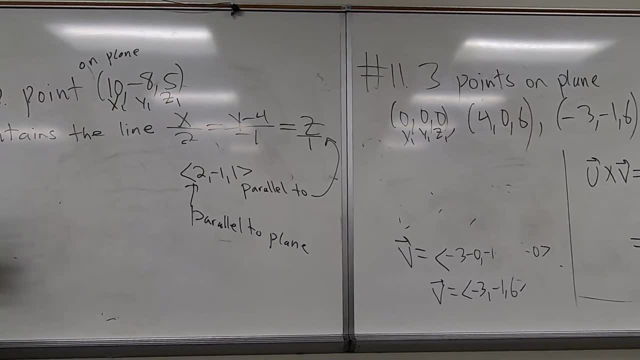 So the question is: can we find another one? Well, obviously yes, We have to find a solution. So we have a point on the plane. So if we had another point on the plane, we could find another parallel vector. 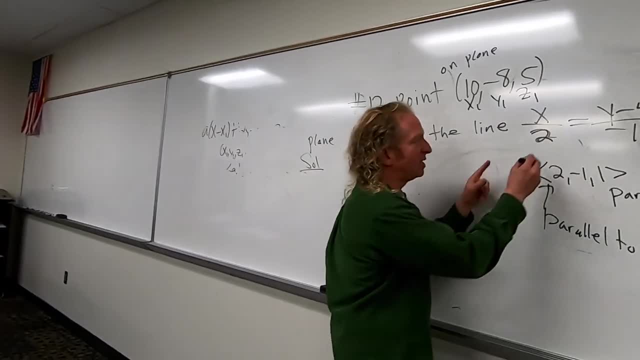 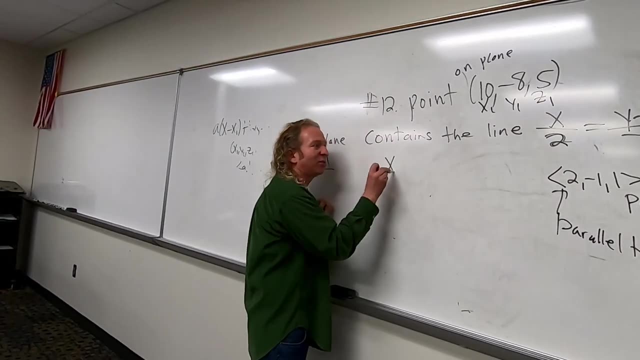 So the trick is to manipulate this to get an easy point, Because this is on the plane. So what's the easiest number in the world you can plug in for x, Zero, Zero. So if we just set x equal to zero, what would that force y to be? 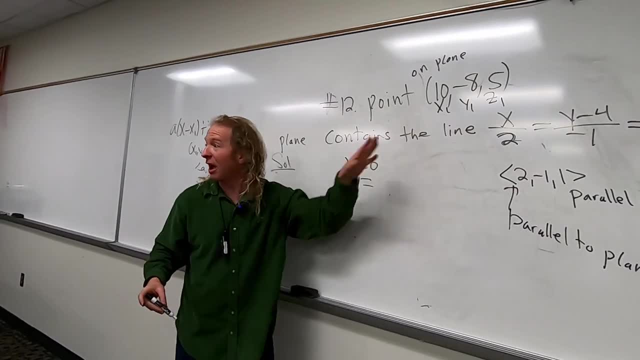 What would y have to be in that case? Four, Four, Because they all have to be equal to zero Right, And then z would have to be zero Right. So we're just making a number up. How did I pick that one? 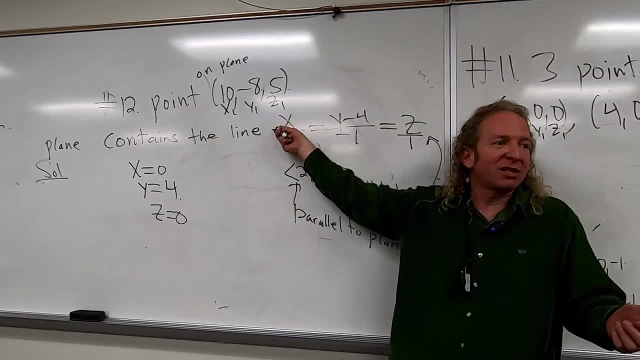 I just picked the easiest one in the world: Right: Zero. So if you make x zero, y is four, z is zero. So if zero four zero, this is on the plane Right. So if you make x zero, y is four, z is zero. 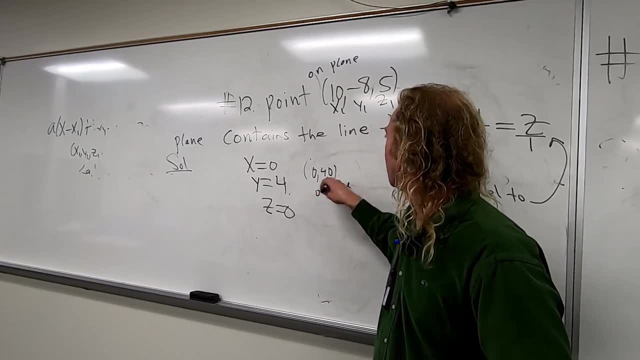 So if zero, four, zero, this is on the plane Right. So this is on the plane, This is on the plane. When we have two points on the plane, we can find a vector on the plane Right. 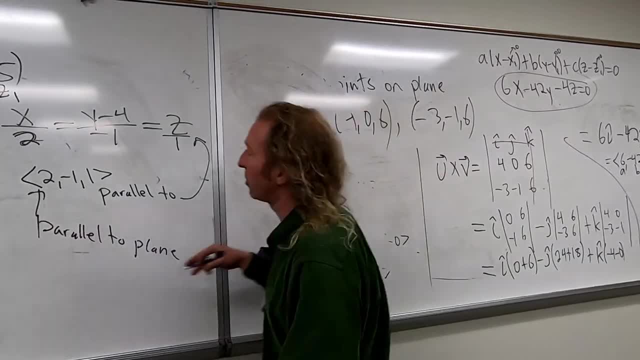 We can do the whole terminal minus initial thing. So let's go ahead and do that. So I'm going to give this a name. by the way, I'm going to call this, I'll call it v. And now let's find u, our other vector, u. 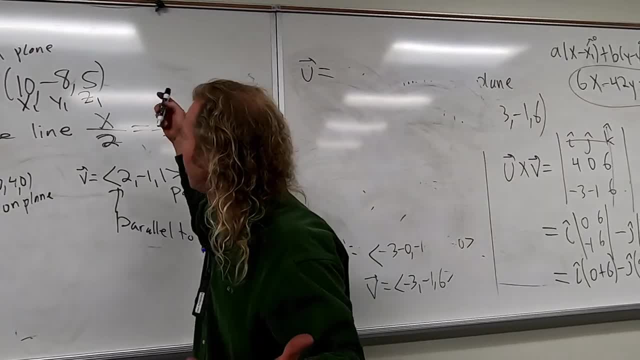 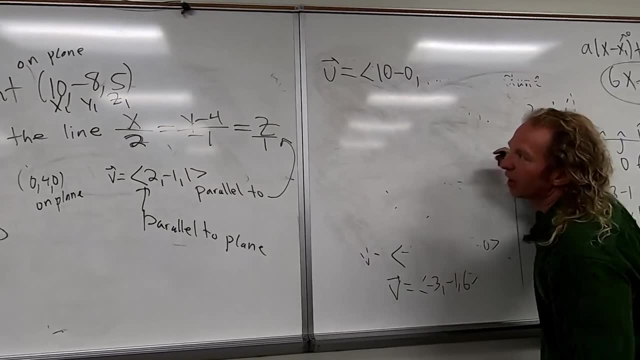 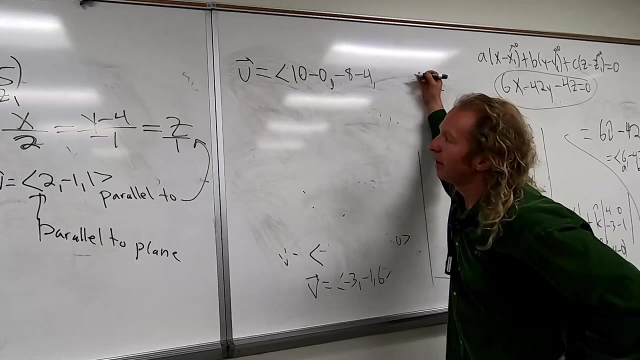 Let's just do- I don't know, let's just do this minus this, So ten minus zero, So ten minus zero, And then negative eight minus four, So negative eight minus four, And then the last one would be five minus zero. 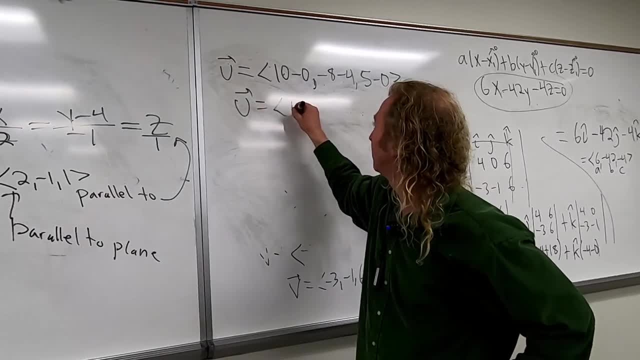 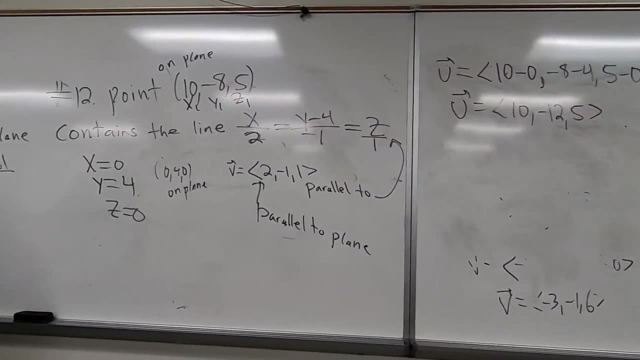 So that gives us ten negative twelve five. Let me pause here because this is tough. If you try to memorize it, it's really hard because there's so many different problems. It's always better to understand what's going on. 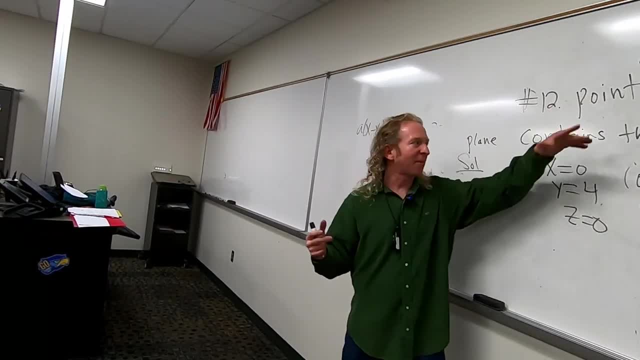 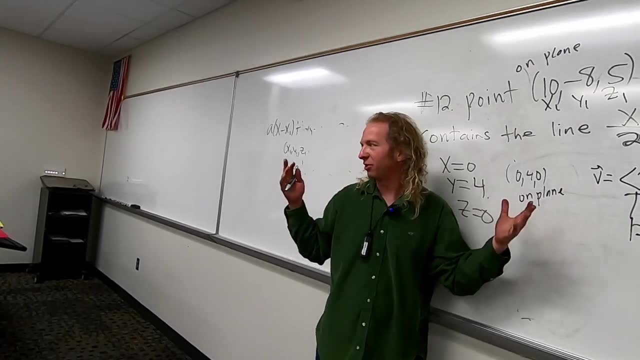 Like you read the question and say, okay, I have a point and I'm told that this line is on the plane. What am I trying to do? I'm trying to find a perpendicular vector. So I can't do it right away because, unless you're a super genius- 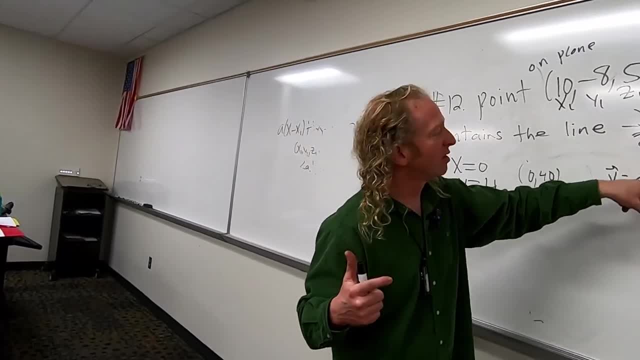 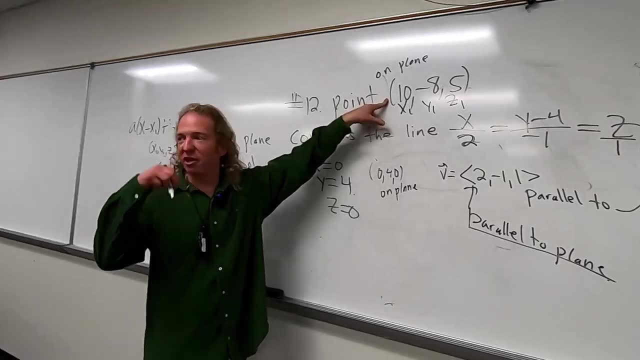 So you just do it in steps. Okay, this is on the plane, So this is parallel to this. So this is parallel to the plane. Okay, so this is parallel to the plane. This is on the plane. If we get another point, we can find another parallel vector. 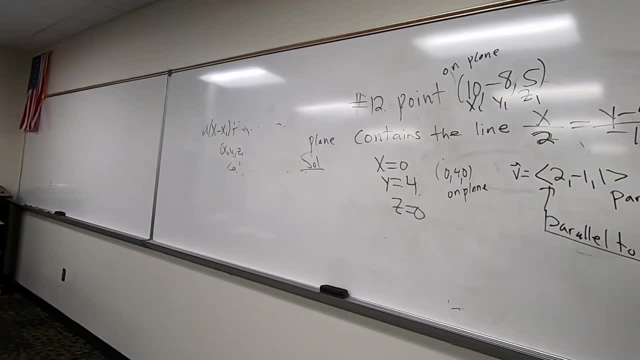 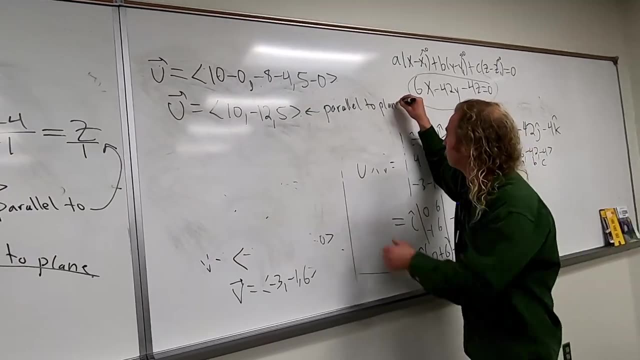 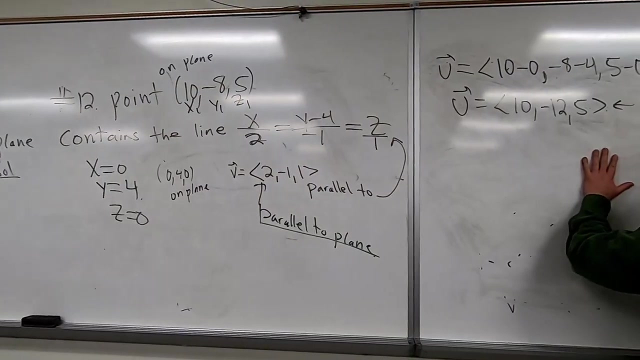 So you make one up, boom, Now we have: this is parallel to our plane, So this is parallel, parallel to plane, Parallel to plane. So we have two parallel vectors, Parallel vectors to our plane. When you have two parallel vectors, how can you find a normal vector? 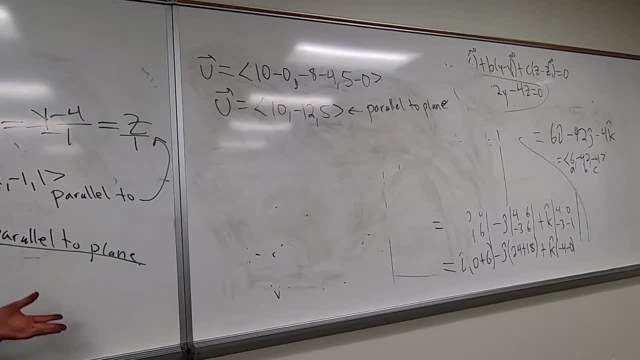 What can you Cross product, Cross product. yeah, It's a beautiful problem. I think this is like the hardest problem we've done all semester. like this is just I love this stuff, So it's U cross V. 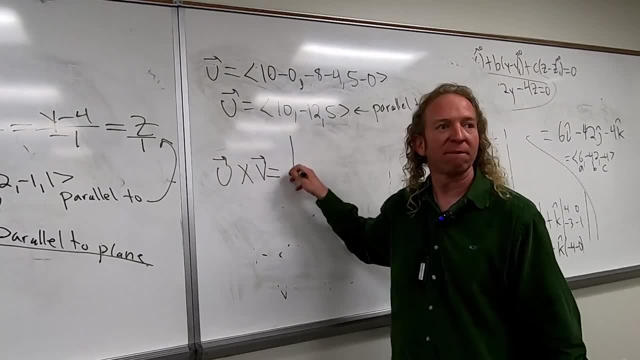 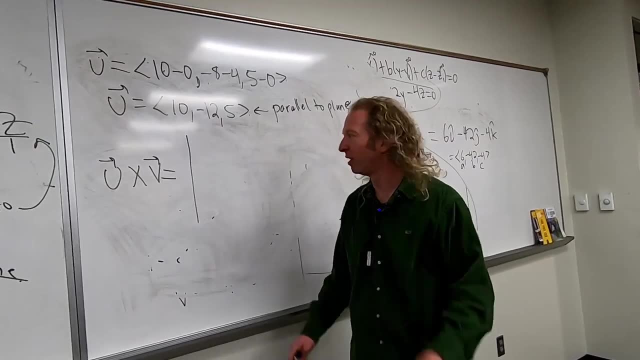 Professor, you said you were doing all of these on the exam Hm. You said you were doing all of these, All of them On the exam Mm-hmm. I'm pretty sure they're all there, Like every single type. 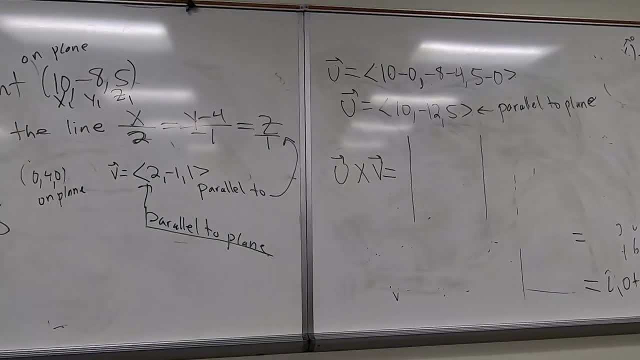 Every single type. yeah, I listed them though too. You have them. I posted them. Oh, you came in a little bit. I don't know if you came in late. Oh no, you didn't. Oh okay. 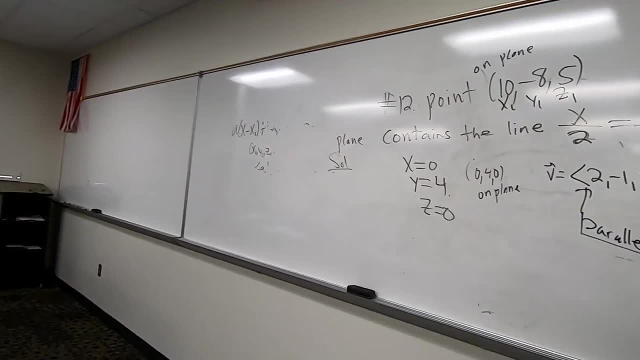 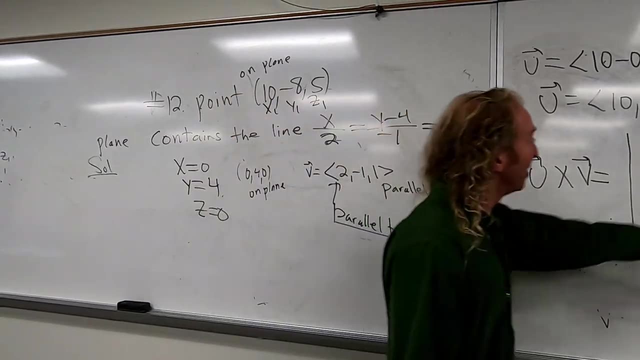 Oh, you said under resources. Yeah, you have the review questions. Yeah, Mm-hmm, Oh, someone's here. Hey, What's going on? Oh, Yeah, All right. So what goes in the? what goes in the first row? 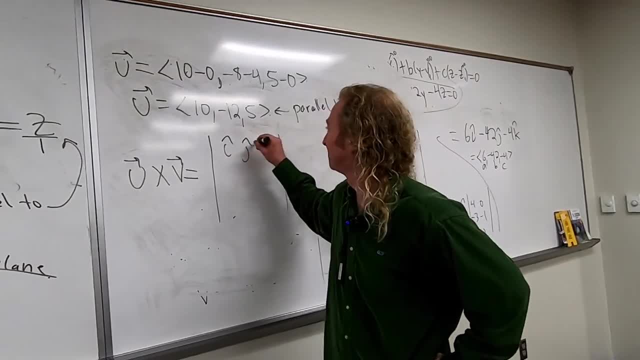 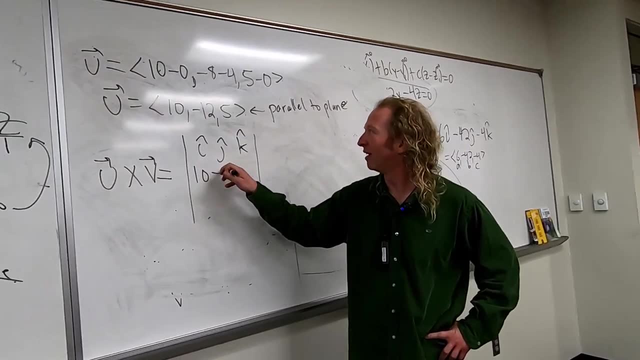 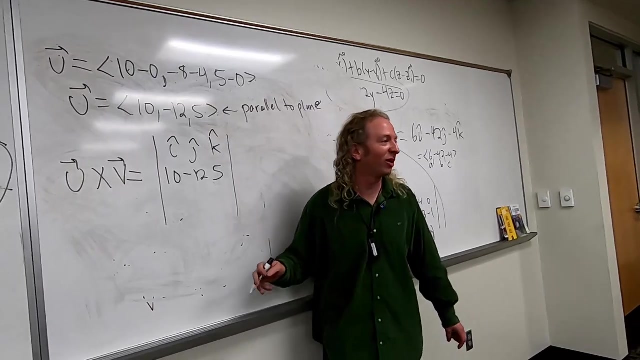 IJK, IJK. And then you put the U. It's your favorite thing, Isaac, And then V. V is 2, negative 1, 1.. 2, negative 1, 1.. So now we'll find the cross product. 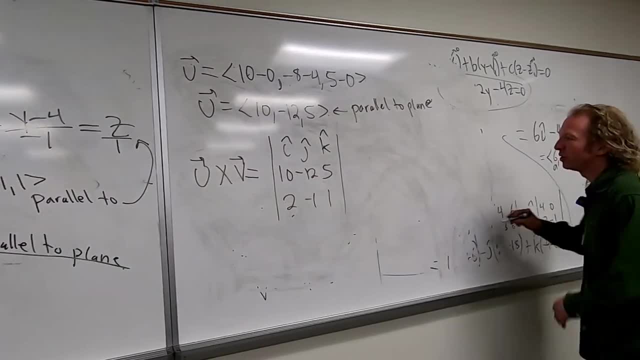 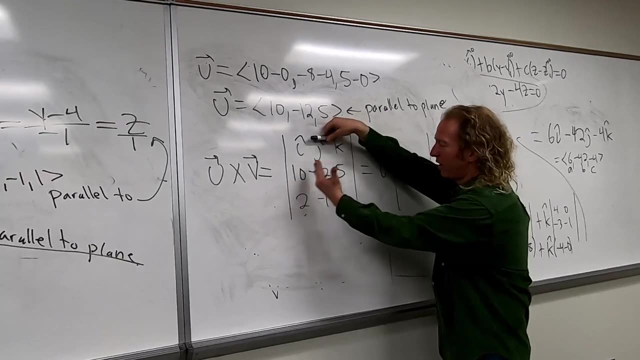 That'll give us a normal vector. right, That'll give us a normal vector, So let's do it. This'll be. I hat Cross out the corresponding row and column right. So negative 12, 5.. Negative: 1, 1.. 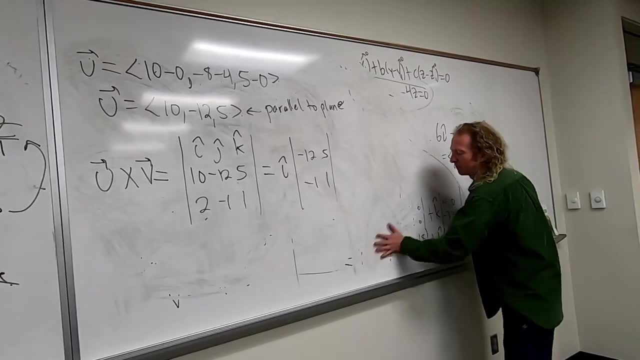 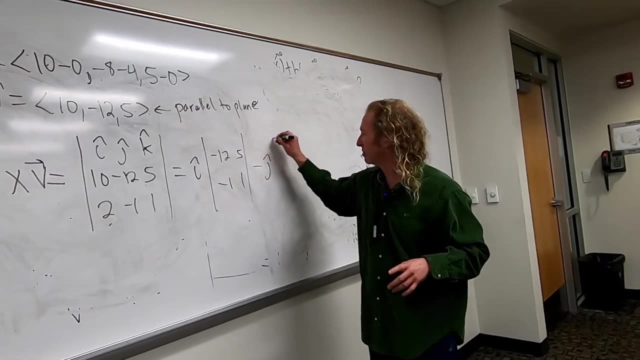 Negative 12, 5.. Negative 1, 1.. So erasers, Erasers, Erasers, Is the next one? plus, or is it minus, Minus, Minus, Minus? I always mess up there, So you cross these out. 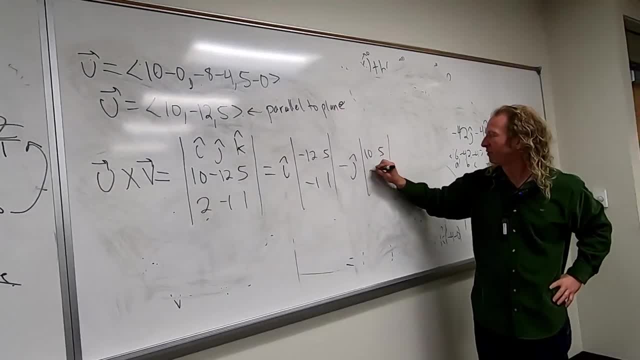 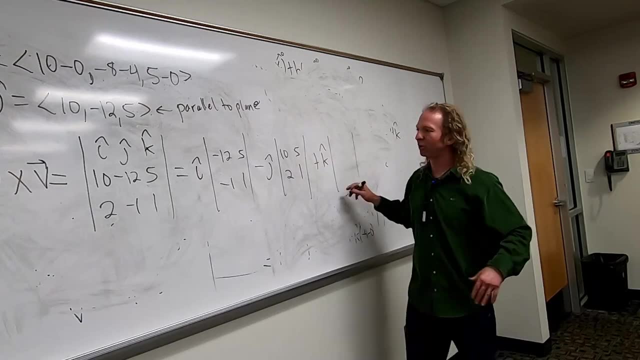 10, 5,, 2, 1.. 10, 5,, 2, 1.. And the last one would be plus. Cross these out: 10, negative, 12, 2, negative, 1.. So 10, negative 12.. 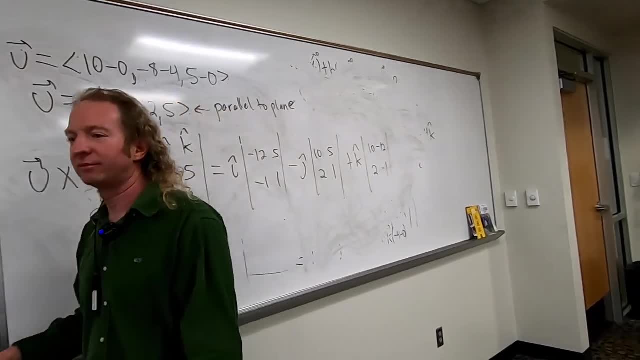 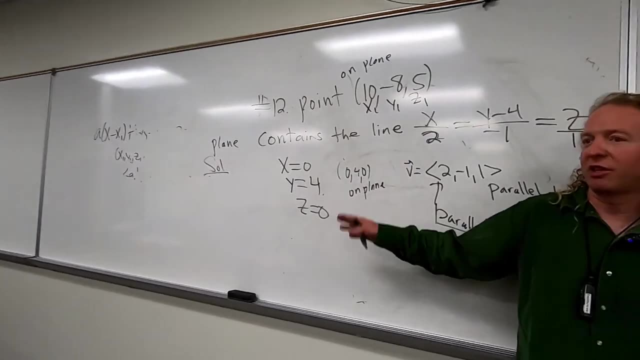 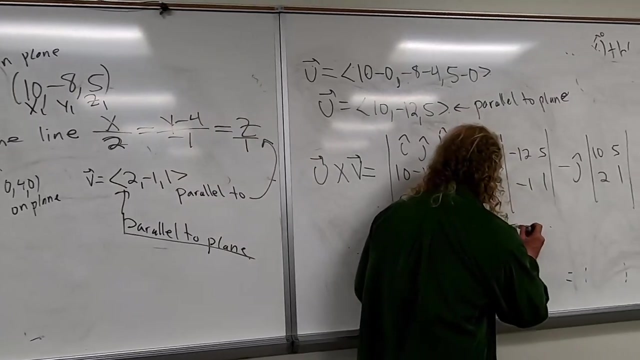 And then 2, negative, 1.. Okay, All right. Any questions so far on any of the logic? Everyone actually understand the logic. how we got the two parallel vectors. Okay, All right. Good, Let's finish this. So this is going to be. I hat. 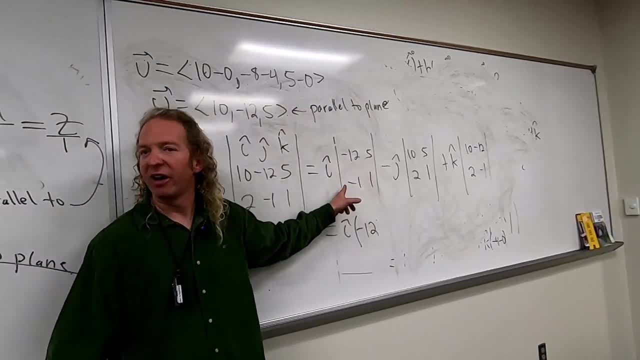 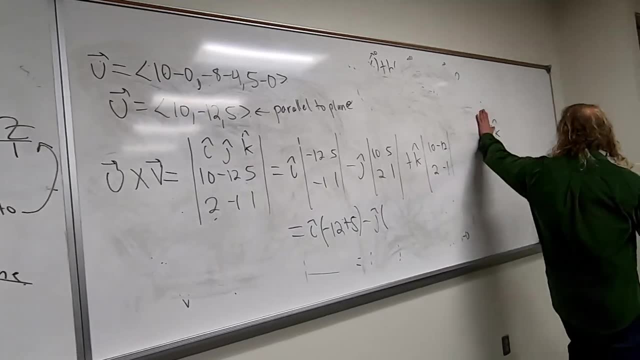 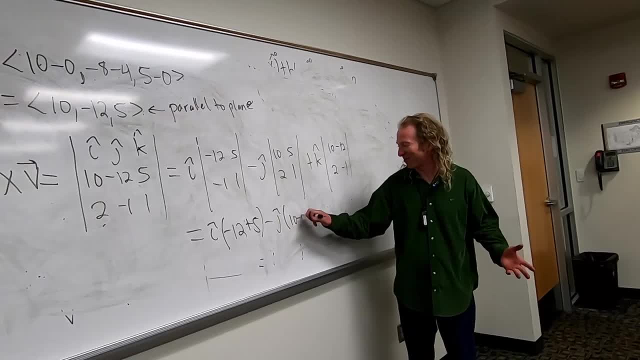 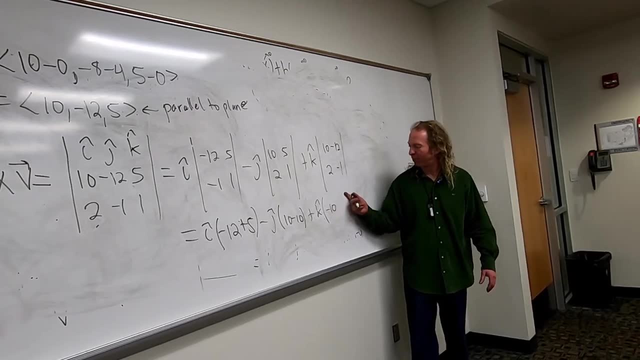 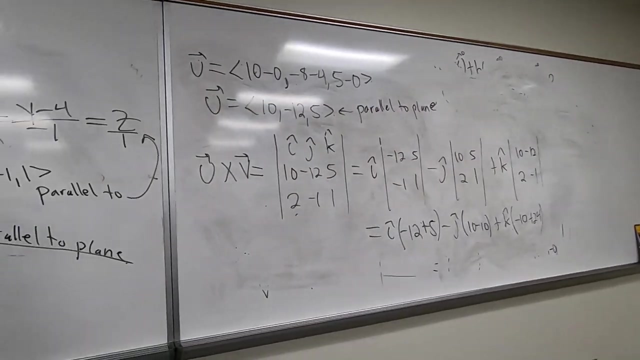 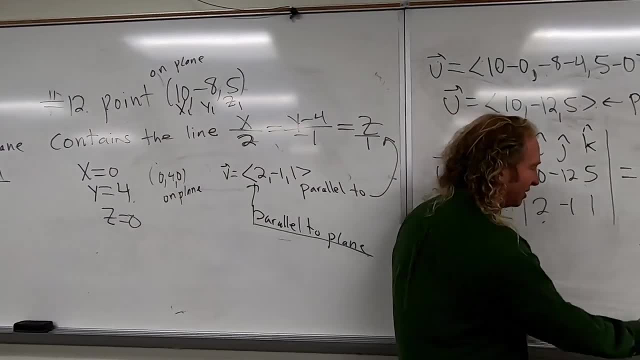 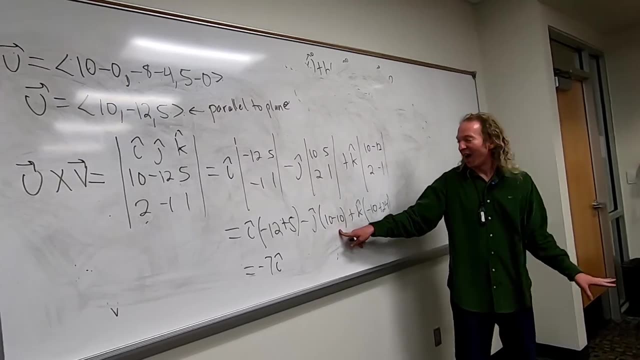 So it's minus 7 I hat. Yeah, Minus 7 I hat. Oh, That's gone, Right, I'm going to be weird, Watch this. Plus zero J hat. Zero, Zero, Zero, Zero Zero. 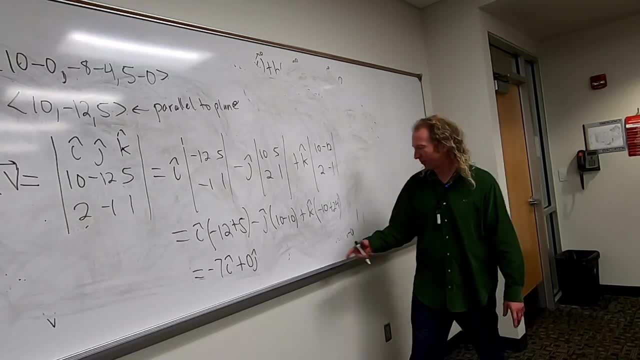 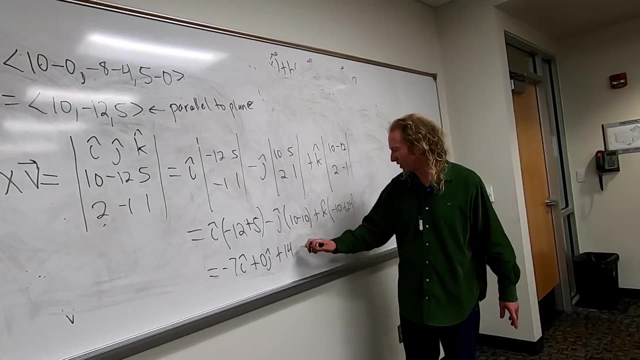 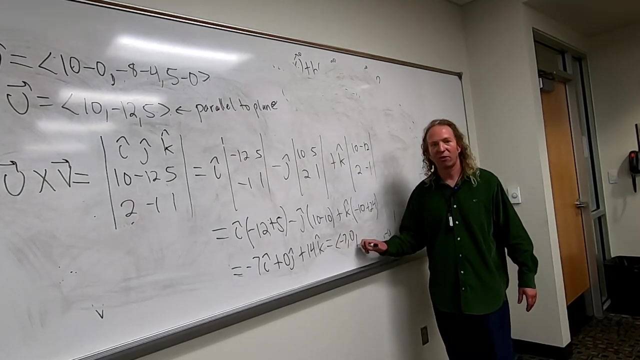 OH, Like orange juice Plus 14,, or the actor- He was an actor. Oh, J Simpson 14 K hat. And then so we get negative 7,, zero, 14.. Right, That's our N. That's our N. 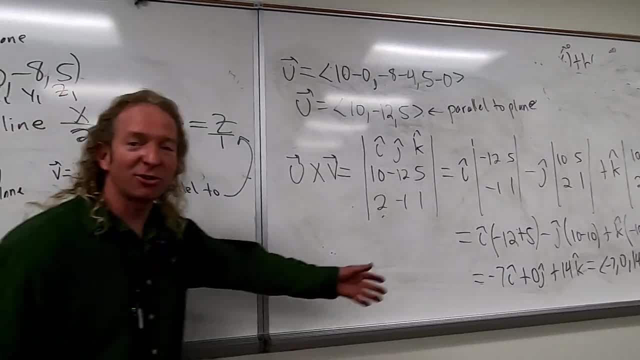 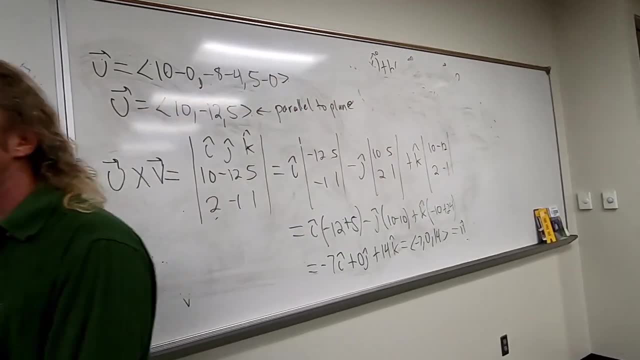 Yes, I forgot we were doing Thank you, That's our N. This is our normal vector. This is our N. Thank you, That's our N. That's our n. That's our n. So that's it. It's finished. 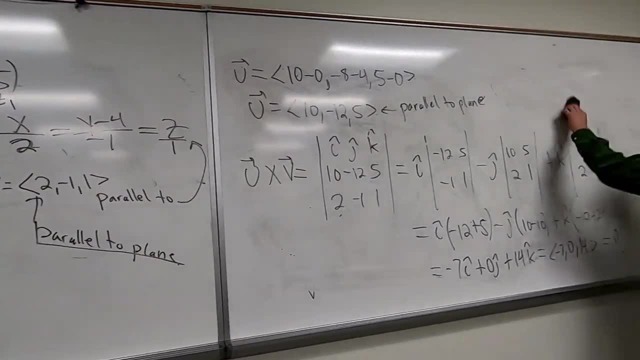 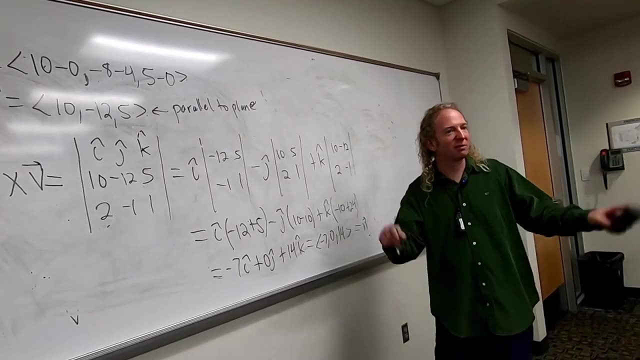 So to finish the problem we just plug it into the formula. The formula is way what's gone. It's a times x minus x1 plus b times y minus y1 plus c times z minus z1.. So this is our a. 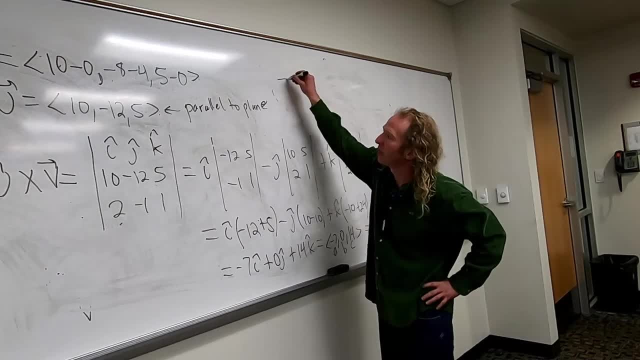 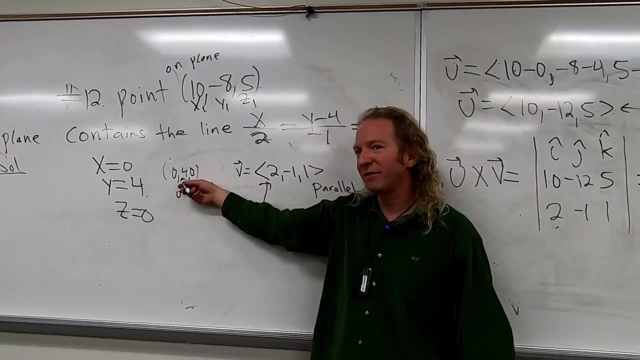 This is our b, This is our c, So it'll be negative 7. And we can use any point we like. Let's maybe just. oh, you know you could use this one, But since I already labeled this, I'm just going to use this one to avoid confusion. 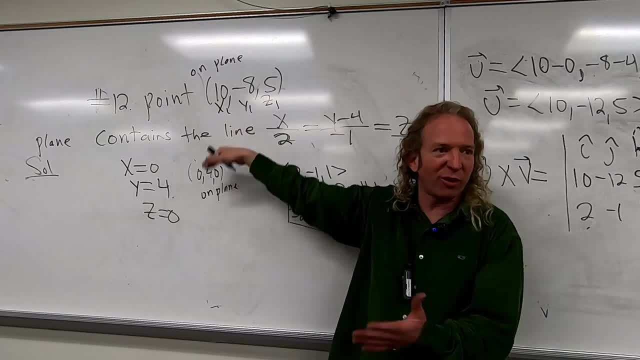 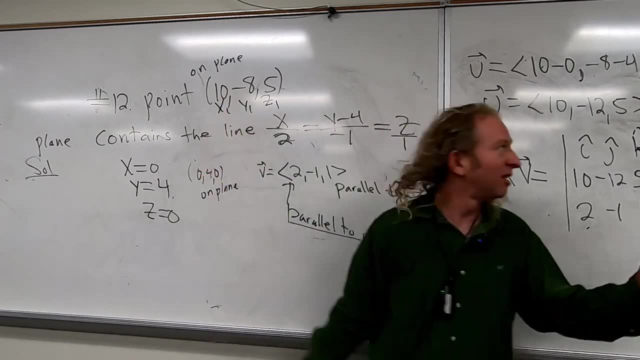 But you could use this one, right, But I don't want to like relabel things and erase things, So I'm just going to use this one, although it's easier to use this one. So x minus 10, right. 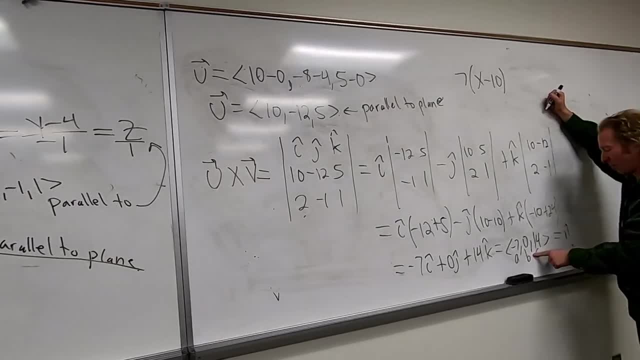 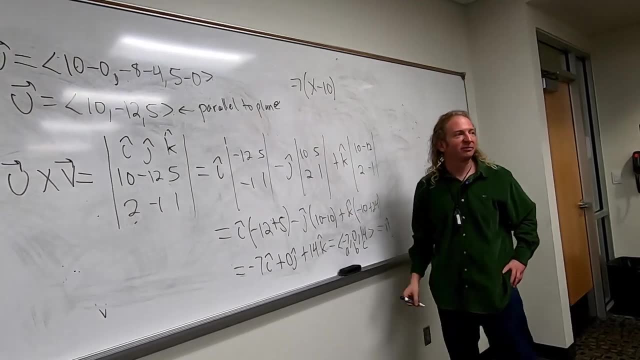 So x minus 10 plus 0. So I won't write that one, right? What's that? Yeah, negative 7? It's a negative. Do you want me to count that or not? Yeah, count it. Oh, why. 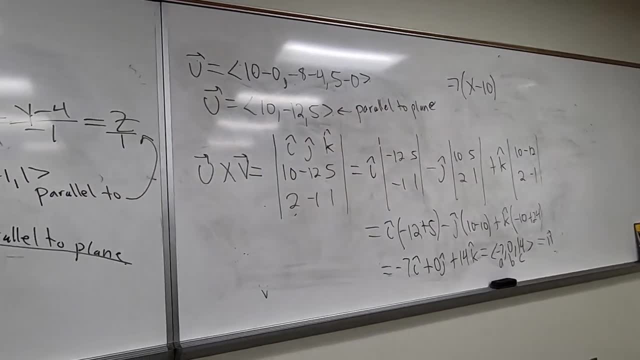 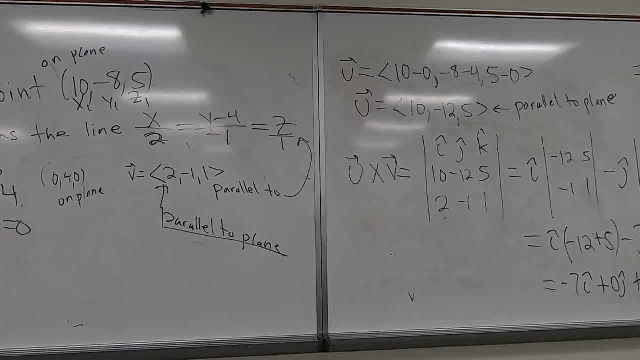 Did you give it to him? No, he called it from his side. Oh, okay, That's good, Thank you. Thank you, Udash. Don't forget to tell him the points. Yeah, Thank you. It's hot in here now. 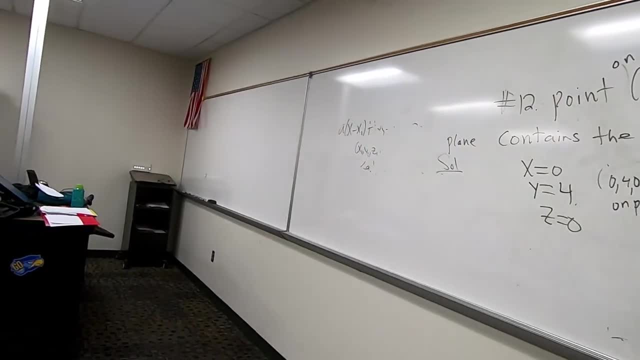 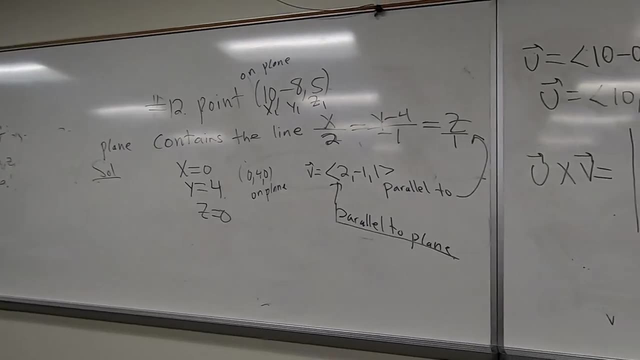 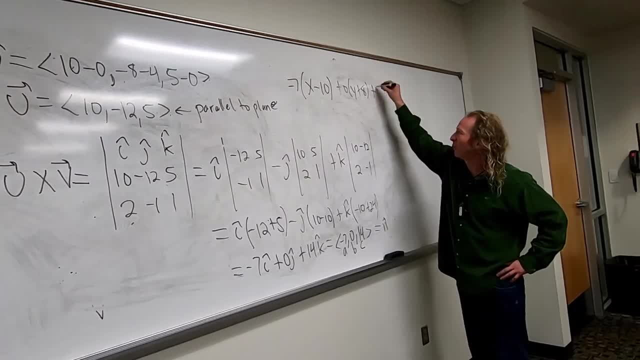 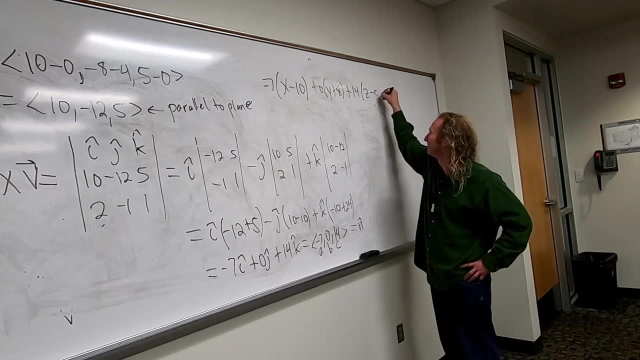 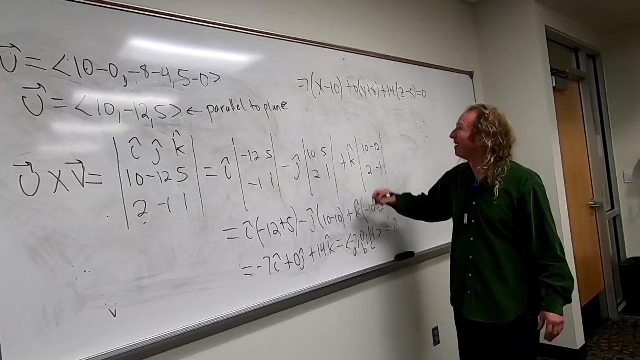 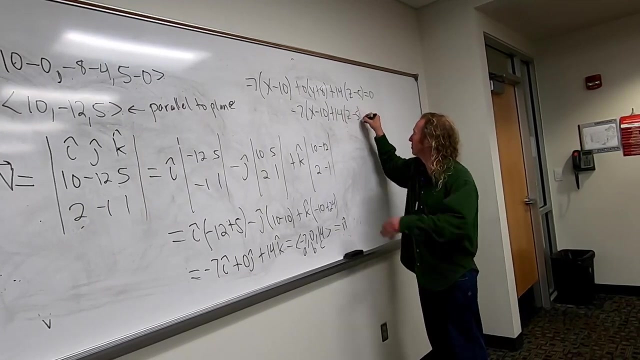 y plus 8 plus c c is 14.. z minus 5.. Don't leave it like that. Don't leave the 0 there. That's weird. No one does that. So this is negative. 7x minus 10 plus 14z minus 5 equals 0.. 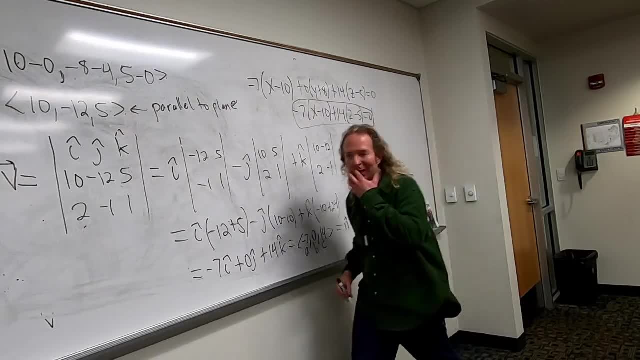 And I'll just leave it like this: You don't have to distribute. Yeah, Can you say this is a harder problem? Yeah, it's a harder one. You think it's hard, You don't? I mean, you do have to think. 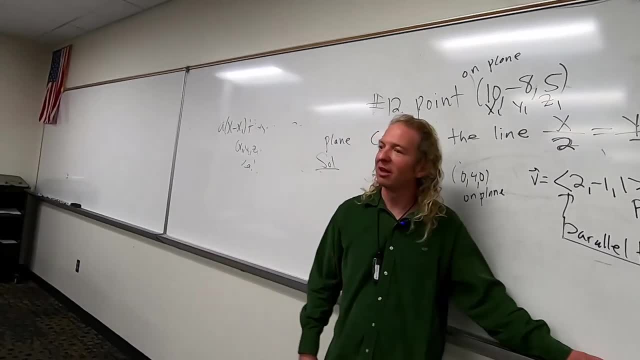 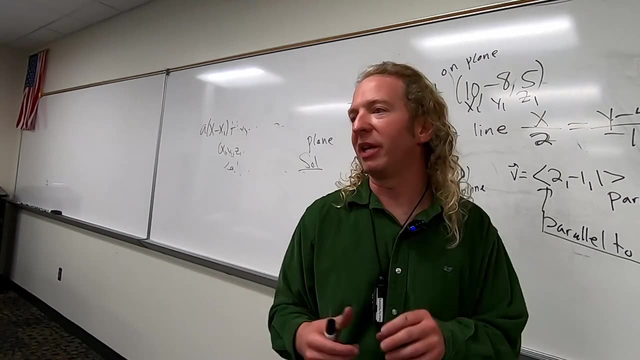 The theory is the complicated part, but what's the process? So when you use the points, you get a different equation for the plane, but it's still the same plane. It is because you can manipulate it and get the same thing. 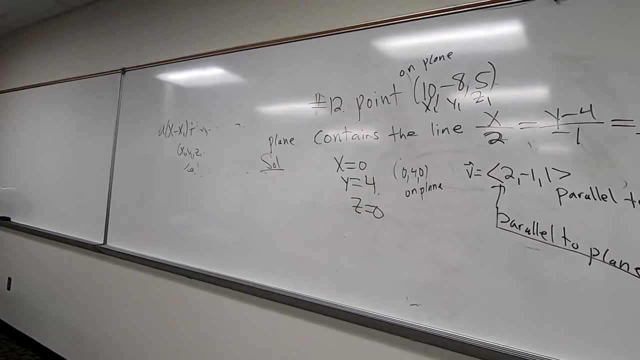 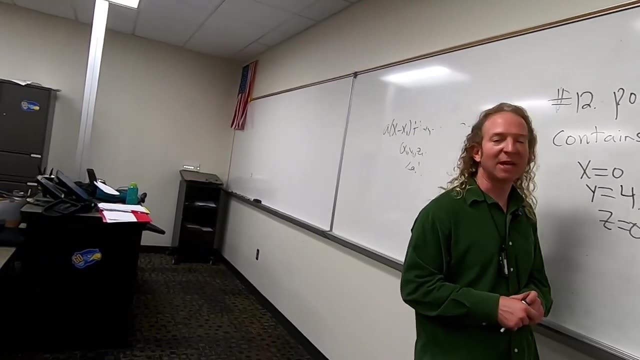 Oh Yeah, I can divide this by 2 and get the same thing. Yeah, it'll work. Yeah, Mm-hmm, It works. You can make them the same. Any other questions on this one? Yeah, this is the hard stuff. 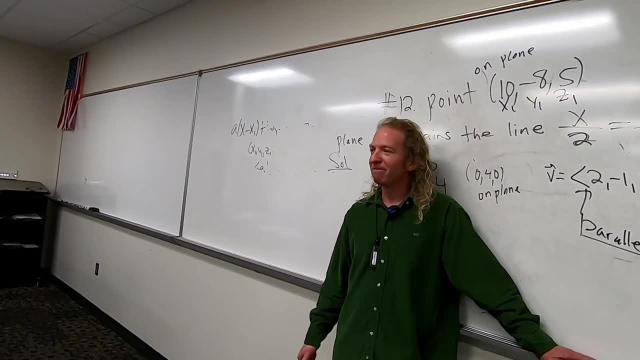 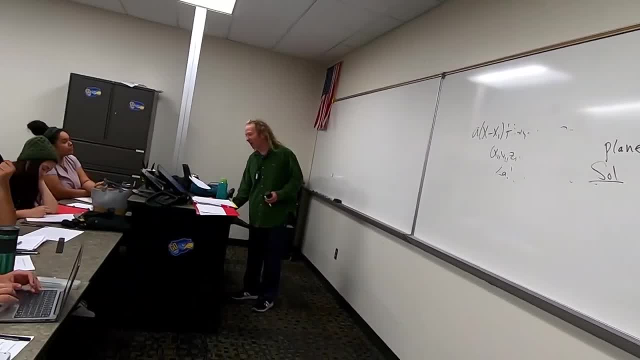 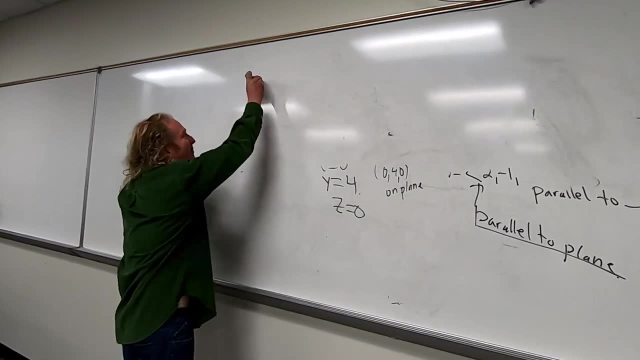 Let's see if you really think it's easy. Oh yeah, Number 13.. Yeah, Here we go. This one's a lot harder. Here we go 13. Game over, 13., Game over. So they give us a point. 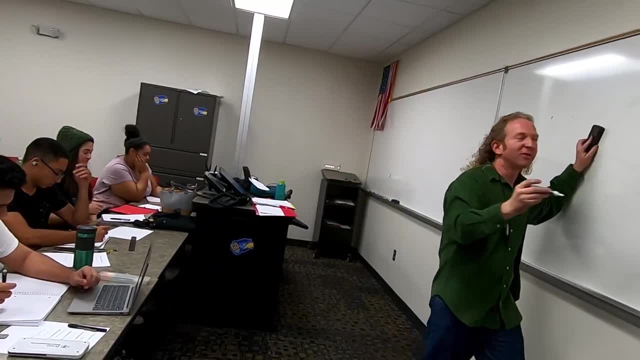 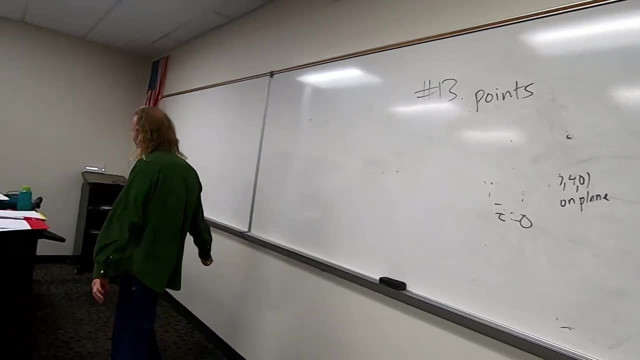 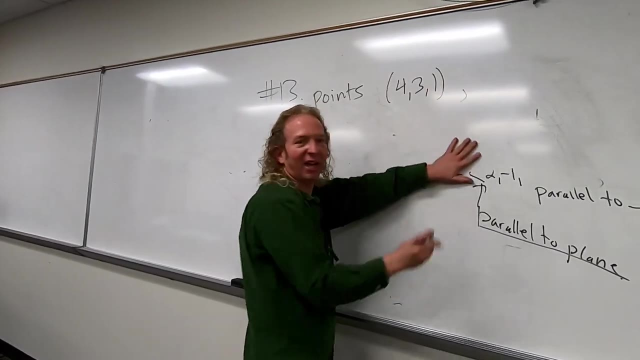 Oh, Oh, they give us two points. How nice of them. So points: The points are 4,, 3,, 1.. So points, These are points on the plane: 4,, 3,, 1. And 4, 1, negative 6.. 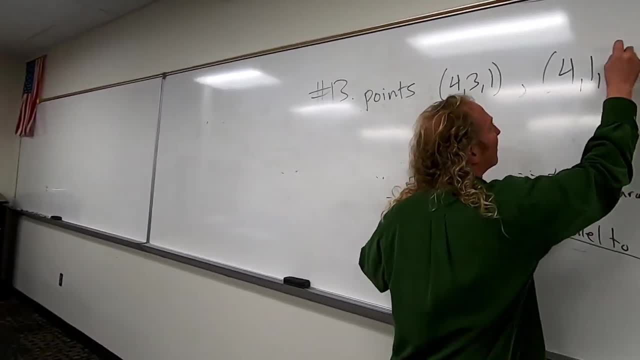 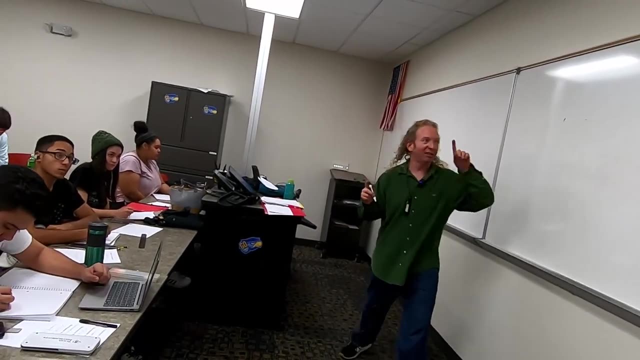 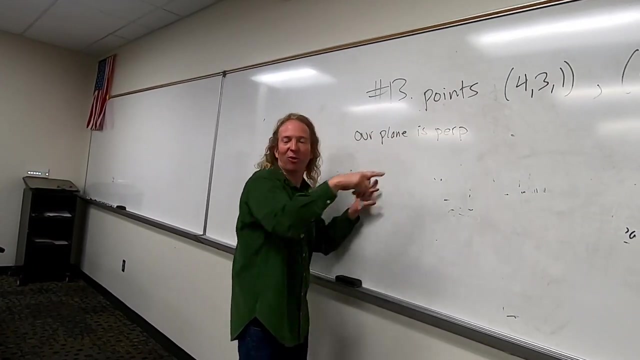 4, 1, negative 6.. 4, 1, negative 6.. And oh, they tell us that our plane, So our plane, Is perp. Now I'm paraphrasing the question right. I'm reading it. 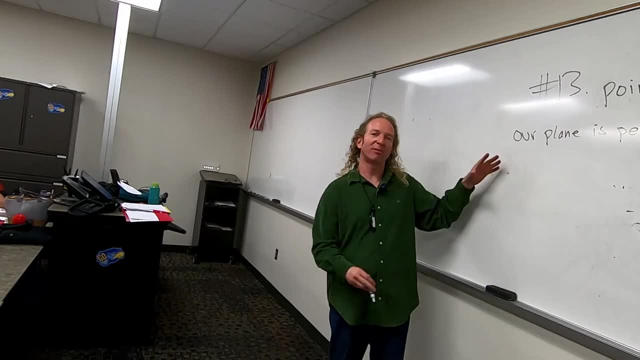 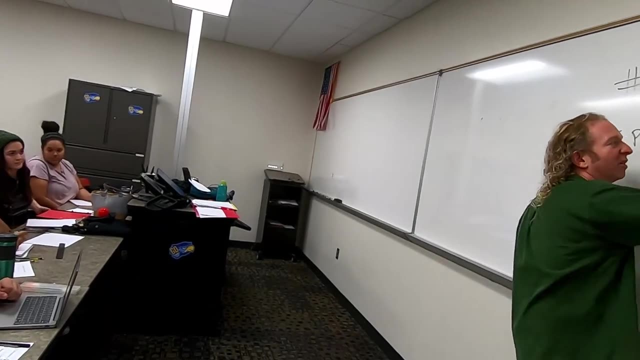 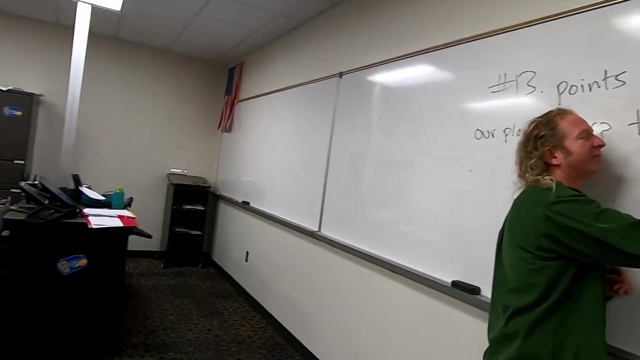 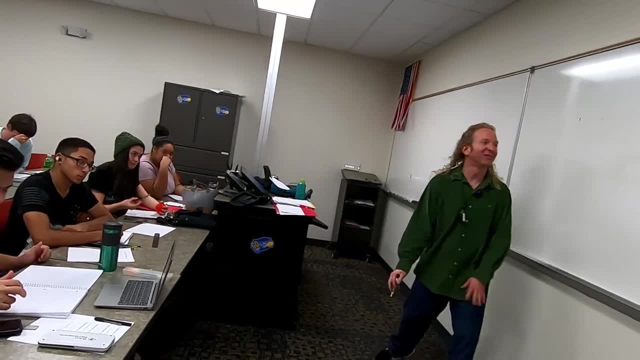 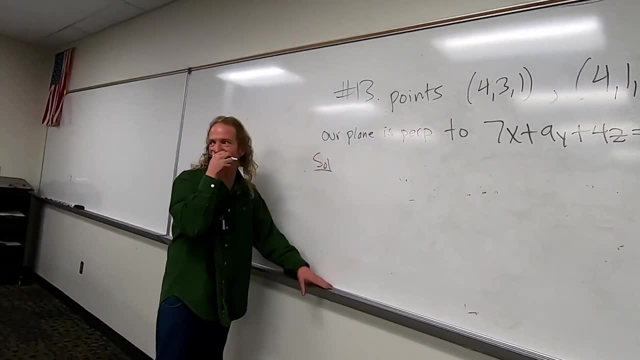 You don't have it up. Oh yeah, Oh yeah, It's 12.. It's 12.. All right, 12.. All right. Do you all want to try this one on your own, Or is that too much? 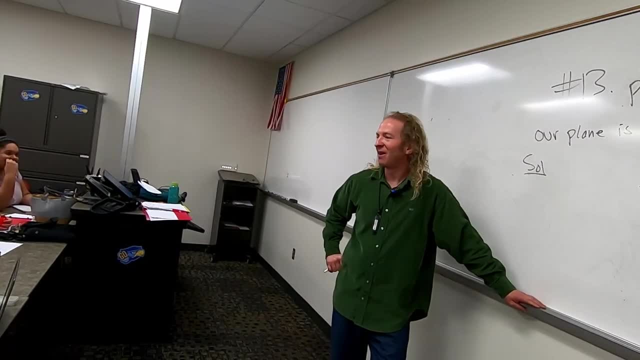 That's too much. Okay, I'll do it. I'll do it. You'll have a chance to try it on your own during the worksheet time. All right, This one's really hard. It's like the hardest one, All right. 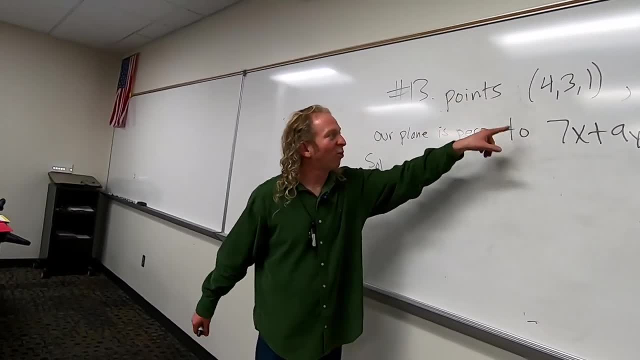 So we have two points on a plane, Even before we read this. what can you do when you have two points? What can you do when you have two points? What can you always do? You find what A, what, What kind of vector. 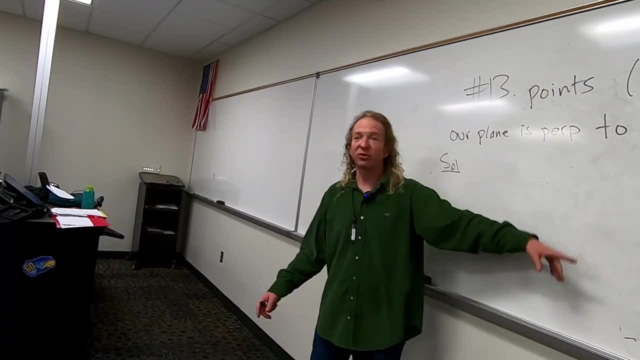 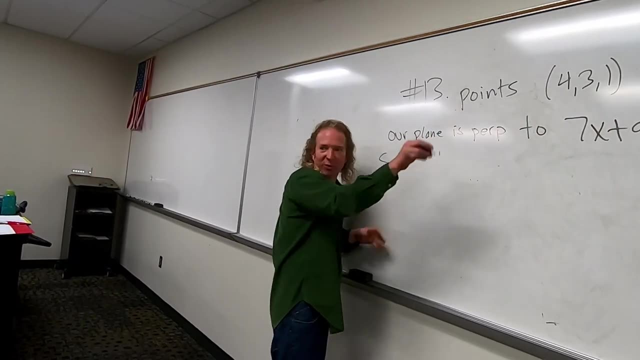 A parallel vector. Yeah, so given two points in the plane, you could find a parallel vector, right. So let's do that first. So I mean let's just even before we read the rest of the question. So I'll call it v. 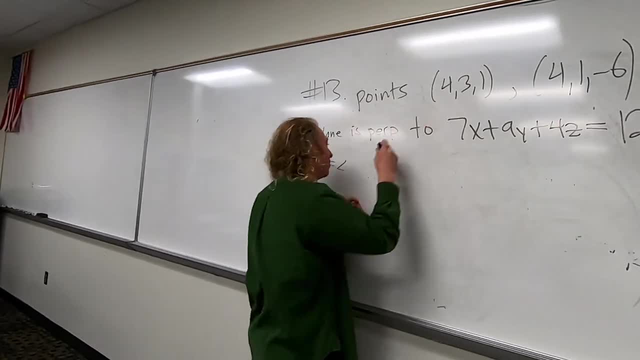 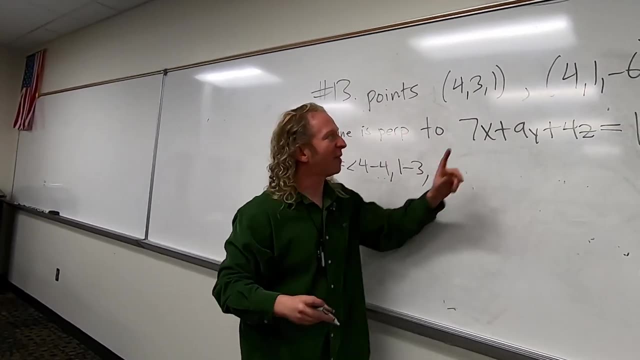 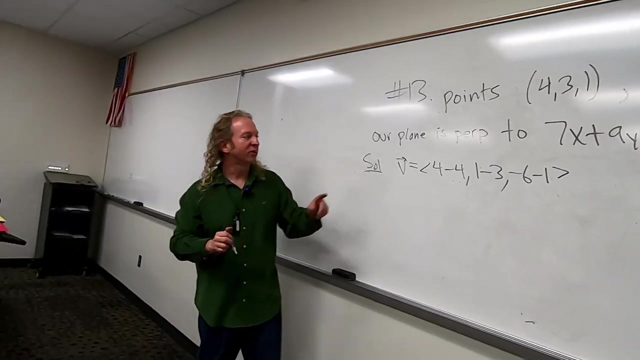 So we could do, I'll do this: one minus this one, okay, So four minus four, And then one minus three- Okay, one minus three, Yeah, this is really hard. And then negative six minus one- Okay, All right, so that's going to give us v. 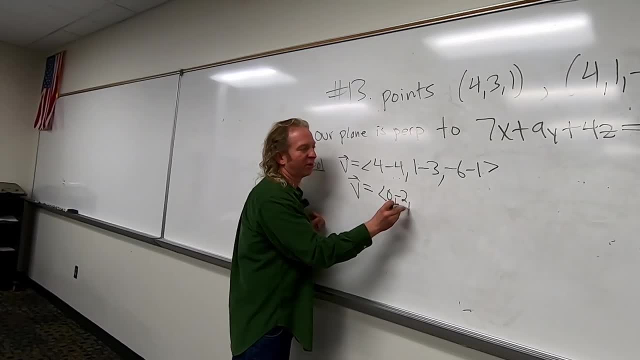 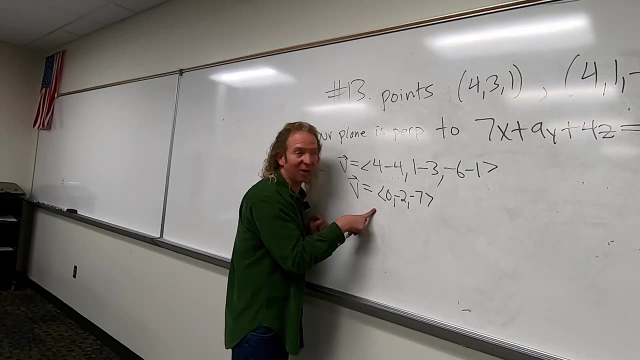 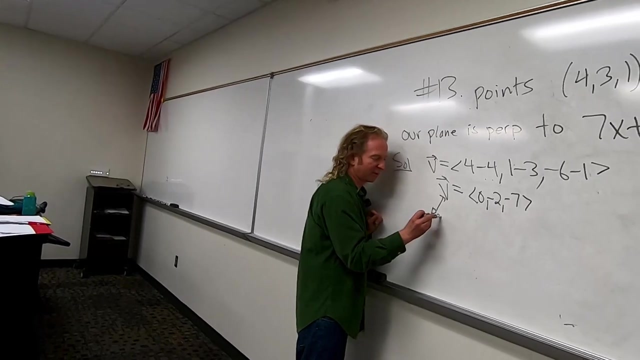 This is zero negative two negative seven, And this is on our plane. right, Because these points are on our plane, We connected, so now we have a parallel vector, This is parallel to our plane. Are we going to use this? 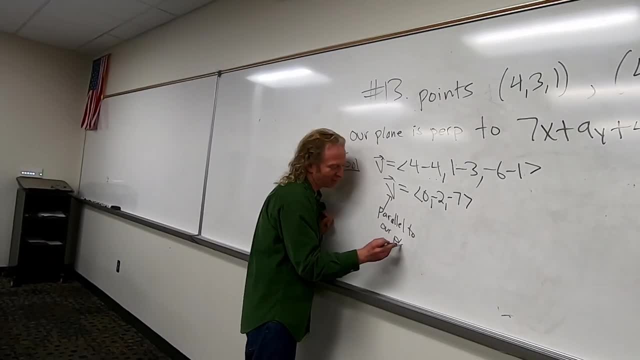 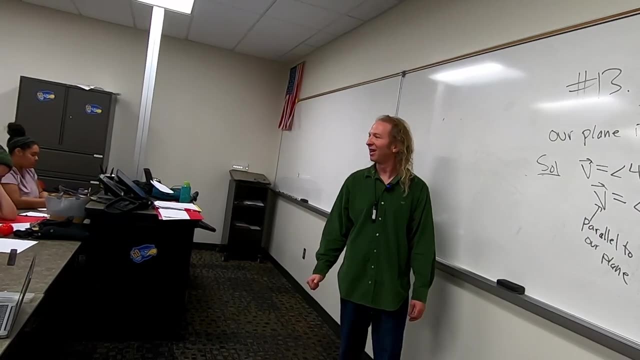 Probably right. It's a math problem, Like I mean we can assume we will. It's a math class, Like the problem has a solution. What's that say It's a two-tag, so Oh, Just tell them it's on. 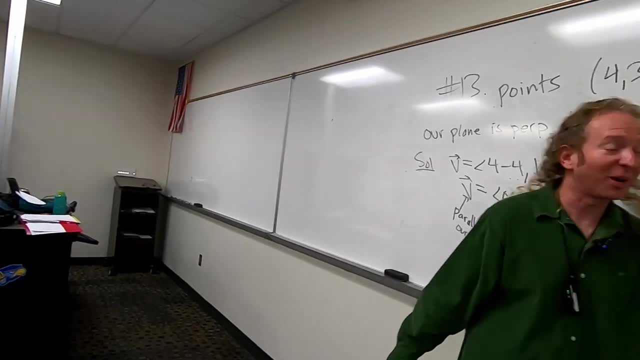 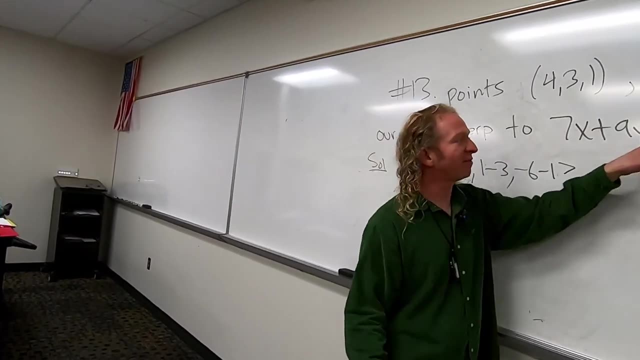 Oh okay, Oh right, right, Okay. so this is parallel to our plane. All right, so our plane is perp to this. There's a vector here: seven, nine, four, right. Seven, nine, four. 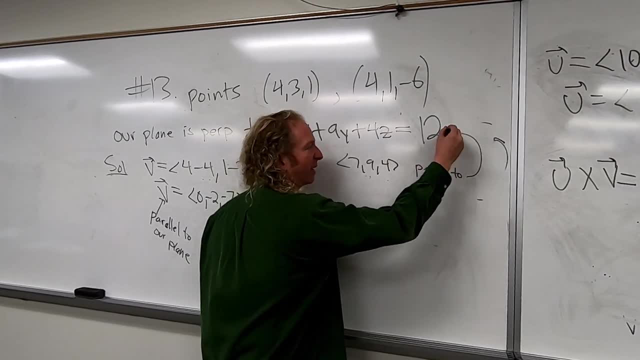 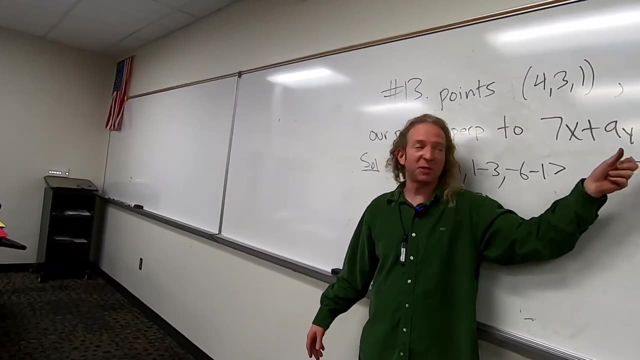 This is perp. This is perp to this plane, right, Right, remember that's from A, B, C, Remember you can just get them from here. This is perp to this plane, Not perp to our plane. 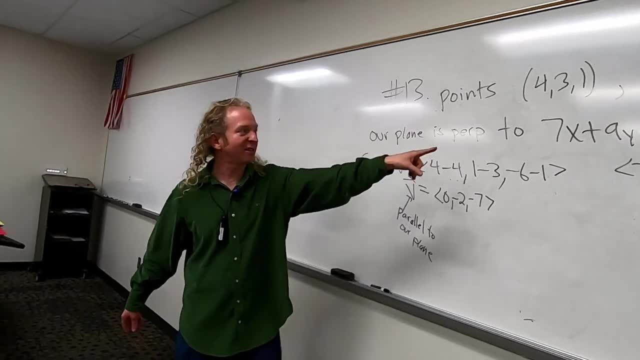 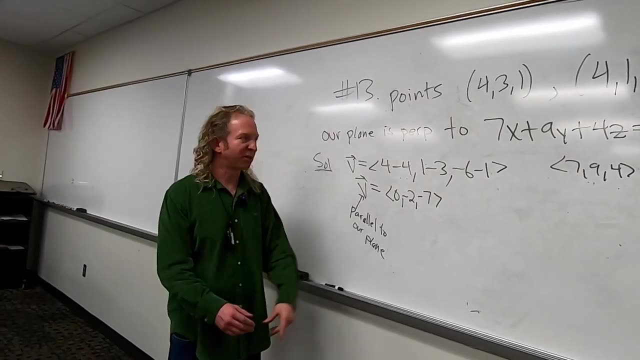 No, no, It's perp to this plane. So pretend that seven x plus nine y plus four z. Pretend that's the board, right? Pretend that's the board. This is the board. This is the board. This is the plane. 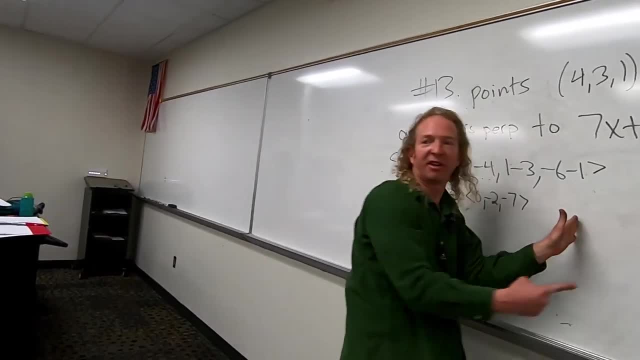 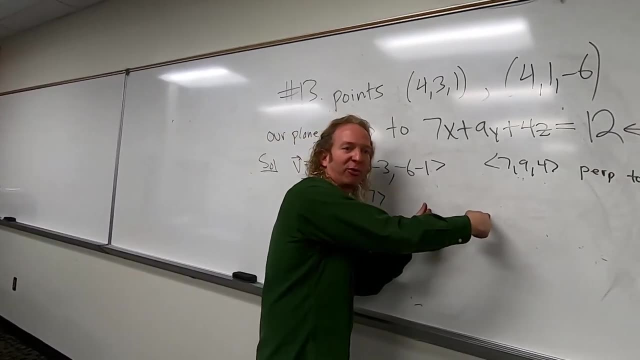 Our plane is perp to the board. This is the vector. This vector needs to be longer. This vector is perp to the board. What can you say about the vector and the plane? They're both what Parallel. So if our plane is perp to the board and the vector is perp to the board, 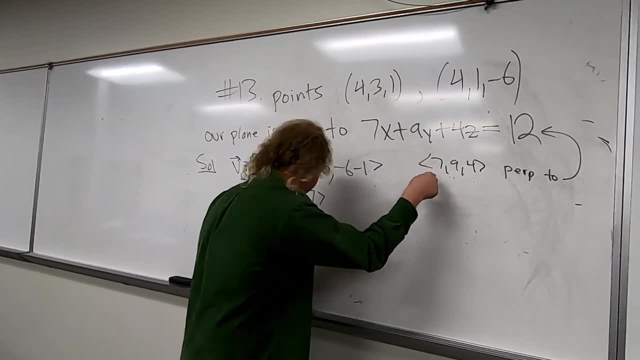 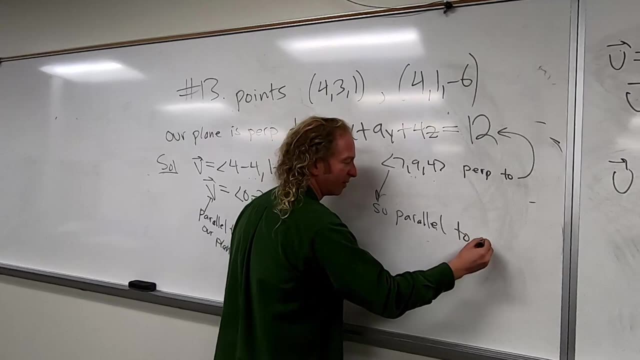 then our plane is parallel to this vector. So this is parallel to our plane, So parallel. I'll explain it again. It's hard, It's beautiful to our plane when you understand it, When you don't, it's horrible. So I'll explain it again. 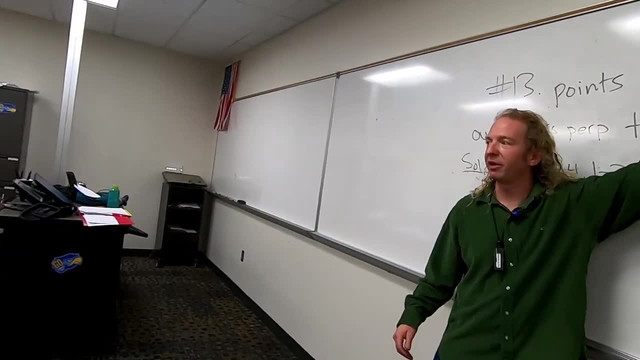 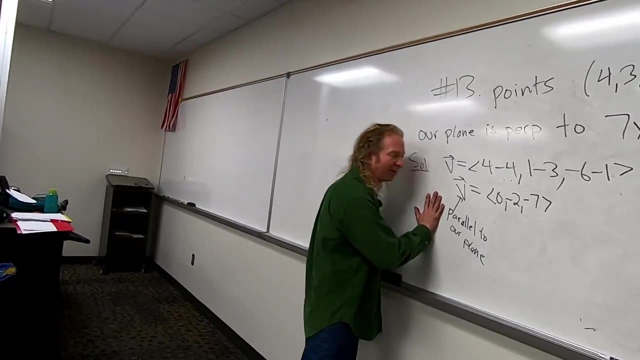 So this was easy, maybe right. We have two points on the plane. We can do terminal minus initial and get a vector on the plane. So we have a parallel vector, Boom, Parallel to our plane. We are told in the problem. you have to read the question. 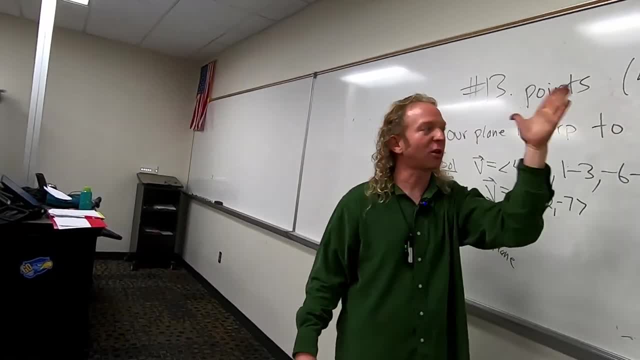 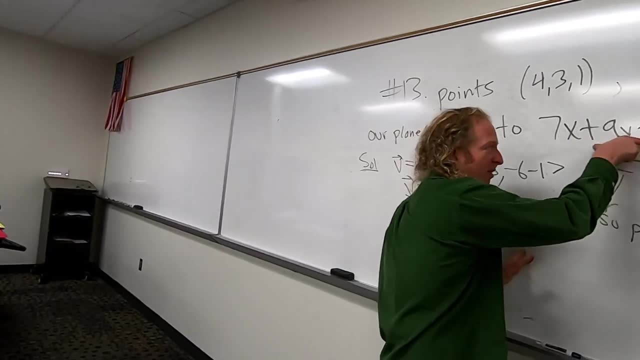 it says that our plane is perpendicular to this plane. So this is our plane. my hand, This plane here, is the board, So our plane is perp to it. But this vector is perp to the plane, So our plane is perp to the plane. 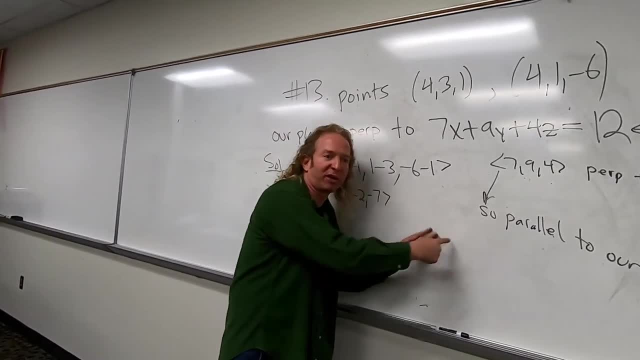 The vector is perp to the plane. Therefore, the vector is parallel to our plane. So that's how you get that. When we have two vectors that are parallel, what can we do to get a perpendicular one? What do we take? 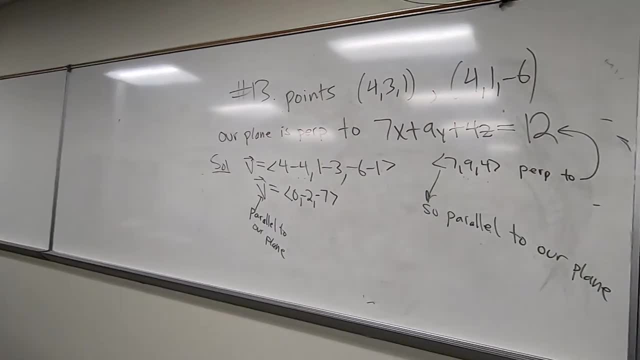 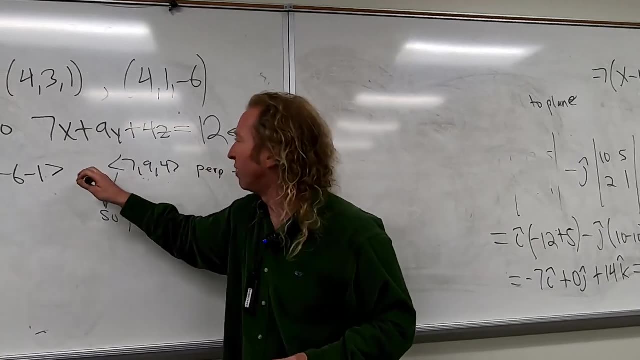 The cross product right. So this is hard. This is considered very difficult. This is like conceptually hard. So let's finish So we can do u cross v. I guess I'll call this. u Give it a name, right. 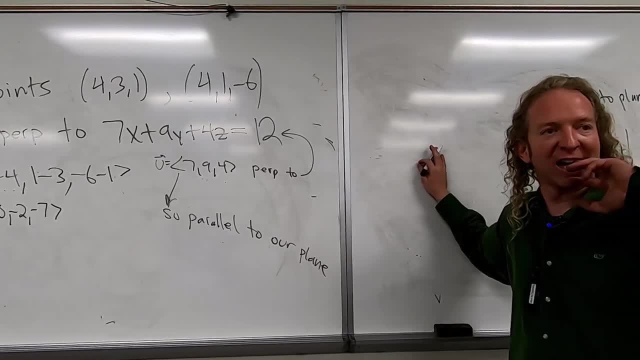 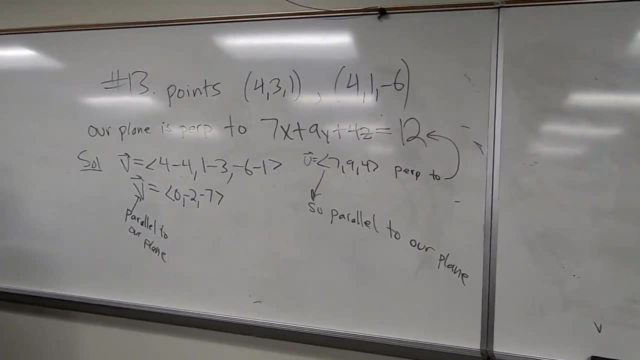 I'm going to give it a name. Yeah, So when you take the cross product, that just gives you the n vector. That gives you the n vector Every time, Every time. In this case, it does, Yeah, Does it matter which order we cross the n? 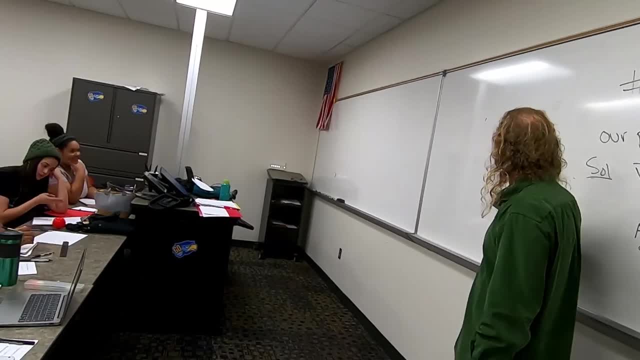 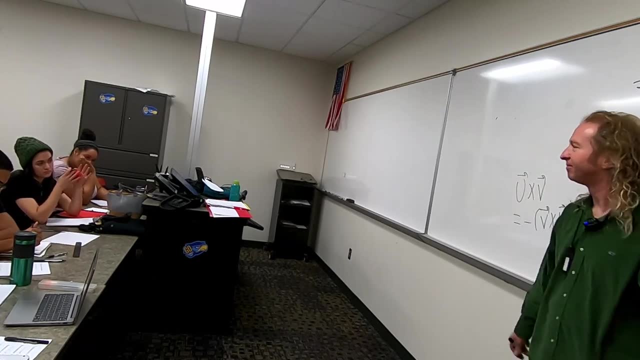 No, you don't, Because remember- very good question, Michael- Because remember u, cross v is equal to negative v cross u. So you just get a vector in the other direction, All right. so All right, let's finish. 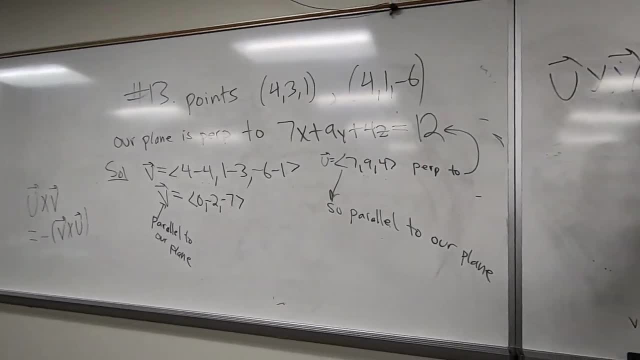 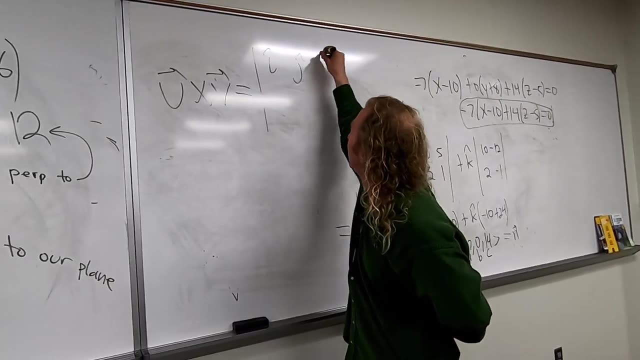 So u cross v. So yeah, it doesn't matter. So we have: i j k, i j k Any questions on this. Everyone gets it No one's confused. That was like the hardest one, I think. 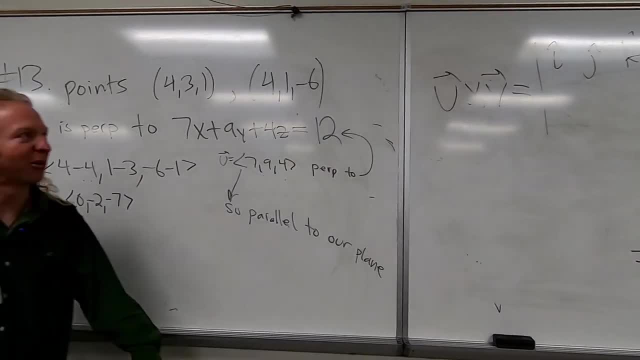 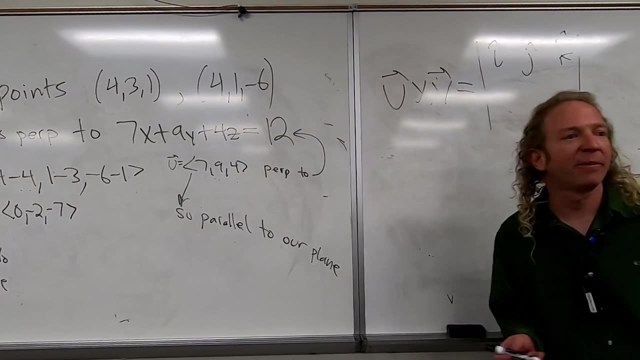 So does it make sense, Gerardo, Does it make sense? I just picked on you because you were there. Okay, So i j k. So u is 7, 9, 4.. Yep, 7, 9, 4.. 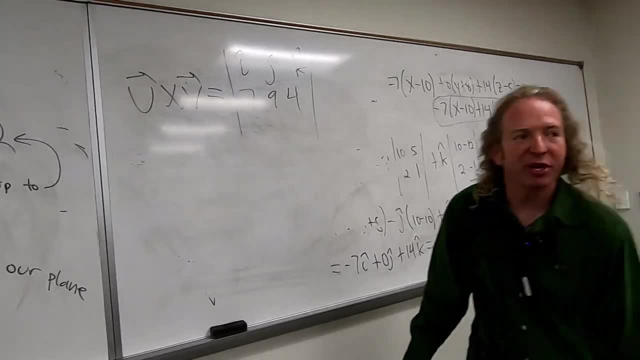 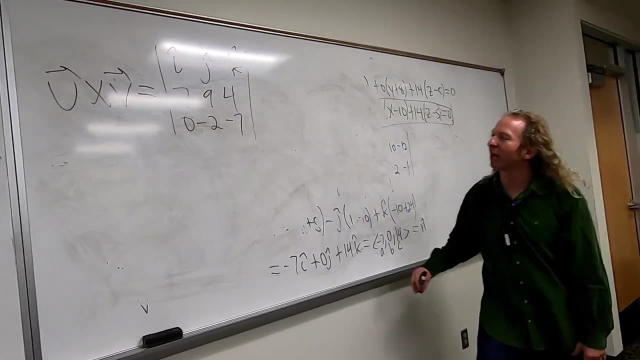 It's marker's starting to fade And v is 0, negative, 2, negative 7.. So 0, negative, 2, negative 7.. All right, let's do it. So you have. i hat boom boom 9, 4, negative, 2, negative 7.. 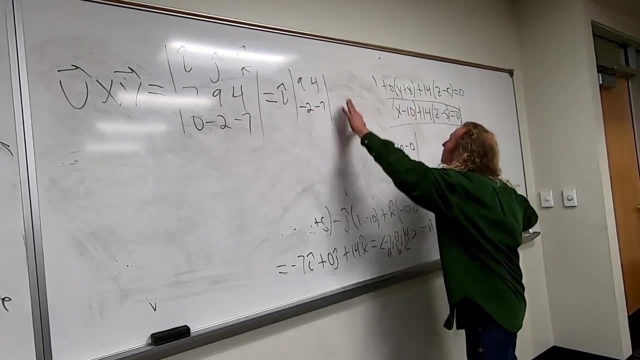 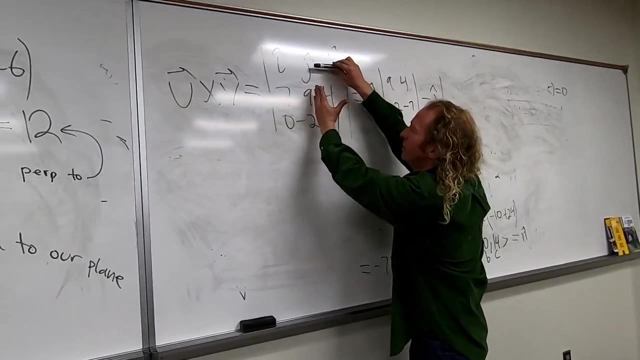 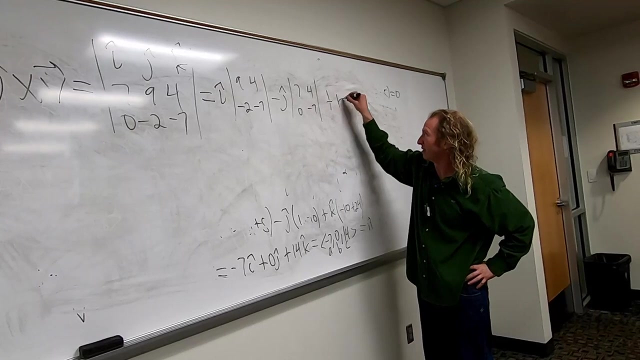 So 9, 4, negative, 2, negative, 7. Minus j hat boom: 7, 4, 0, negative, 7.. 7, 4, 0, negative, 7.. Plus k hat: 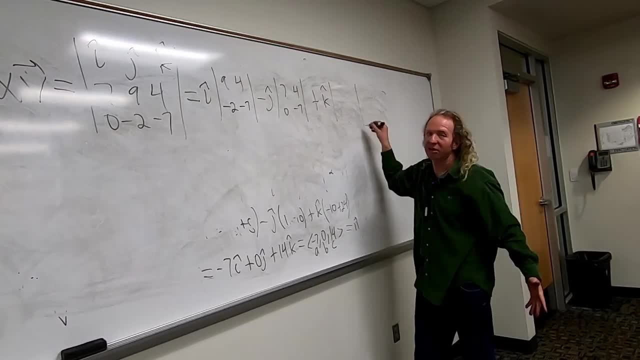 It's good you all have extra credit too. I mean it's good There's no extra credit on the test. So I mean there's no harm by you know, Yeah, yeah, so it doesn't really matter. 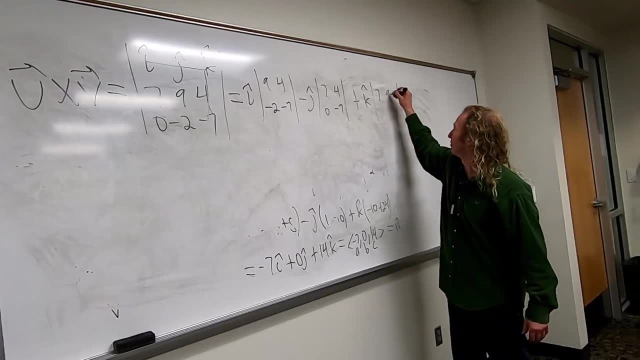 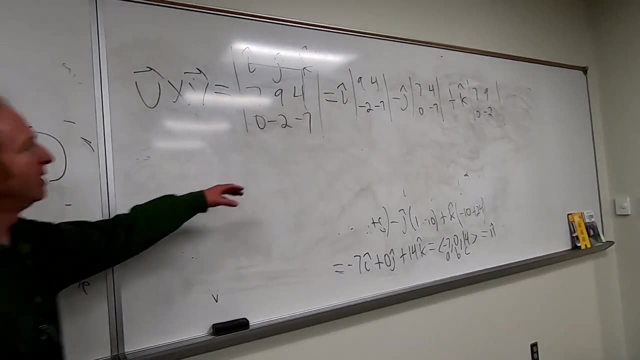 7, 9, 0, negative 2.. 7, 9, 0, negative 2.. So we're there. Let's clean this up. This is i hat, i hat. oh, 7 times 9 is 63.. 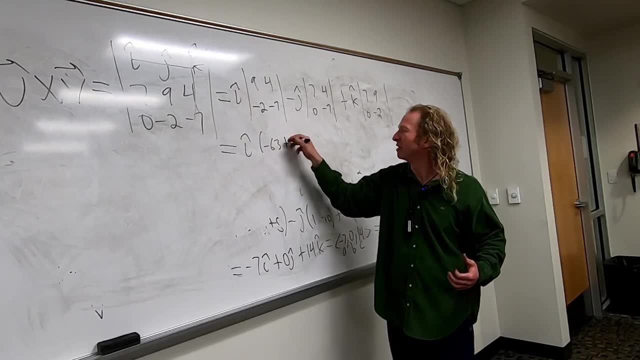 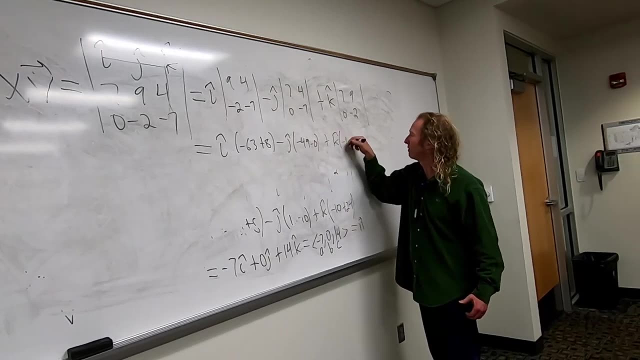 And it's negative 63 plus 8. Ridiculous. Minus j hat Negative 49 minus 0, going fast. Plus k hat Negative 14 minus 0, went really fast there. I think we've done a lot of cross products today already. 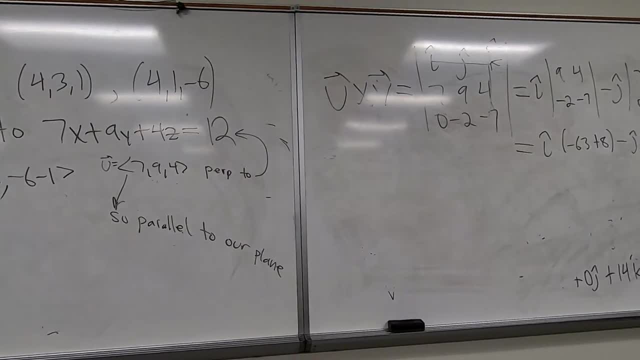 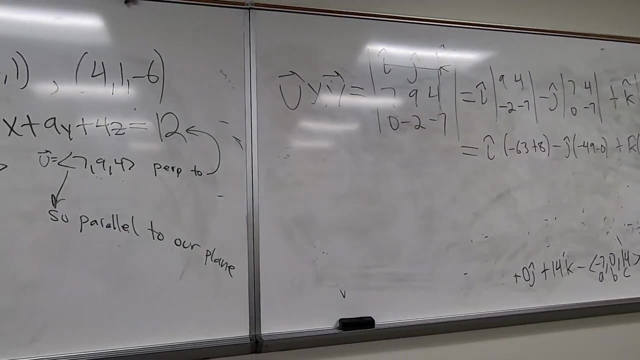 So this is cross products. Everyone okay with the cross products. I did that really fast. That's the fastest cross product I've done all semester. So, feeling kind of guilty, You can get a better marker. What's this? That was red. 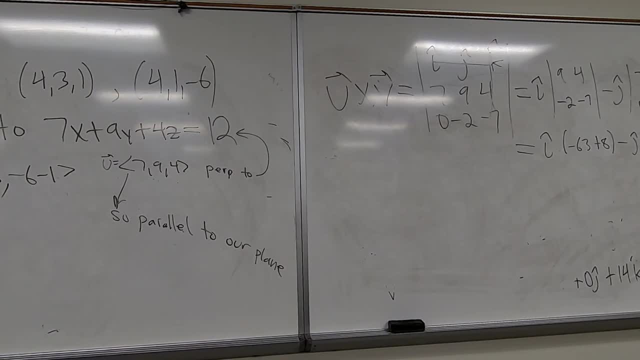 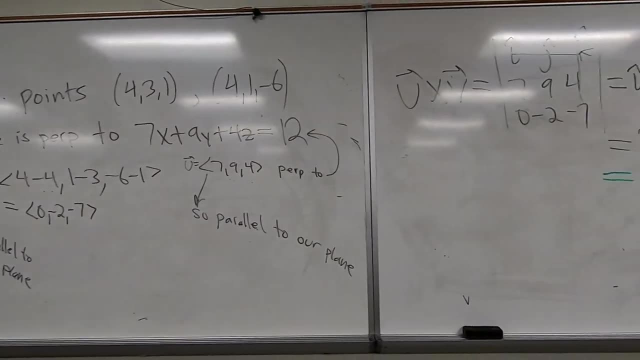 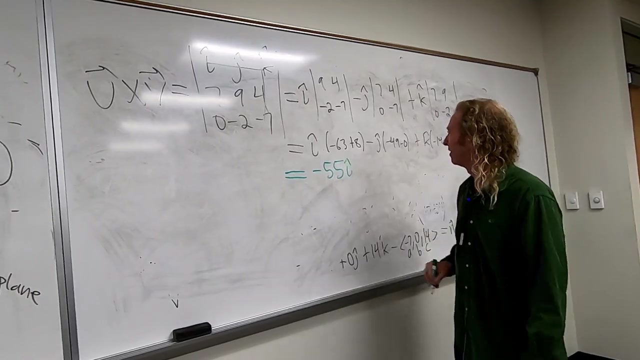 What's this? Ugh, There you go. It's like Christmas trees. All right, So this is equal to What's negative? 63 plus 8? 55. 55,, okay, negative 55,. i hat plus. can you see that okay? 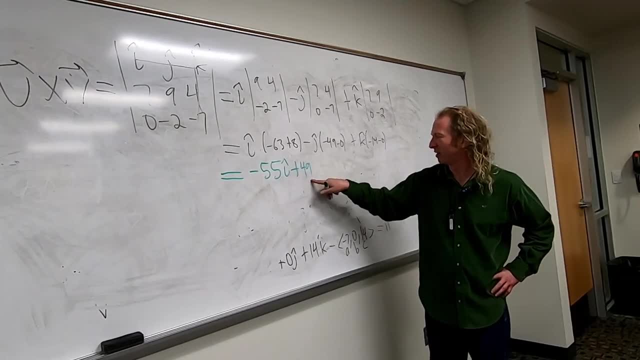 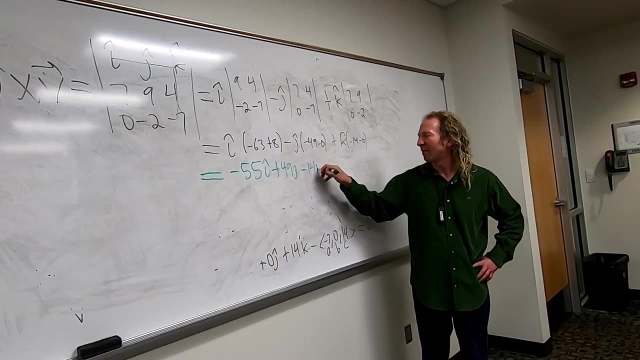 Yeah, I don't like it. I should go back to the. I'll switch back in a minute. I don't like it. Minus 14k hat. minus 14k hat. I'm going to write it in component form. 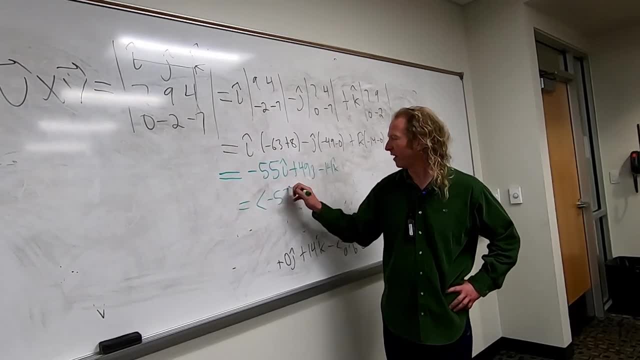 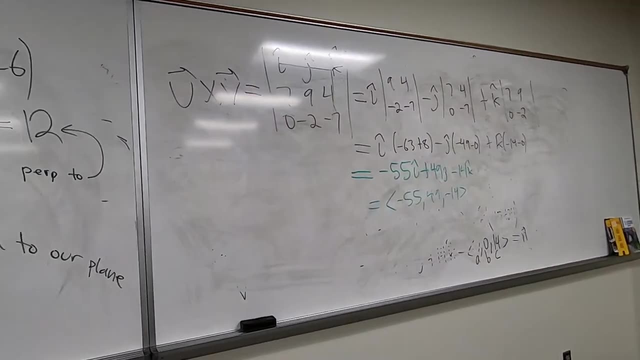 I don't like this notation, So this will be negative. 55 comma 49.. Comma negative: 14.. Let me get a better marker. So what is that? What did we just find? What is that called? That's our normal vector. 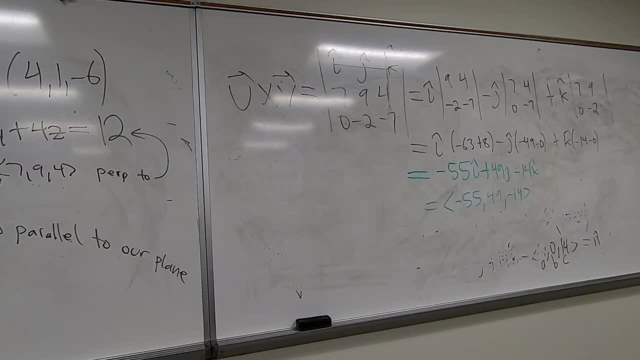 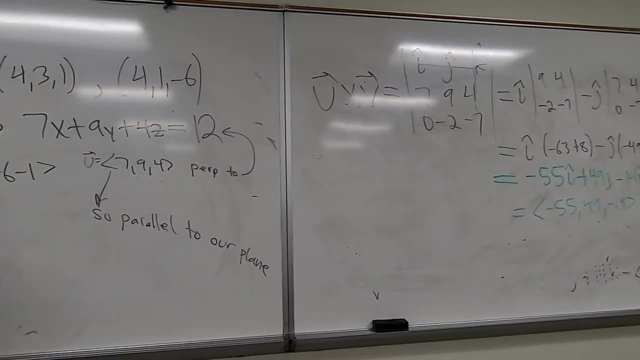 Very good. It's our normal vector. I think this is the hardest problem in all of the homework. I don't think there's anything that's harder right in the homework. So now we have our normal vector. So this is our ABC, ABC. 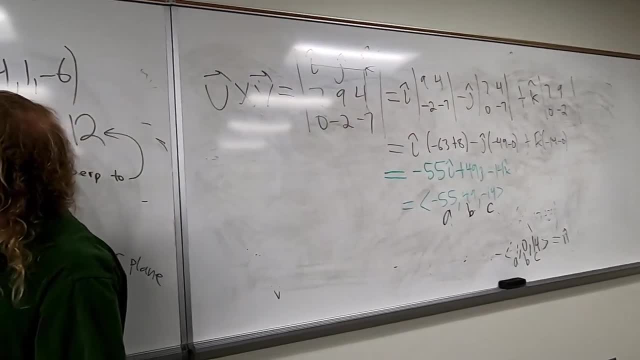 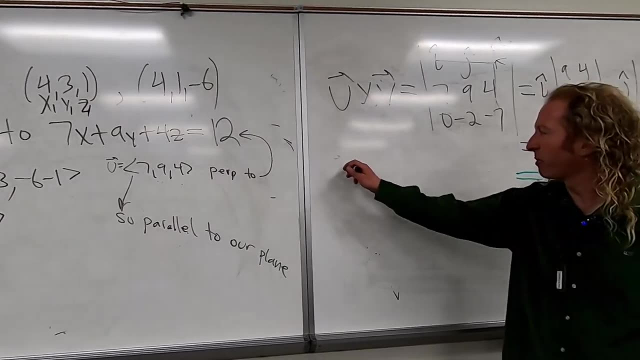 And now we can use the formula. I'll just pick this one, That's X1, Y1, Z1.. It doesn't matter which one you choose. It doesn't matter which one you pick And let's do it. So I'll write the formula down this time. 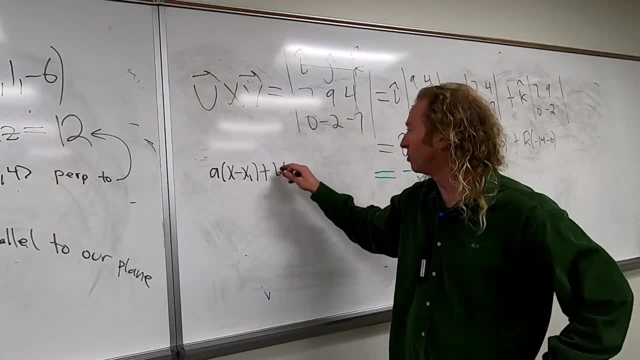 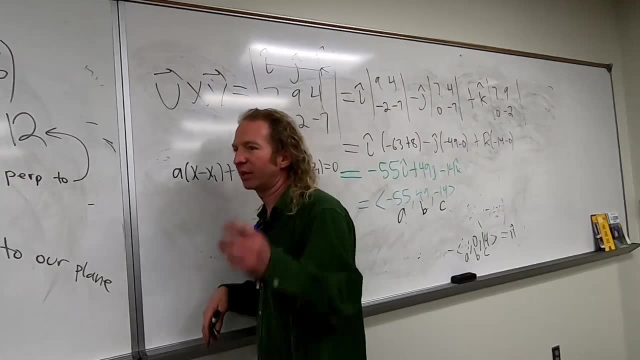 A, X minus X1, plus B. That way, when you go home, if you're looking at your notes, you have some understanding. There's a video for this one, too, already in the playlist in the Calc 3 one. 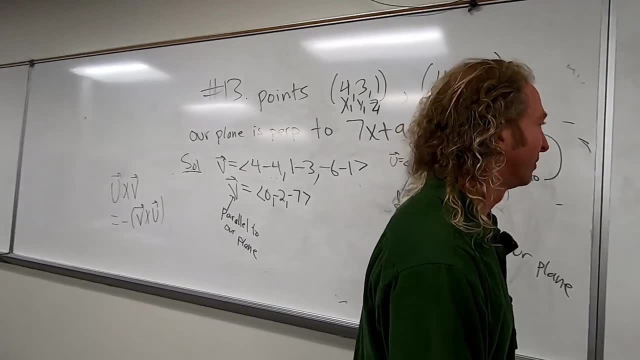 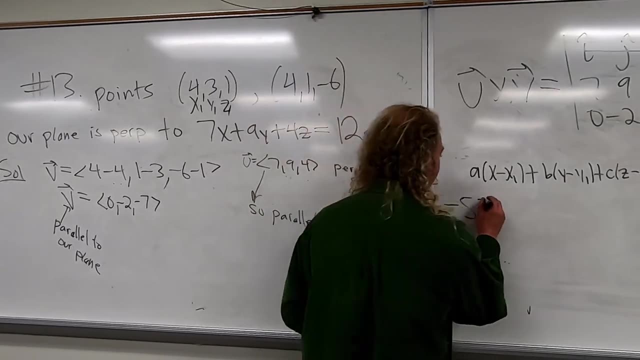 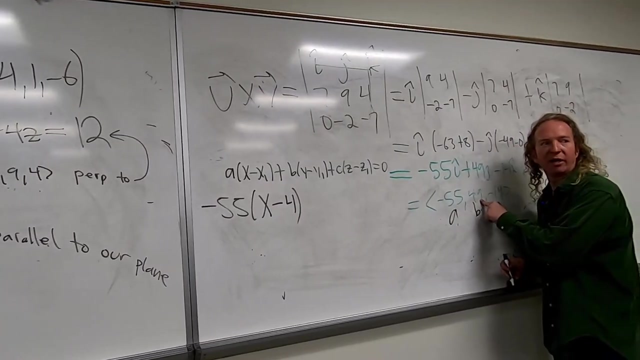 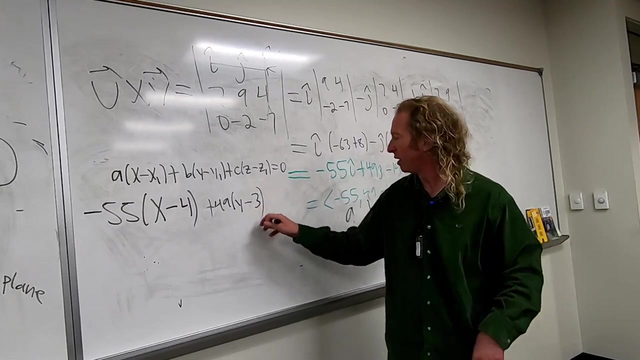 There's videos for all the hard ones already. This one already has a video, So yeah, it definitely does. Then A was negative 55. And X Minus 4.. B was 49. So 49. Y minus 3.. 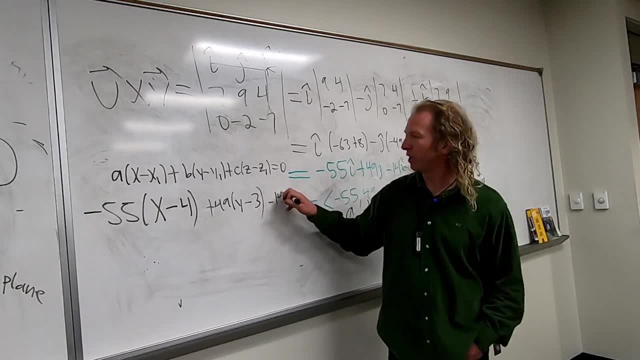 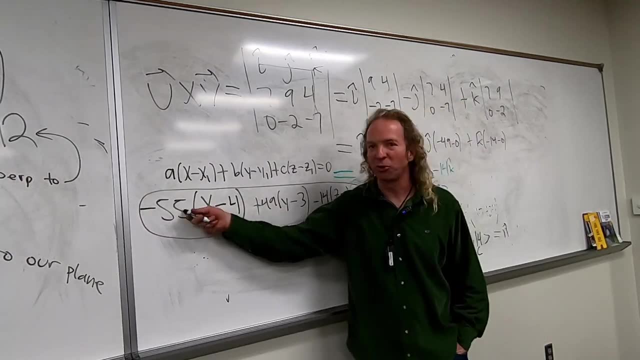 C is negative 14. So negative 14.. And then Z minus 1. And the whole thing is equal to 0. And just leave it like that. It becomes a lot more tedious if you multiply it all out, You know? hey, oh, you scared me. 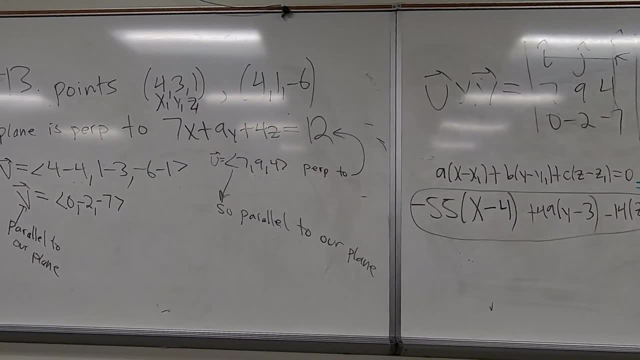 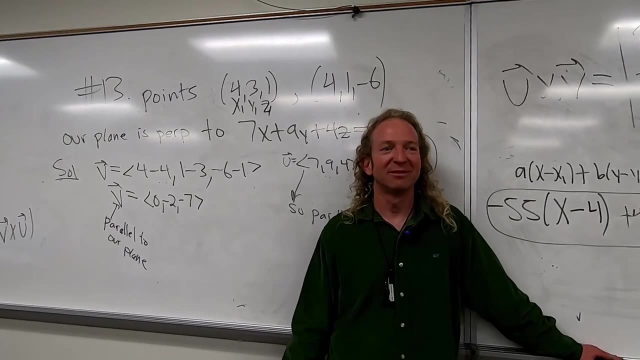 Creeping in. That's good, That's quiet. That's good, That's good. Any questions on this one? Is it harder, Rafael? Are you confused? No, It's pretty similar to the last one, But it's different though. 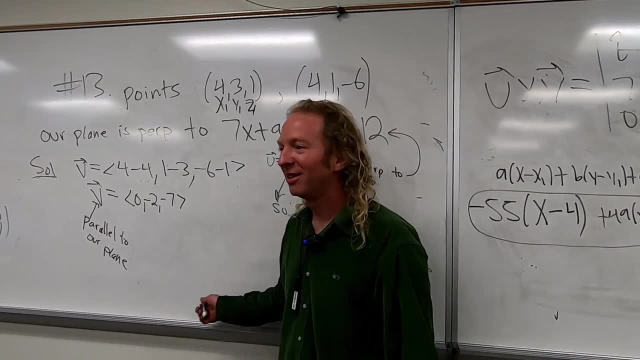 Yeah, it is. It is different. No questions on this one. If you had to do it again, could you do it on your own, you think? maybe This one Maybe A little bit. Do you want me to go over it one more time? 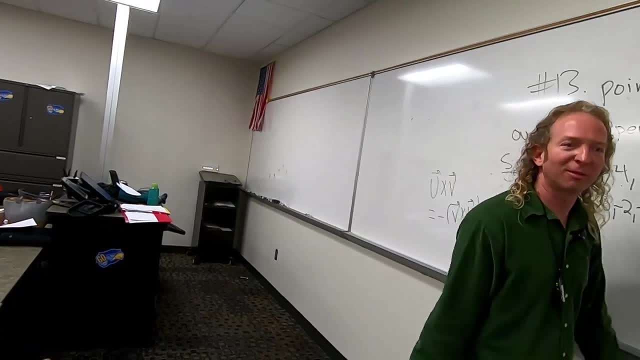 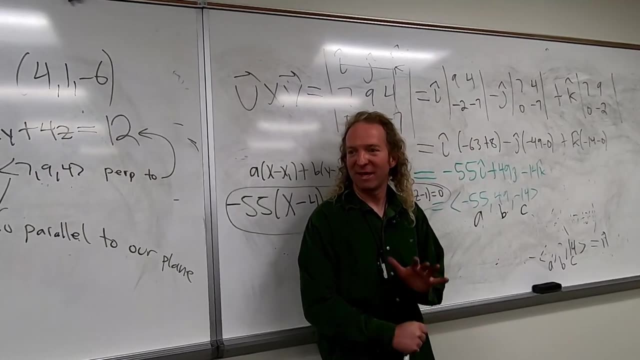 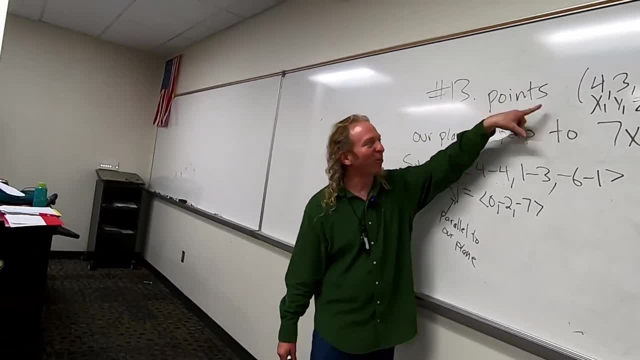 No, No, No, No. I don't want to go over the cross product again. No, All the computers say no. So the point: We have two points on the plane. So when we have two points on the plane, we can find a parallel vector. 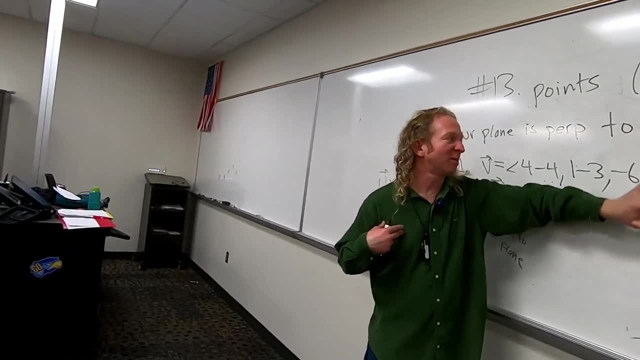 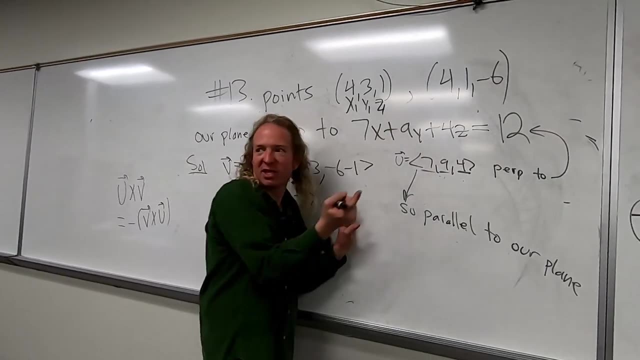 So we did that. So our plane is perpendicular to this. So pretend that this is the board. So our plane is perp-to-it And this vector here is always perp-to-this plane. Why? Because it is right, It's the form of the ABC. 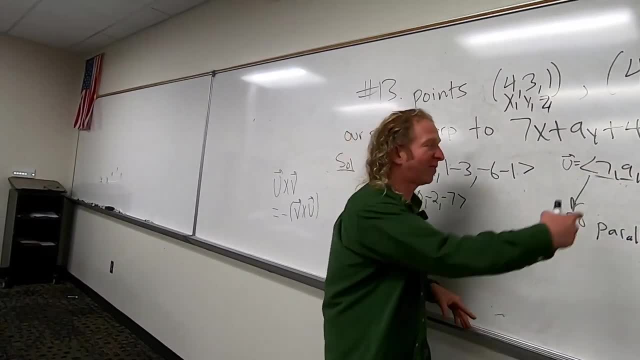 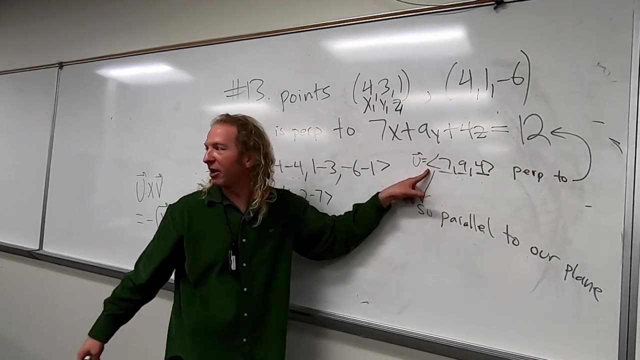 These numbers here will always give you a vector that's perp-to-this plane, Always. So this vector is perp-to-the-plane plane is perfect. the plane, therefore our plane, is parallel to this vector. so you have a parallel vector, a parallel vector. take the cross product, you get a normal. 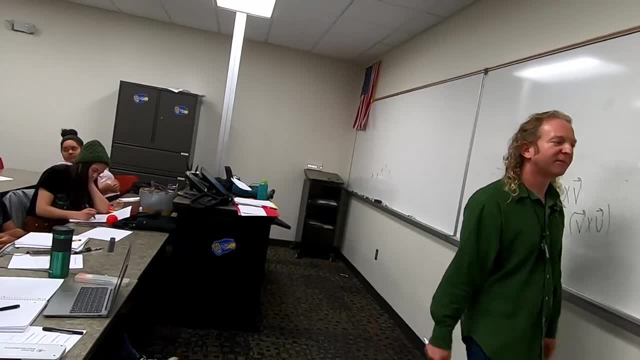 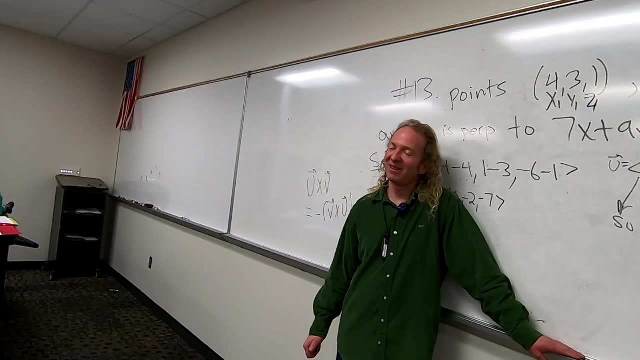 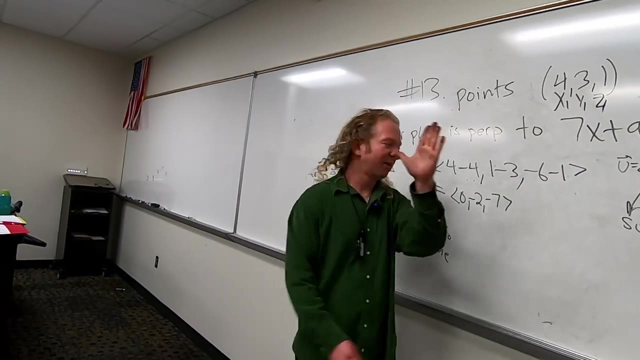 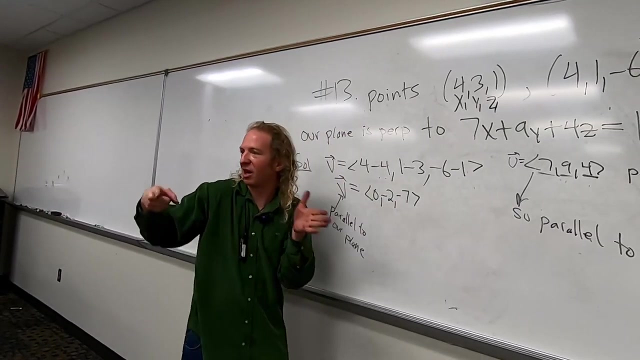 vector done. yeah, you sure, oh, okay, yeah, well, okay, so if this is the plane, the board the plane right. so this is the plane, this is our plane, my hands are playing, this is the vector, they're both perp, so they're parallel. yeah, so yeah, because, like, if you're the plane and my hands perp to you, my fingers perp to you. 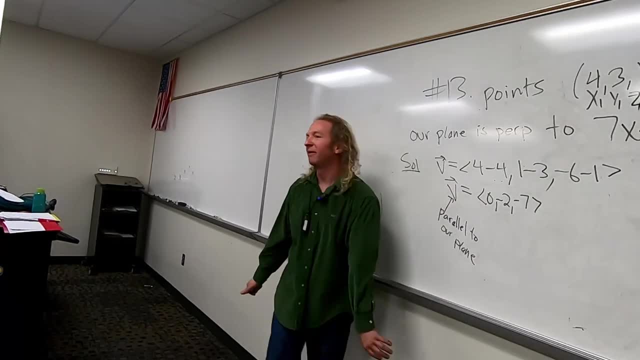 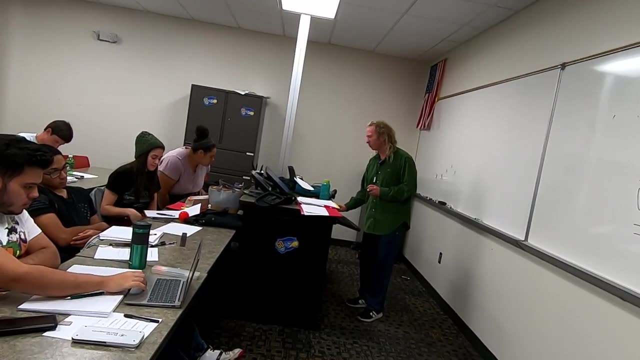 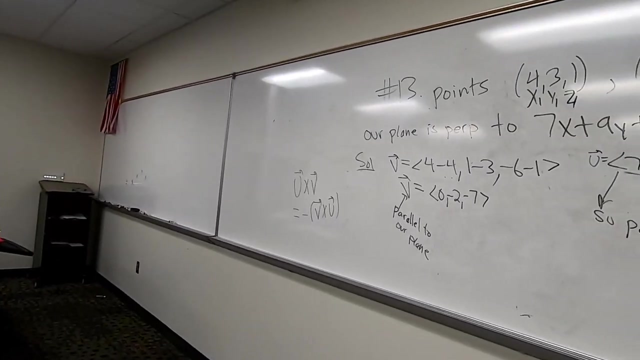 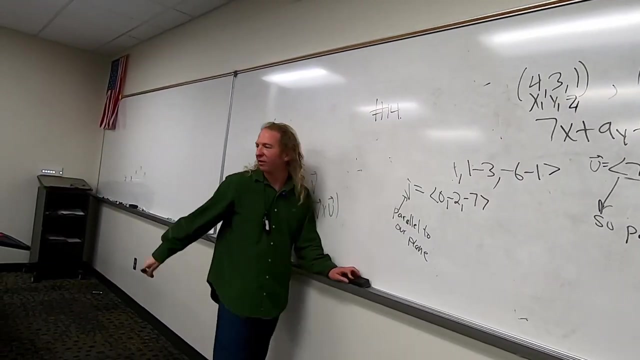 they're both parallel. yeah, same thing. yeah, yeah, all right, let's do the last one. right, the very last one: 14, because 15 is kind of weird. I will do that one later. it's really easy. 14, 14, 14. so 14- they give us something else, so 14, they give us two points. and these points. 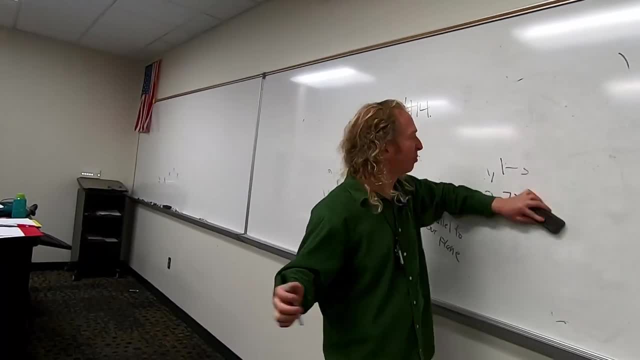 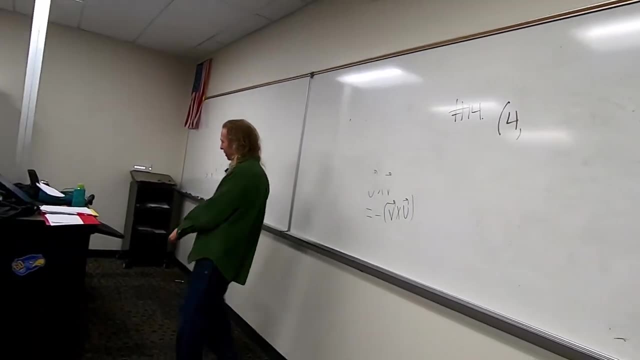 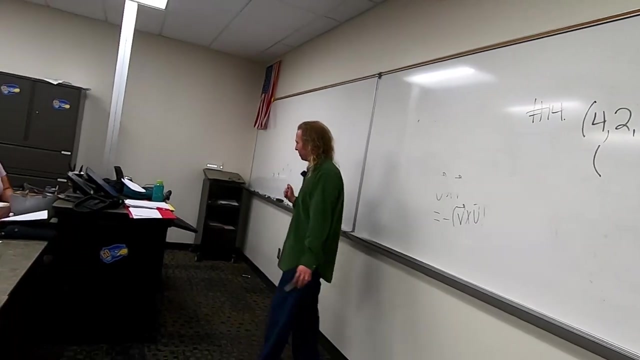 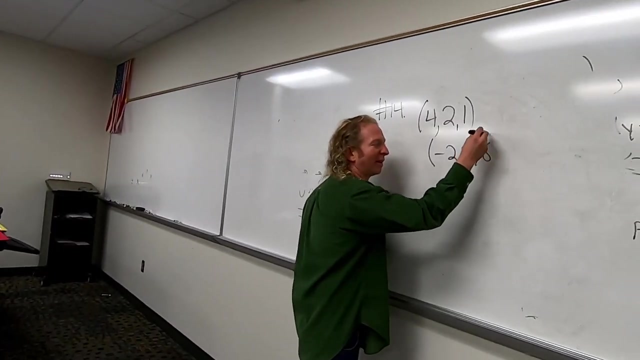 are on the plane, so the plane passes through these points. that means these points are on the plane, so the points are four to one, to one and the other point is negative. what really the points are always on. yeah, they are you. yeah, I think they always are. yeah, yeah, yeah, be really weird, like, yeah, I'm gonna test. 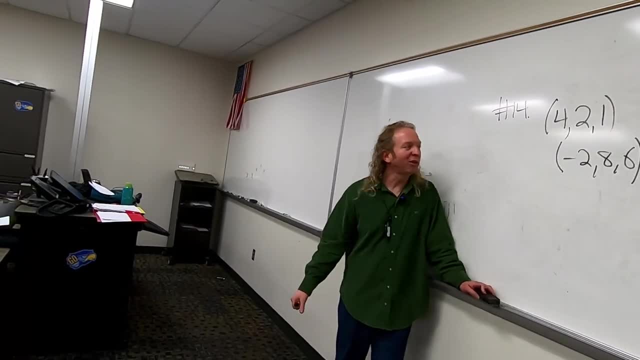 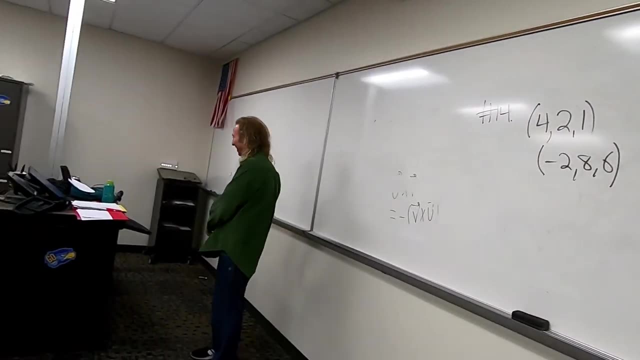 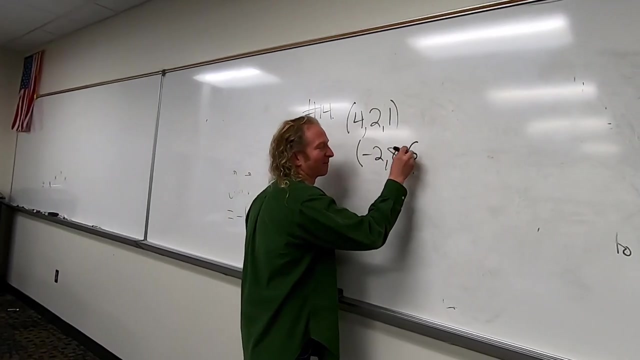 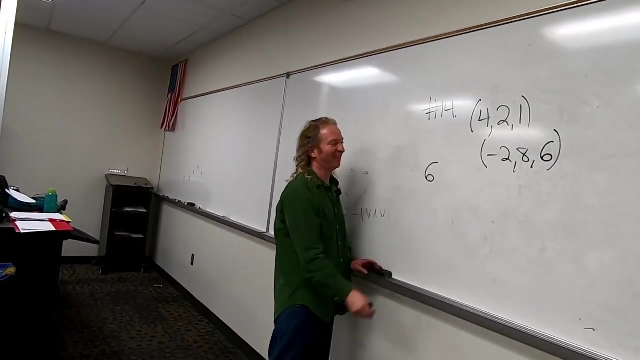 the. the point is off the plane, the point is on the moon, 500 kilometers from the plane. use the force of gravity. yeah, this, this, that's six. sorry, what curve. oh, that, that, that, that, that, yeah, wow, that takes a lot of effort, that's like. and they tell us it's parallel to the z-axis, so I'll. 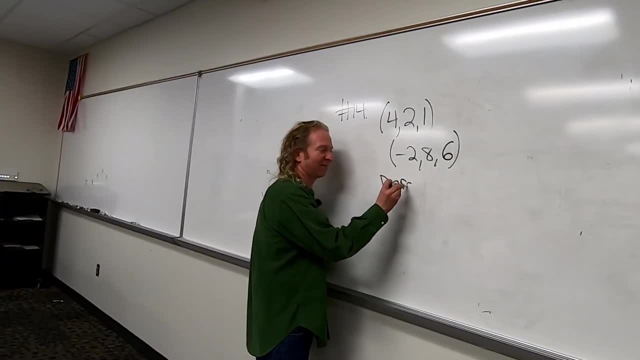 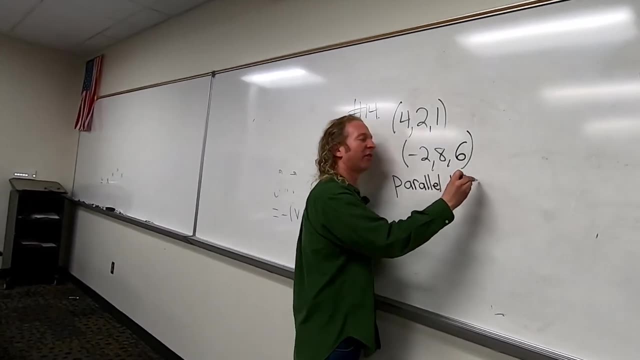 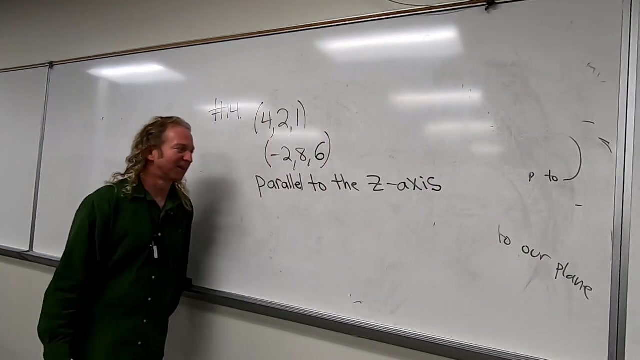 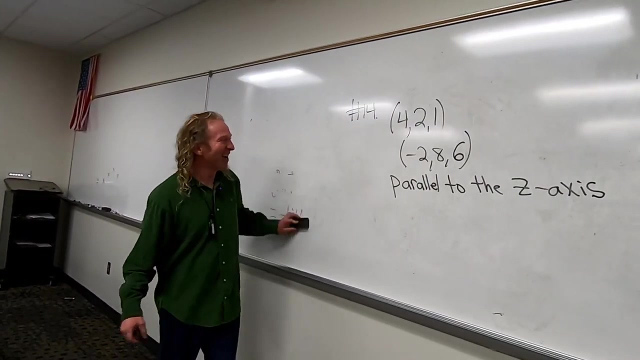 try to write better. look, I can write nice parallel to the z axis. no, come on. come on. no, try it so hard. I walked into this teacher. She doesn't teach here anymore. I walked into her class once. She needed me to do something. 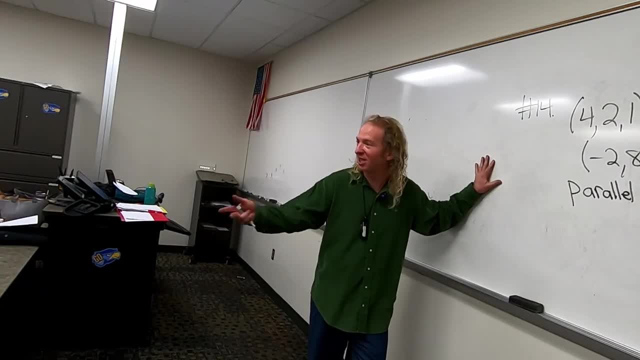 I forgot what it was And she gave me a Starbucks gift card because I did it. But anyways, I went to her class. Oh, I subbed for her for like 30 minutes And I walked in And she had such good handwriting. 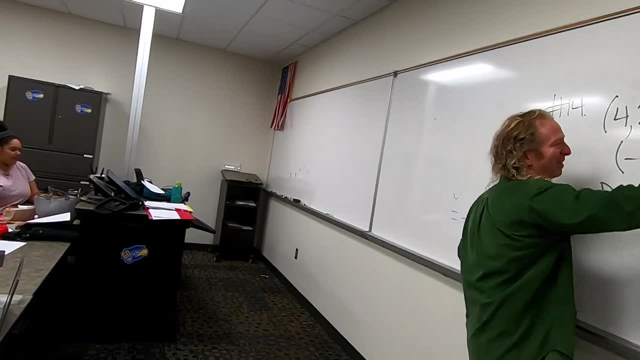 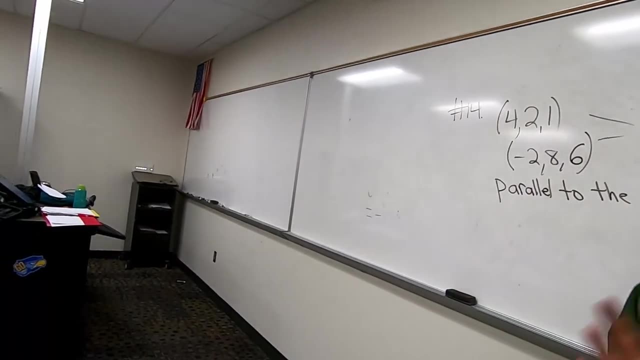 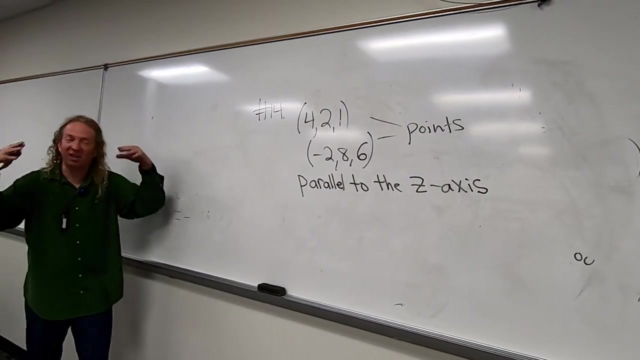 I felt like I just can't compete. All right, this is terrible. All right, so we have two points. What can we do when we have two points? What can we find? What kind of vector, Parallel? yeah, So it comes up again and again. 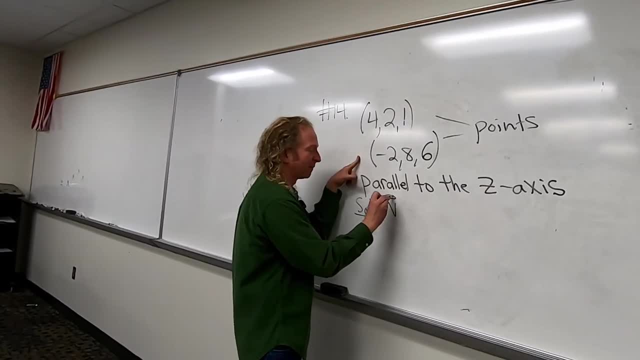 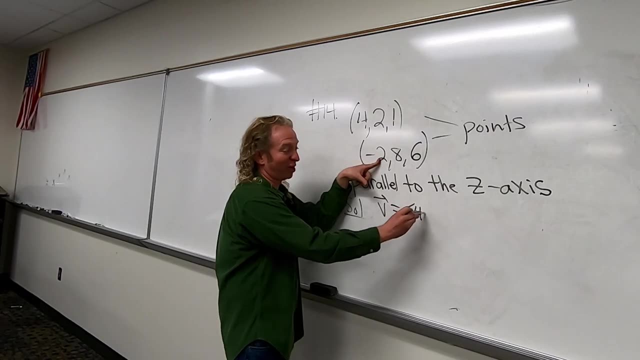 So solution. So let's do that first. But even before we read this, So V, So I do. oh yeah, there's a negative there, But we can handle it. 4 minus negative 2 is 4 plus 2.. 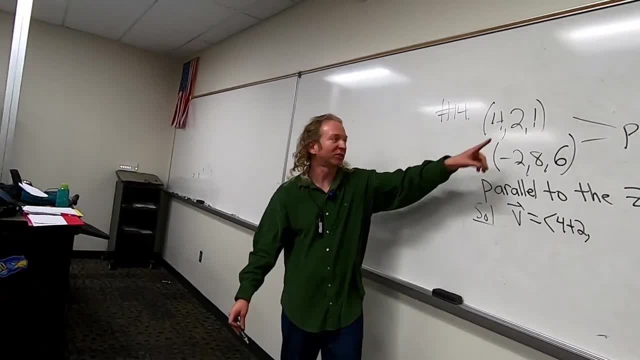 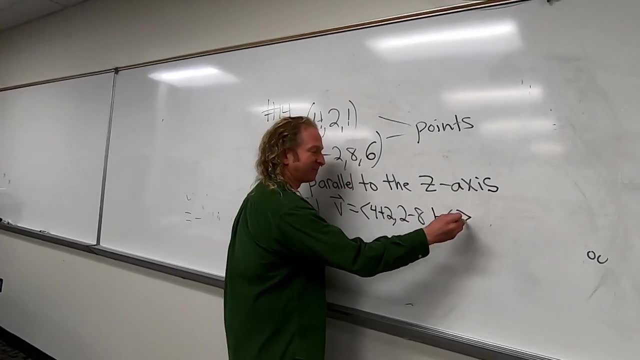 No, it doesn't. No, it doesn't. I just want to start with. this is easy. So yeah, 2 minus 8, 1 minus 6.. So V. So 4 plus 2 is 6.. 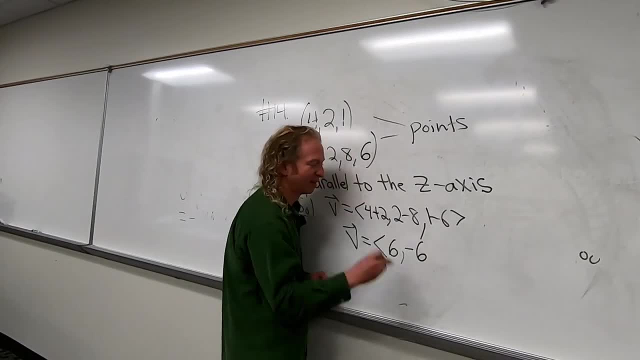 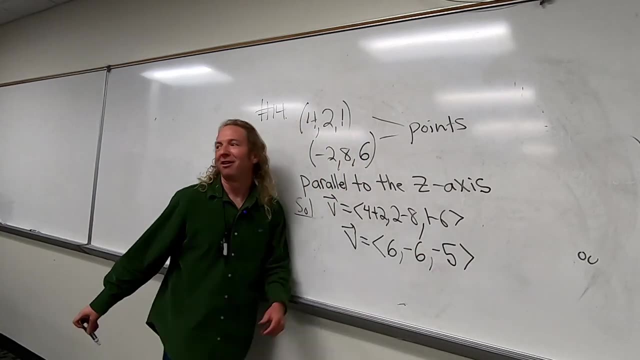 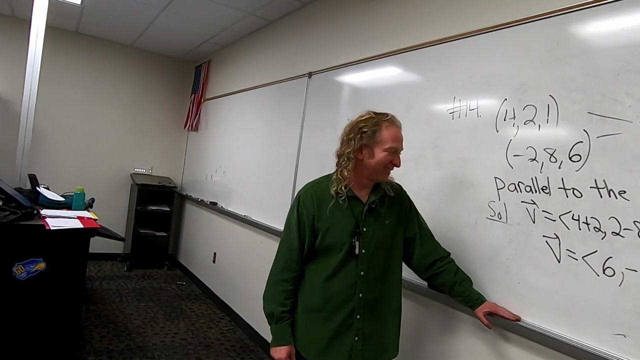 And then we get negative 6. And then 1 minus 6 is negative 5.. Trying hard, There's that curve. Look at that. Those are fancy 6's. That's pretty cool. Okay, so this is parallel. 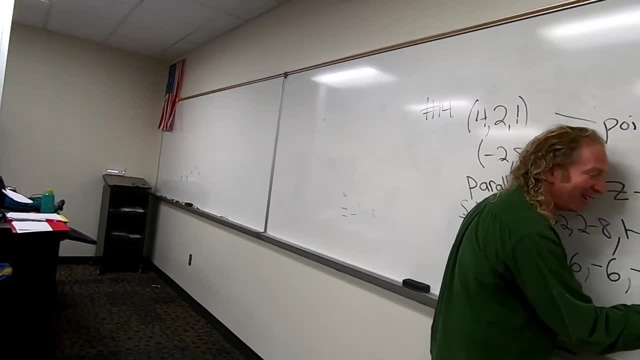 This is parallel. I know I'm all into it now. This is parallel. This is parallel to our vector, right To our plane, To our plane, Sorry, to our plane. I don't even know what I'm saying. 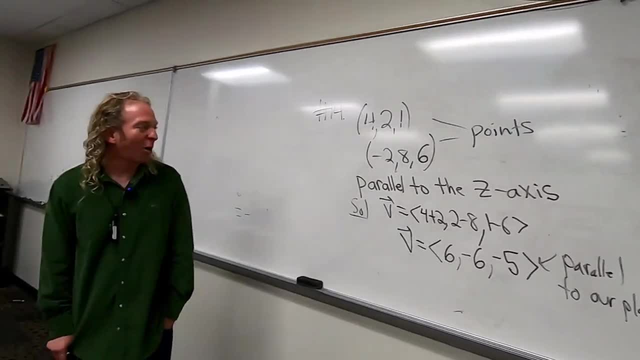 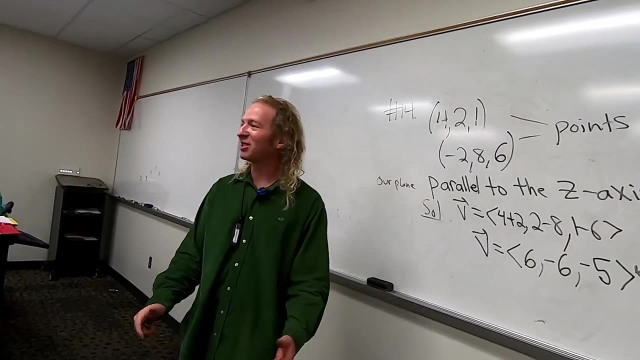 It's parallel to our plane. We're also told our plane is parallel to the z-axis. Our plane, Hardcore. That has another name. What's that called K-hat? Yeah, k-hat. So our plane is parallel to the z-axis. 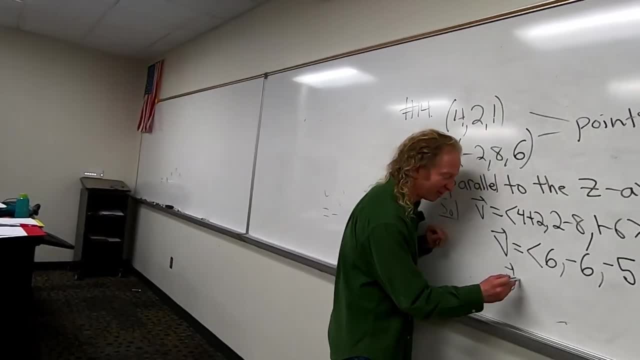 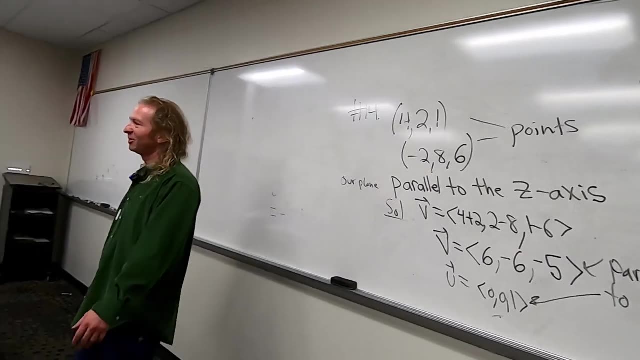 That means it's parallel. So our other vector, We'll be 0, 0, 1.. This is parallel to our plane Right, Because that's k-hat, That's k-hat, Hardcore Wudash. 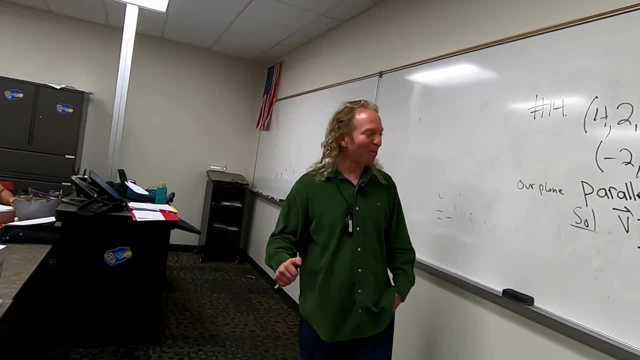 That was a big. that was pretty slick. That's what statics does. It's a moment of brilliance Or no, just brilliance. They're just really good. That's really good. You do this in statics a lot, Yeah. 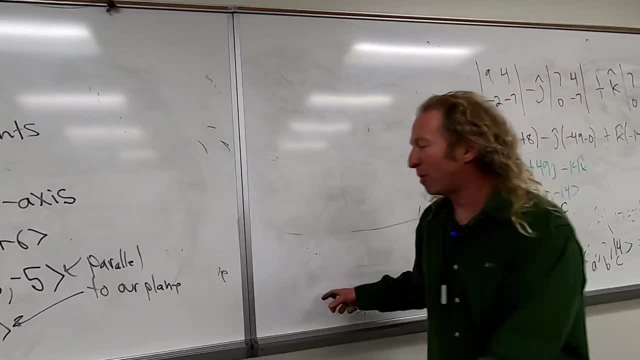 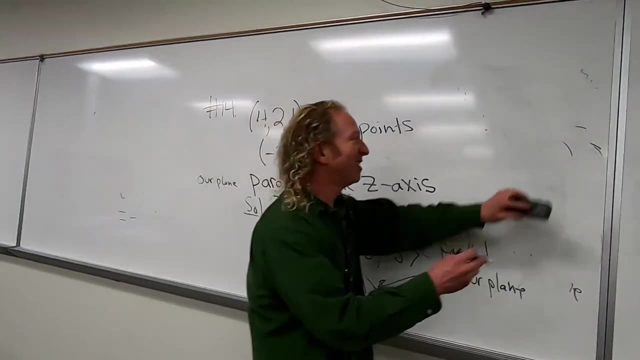 Yeah, it's pretty hardcore, It's good. So we have two parallel vectors. How do we find a normal cross product? That's it. So now let's take the cross product of these things: So v cross u, So v cross u. 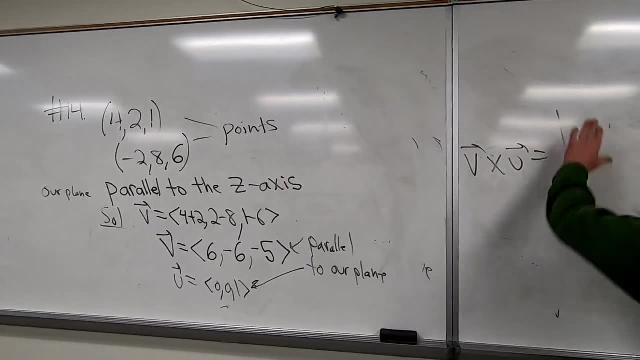 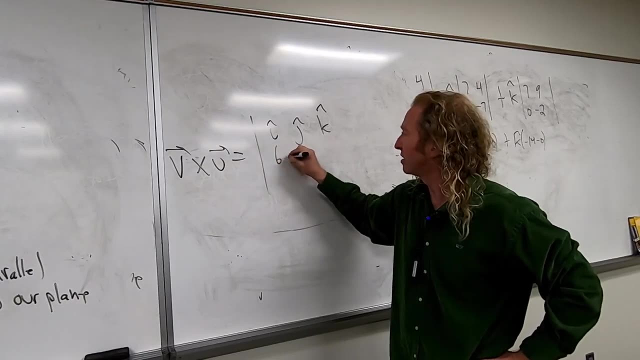 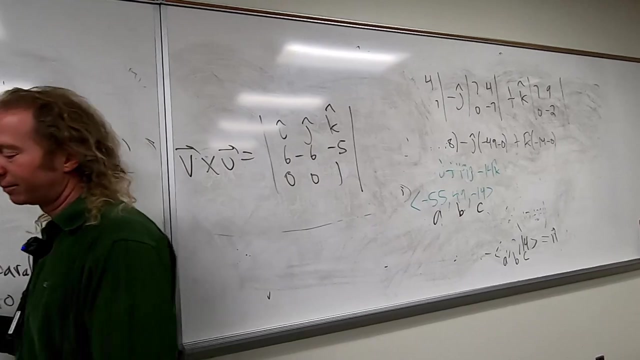 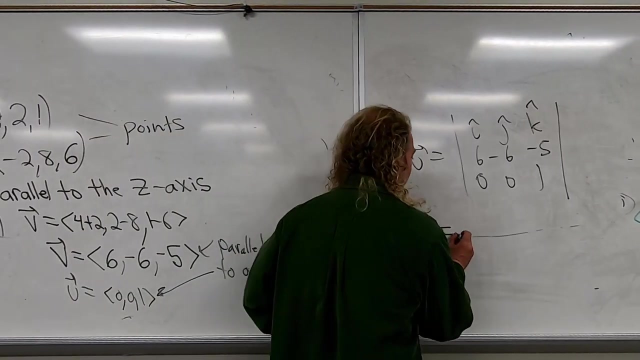 So we have i-hat, j-hat, k-hat. So v is 6, negative, 6, negative, 5. And u is 0, 0, 1.. So now we can just find this. So we have i-hat. 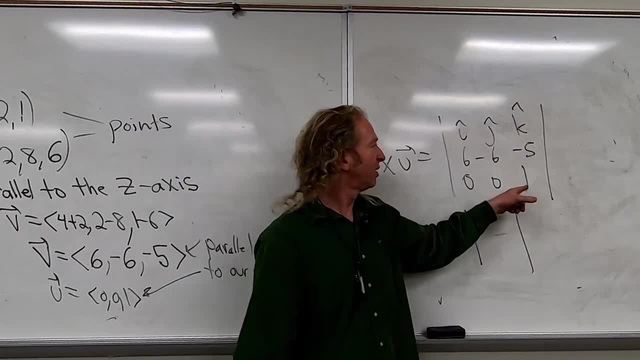 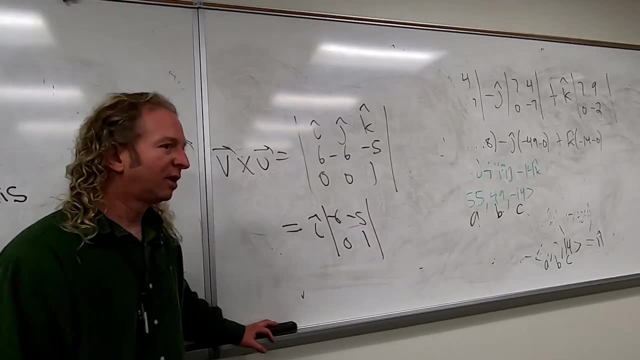 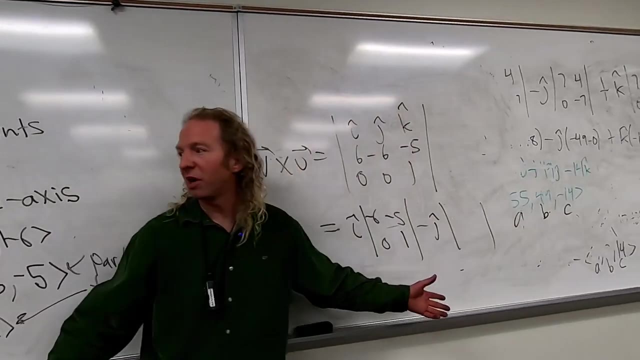 So we cross the corresponding row and column out right, So it'll be negative 6, negative 5,, 0, 1.. And then minus, minus j-hat, right Minus j-hat, And cross out the corresponding row and column. 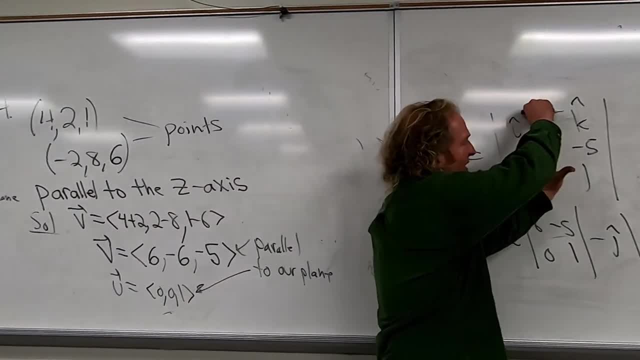 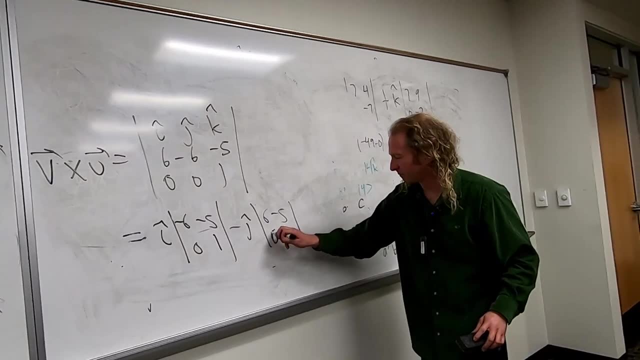 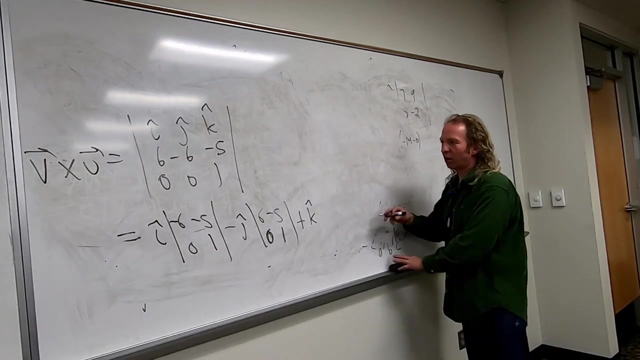 So that would be 6, negative 5, 0, 1. 0, 1. 0, 1. Plus k-hat, Plus k-hat. So we cross out the corresponding row and column. So cross these out. 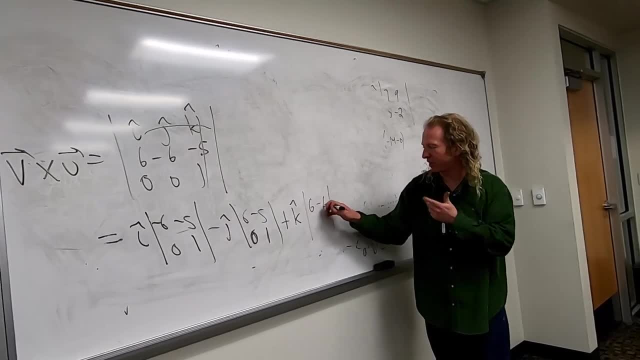 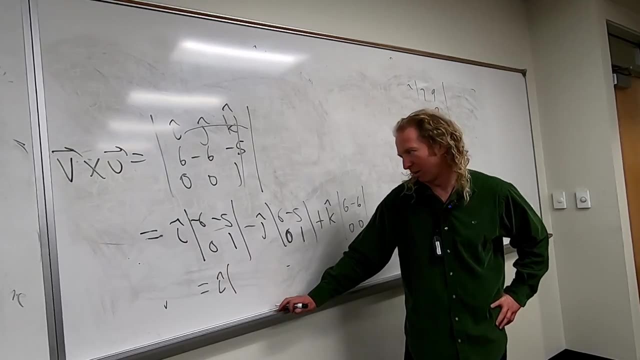 So we get 6, negative, 6, 0, 0.. So 6, negative, 6, 0, 0.. So this is going to be i-hat. We've done a lot of cross products today. Negative: 6 minus 0, minus j-hat. 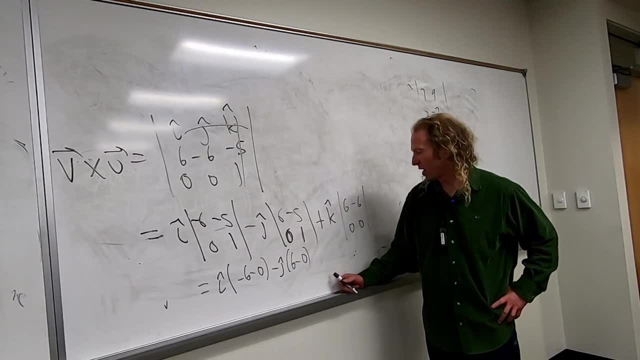 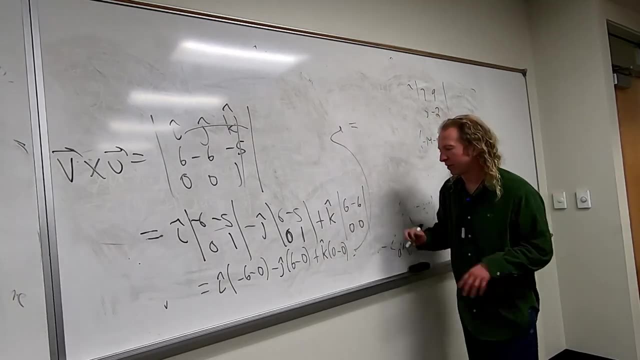 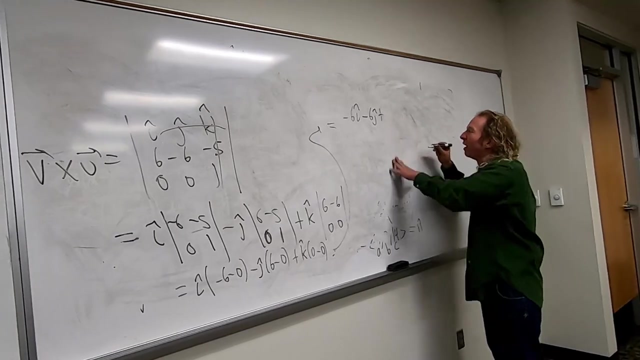 6 minus 0, right, 6 minus 0.. 0,, 1.. 0, 1. Plus k-hat times, 0. 0 minus 0.. So it's going to be negative: 6 i-hat minus 6, j-hat plus OK. 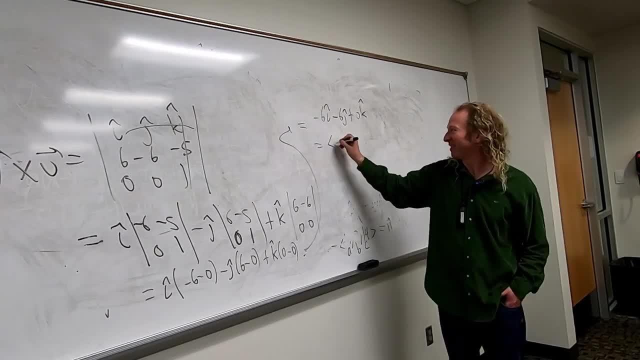 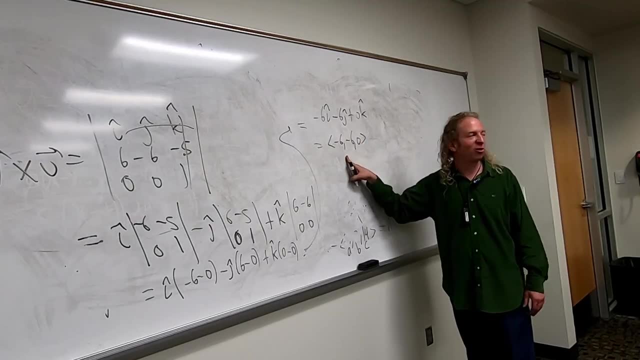 Doesn't it spell? OK, I love that. So this is negative 6, negative 6, 0.. What is this? What is this? N? N. This is our normal vector, right? This is our normal vector. This is our ABC, right. 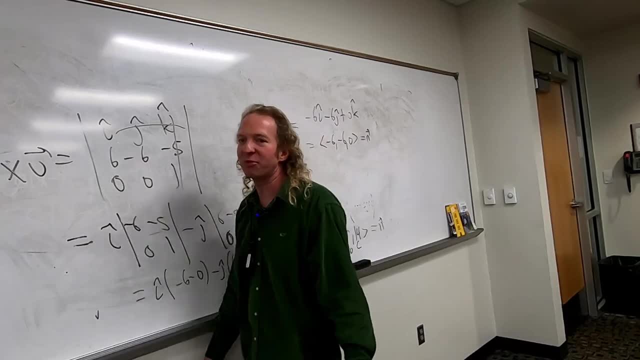 This is our N. This is our N. I'm becoming plane masters. You do all these problems. you can do any plane problem. It's like it's ridiculous. We did every single one, So now we'll finish right. 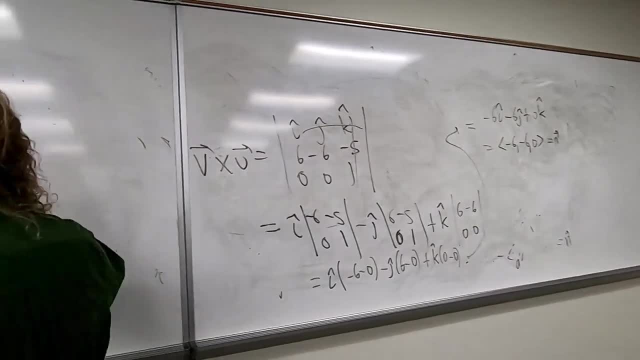 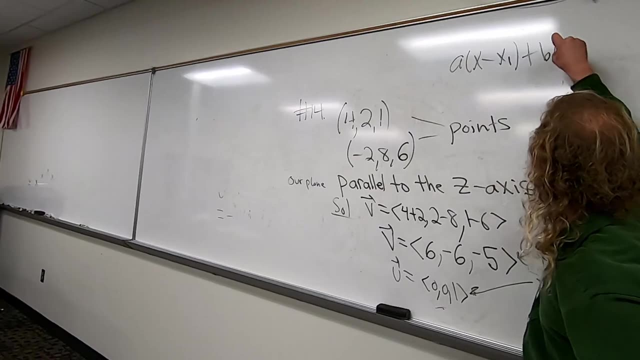 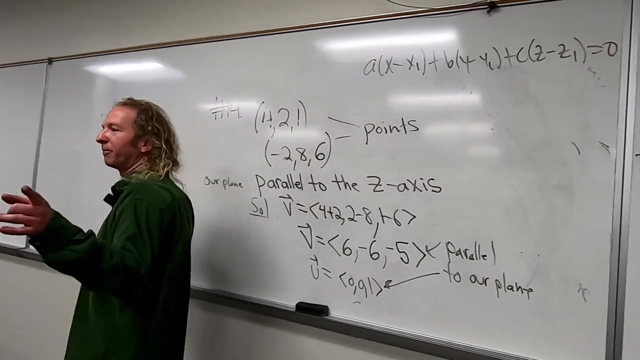 Now we'll plug it in to the formula. I'll come back over here. So the formula was ABC. So it's A: x minus x1 plus B, y minus y1 plus C, z minus z1 equals 0. That's the formula for all the problems, right? 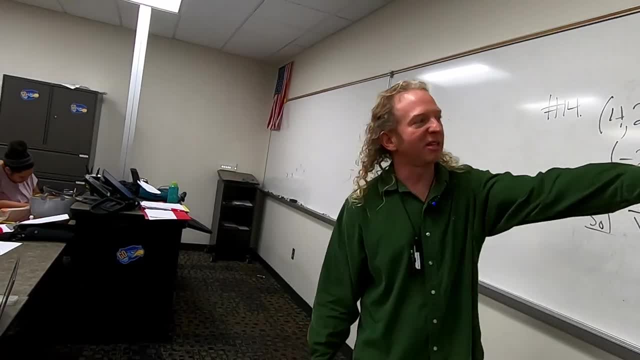 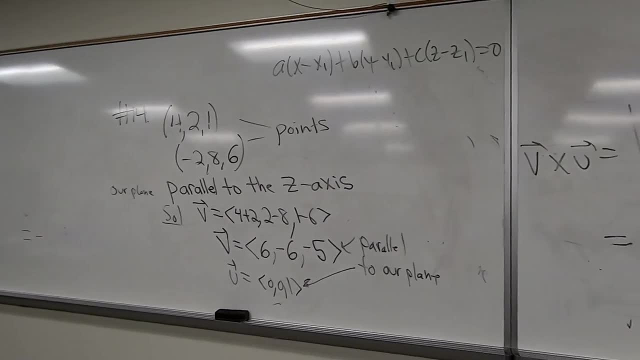 For all of them. And then, And then your ABC. it's those numbers over here, right, This is your ABC. So A, B, C, So it'll be negative 6. And then I guess we can use any of these: 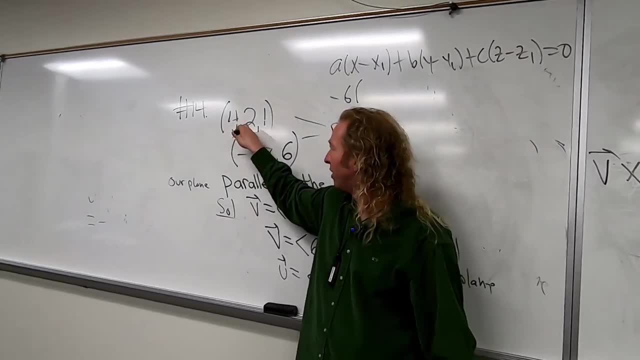 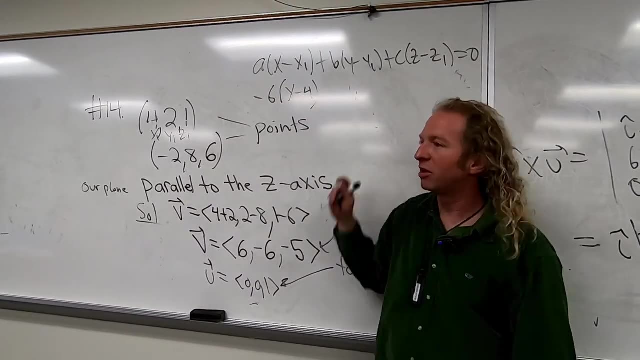 It doesn't matter which one we use, right? So I'll just go with this one here. So this is x1, y1, z1.. So it'll be x minus 4.. B was what was B Negative 6.. 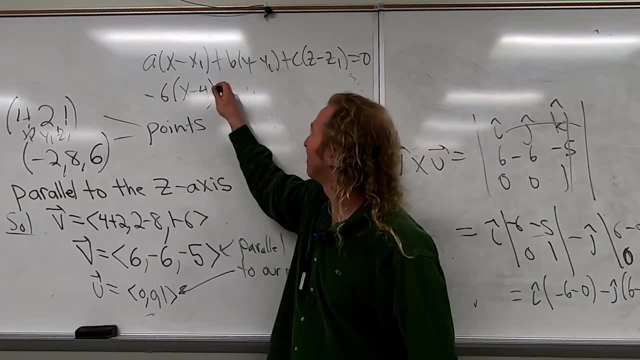 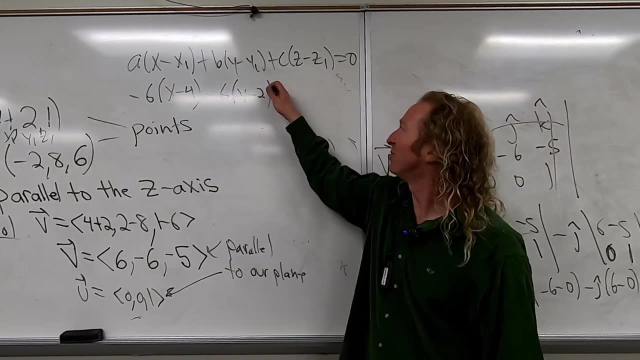 Negative 6?? OK, now, I believe you. now Negative 6, y minus 2.. And then C was 0, right, Yeah, Trust equals 0. And that's it. That's it. We finished all of the plane questions. 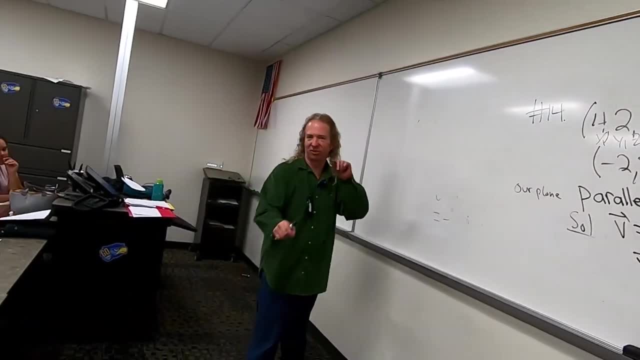 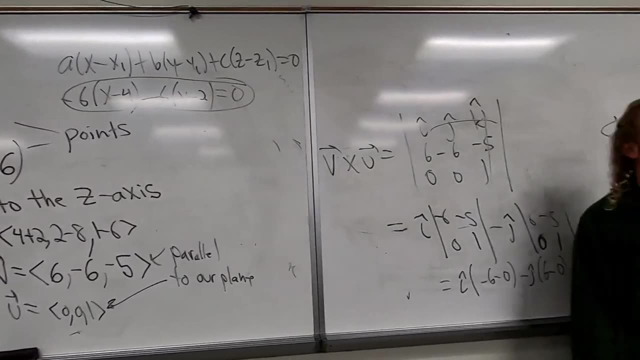 There's one more in the homework, but I'll show you how to do it later. It's really easy. It's easier to bring it down and show you. It's graphing a plane. It's really easy. So just plug in numbers and it works out.